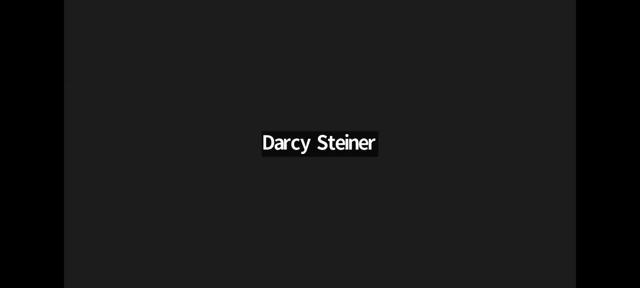 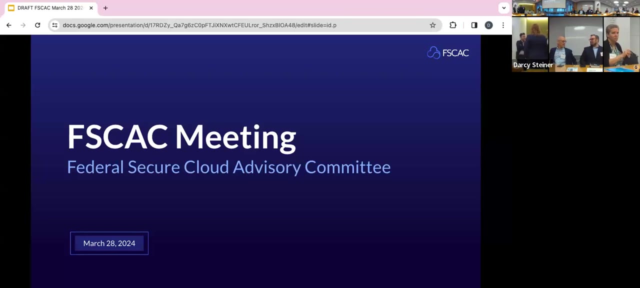 Thank you, Thank you, Thank you so much. Welcome to March 28th 2024.. It's the meeting of the Federal Security Advisory Committee, ASCAP. My name is Michelle White and I'm the designated public officer, or DFO, for this advisory committee. 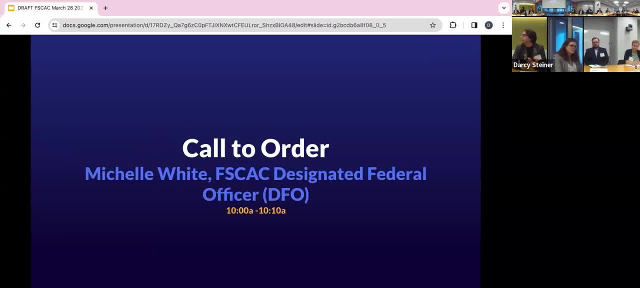 I would like to thank all of the presenters, attendees and stakeholders for joining us today, including those who provide public comments. Public comments that were submitted via the ASCAP public comment form by last Wednesday, March 20th, have been provided. 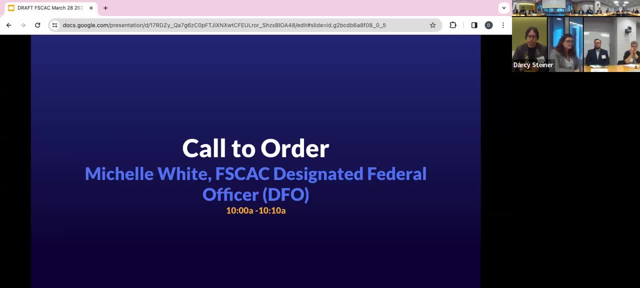 to the committee members. Before we start, there are a few things that you should know. This meeting is being live-streamed and reported via Zoom. The advisory committee is statutorily required under the James N Inhofe National Defense Authorization Act for fiscal year 2023. 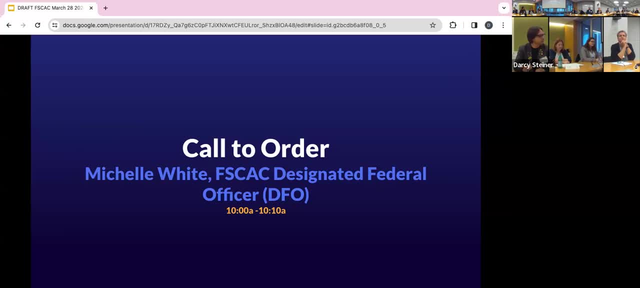 and thus formally established under the Federal Advisory Committee Act, or FACA, as of our charter's official filing date of February 28th 2023.. This committee is considered a federal advisory committee and is governed by the requirements under FACA. 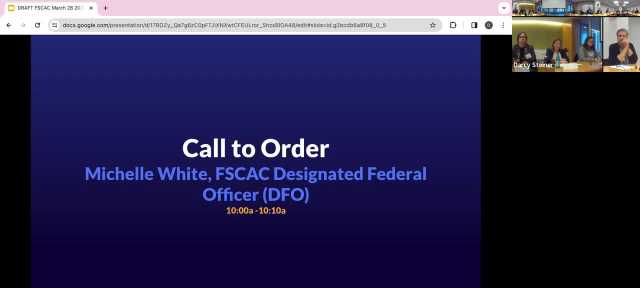 My role as the DFO is to manage the day-to-day administrative operations of the committee, attend all committee meetings and ensure that the committee operates in compliance with FACA. The duties of this committee include providing advice and recommendations to the GSA administrator. 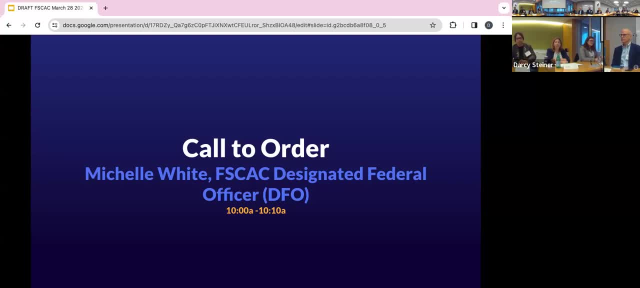 the FedRAMP board and agencies on technical, financial, programmatic and operational matters regarding secure adoption of computing products and services. The majority of the work of this committee are focused around the Federal Authorization Act of 2022, which includes statutory requirements. 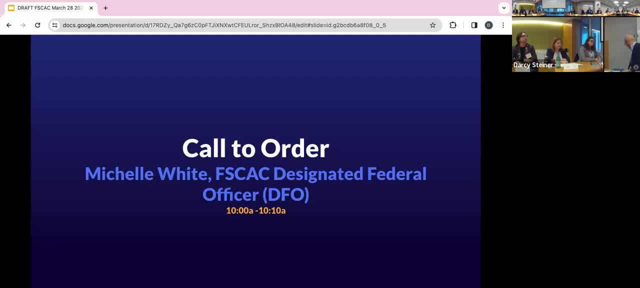 and purpose. Specifically, we examine the operations of FedRAMP and determine ways that the authorization processes can be continuously improved, collect information and feedback on agency compliance with and implementation of FedRAMP, and serve as a forum that facilitates communication and collaboration among the FedRAMP. 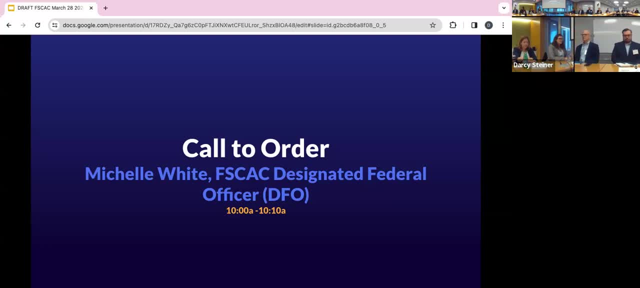 stakeholder community. I will now go to a roll call for all committee members. Please let me know you're present by stating: here Ann Lewis. Here Daniel Payne. Here Michael will be a second Here John Beasley. Here. 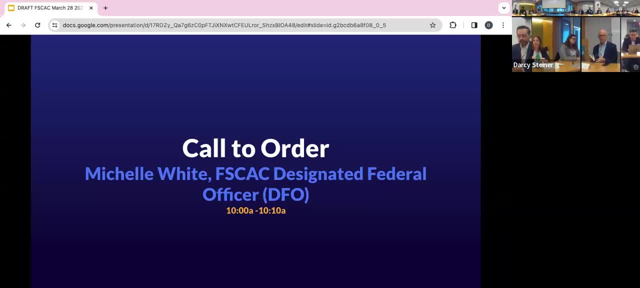 Marcy Womack Here Bronco Volcan, Present Matt Schull Here. Bo Gervas Here Lamont Yarbrough, Here Nauman Ansari, Here Jackie Snopper, Here Bill Hunt. 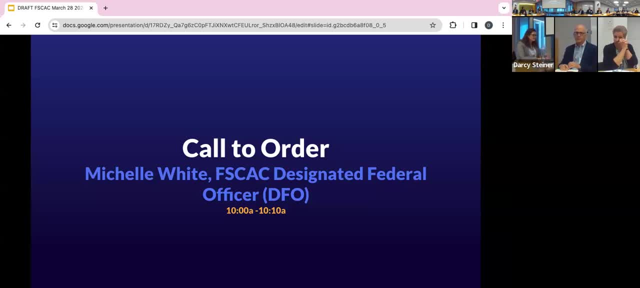 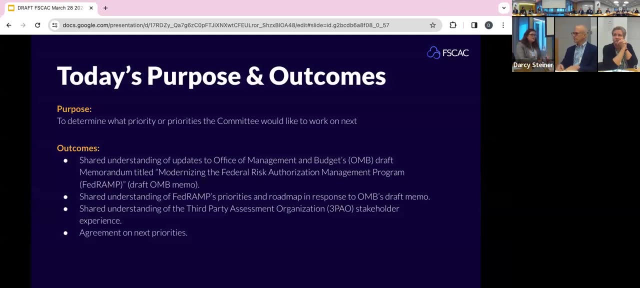 Here And Joshua Cohen Here. All right, Thank you all. It looks like we do have a forum established. I will now go ahead and review some background from our last meeting: the purpose, outcomes and agenda for today's meeting. 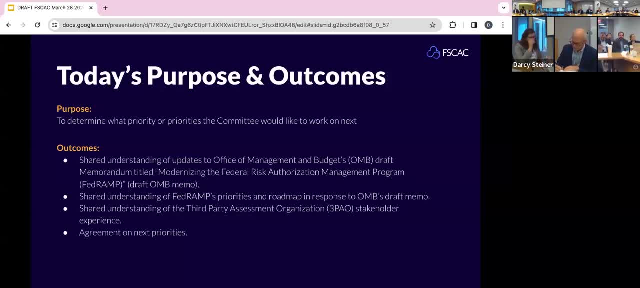 and just for everyone's awareness, After our January 18, 2024 meeting, the committee approved their top actionable recommendations on their initial priorities of the authorization process improvements, continuous monitoring or common process improvements and automation opportunities and initiatives. The chair drafted an executive summary. 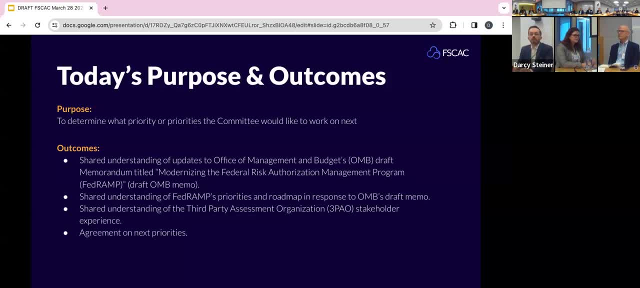 based on the committee's recommendations and delivered the memo to the GSA administrator on Tuesday, March 5, 2024.. This final deliverable is available on our website. So, therefore, the purpose of today's meeting is for us to have to determine what priorities. 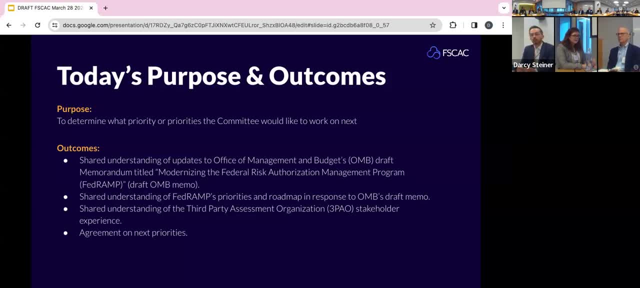 or priorities the committee would like to work on. next, The committee has requested specific presentations for today to include an OMB memo update, FedRAMP's response to those updates and more information from the 3PO experience By the end of this meeting. 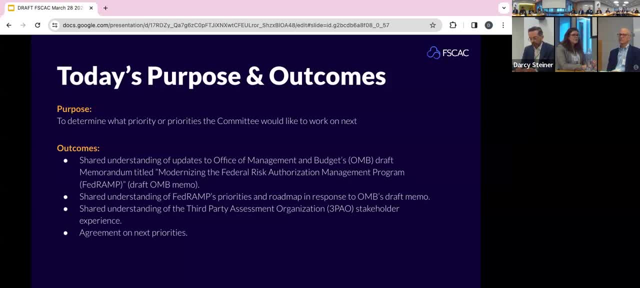 we should all leave with an understanding of what the committee's next priorities are, or additional information the committee needs in order to determine those next priorities, To support the development of our priorities. we will also be briefed on updates to the OMB draft memorandum entitled. 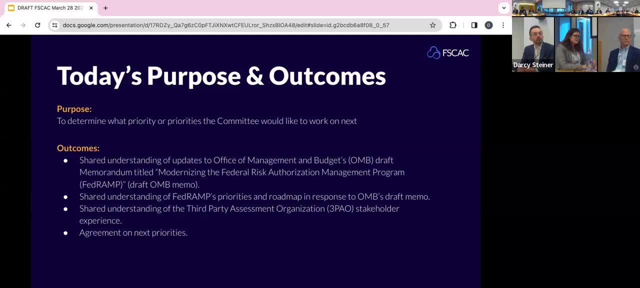 Modernization of the Federal Risk Authorization Management Program, FedRAMP. It's a draft OMB memo: FedRAMP's priorities and roadmap in response to OMB's draft memo. The third-party assessment organization, or 3PO, St Colbert Experience. 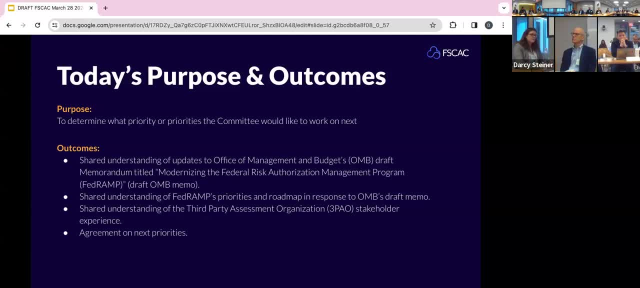 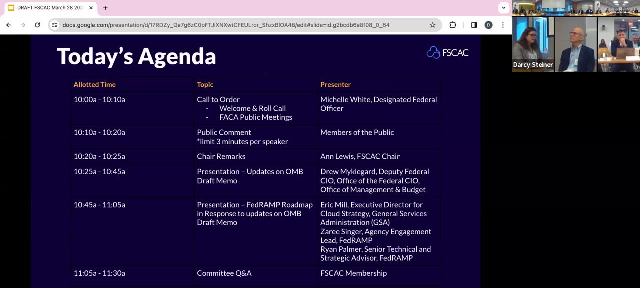 and again we'll leave with an agreement on what EPSCAC's priorities will be. So, as you can see, our agenda is listed. We're doing the call to order now. We will first have our public comment. our chair remarks. 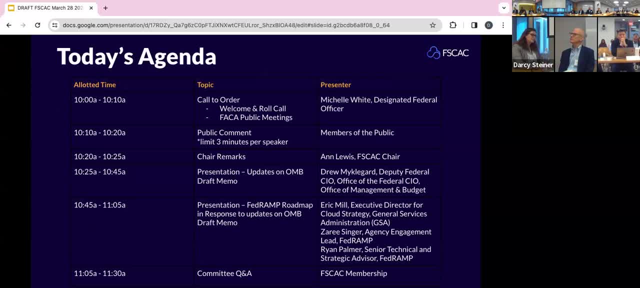 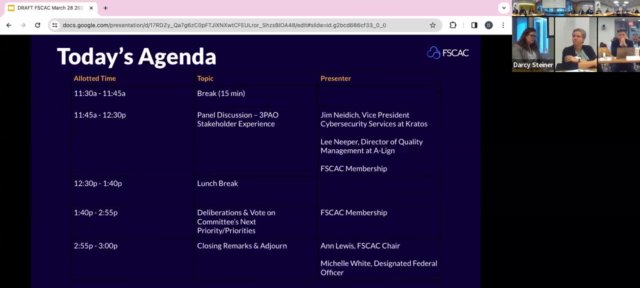 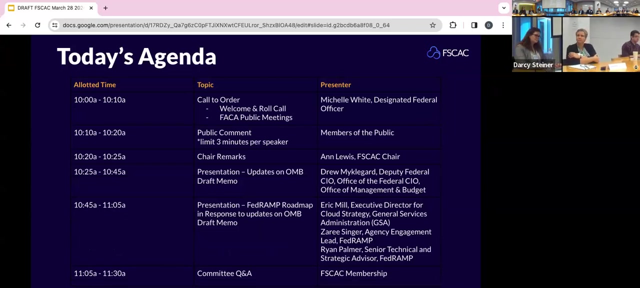 and then we will have an OMB update from juvenile regard and a presentation from FedRAMP on their roadmap and response to the draft memo, Draft memo being the one that we sent The response to the draft. no, the OMB draft memo on FedRAMP. 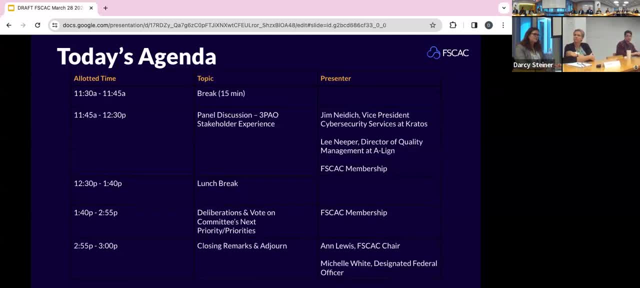 And then we'll have our 3PO stakeholder experience discussion at 11.45.. We do have some breaks scheduled in here for you know, just a break to break things up. And then we have our lunch break from 12.30 to 1.40 today. 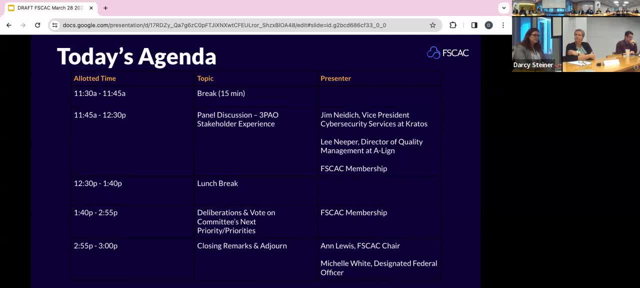 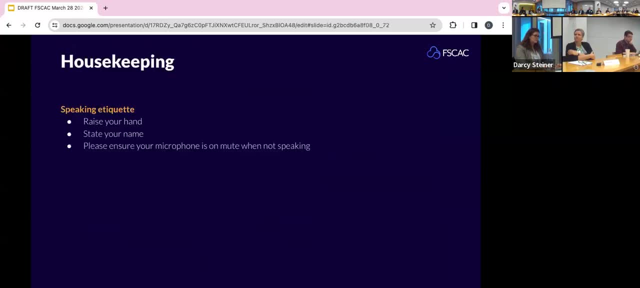 From 1.40 on, we will be deliberating and voting on our next priorities And then, finally, we'll have our closing remarks and close up at 3 o'clock. Few more housekeeping items for the committee members. We have a lot of presentation. 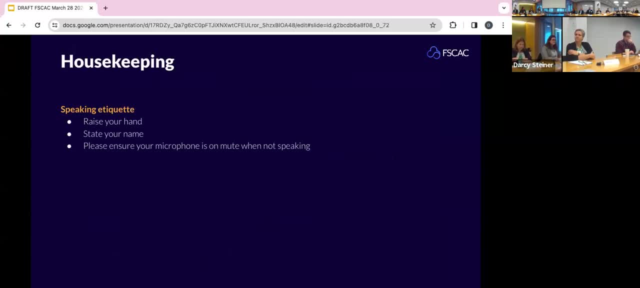 and discussion scheduled for today. Unless otherwise requested by our speakers, please hold your questions until the committee Q&A portion of the agenda. If you have a question during the discussion, please raise your hand and you will be called on based on the order you are in the queue. 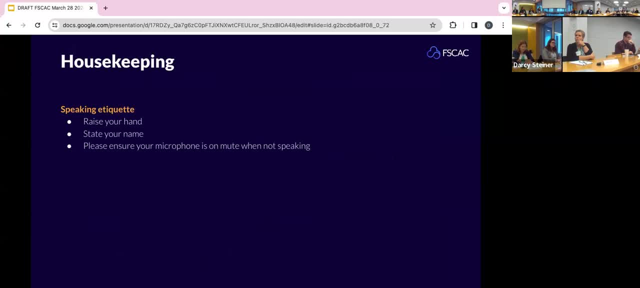 Again, please identify yourself before speaking So those listening via the webcast or reading the minutes after the meeting will know who made which comment. And finally, if you are not a committee member, please hold all comments until the public comment period, which actually is now. 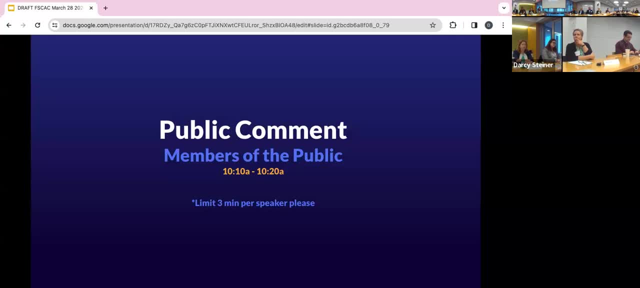 So we'd like to go ahead and invite the public that is in person today to share their comments. Your speakers, please note that there is going to be a timer displayed on the screen indicating your time remaining, and the alert will indicate you were out of time. 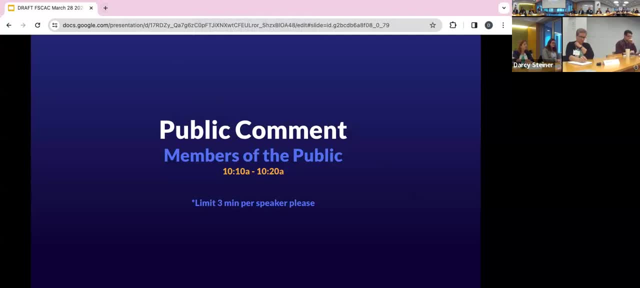 Each speaker is allotted three minutes to make their comments. We will be interrupting speakers that exceed three minutes, so please speak succinctly and please be respectful of the time. As a reminder, all public comments submitted by Wednesday March 20th were presented to the committee members. 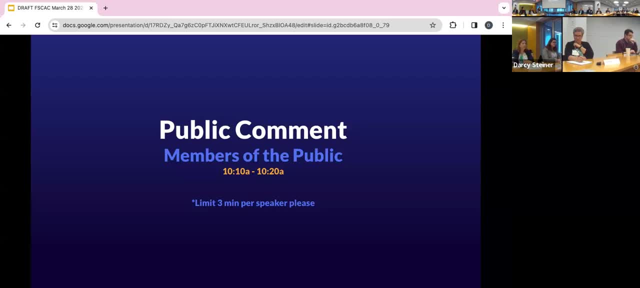 prior to the meeting. And with that, please go ahead and raise your hand if you'd like to provide a comment, and I will call on you to speak in the order in which your hand was raised. And once I call on you, please step to the podium to speak. 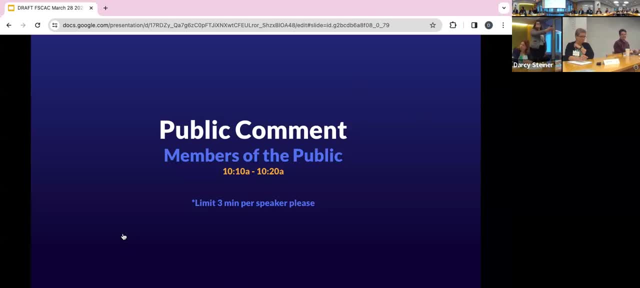 Yes, sir. Please come to the podium so that the webcast can hear and see you. Good morning, My name is Josh Blair. I'm part of the FedRAMP team at Red Hats and I'm here today to offer input on what Red Hat meetings. 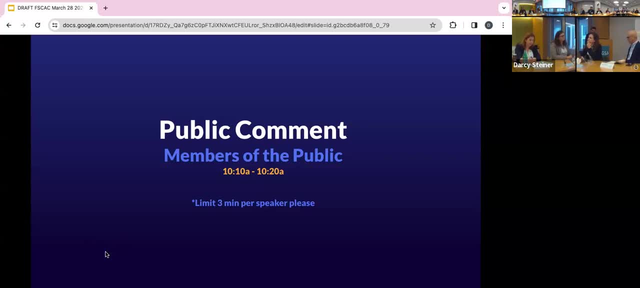 this committee's priorities should be for the next year. First and foremost, this committee should focus on the FedRAMP's digital mission, the acceleration of software procurement for the federal government. In that light, it is imperative that the intake process to an agency-agnostic authorization 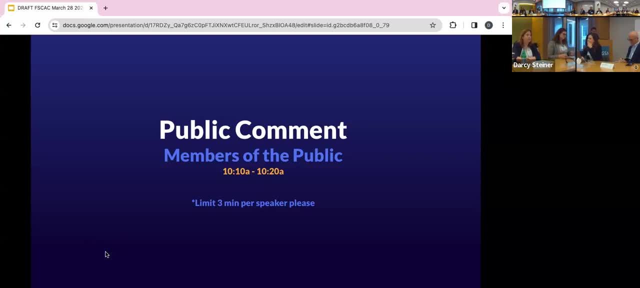 ie JAB or whatever replaces it- is re-established and streamlined in a way that continues to benefit CSP, who is looking for a way to continue to deliver software at speed, Being able to expand access to the CSP's path to authorization as well as streamline the SCR process. 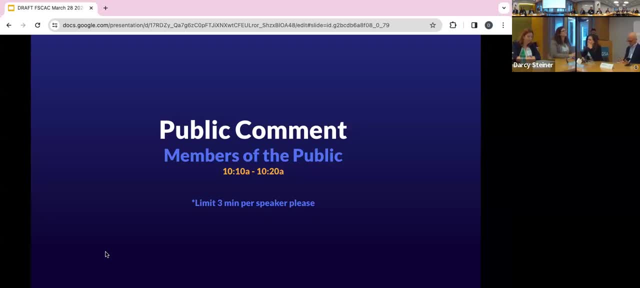 is critical to that original objective. The second part of FedRAMP's original mission is effective risk management. The National Vulnerability Database increases on average over 20% every year the number of vulnerabilities reported. Currently, vendors are expected to patch low and moderate CVEs. 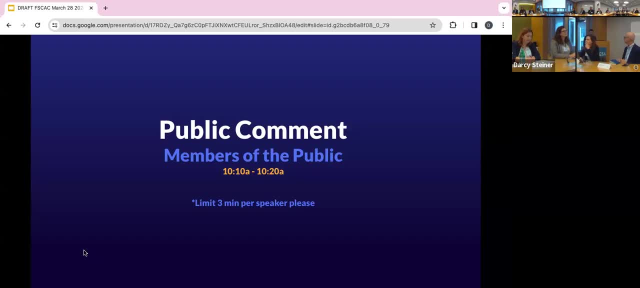 within 90 and 100 days respectively. According to Stanford University, 88% of data breaches are in error, leaving the remaining 12% to technical experts, which is what vulnerability remediation and patching addresses. Risk management is really about effective resource utilization. 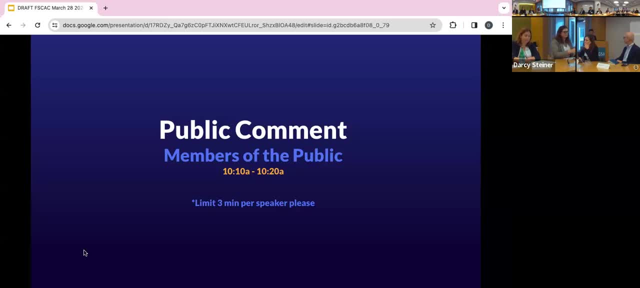 Right now, CSPs are expected to withstand finite engineering resources to fix these vulnerabilities, particularly where we already know the risk is low, as opposed to just fixing the known- as opposed to just known- exploitable vulnerabilities, instead of innovating and delivering new products. 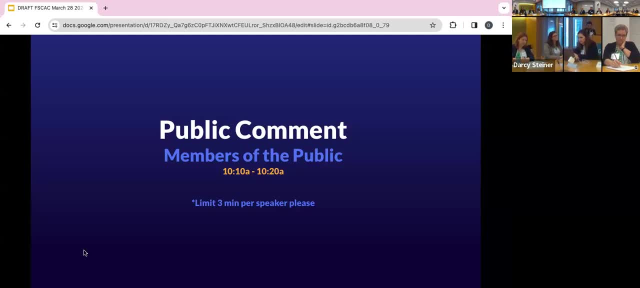 to federal government. We ask that this committee look to identify better ways to manage risk. Let's focus more on that 88% of breaches rather than the 12%, while ensuring that the engineering hours are maximized within that 12% as part of a risk-based approach. 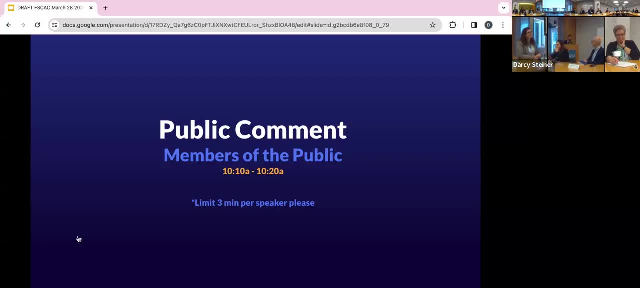 to vulnerability management. Thank you. Thank you, Josh. Do we have any other public speakers? This will go ahead and conclude our public comment for today. Thank you all. We will now go ahead and jump directly into our agenda's first topic today. 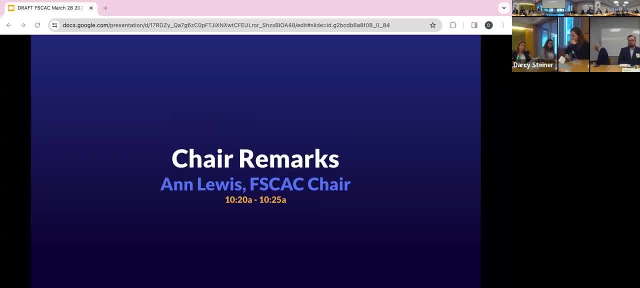 which is our chair. remarks: Anne, as the committee chair, I would like to invite you to make any remarks you'd like to make at this time. Thanks, Michelle. Hi everyone, I'm Anne Lewis, FSPAC chair, As Michelle previously mentioned. 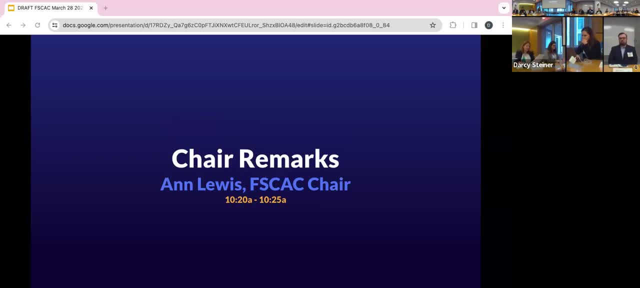 we approved our top actionable recommendations and our initial priorities of authorization process improvements, continuous monitoring, process improvements and automation opportunities and initiatives, And I just wanted to commend the committee on their work on these three initiatives. I delivered the final edition of our memo to the GSA administrator. 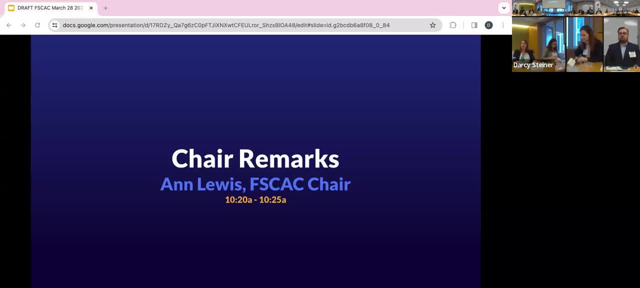 on Tuesday, March 5th. I'll give you it on our website. She has since been briefed several times on the memo, understands much of it and has started to work with the FedRAMP team on bringing the recommendations that you all came up with. 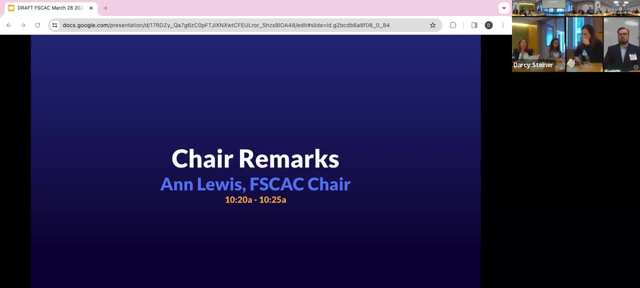 and put in the memo into the FedRAMP's roadmap, the FedRAMP team's roadmap. So I just wanted you to know that we have completed the cycle on talking about what's important, trying to figure out how to create actionable recommendations. 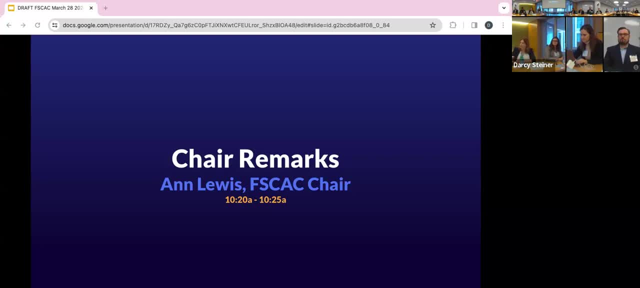 delivering them to the GSA administrator, and those recommendations have reached the FedRAMP team. This is a big deal. This is a new committee, It's a new organization, So I just wanted you to know that all the work that you've done- 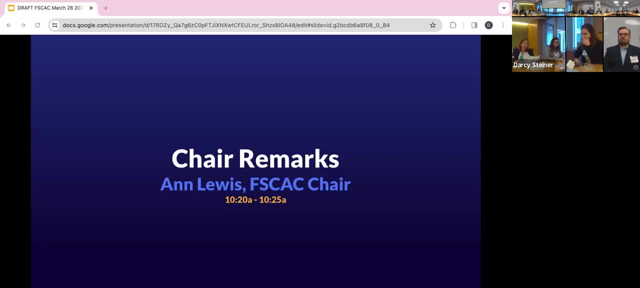 over the last year matters and is being actioned now, So let's celebrate this. I'd like to take a minute and just applaud everyone on achieving this goal, like that happens, So let's do more of this this year, Having completed our first set. 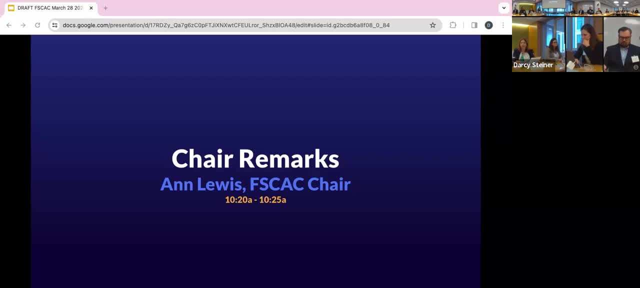 of key recommendations to the administrator. we now have the opportunity to start talking today about what our priorities are for the next year. What do we want to work on? What do we want to provide guidance on? in this unique public-private conversation? There's, I think, a lot that we can do. 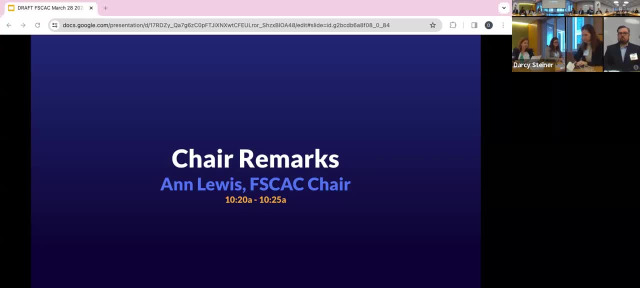 and, as always, the challenge is figuring out how to prioritize. So during our last administrative meeting, a few topics of interest were noted, and we'll now receive some additional information on those topics from a brief from folks in the room today. And so the topics: 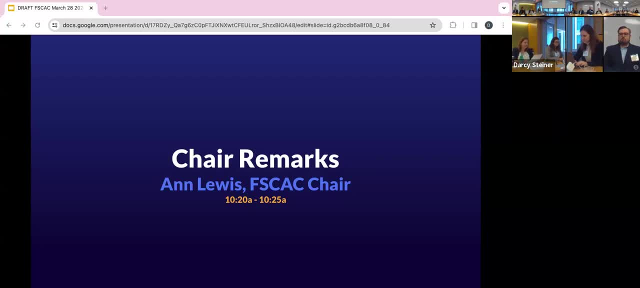 that we're going to hear more about and consider, that you've discussed in previous meetings, are updates to the draft OMB memo that OMB has made. what FedRAMP's response to these athletes are? what is the third-party assessor stakeholder experience? 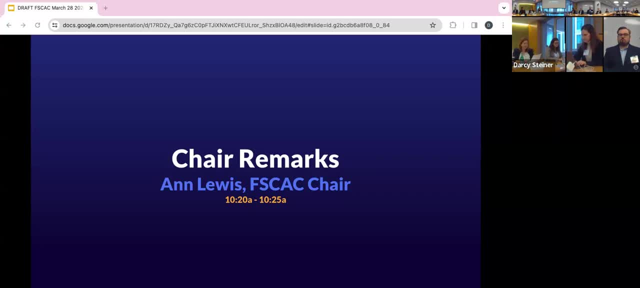 and are there ways that we can improve that to support the third-party assessor market? So that's a great place And a few other topics as well. So we'll get into the meat of some of those topics and, as always, the committee can drive this. 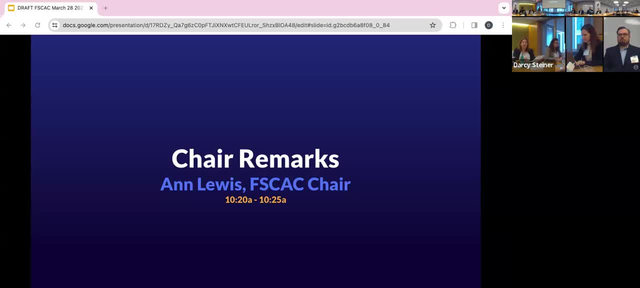 in whatever direction seems like it's most productive. We'll see if we can align on a set of priorities today. If not, that's okay, We can also continue this discussion later. So today our goal is to discuss the potential areas of interest. 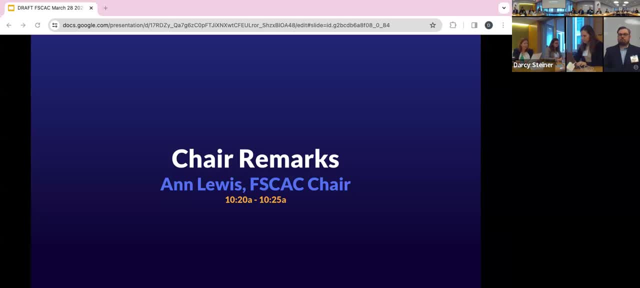 of what we would like to prioritize over the next year and figure out if we can determine a plan of action for diving deeper into these topics. So thank you for your work last year, Looking forward to our work this year, And with that I'll pass it back to Michelle. 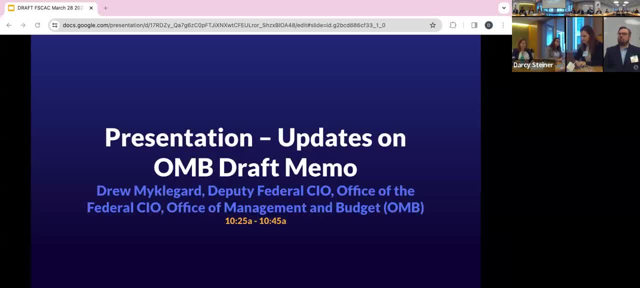 Thank you so much, Anne. Now I'd like to open the floor to Drew Melkegaard, the Deputy Federal CIO from the Office of Federal CIO of the Office of Management and Budget, who will be presenting on their updates to the OMB draft memo titled. 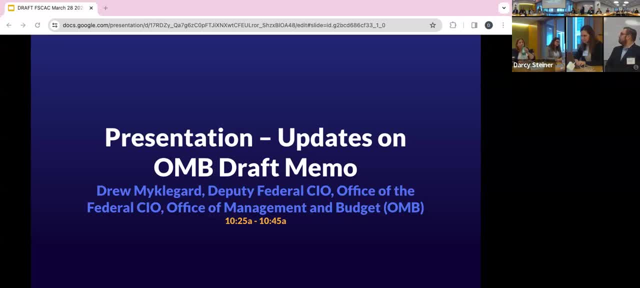 Modernizing the Federal Risk Authorization Management Program. Drew, thank you so much for joining us today. Thanks, Michelle. Do you want me here or here, Which is fine, It's fine. I just want you to be sort of close to the owl. 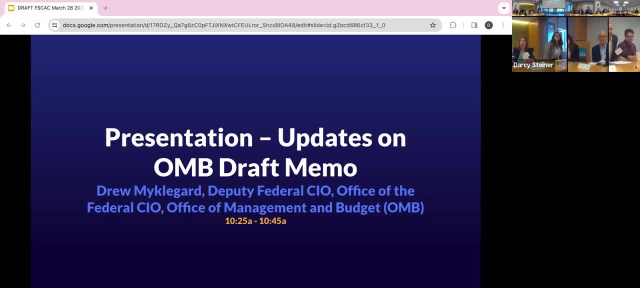 so that you will appear on screen. So I always learn a lot when I'm next to Jackie and Matt, So I'll cheat off this for my for my talking points. I just want to first off say good morning to everybody. For those of us, 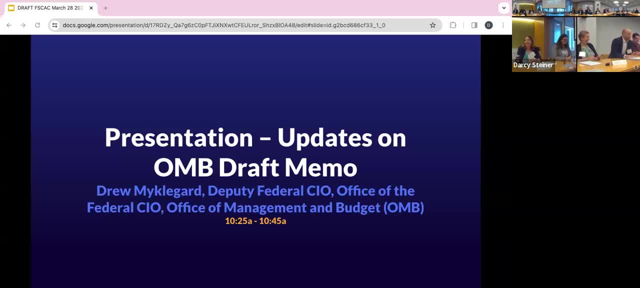 that are balancing spring break and what, what things we have going on. I really appreciate you all timing this early like this, because my kids are on spring break and they're teenagers, So by the time we get to spring break we're going to be. 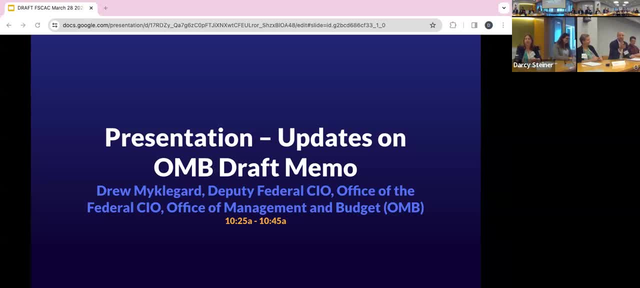 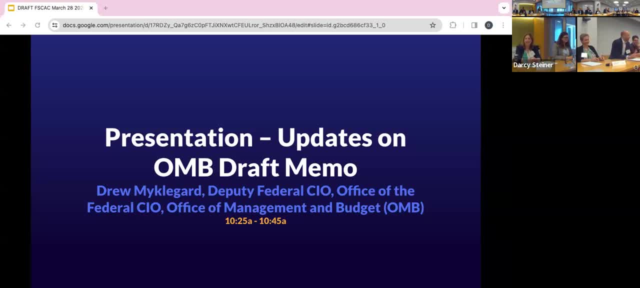 And I'm like: Well, I've been already successful, So just wanted to talk quickly about a couple of areas. One is like the: the level of OMB leadership that is committed to the FedRAMP program. We and I didn't know this. 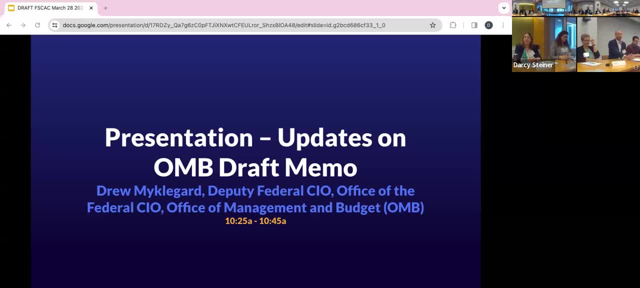 but OMB uses GSA as our executive, as our execution arm. We don't have any, as you probably realize. we don't actually, we don't do anything internally besides write, but we can't execute. But we have valuable programs that we want to see. 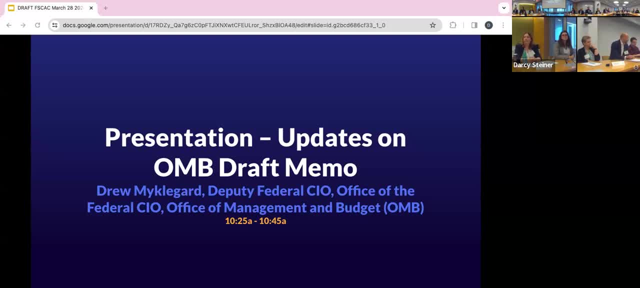 move forward because they're presidential initiatives and came up with four of them this year and FedRAMP is one of the four- And we've consistently worked with Ann and her team and Kunda to make sure that these efforts were prioritized Also. I just want to mention 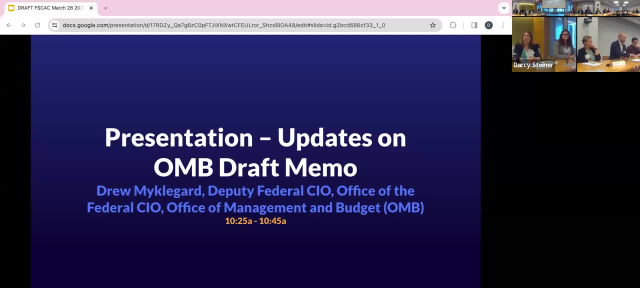 you know, from an OMB leadership perspective, like our deputy director of management, Jason Miller, his senior advisors, our CIO, always say: ask about FedRAMP, partly because they hear about it from externally. There's, you know. 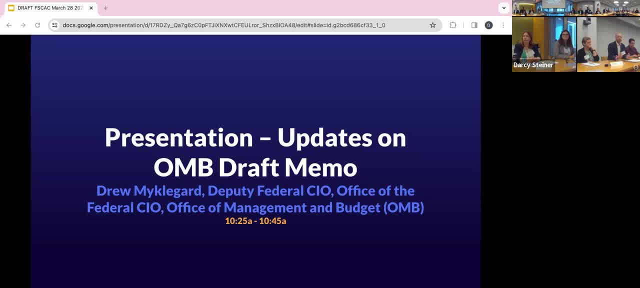 like this is one of the great interactions we have with the commercial sector. but also they see the real value in this. They've all been at agencies and know that, like when they can get in software, they can execute their missions faster and better. 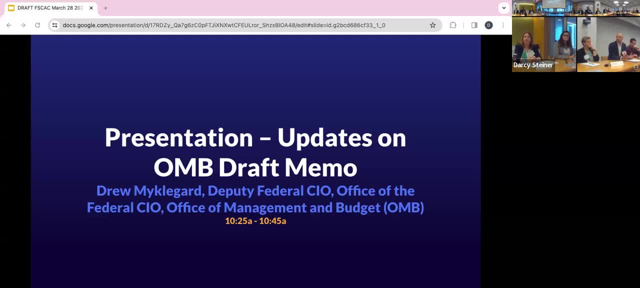 The last part is just like in these sort of events. just want to remind we all have multiple identities. Oftentimes I'm in meetings with a lot of other bureaucrats, government officials, government servants. This is a chance where, like software providers, like I've read- 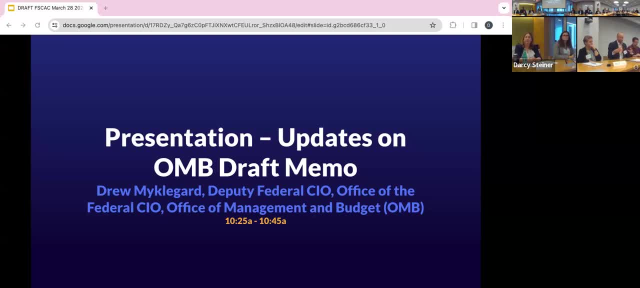 you know we got to. I've worked with Anne and another group to read all of your applications. when you came on I was like God. I'm glad I don't have to apply for this, because like never be picked for a board like this. 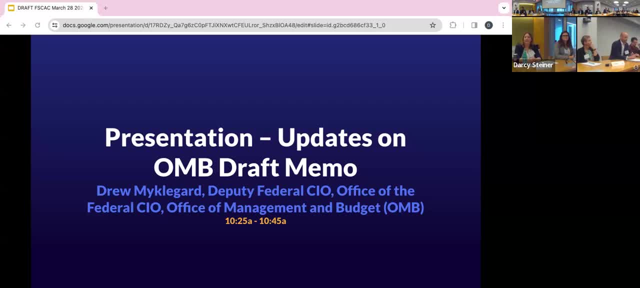 So it's great to have you all and great to be picking from such a great team from government. I know a lot of you, whether we've worked in government, commercial sector or just you know focus groups that are helping try the government or helping the government. 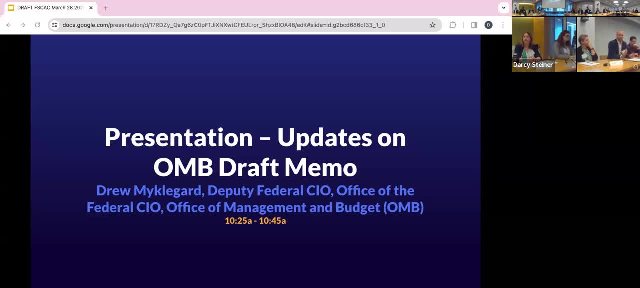 work a little bit better. But I would also encourage all of you in these times where, in person, you know where we're in a place, like learn more about the people that we're working with, because for myself, like whenever I can, whenever we're writing policy, 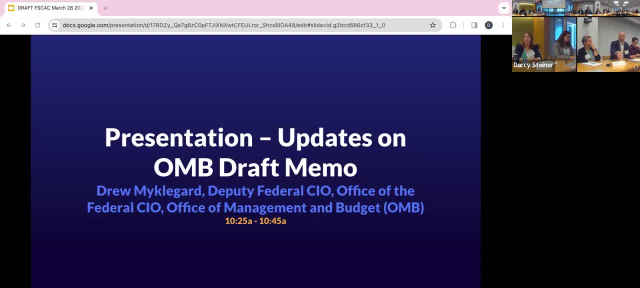 or making budget decisions, when I know that there are people that are directly impacted on the other end. like I put in more time, So I'd encourage you all to just like make those relationships while we're in the room, Just want to give you. 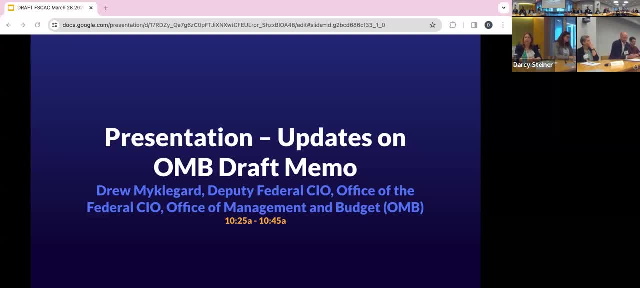 what everybody. nobody cared about what I say up until this point, probably. So policy update: This is what everybody wants to hear. It's been 10 years since we wrote the last policy. We put the draft policy out And first off, 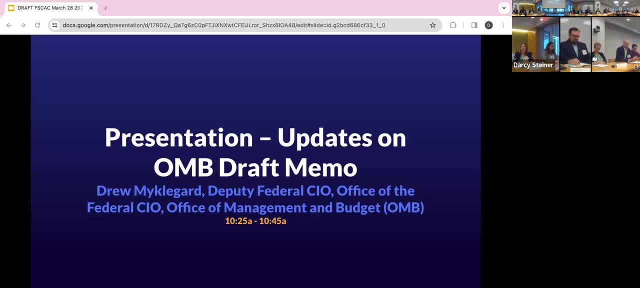 I just want to thank you to the FISCAC for your comprehensive and thoughtful comments and draft guidance We have found- and this is in part to a lot of work that Eric Mill did and Krista Rush early on in the administration. OMB isn't usually 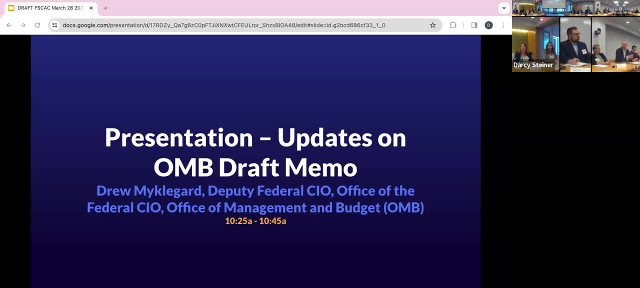 doesn't go out and seek feedback on our policies, but we've found that it actually iterates, makes better policy, much like software. We write a lot of waterfall in policy and we're trying to be a little bit more iterative about it. 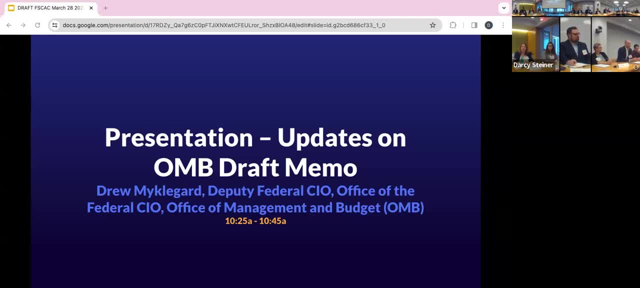 But we have the same challenges internally. I would say that this has been next to AI, like our most successful as far as getting feedback. We received 165 comments from at least 155 commenters, And we've reviewed each and every one of them. 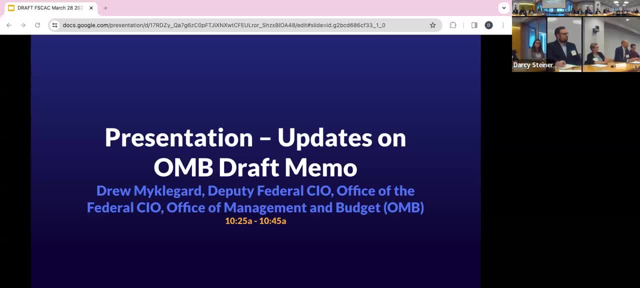 And we've sent out thank you notes. Thank you to everybody that responded. So we really do appreciate it and have spent a lot of hours. It drives a lot of the way. we think I did want to mention that some of the commenters 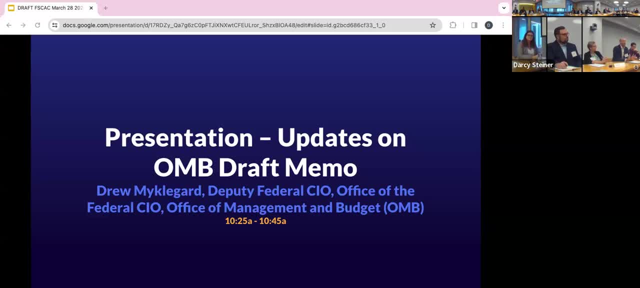 submitted multiple page documents and we really appreciate that I'm counting those as one comment and not like the total number. Otherwise we'd be over 200 and really giving AI a run for its money. But AI comes up in almost everything we seem to be doing. 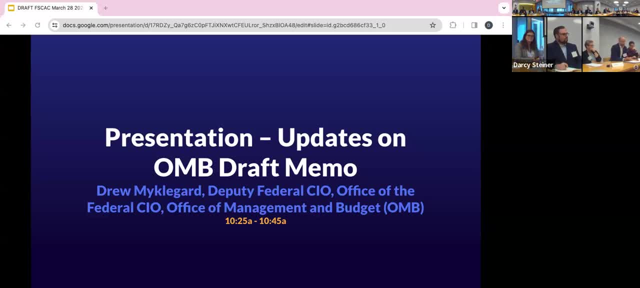 these days. You all specifically raised some good points And, as we're updating this guidance, addressing both what we heard from you as well as broader community, And I think, just like from a personal standpoint and writing, that policy was, you know, it's very challenging. 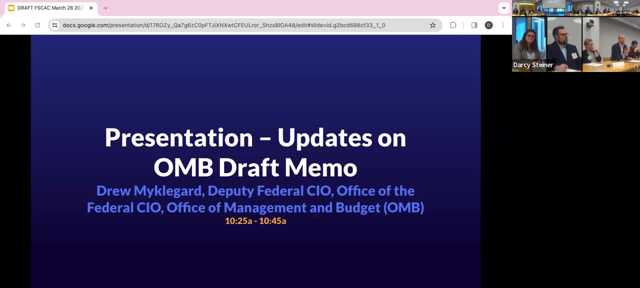 You want it to endure and then to put it out and get good and bad feedback makes it much better. So when I was reading the comments I'm like: oh yeah, I struggled with that point, Like red teaming, for instance. 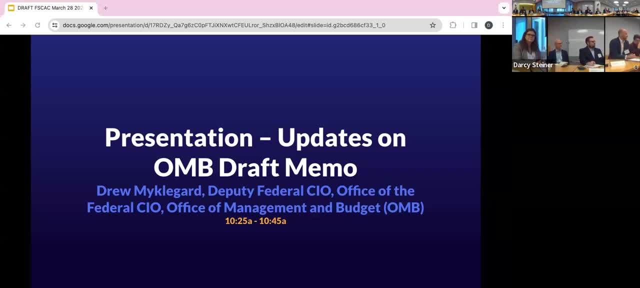 Like we really struggled with red teaming. Hearing from you all makes it a lot better And we hope that this policy will endure. So the next area is hopefully me talking a little bit less and hearing from you all. So this is the assistance. 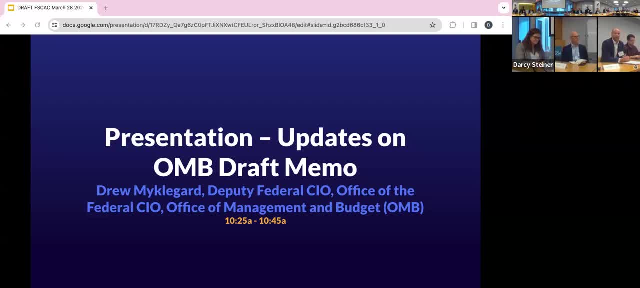 going forward from the FISCAC And we want to collect feedback in three areas. So I'm going to throw out these three areas and go one by one and hope that you all give me like some pointers such as this: you know, like, give me. 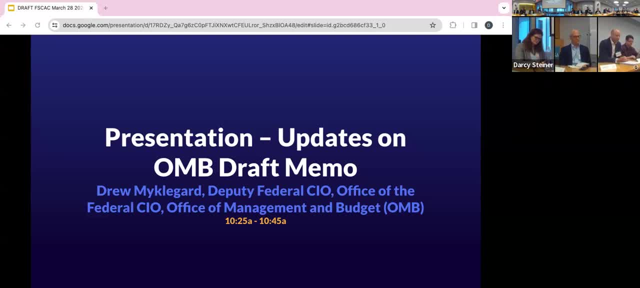 give me some steers on that. So the first one is FedRAMP and small businesses. So our prompt is: provide additional insights into how FedRAMP can support small businesses in overcoming challenging and obtaining- or sorry, overcome challenges and obtaining and maintaining a FedRAMP authorization. 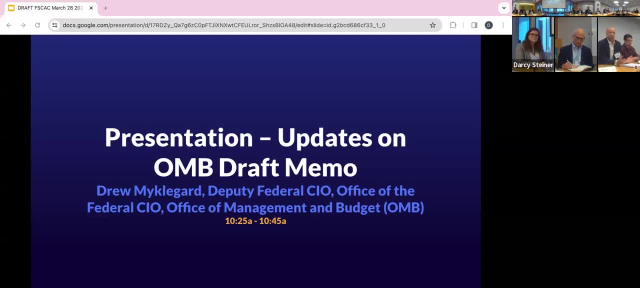 without comprising security rigor. We all want to see more small businesses. We're all dedicated to that, But we we're not sure like the best ways to do that. How does that resonate with you all? Is that an area that's salient? 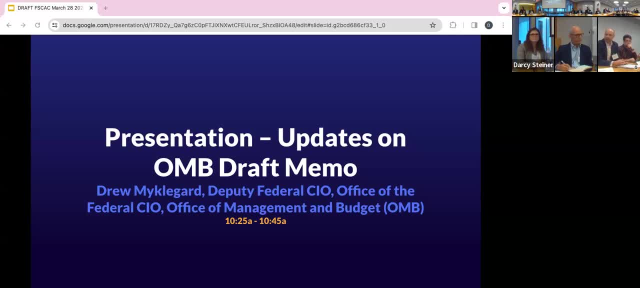 Do you have for the, for you at agencies? Is that something that you're challenged with? I know, when I was a VA, Josh, like we had goals for what we were trying to get. We do It is hard to get a small business. 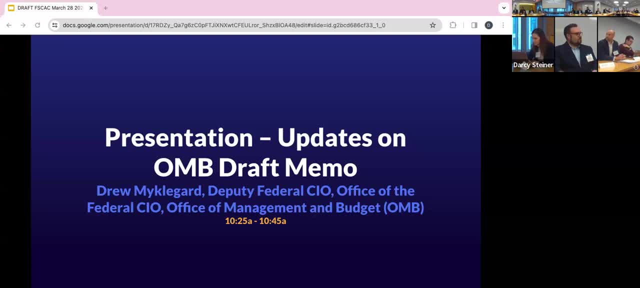 who especially has never done business with the government, into the government in general, just through all the procurement and all the other rules that apply, to then add what to them I think seems like a tax that doesn't exist in other markets Makes it hard to attract. 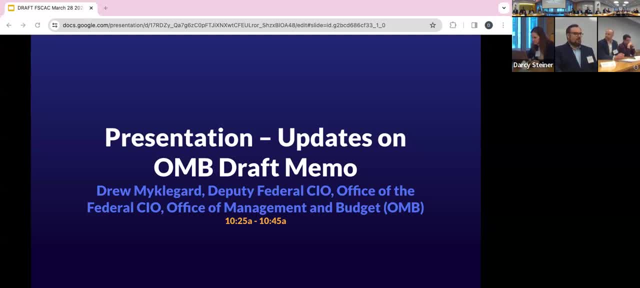 It's a it's a difficult conversation. every time we have it And I don't know there's a great answer to it, I think we just kind of try to be supportive as we can. But it's certainly been an issue, continues to be an issue. 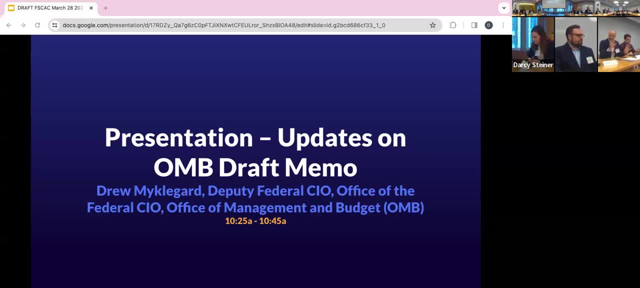 And Jackie being over at DISA. you're, you're at a high level, so you get to see across all of the branches, Do you? are you seeing a pathway or anything that works? So I think part of this conversation is around SAS and leveraging. 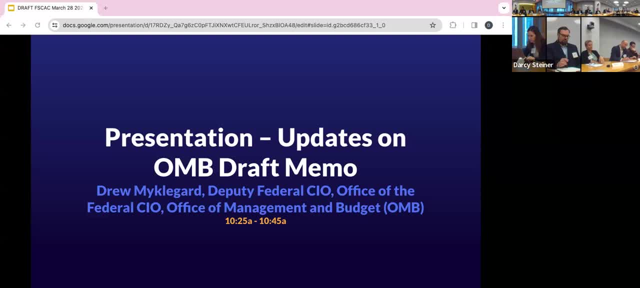 the infrastructure that we already have, infrastructure and PAS, IAS and PAS for the the use of SAS, And we've not evolved FedRAMP to consider inheritance as we authorize SAS, And so I think if we can pursue that path it reduces cost to the small business. 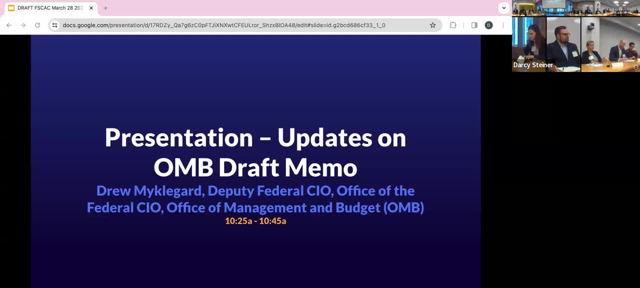 And I think cost is a barrier- from what I have heard- to for small business entry into the FedRAMP marketplace, And so I think that that is one area. you know, when FedRAMP started we were really focused on IAS because that's where the industry was. 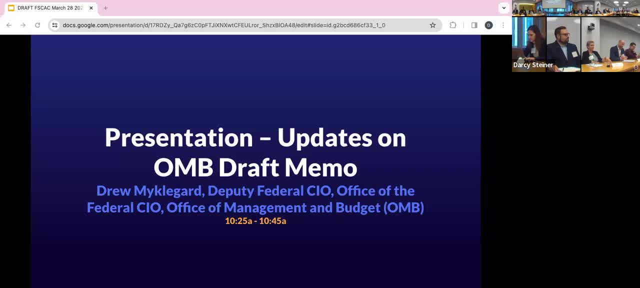 Today the industry is in SAS And so we've got to figure out a faster path and a less, again without compromising security and that type of thing. But how do we, how do we figure out, how we make that possible Right? 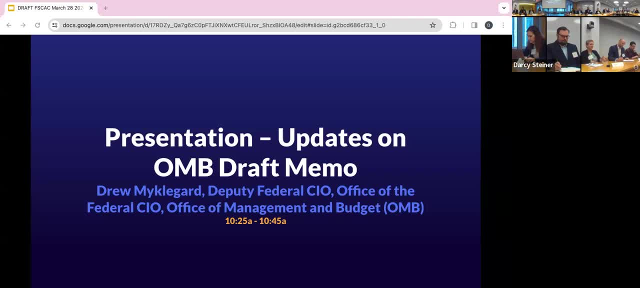 And so for some of our SAS providers, we've tried to pair them with an IAS or a big provider that says: can we get office space with you where we know you've got access to the network and help desk resources, And how do we pair up our small business? 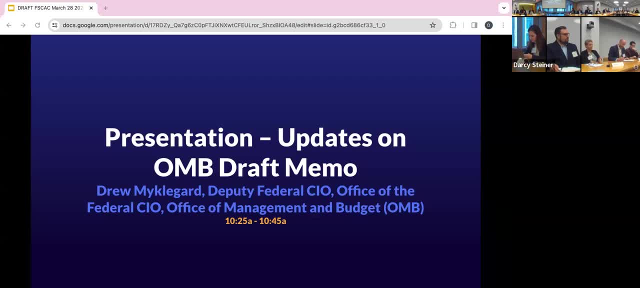 and our large business to work together, whether that's inheritance or, you know, sharing of resources And again, trying to lower the cost As a barrier to entry. So from my perspective, that is one thing I think that this group could potentially tackle. 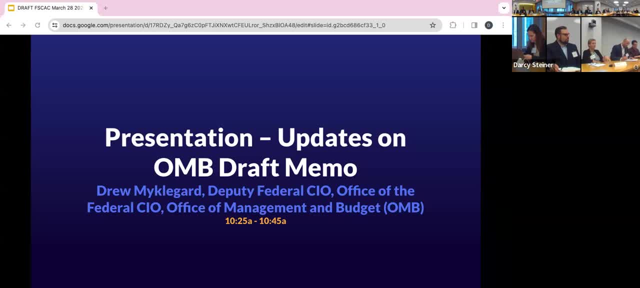 is: how do we streamline that process and evolve our requirements and processes around evaluating SAS? So this side of the table, how about you all, Anybody else? So I'm a part of a software company, a small business, So we've gone through this process end to end. 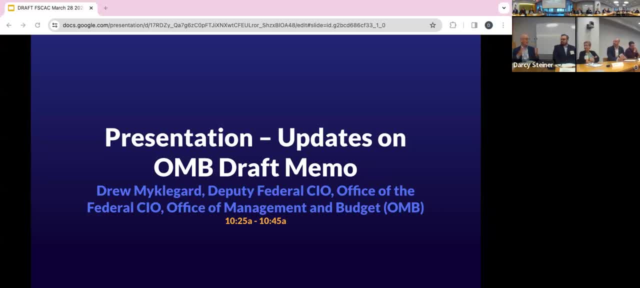 So I was there when we built the initial business case for our company. So the pandemic. we make a sort of decision support tool. It's visual, widely used in the commercial world: movie studios, big businesses. Amazon's a big customer. 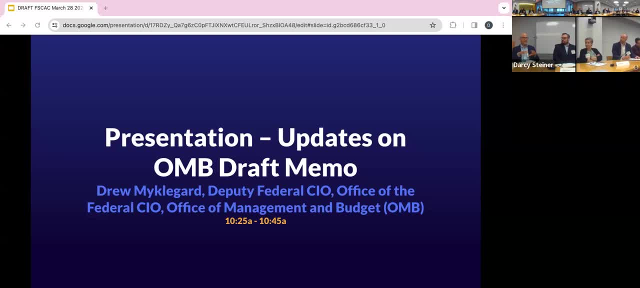 So we have a big contract with the intelligence community. I only set this out that we didn't come into the FedRAMP world with no concept of what security is- Enterprise security, intelligence community, top secret. We've got some grounding and some good technology. 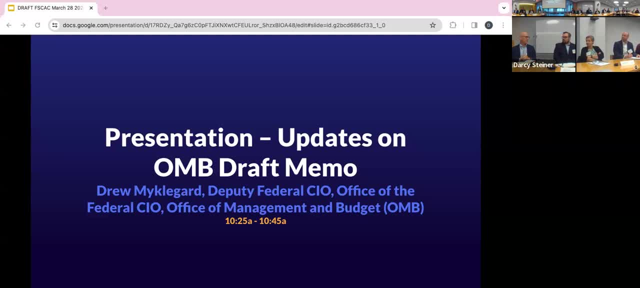 Pandemic happens and what we hear from DoD is that, look, if you're not FedRAMP approved, we can't- I mean we're not even touch your software. So we make the business case to go through the FedRAMP process. 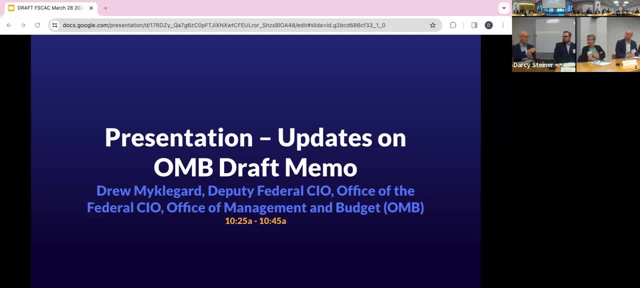 We got a lot of great assistance along the way, Really- And if you read my application you'll know it- And we weren't. our team was genuine. We wrote the application that got great assistance from the FedRAMP PM. There was actually great. 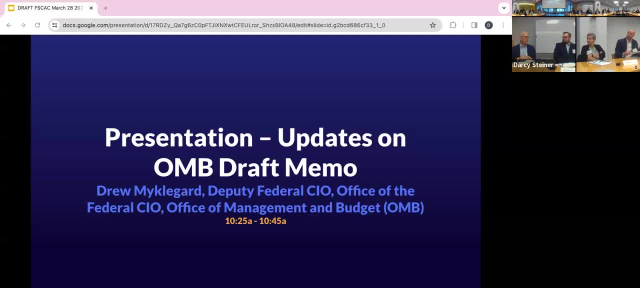 educational materials online if you want to understand the process. We actually got great help from people on Jackie's team as well going through that. I mean it's a process. It took two plus years. There are a lot of delays. I'm not going to say it was super fast. 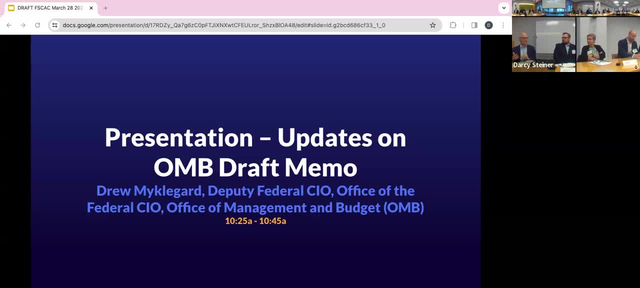 And, yes, there were a lot of costs incurred, but we did get through it And we're still stumbling. In fact, we just had to have Jackie help us with something a few weeks ago, So we're getting through. The costs are an issue. 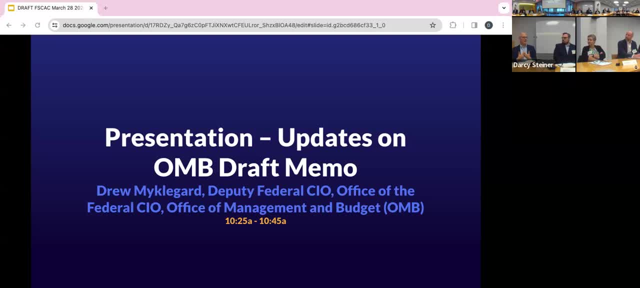 for a small software company, but my board will excuse it if there's revenue associated with the other end And what. I think that and again, we can absolutely. we need to improve the processes, Things need to be streamlined And I think it was great comment. 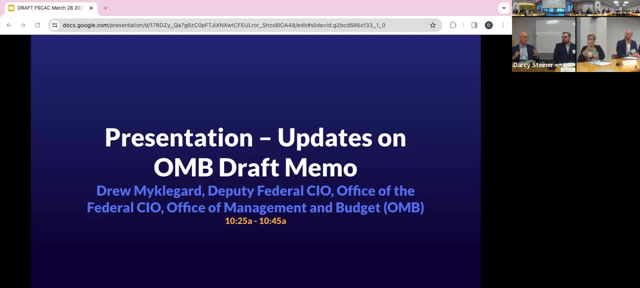 from the public comment from the gentleman from Red Hat around, you know, accelerating- I forgot how to put it- sort of accelerating the software procurement so people can get their emissions faster. I think it'll be focused a little bit more on that for small businesses. 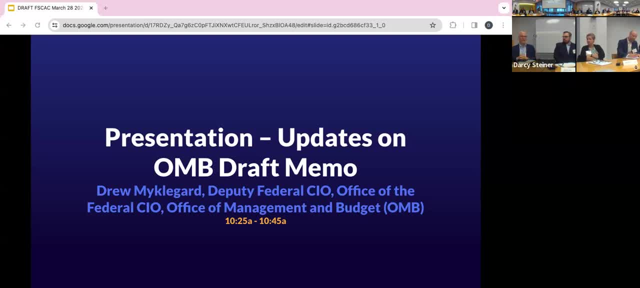 how to get your product sold And I would say probably for all the CSPs people- and I've talked to other CSPs who maybe not on the committee- and they all say yeah, it's okay, but the return on the investment? 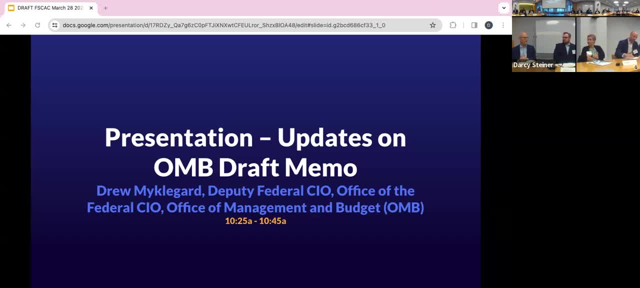 it doesn't matter what the investment is, It's the return isn't quite there, And so I don't know how to give that feedback, other than maybe if the pull for SAS was stronger, then people would put up with more costs and more process time. 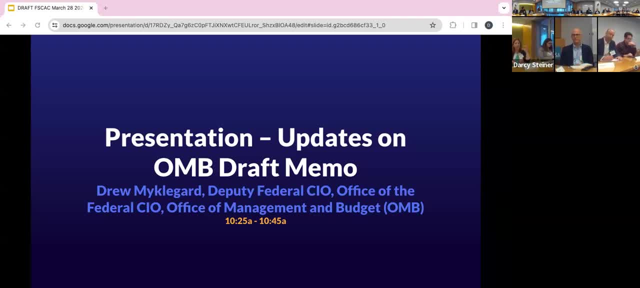 Just to keep going with that a little bit like: what kinds of metrics or outcomes do you think would couple that- like your small business and other small businesses goals with the goals that are associated with the authorization processes? now, So it's not, I don't want to make this a process thing. 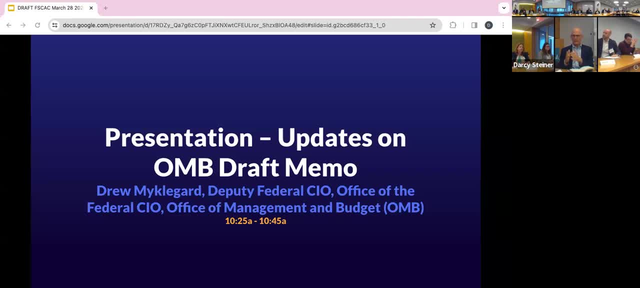 It's a different than process, because I think the first two comments where we need to make the process better, faster and cheaper. So I'm all with that. Literally it's dollars, Like you know from the CFO of my board. 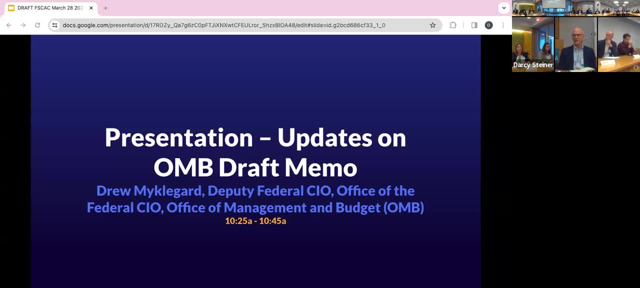 run the reports at the end of the month. How much did you sell? How many customers? Where's the? you know it's basic, classic business forecasting On the marketplace and I haven't tried to sort this way. Do you have criteria that says: 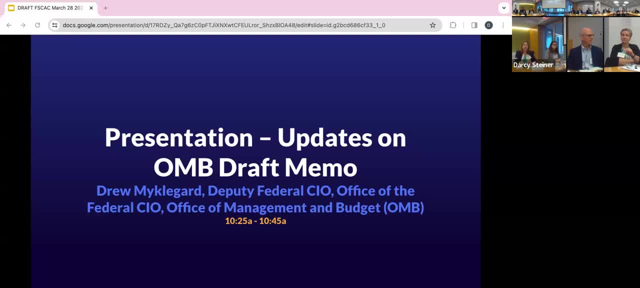 this is a small business Because people need to look at it, because people need to look for small business. So is that part of the criteria? Do we have good descriptors and certain criteria to say: I need this, you know, and so how can the marketplace be shaped? 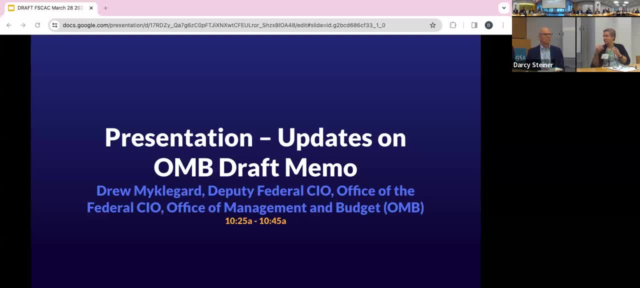 to help us get to small business, And it's been a while since I've gone and filtered, So usually looking for specific things. I have some thoughts on that And it's interesting because there's two policy worlds here that kind of collide. 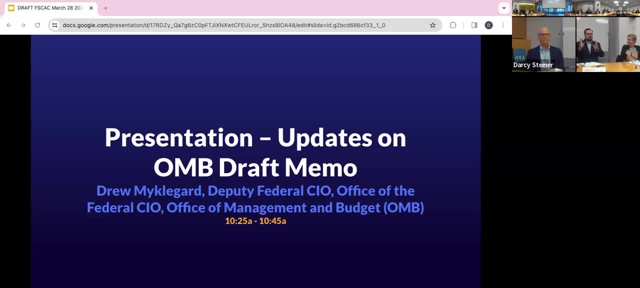 Right, There's procurement, which is- it's got a long history And you know obviously where I come from. that has a lot of- like security does, impact, I don't know- dogmas. Maybe it's a good way to think about competition. 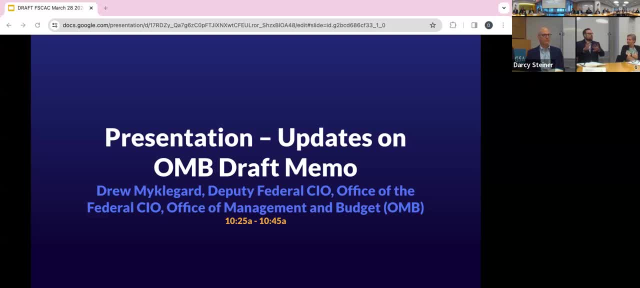 and what is a small business and how do we engage with them. I guess without getting into real specific things like more consideration for how those two things merge together. So for a small business, there are different ways to set business aside for a small business. 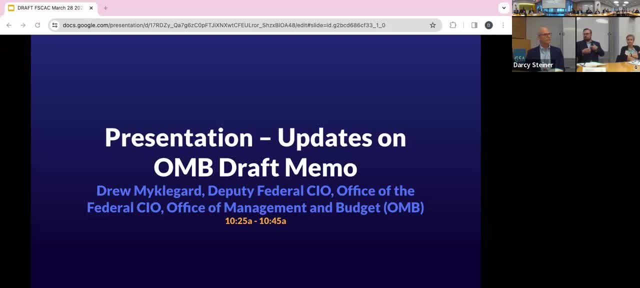 but FedRAMP doesn't really talk to that And there's also not necessarily, you know, an incentive on the back end of like if I go through this, I can be guaranteed a certain amount of business. We do what we can. 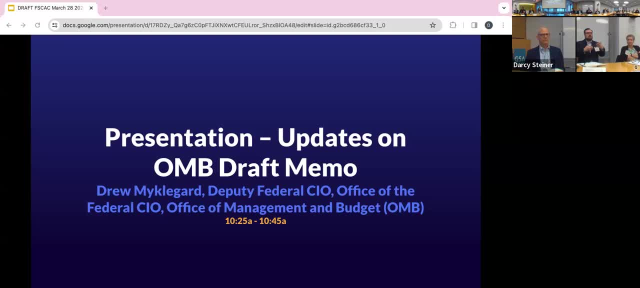 at least VA, to try to build flexible contracts that can give us a way to scale things. but that is perennially an issue And the length of FedRAMP makes it a really hard value proposition for a company. So it's like: 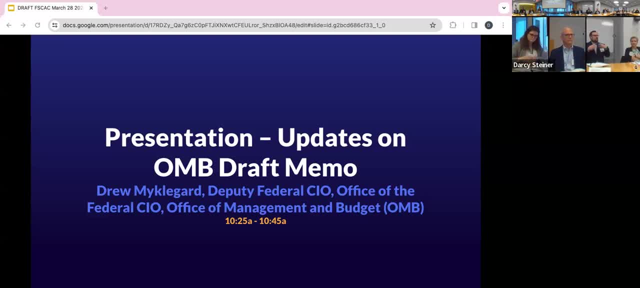 deal with the six months it takes to like deal with us and get money from us and get some footprint on the ground in terms of the contract, then wait two years or a year and a half, I know by trying to say it on the virtual timeline. 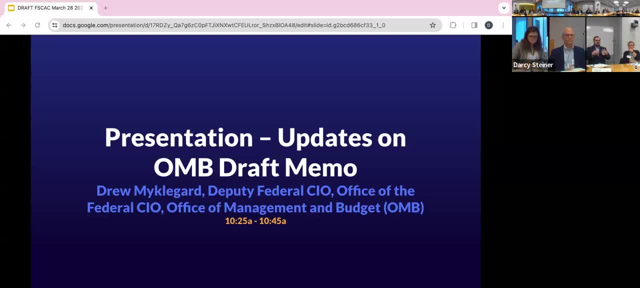 it's seven months, 10 months, but it's still a long time. Build into that the complexities of the budget process and how we are asking for the money to pay for those things years out, It's really, really tough. And then pile onto that. 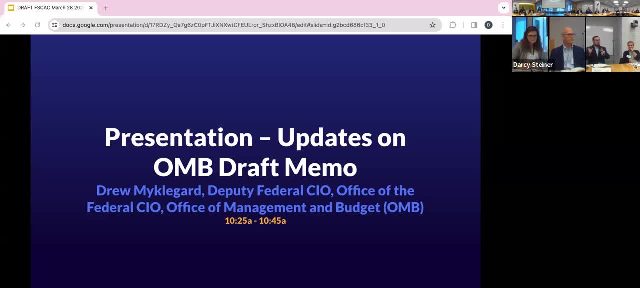 to your point, Drew, around AI, right. So now there's another set of memos, a third, very new infant, you know, in its infancy policy round, that's also playing in and that's just like: go to these pilots, go care about these specific things. 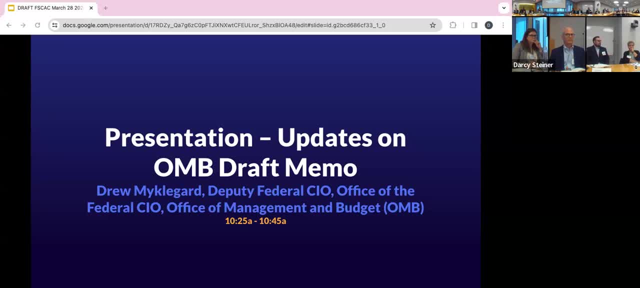 that also have to be. you know, considered FedRAMP and then all of the procurement and regulation rules, Just like some small business seems like an opportunity where there's already small business, set asides and things just somehow create tools for people that are. 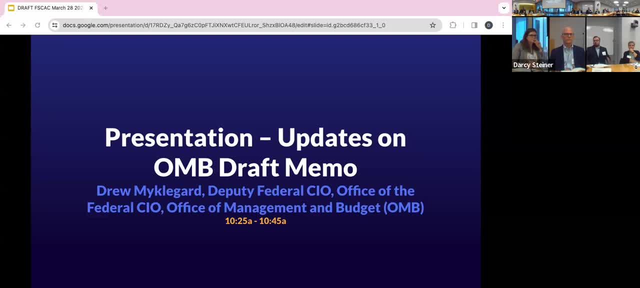 at the agencies buying things to make some of that easier. And then, when I'm in the room with a small business at a conference and someone's selling us in something I know we would otherwise be interested in, we would have a path we could say. 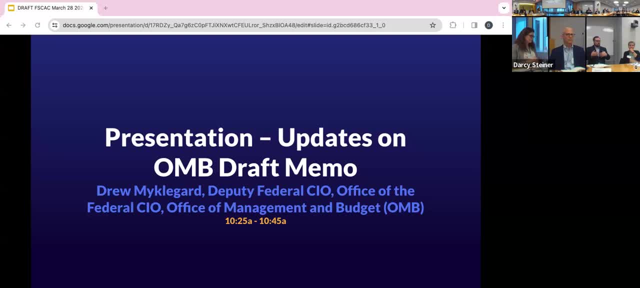 you know, at least to the smaller vendors, and then you can even get into the. where do they get the money from to do those things as a small business, right? So they have to go to their investors, to, you know, private equity firms and stuff. and bump them into what I just described as like a good investment. you know, and a three-year horizon for a small business is a very long time for them to do this. So I just think FedRAMP has kind of been shoved into that. 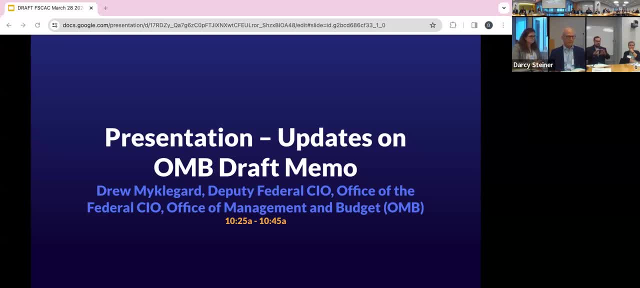 that conversation and we are, all you know, even just telling us what we're supposed to be doing with the small business piece and are we allowed to set things aside, would help the other side of that conversation: the lawyers and procurement officials and the agencies. 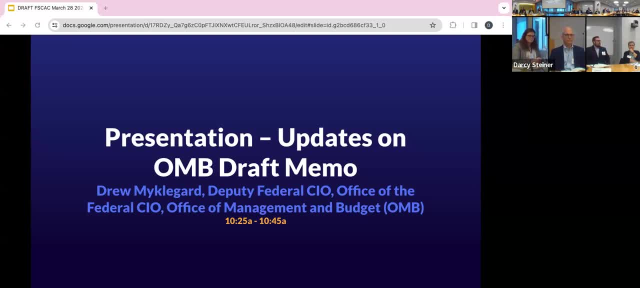 come to terms with when we ask you to do this. and from the IT side, yes, there's a you know some regulation in that space. If I could just belabor this just a little bit further- Not that everybody isn't doing a fine job. 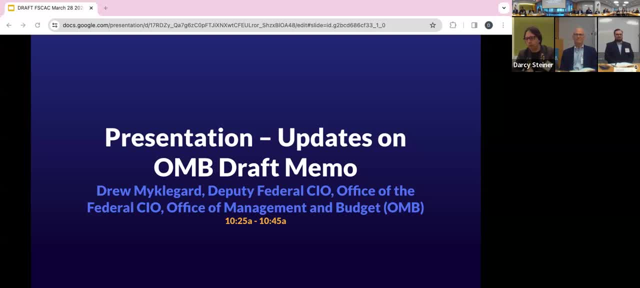 but I tend to filibuster as well. I think I'm at my federal agency now and of all sizes now, small, large, everything in between the VA, the OMB, the DOT, the SBA, the SEC, And during my time, 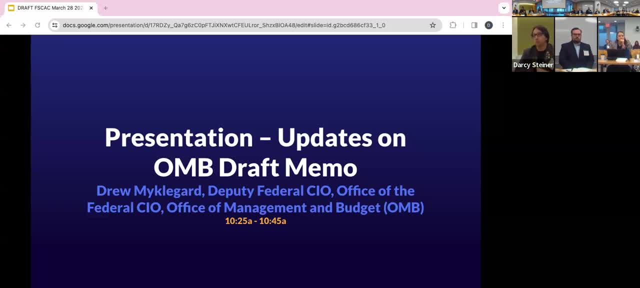 at SBA. you know there's been a lot of focus there on getting the small businesses into government. That is a priority. That's part of the mission of SBA. I think we can all agree that small businesses aren't going and standing up. 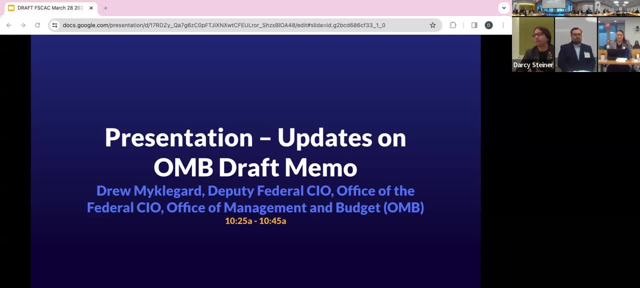 biases right. They're not going to go and build a data center. They don't have that kind of capital. That's not going to happen. I've also seen in my spread of agencies that there's a lot of most of the people. 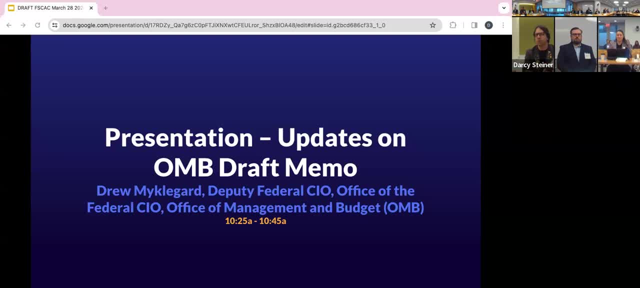 coming to me and wanting a small business solution that's a SaaS, typically aren't coming from like central OIT, They're typically coming from a program And that impacts the small business because you're not getting the entire agency wanting to buy your solution. 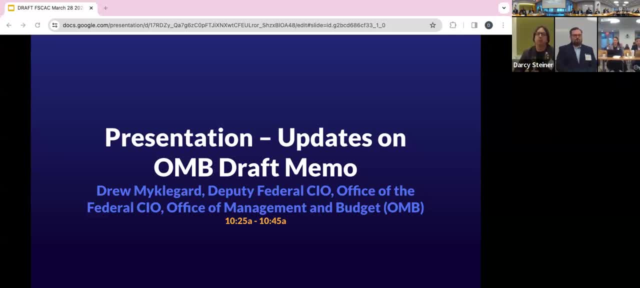 You're getting an office that maybe 15 people that want to buy your solution And that is not a thing that you can get a return on investment unless you can get every single agency that wants that to come to the table. That's really hard. 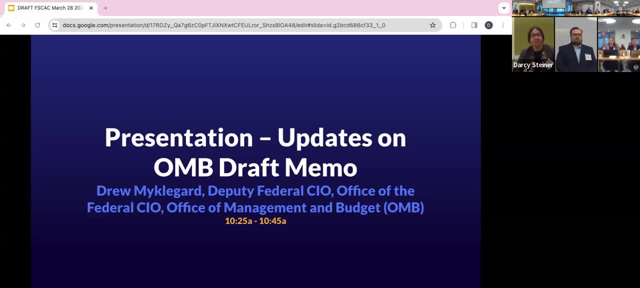 I don't think there are easy solutions for that, because there isn't The juice, isn't with the squeeze in those cases. But I will point back that it's probably outside the scope of our friends here at the table, but you all could do more work. 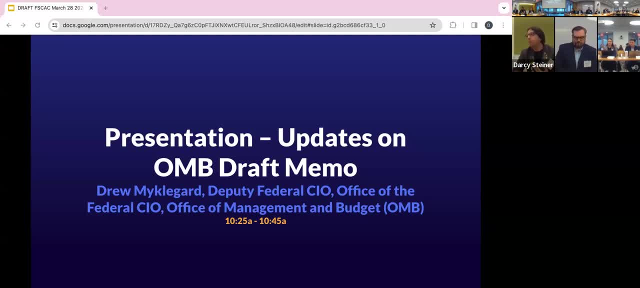 probably with SBA, in leveraging the ADA program to be able to get those solutions, to make more opportunities for that sort of funding for people to get through this process, specifically working with the Hill to make sure that those dollars are being put so that these solutions. 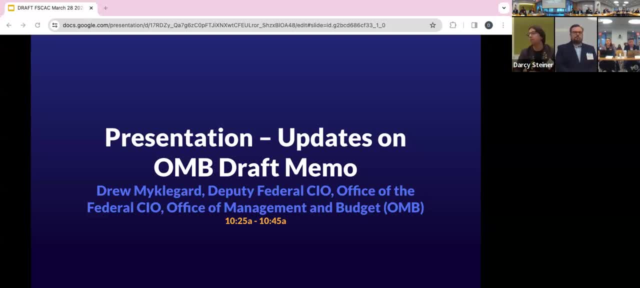 can be funded by the government for the government to use. I think that's really critical because I don't think the money is going to come from the investors in those cases. They're not going to see that. for the smaller ones that have the really interesting 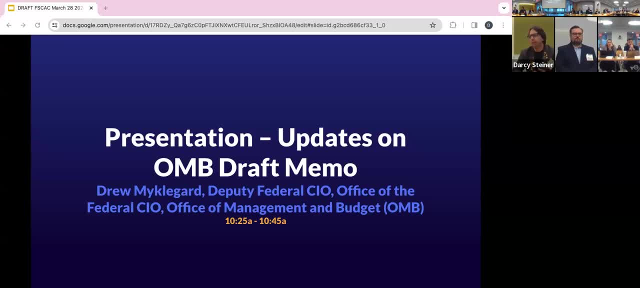 innovative products these days, So I think that is going to be probably one of the things that are going to be poked at. I will also be the cynic that I always am and say I don't want to see the standards lowered. 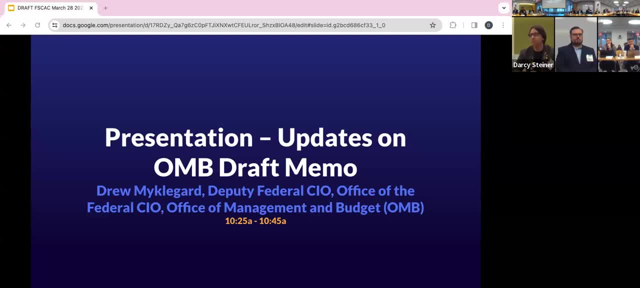 You know, after we've seen with SolarWinds, after we saw with the Microsoft breach, even the biggest companies in the world are struggling with IT. Technology is hard. I've been a software developer for I don't want to say 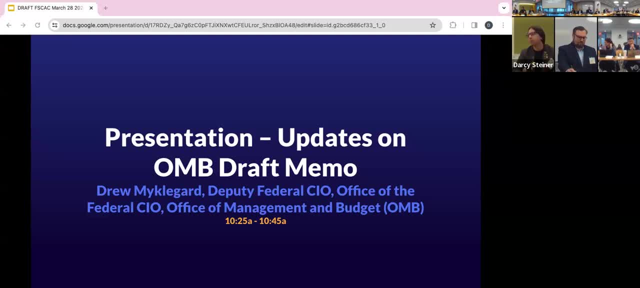 a long time And we all. bugs happen. It's always going to happen. These vulnerabilities are always going to pop up, no matter how good your systems are, no matter how rigorous you are, And so, as a person who runs a company that runs a lot of IT, 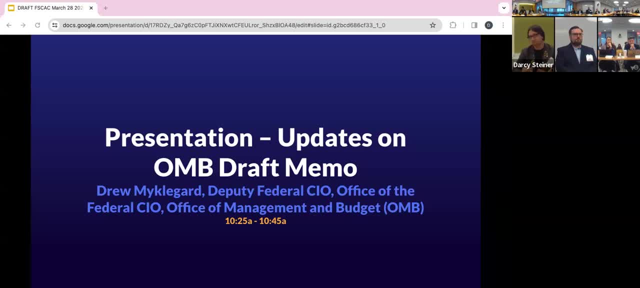 I don't want to see the standards lowered for small businesses. I'm sorry that that's not what small businesses want to hear, but I have to protect my name, So that is a priority for me: Making the funding available so that they can meet the standards. 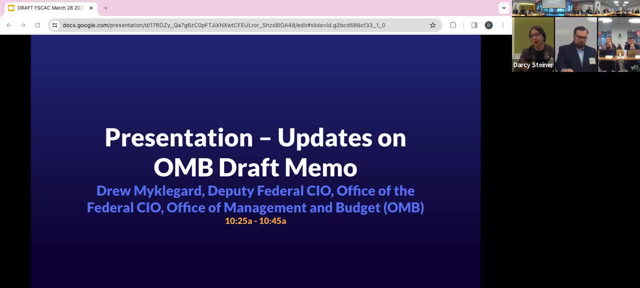 that everybody else has to hit and using inheritance if they're just riding on top of NIS anyway, like let's leverage the continuous ATO process and get them through that? Yeah, Definitely, to echo Bill's point on inheritance, I think that that's probably. 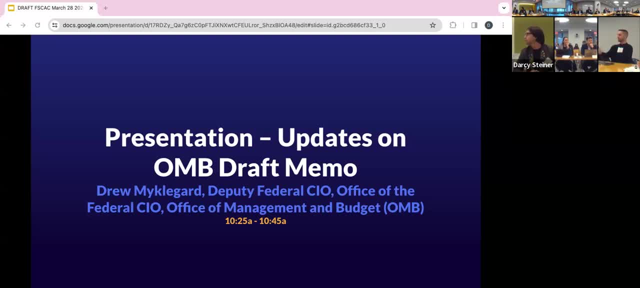 one of the quickest ways to get to that level of, like large CSPs, delivering these controls to a GA level and then having small businesses ride on top. I think that's probably one of the best bets we got. The other thing that I brought up last time: 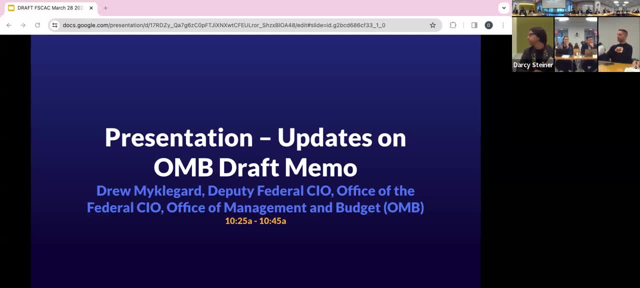 and I just want to flag again is that NASA's got a really great technical readiness level risk management program where they have levels of scope and impact versus the technical controls that are in place and they graduate those technologies up until they're ready for humans. 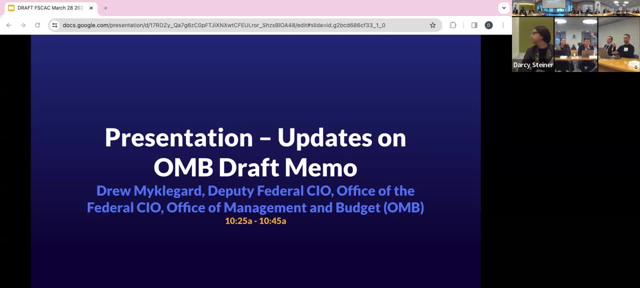 We should do something similar or have a smaller path in our program where that would unlock small businesses to be able to use maybe a smaller set of controls for a specific targeted mission or a specific targeted program And then, as they're going into more and more adoption. 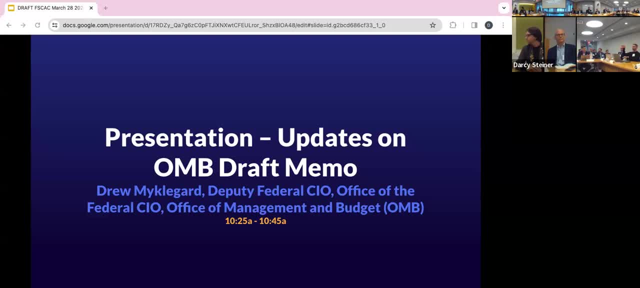 we kind of crank and turn on more and more levels of control on them. Yeah, I know we have low median high right now. Maybe that's something we should look at more and more. It's a low moderate high, Maybe that's something. 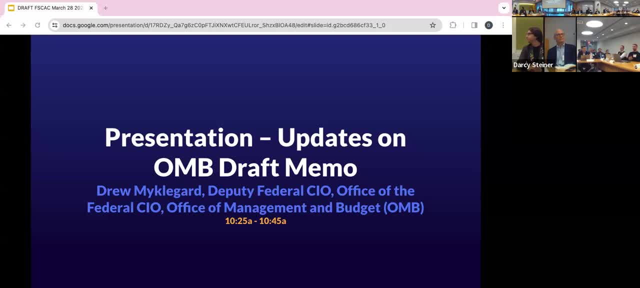 we should look at in 2024.. Maybe there's a better path that we could put in place to think about how we can think about pilot programs versus large CSPs delivering for hundreds of agencies and investors. I can add on, just to tag on to that. 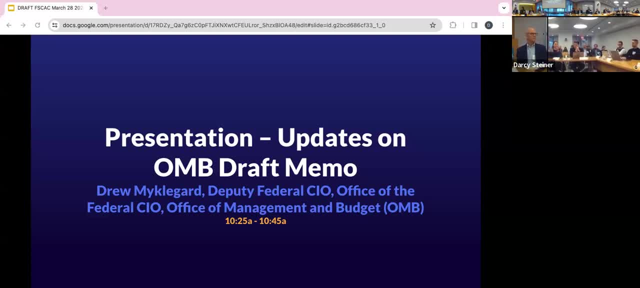 the low impact SAS offering, I think is probably most in terms of what we have currently in line with kind of that first step, maybe very narrow use case or still that kind of thing. So just wanted to add that. And then one thing: 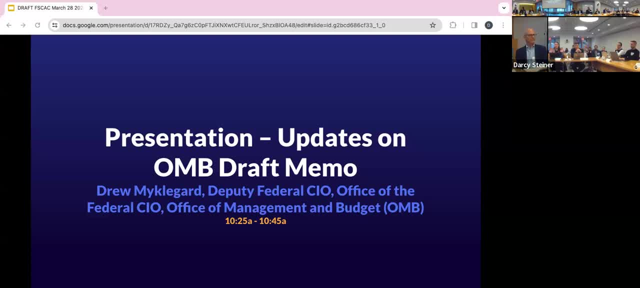 so, Marcy Shalma, through PAO perspective. So you know, we have a pretty limited purview in terms of like before CSPs get to us and after they get to us. It's like during the assessment and authorization life cycles. 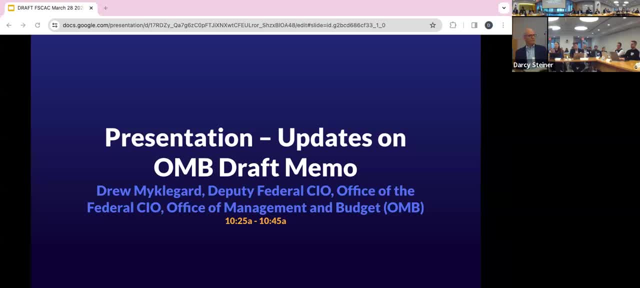 when we deal with them the most. But what we hear from our clients is that they kind of- or they- anticipate that they'll get an authorization and then agencies will be banging down their doors to use their products, and that's not the case. So it's more of like 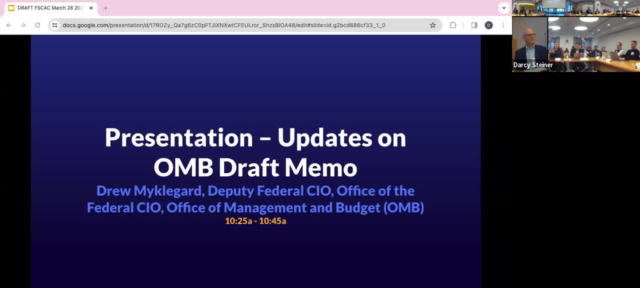 what happens after, and maybe that's an education, maybe it's awareness, maybe I don't know, But I think that there's the expectation versus the reality. post authorization: Yeah, Please. So, Naman, I'm sorry, in the Small Business Administration. 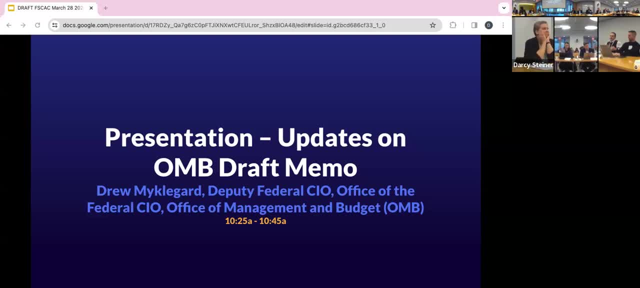 I want to talk about two points here. So first, from the procurement side, when we get to execution, we're not frankly thinking about certification standards. Those needs already have been baked into the requirements that are presented to the procurement professional contracting officer. And then, what drives that decision? 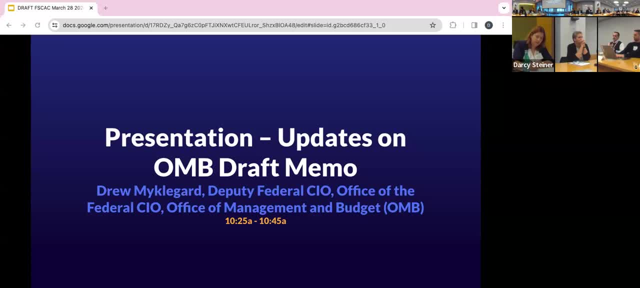 It's speed to contract. So what's category management driving us if we can get to a set aside in the 8 program, or are there any other sole source authorities? Those are the kind of the driving forces or the driving factors in terms of what procurement. 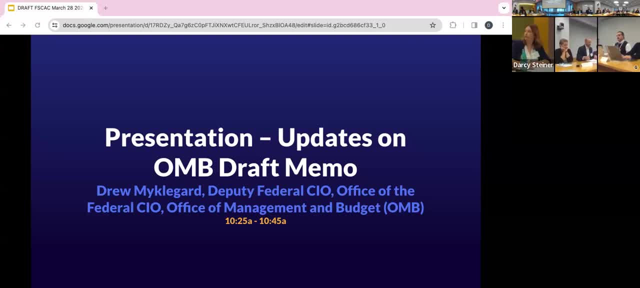 we want to get to. So I think one of the ways that this issue can be addressed is programs that have worked successfully. So Mentor-Protege has allowed and I think it's worked really well at DHS. It gives program offices a level of comfort. 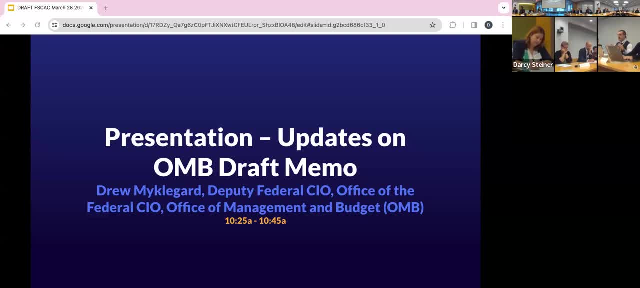 on larger scale projects to have bandwidth and capacity for large business but mobility and ingenuity of the small business working together. So maybe that's a path to mediating some of the issues that we're talking about. Also, you know the programs like SPIC. 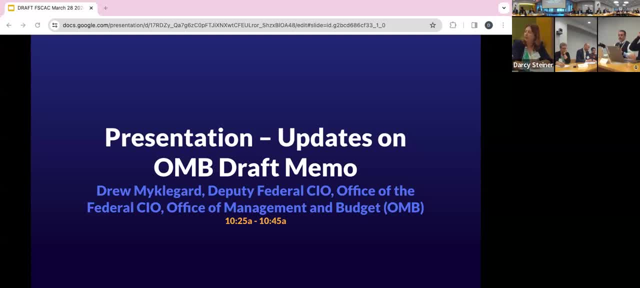 the Small Business Investment Company, SCTR, all those programs that currently exist at the SBA that offer funding and offer grants to small businesses in the technology and innovation space. Maybe we can leverage some of those funds and redirect them towards this effort. I'd be happy to connect with you. 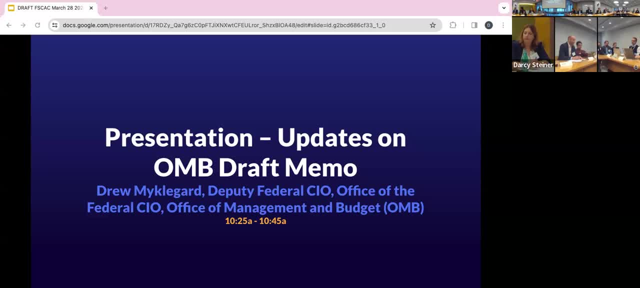 and put you in touch with the right individuals and build offices to see if there's other funding. I would appreciate that. That's an area that I feel like we underutilize. Yeah, Drew, I mean one thing that we do here at GSA. 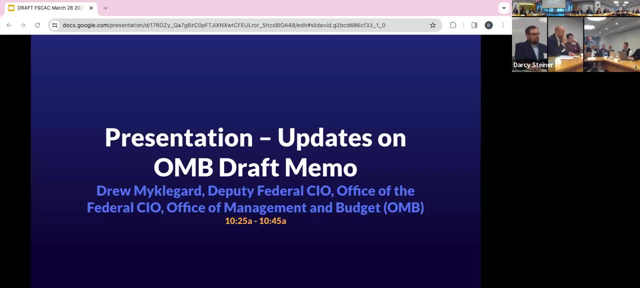 we work a lot with a lot of Luthier IoT service providers that are increasingly providing SaaS-based solutions, EVSE being one right now, you know, as well as a lot of smaller companies that provide SaaS-based services, And you know. 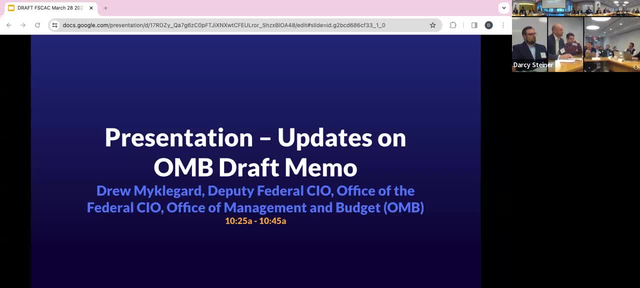 similar to what Michael was describing what NASA does. we actually have an agile, risk-based authorization process that allows us to be able to get to the services provided by a cloud service provider using more of an incremental approach, And the way that works from a contract acquisition standpoint. 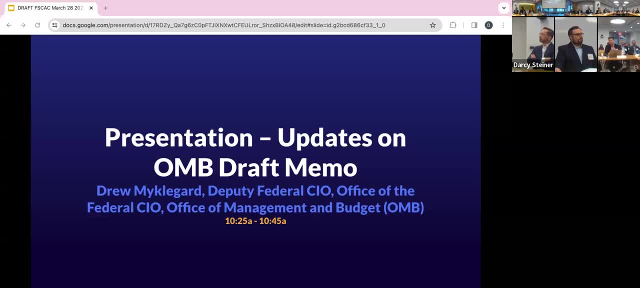 is that you either are federally authorized or, as part of the contract acquisition, they essentially have to go through and achieve an authorization through what we call our live SaaS or our my SaaS processes, which is really focused on a subset of the very technical set of controls. 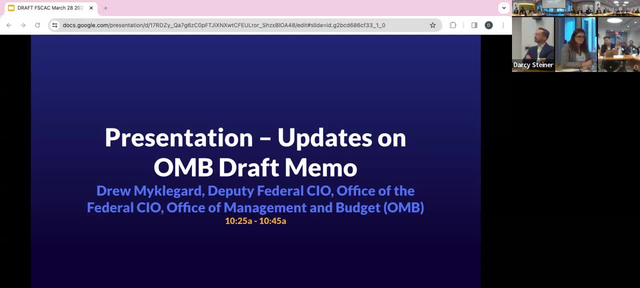 corresponding to the FedMan baseline, be it low or moderate, requires they effectively run on top of an existing FedMan authorized platform or infrastructure, And what this benefits is a vendor to allow for them to start to realize revenue while they're working through the FedMan authorization process. 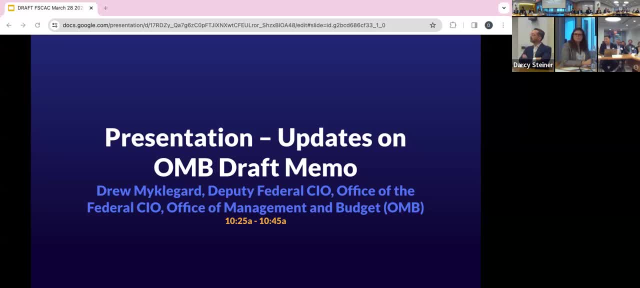 And it provides the government an ability to be able to understand their technical architecture, their understanding of cyber hygiene and how well they actually perform in the delivery of their responsibilities that relates to cybersecurity And as they move through that process, the initial live SaaS authorization. 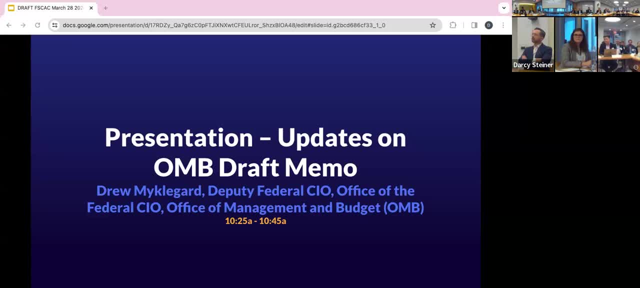 allows us to be able to use certain functions, features and expand to certain sets and certain volumes of information. And based on that, based on that initial authorization, and once they move forth with the FedRAMP authorization, that's when the you know. 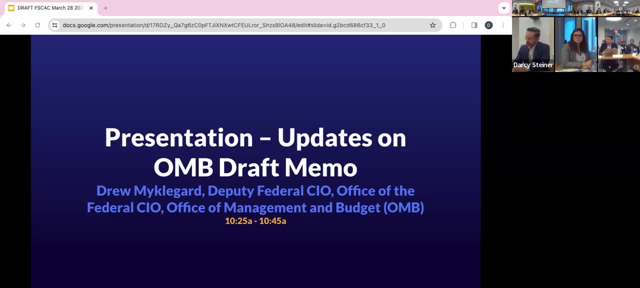 those guardrails effectively come off to allow them to be able to go through and realize the full functions and features of that SaaS offering. We found this to be incredibly helpful for the majority of the SaaS solutions at GSA, particularly those that are low impact. 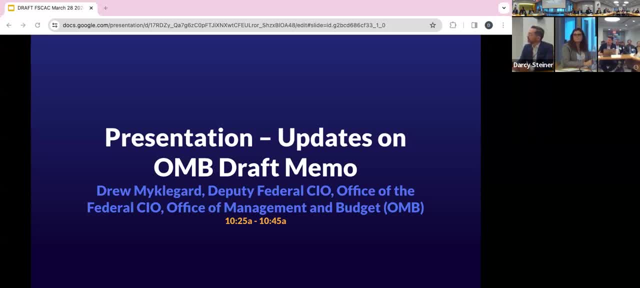 They've all facilitated to initial live SaaS authorization and then promoted into a FedRAMP tailored authorization or FedRAMP low or FedRAMP moderate authorization. So this agile notion, I think, is really important because it does go through and talk about an inheritance. 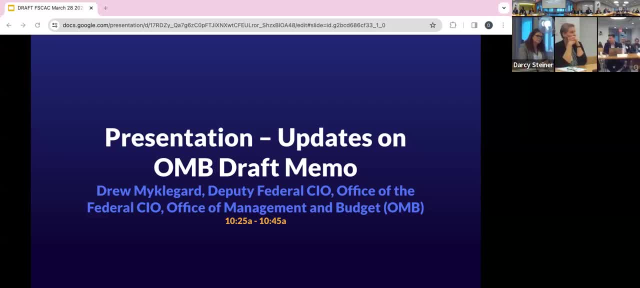 leveraging existing infrastructure. its platform providers or FedRAMP authorized. It does allow for the challenges that John was talking about relative to revenue recognition and be able to go through and justify to their boards and companies around continued investment to be able to go through. 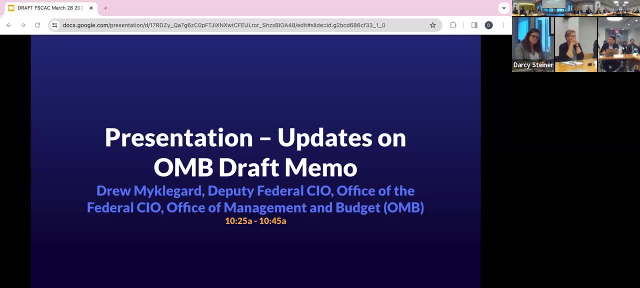 and you know, justify an ongoing commitment to the FedRAMP program and the changes that higher level authorizations would typically require. Well, I think that's a really powerful idea And thank you for detailing the process that your CISO shop uses at GSA. 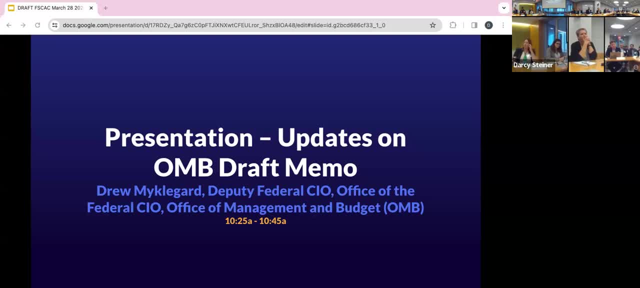 I wonder what it would take to encourage other CISOs or CIO shops to consider a model like that, doing incremental risk assessment. And then I also wonder what's the connective, what, what's the layer between having that process at more agencies? 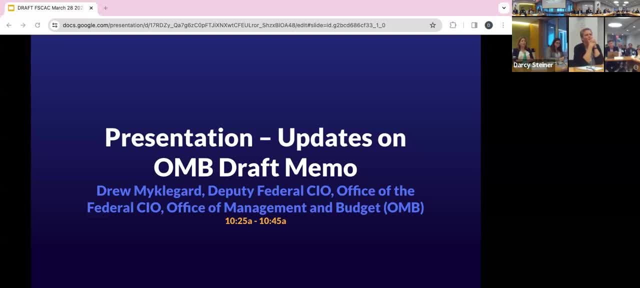 if it makes sense and small businesses knowing about that and being able to pursue contracts at those agencies where there might be a path available for them to, while they're getting FedRAMP, go through an incremental risk assessment process like YSAS. 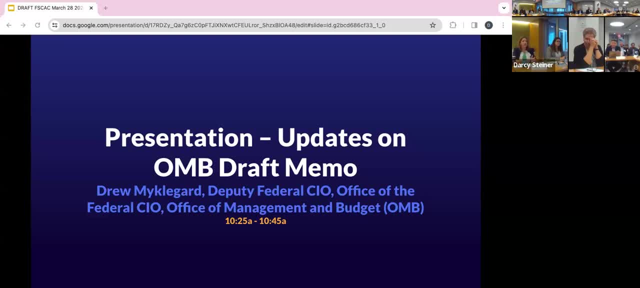 Because this is something that you've heard of or you've encountered, you know, when you are exploring government contracting opportunities. So I think the question is for me again, John from Bluescape, I'd have to learn more about what Beau's describing. 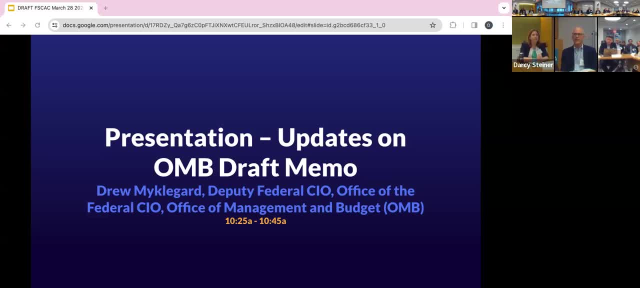 I will go back to the point that Bill made, that the interesting thing about selling SAS and why SAS is so great, for you know why it's taken over the software application world is. in the commercial world you start small. You start with a project team. 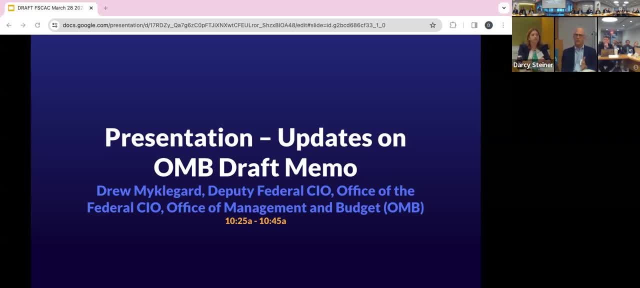 You start with 10 users, 15 users- You charge a per user per month price. Maybe you lock them into a one-year contract. that's very flexible, that people can scale up and true up at the end and as usage expands, It still means that. 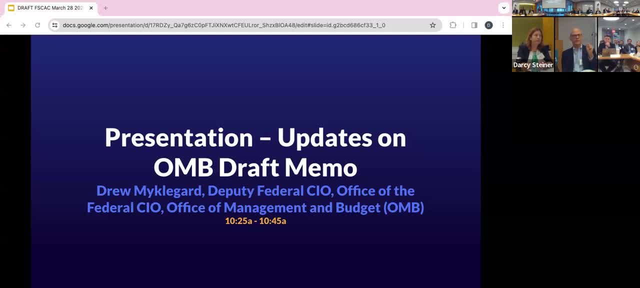 that first touchpoint into an agency, that first touchpoint into a customer, is $5,000 sale. I don't know, I'm taking a random number but it could be even lower than that. Yeah, probably a little higher, But the point being, 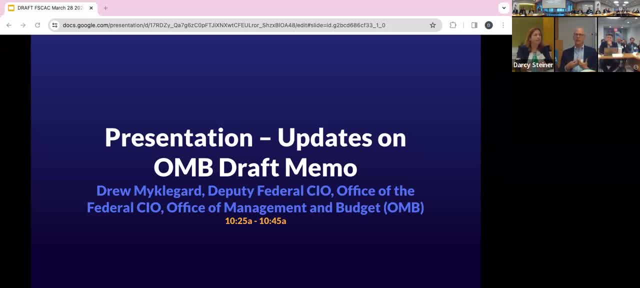 it's still So. I'd have to learn more about Beau's commitment. People want to try before they buy. They put on 15,, 20,, 30,, 50 users. It's There's still some sort of I think. 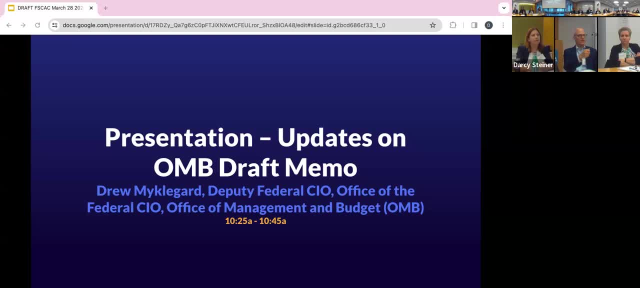 either marketing or incentive. piece missing because the business case has an extended potential to the entire agency. It might- just It might- end up still having to do a lot of work just in an individual agency for just a project team of 15 or 20 persons. 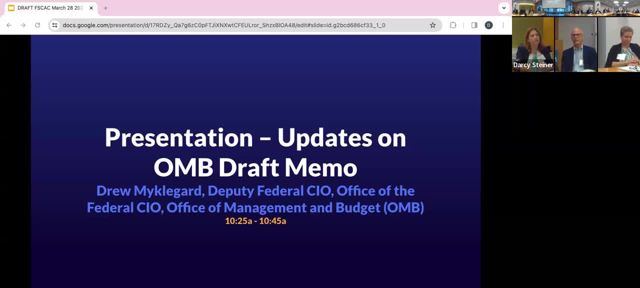 You add tremendous value for that team, but the costs sometimes outweigh. So again, I don't know enough about Beau's process. I don't know if I answered your question, Anne. You did, yeah, You know. I think it's something. 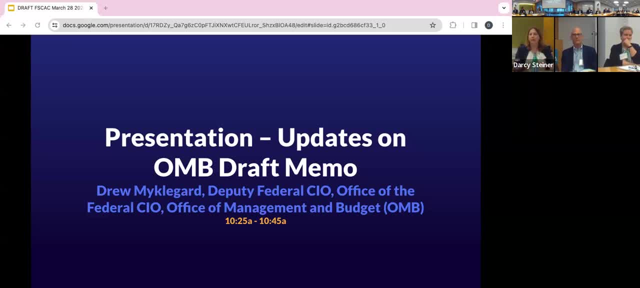 that would be helpful to consider, Like is the model that Beau is describing, something that could be scaled out to more agencies? Is there a way of better reaching small businesses? It sounds like you're describing kind of like a free, freemium or starter model. 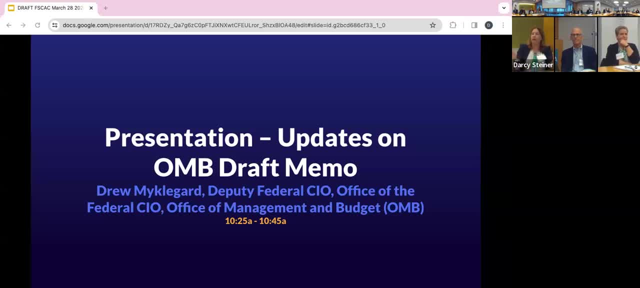 that would lead to an enterprise level contract which would then start some sort of security monitoring process, I guess just to completely broaden the scope. Nalman, from the SBA's perspective, is this something that SBA considers or is part of the strategic planning process? 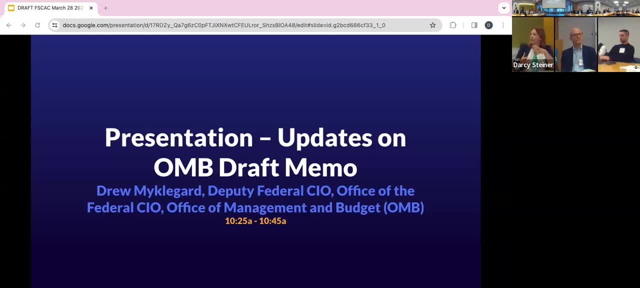 to assess specific strategies for enabling small businesses to have more incremental on-ramps into agencies based on 15 licenses that then grow into a larger contract, or parallelizing FedRAMP authorization with an incremental risk assessment process. Is that something that's So? I don't think SBA currently has. 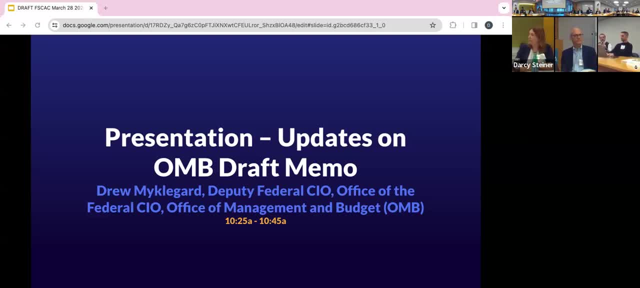 something specific for FedRAMP, but just the model of allowing small businesses to grow and incrementally achieve an end state is a model that's been applied by SBA for many different programs. So I think that there's a lot of opportunities. I think, to rely on the government. 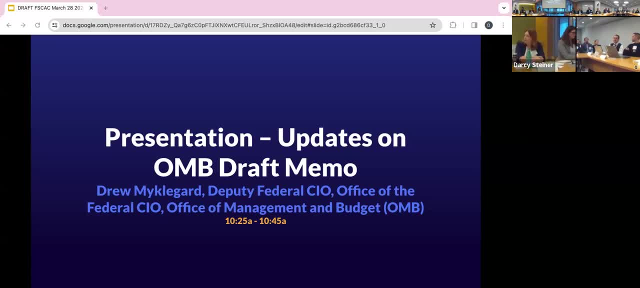 contracting business development side of the House of SBA and see what we can do. I do, I'm sorry. one more point And just interesting because you did bring up the CBER and SCTR process And I've known other small business. 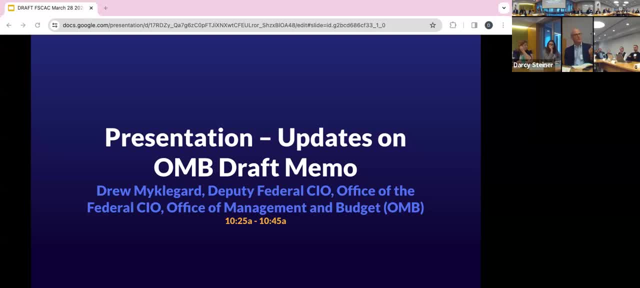 other small CSPs who've tried to, and maybe just an idea throughout. I don't know legally if it's possible or how any of this stuff works, because I'm not a government person. unfortunately, I know another- actually two other small business. 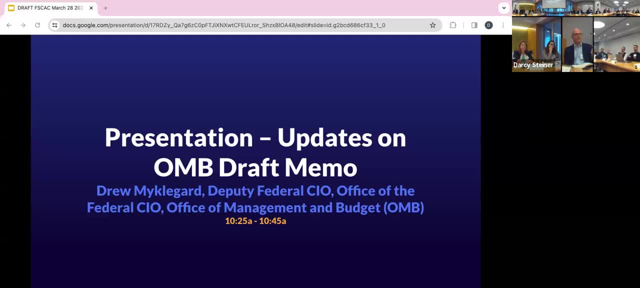 that either got or tried to get SCTRs or CBERs specifically money set aside to help with the FedRAMP process, So that was the deliverable as part of the CBER. Now that's not the way most CBER announcements. 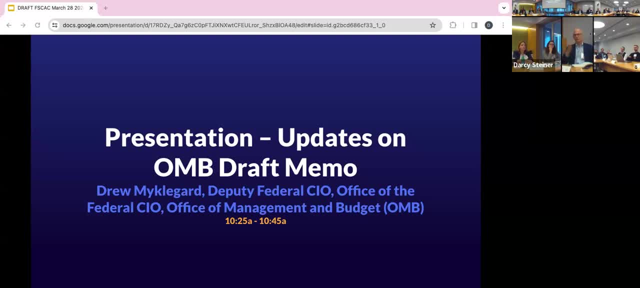 or comps come out. They come out to solve emissions, solve a problem. but the barrier to sometimes solving the problem is you don't have the accreditation ahead of time. So there's this, like if there was a some sort of CBER milestone. 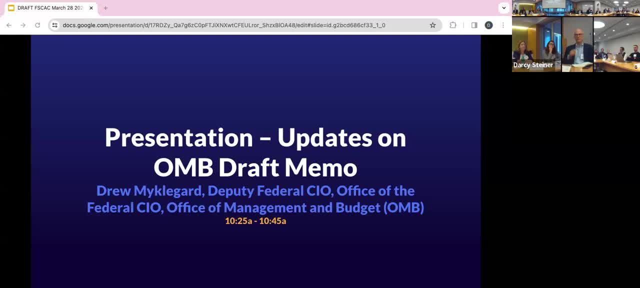 and fund set aside or assistance to help somebody who wins a CBER get through the accreditation process. maybe that's an idea. Again, I don't know if that's even feasible or I think it's something we're looking for. Sorry to interrupt. 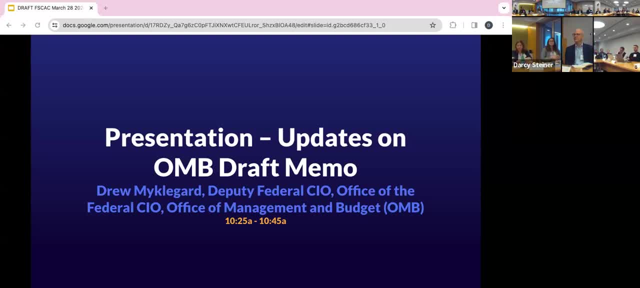 I did want to do a time check. We've got about one minute left on this. I wanted to make sure that you got all of your points. Yeah, I was just worried I wouldn't like nobody would respond. Yeah, it's just. 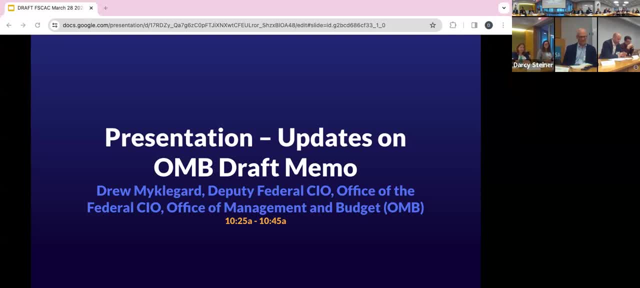 you know how their day was when they come home from school. No, thank you The last two and probably take these offline. The first one is just cost around the FedRAMP process And there's two that we look at from OMB. 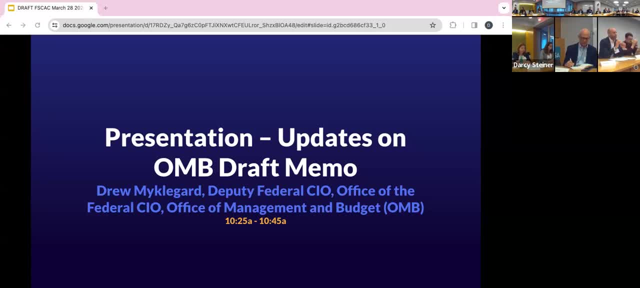 And just in full connection, we have, like, only urban legends and anecdotal information here, but it's how much it costs for an agency to bring in a CSP, including ongoing or ongoing con mon. I think, Jackie, you have probably some of the best numbers. 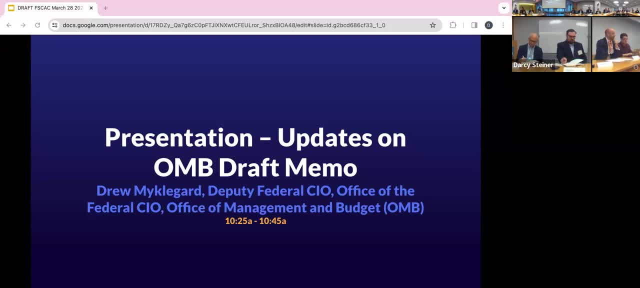 And then the other one is how much it costs for a CSP. And the challenge is like if you're a somebody that's done a lot of work with the federal government and you understand the RMF framework and understand what you're going to go through, 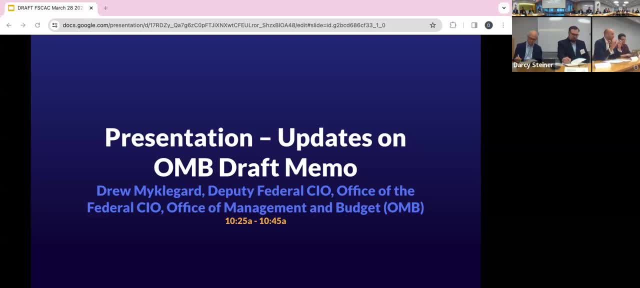 like it's always faster. If you're an amazing Silicon Valley company that's going to change the world and, like you, don't understand the way that we look at risk, it's a little bit harder. So we're really trying to dig in what the FedRAMP costs are in a consistent way. 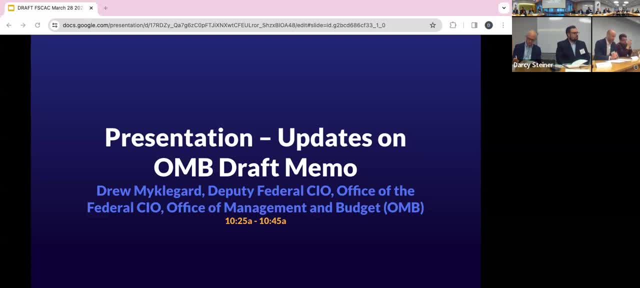 And then the last one, and this would really- this is more than anything just a call to help us make OMB better and the program better is around metrics. So what metrics can we put out that aren't easily gained? that would show both transparency on our side. 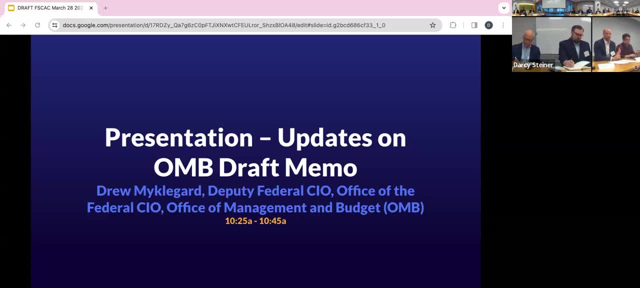 allow us to improve the program over time and then provide the most effective and most value to CSP. So that you know, like John, you talked about like signaling in different ways. I feel like if we can consistently signal through the right metrics, 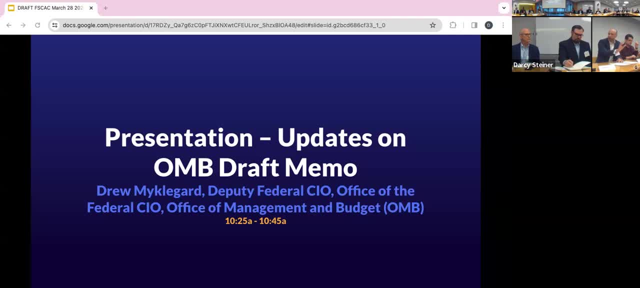 like. this is what. even though dealing with the federal government isn't for the faint of heart, this is what it really looks like, and looks like over a couple of years. So those are my three. The first one's great. I wish we had more time. 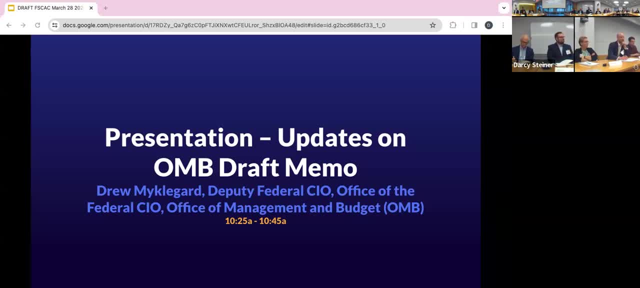 but Michelle's going to keep me honest and not let me go over- but the metrics would be great for us. So I think, just you know, in terms of cost, I think, as well as the metrics, I think we need to be thinking about this. 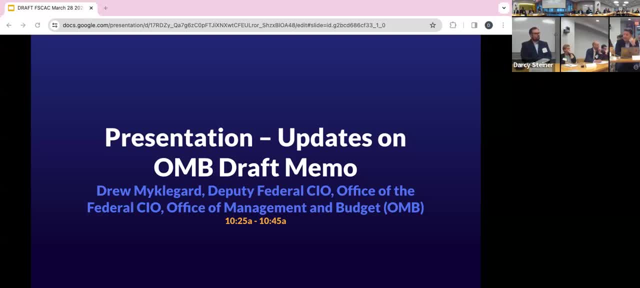 both in terms of repouse vendors and agencies, Yeah Right. And the benefit and effectiveness I think need to be across all stakeholders that are engaged in this process. You know, in terms of metrics, I mean, I think we can probably sit down. 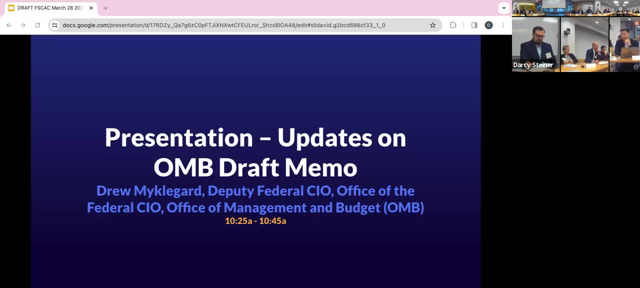 and talk about. you know what agency specific metrics would be, especially when we're having discussions around risk and security and not wanting to lower the bar to be able to go through and facilitate. You know we have incidents all the time, right? 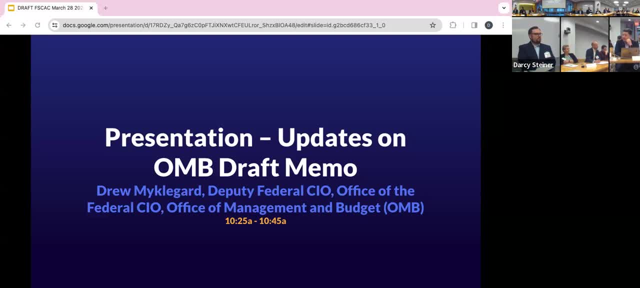 We correlate incidents to that may have authorizations in terms of the level of quality of authorizations relative to the expected outcomes that we intend particularly relative to this process right. We see fewer incidents corresponding to federal authorizations versus other type environments. I think there's a value. 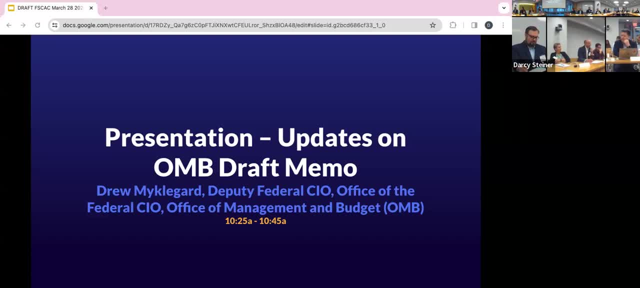 and a story to be told there that I think we're probably not taking advantage of. Agreed And sorry, Michelle, but I wanted to just say one additional point that I'd add to the cost conversation, Drew, is that it's not just the cost. 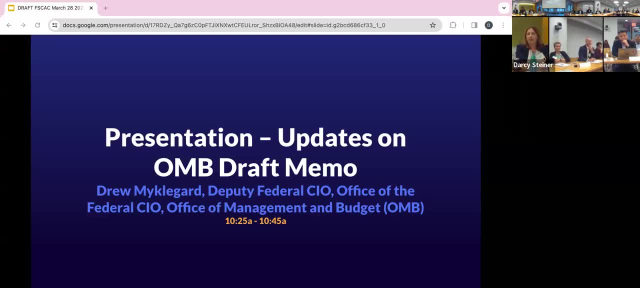 of doing the FedRAMP stuff. It's the cost of taking a system in some state of maturity and bringing it up to a level system security maturity and security ops. And all small businesses are coming from some place. They need to get to a place. 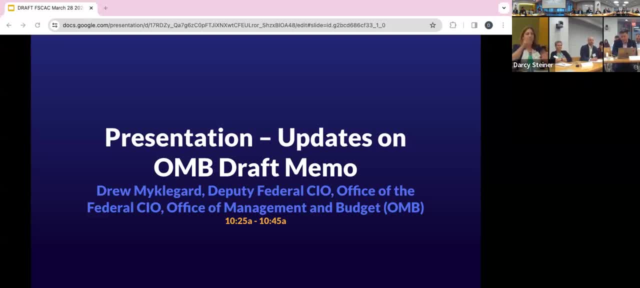 where we have common language around, what good enough for government means, But the cost there is like it needs to be aware of where small businesses are coming from Once they've reached a certain level of maturity where they think they could handle federal scale. 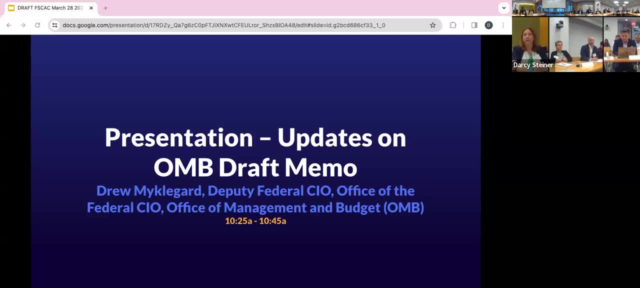 and a contract, then it's: what does it take to bridge the gap? to go from some database that everyone can log into to- oh wait, we have to encrypt data at risk, We have to do like financial management, It needs to be independently audited, et cetera. 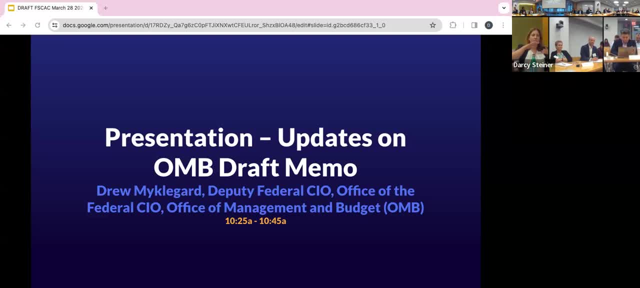 So I think, to make sure that we're measuring something meaningful, it's understanding where small businesses and the ecosystem we're starting from, and then the cost to get up to that necessary maturity level. If I could have 30 seconds, Bill Hunt, SEC again. 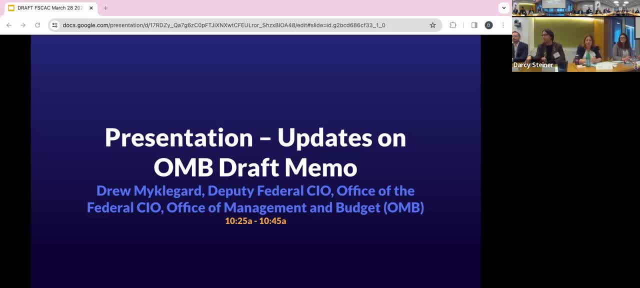 When we're talking about the agencies and the financing on that side, I will flag that us small agencies have very unique needs and we are very hungry for these sorts of tools. We do not have the budgets to necessarily take them through the process. We have a flat budget. 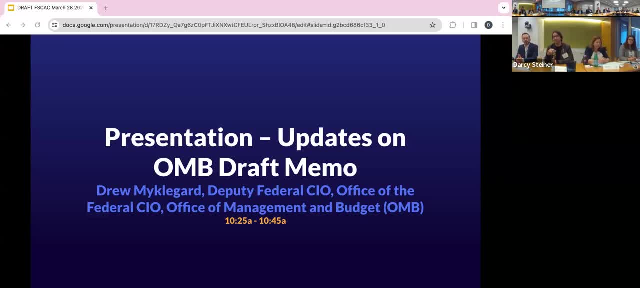 from last year to this year. So I don't have dollars to do any of this stuff, but we desperately need them. We desperately need these solutions today and we can't really wait for them. So we are eager to do labs to try this stuff out. 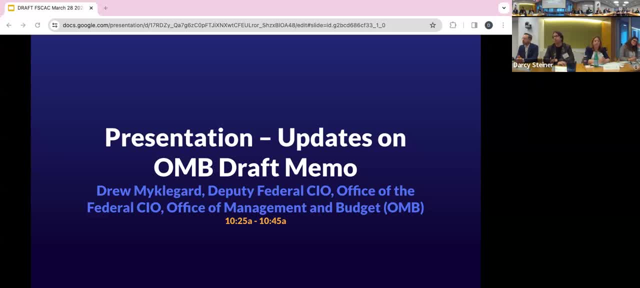 but we do not have the budget to execute. Is it the FedRAMP? Can you ATO them, Or is that even too expensive? ATOs are very just as expensive. basically, That's what we have, even at a bigger agency with more research. 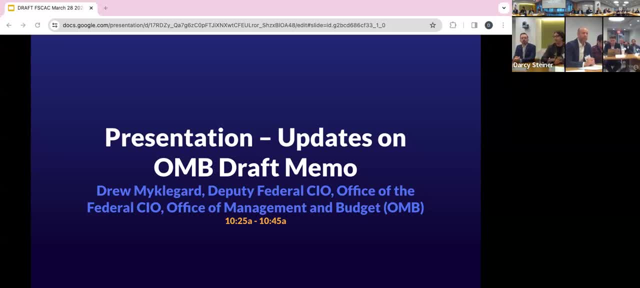 Which is also why we need the exception process, Which was something new. Yeah, just very well, by the way. Good, yeah, Appreciate that. All right. Well, thank you, Drew, And thank you to the committee for a very engaging conversation. 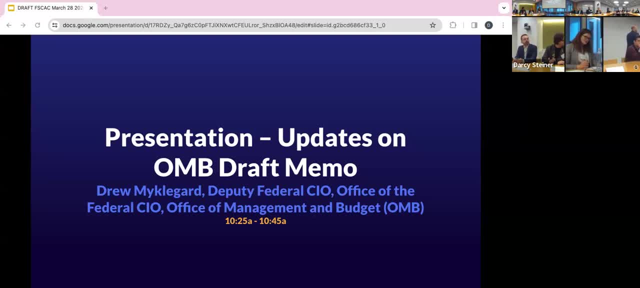 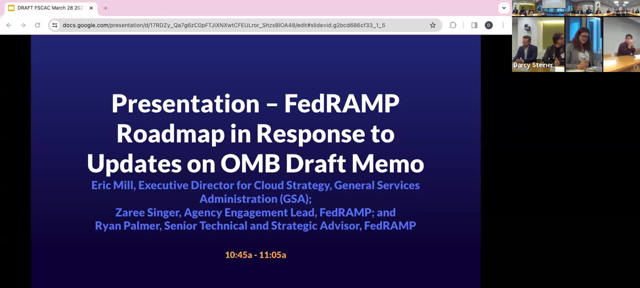 We definitely appreciate it. Now I'd like to welcome to the floor Eric Mill, who is now the Executive Director for Cloud Strategy at GSA, Dari Singer- she is the Agency Engagement Lead for FedRAMP. And Ryan Palmer, the Senior Technical and Strategic Advisor. 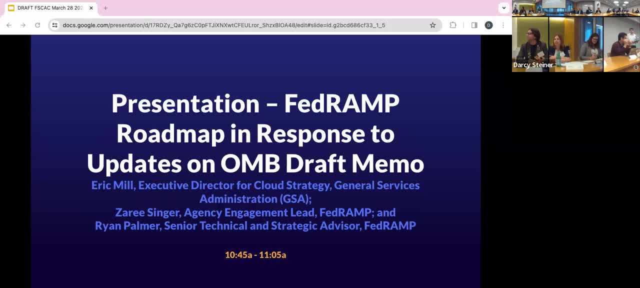 at FedRAMP. They have kindly joined us today to provide additional information on FedRAMP's sort of runs, so that they won't be memos, Eric, sorry to keep you from joining us. Thank you, Thanks Brett, Thanks Sarah. 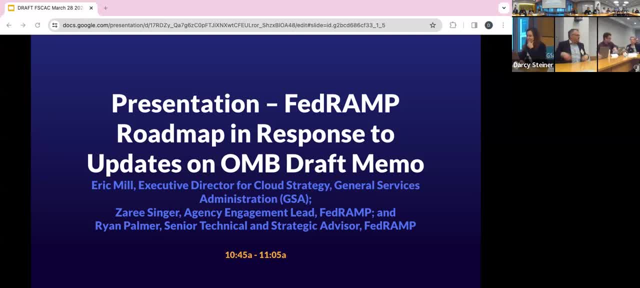 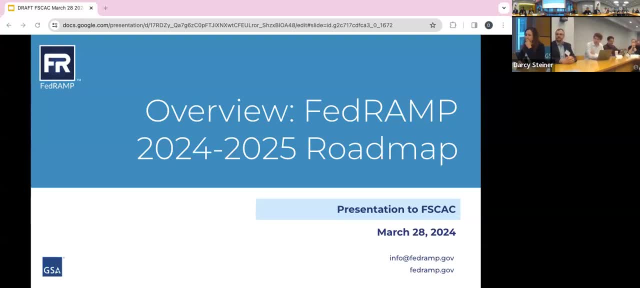 Your seat's about lovely, All right. Thanks for having us. Thanks for the introduction You're mostly going to hear from Ryan, I'm sorry to say, but I thought I'd just give a very brief introduction, So we're going to talk through. 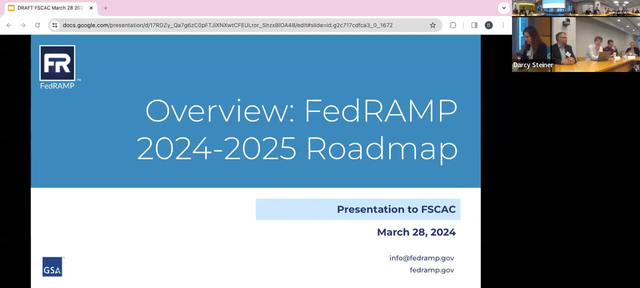 FedRAMP's public plans today in more detail than I think folks are maybe used to hearing from the program looking forward, And this presentation will have some detail. There's actually going to be a lot more that you can find online today. We'll have some posts going out. 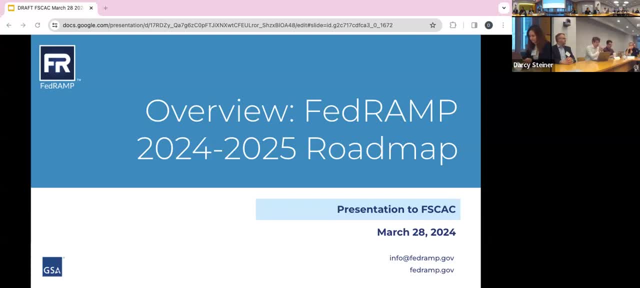 We'll have a roadmap artifact that gets published on the web. So we'll be happy to answer, of course, some questions here, but there'll be more there. You know there's been a lot of focus here on Congress and OMBs. 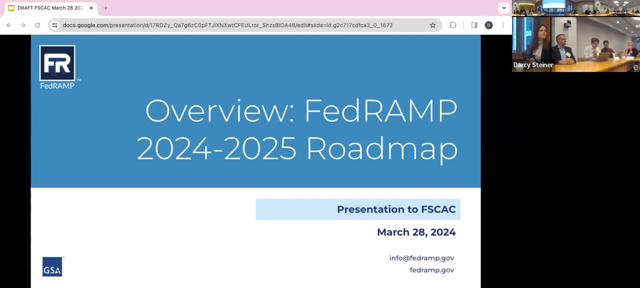 important work on FedRAMP. Obviously, we just talked a lot about OMBs, which is an active item. You know, on the agency side, at GSA, what we really have to do is focus on, you know, on the machine that we have. 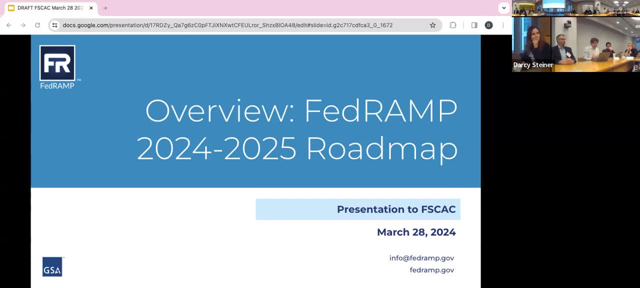 on the implementation, on organizing our efforts, prioritizing what we do, sequencing things in time, reallocating resources, And it's a different problem, and it's a very important one, right? So the number one question that you know: 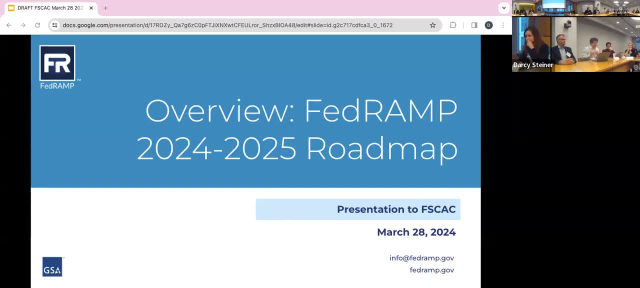 I get when I'm not talking, or the team gets when they're dealing with folks. is you know, how are you actually going to be able to do all of these seemingly infinite hopes and dreams people have for the FedRAMP program right? 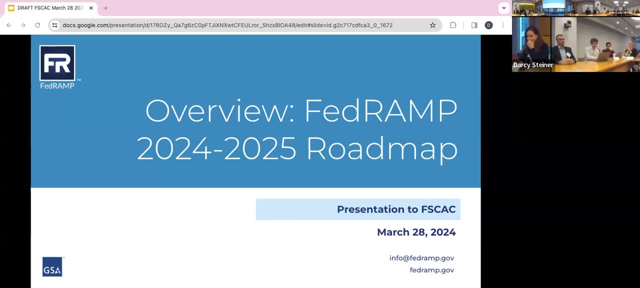 And we do have to actually pick an order in which you do things and which things you're going to focus on first, And we've been engaged in the process of doing that. So, and one of the things I also really want to point to, 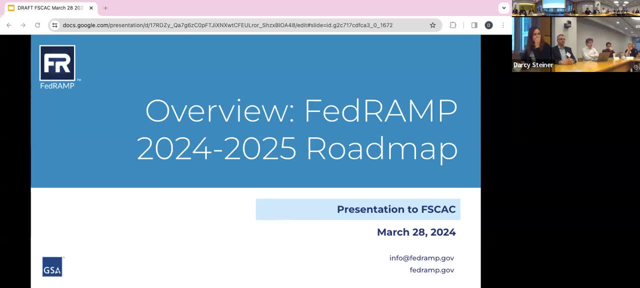 is that you know we're making a significant effort to make sure we're delivering some tangible evidence on a number of these things early enough in the process that we're both showing some momentum for ourselves and our stakeholders, as well as just being able to course correct. 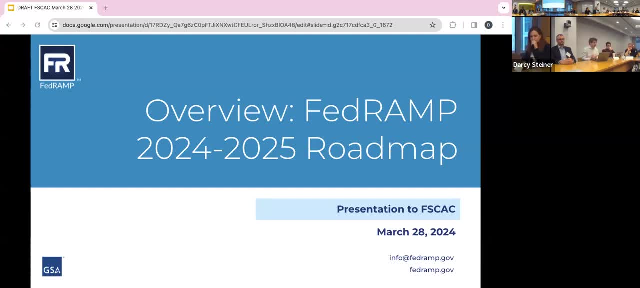 and get feedback so we can change it. Same kind of agile principles that folks who work on software products keep in mind as well. So with that, I'll turn it over to Ryan and Zahra. We'll take a step, All right. 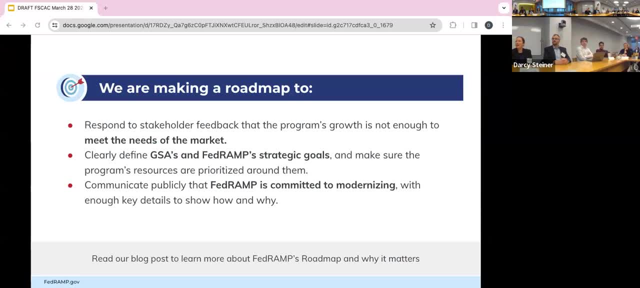 Go ahead. Okay, So, as Eric said, we are today going to be releasing our first big sort of public roadmap. that is a response to all of our stakeholder feedback about many of the challenges that we have, but in particular that really the program's growth. 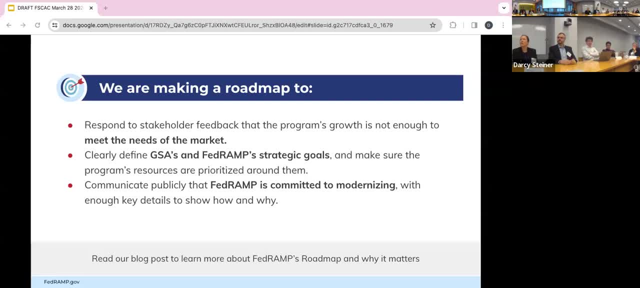 is not enough yet to meet the needs of the market. It's meant to organize all of our work around a clear set of strategic goals and make sure that we're prioritizing around them, And it's also meant to really communicate publicly that we're committed to modernizing. 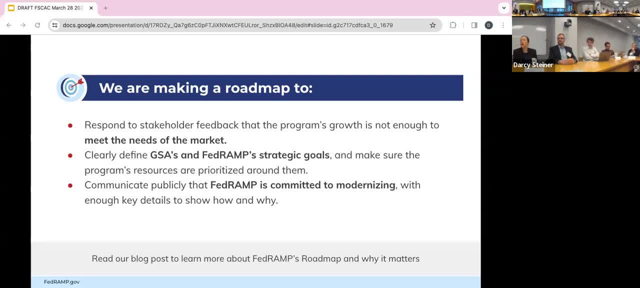 with enough key details to show how and why. So, as Eric mentioned, there's a little line here, but we're going to be posting a blog later with a lot more context on that today. You can go to the next one, Darcy. 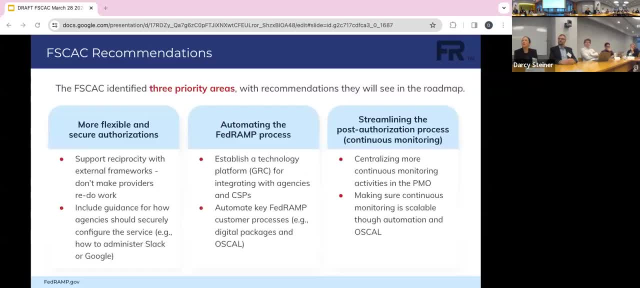 Thank you so much. Okay, So we reviewed the recommendations of this group, So thank you all so much for that, And we are hopeful that you will see in the details of the roadmap many of the recommendations that you put forth. So, in service of more flexible. 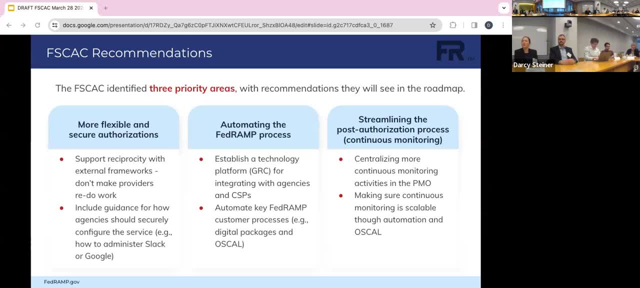 and secure authorizations. we do intend to support reciprocity with external frameworks, with the ultimate goal of making sure that cloud providers do not have to redo work just for veterans. We also are going to make sure that we include guidance for how agencies can securely configure their services. 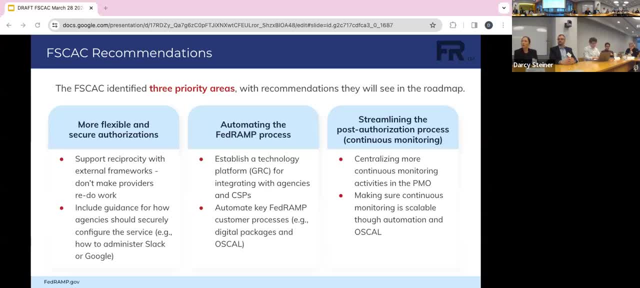 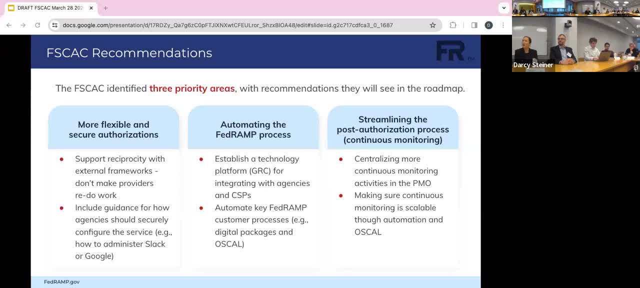 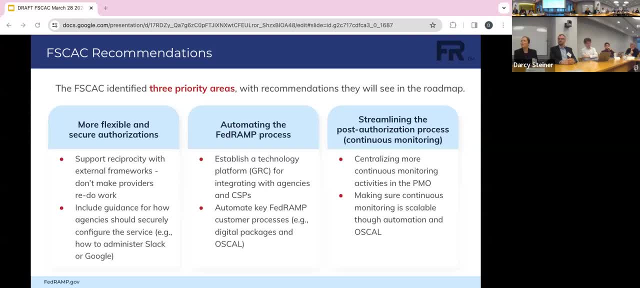 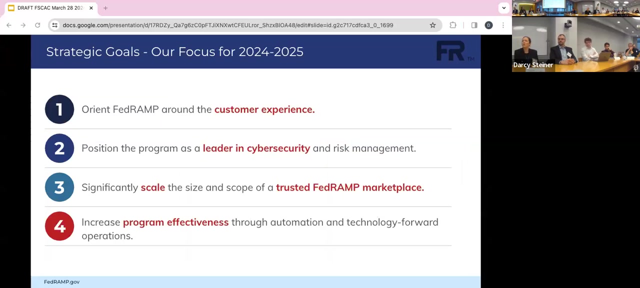 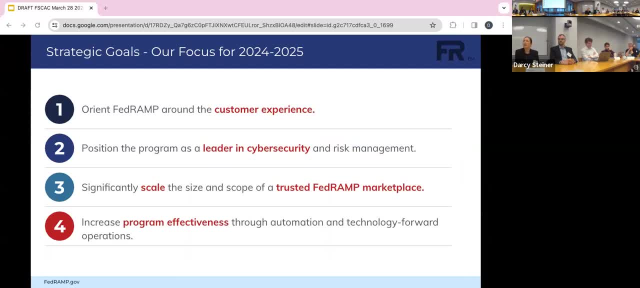 one is really orienting FedRAMP around the customer experience, and in a different way than we have before, so making sure that we're really clearly and regularly, at a regular cadence, identifying what our customers challenges and obstacles are and then being responsive to those, and this is going to include taking more of a stance on things like time and costs, in a way. 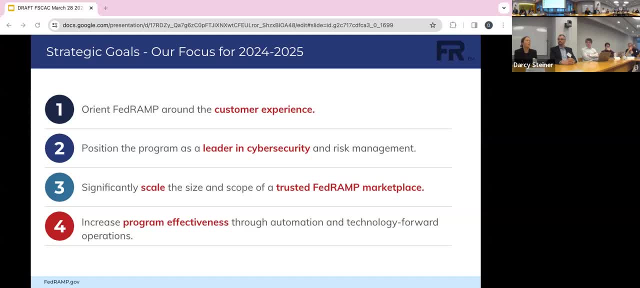 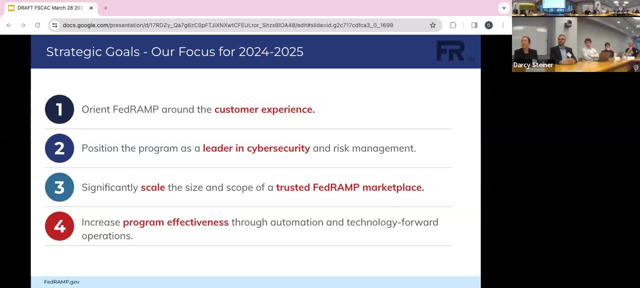 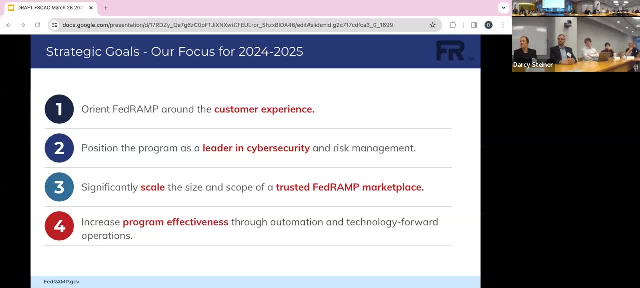 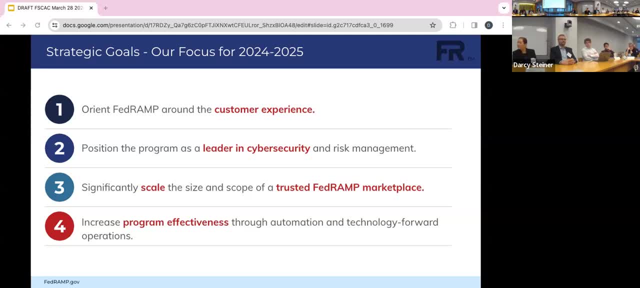 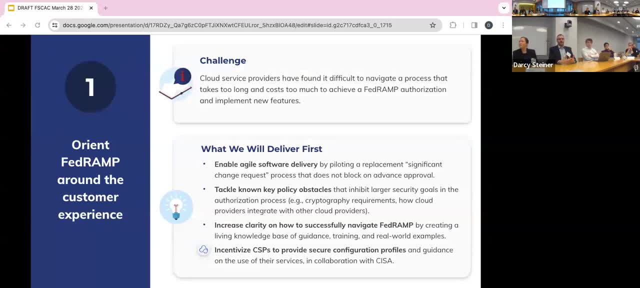 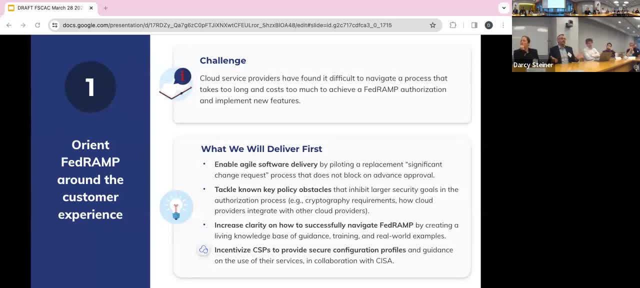 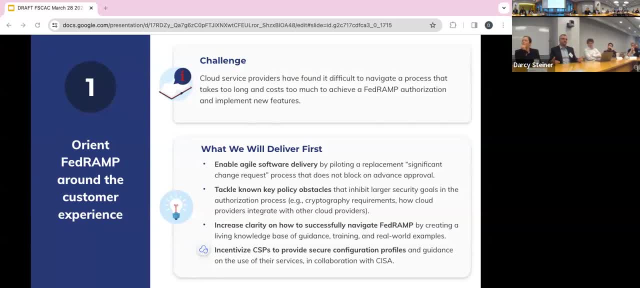 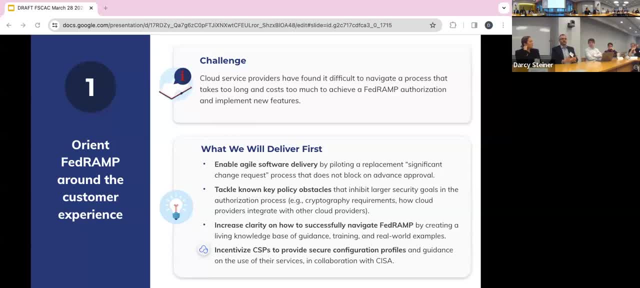 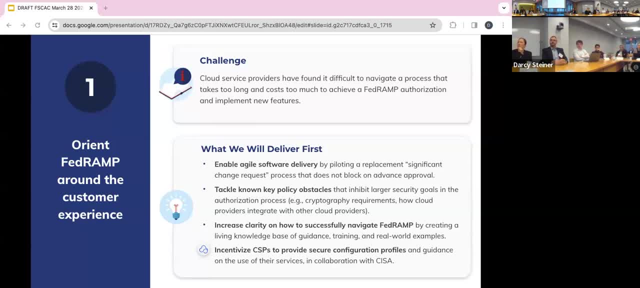 of those changes could probably be accommodated in a non-black way. um, we also want to look at engaging on known key obstacles that the cloud service provider has had over time. these have been consistent things, um with boundary guidance, mainly with external services, but also looking at 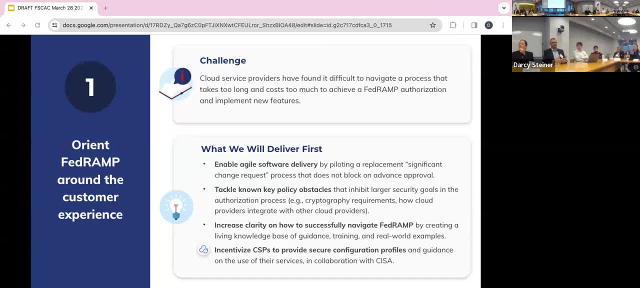 like some of the cryptography challenges that people have dealt with, where you're asking: do i need to be compliant or do i need to be secure? how do i navigate that? we need to provide better guidance and help people navigate that from a navigation of bedrock in general, we're 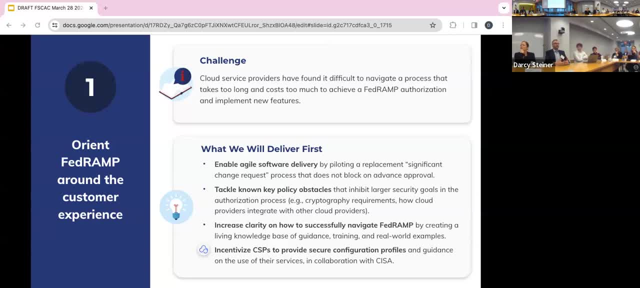 going to work to better deliver on the knowledge base and other information. we understand that our consumers aren't just isos and isms. these are people who have technical backgrounds. these are people in three paos. how can we get better guidance and make sure it's available to everybody in the right way? 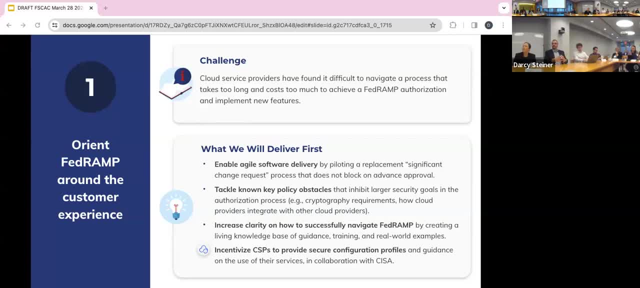 so we are speaking to them and when they start that federative journey, it's much easier. um from this group, i want to call one thing that we've heard a lot about, and this is secure configuration profile. so now we have a marketplace listed cloud service. how do i configure that? i know gsa has. 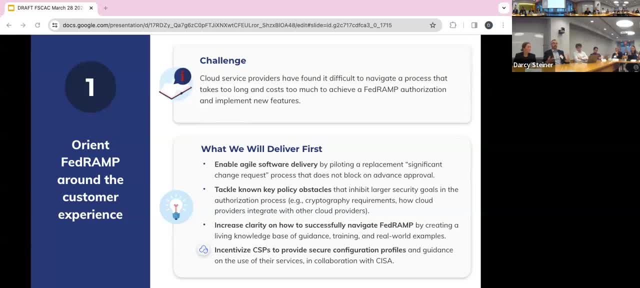 done a lot of work with some vendors to bring in and say, hey, this is how we're going to configure this. how can we scale? that? sys is doing a lot of great work with scuba, so we want to partner with the sys and figure out how we can make that approach scale out and that can benefit both. 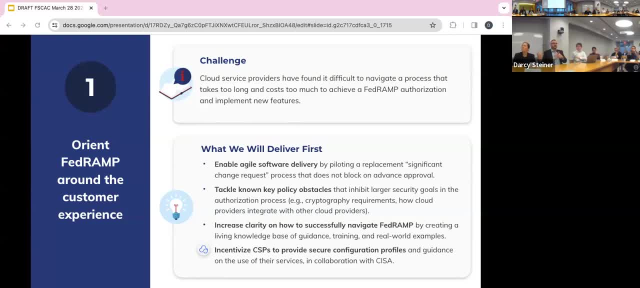 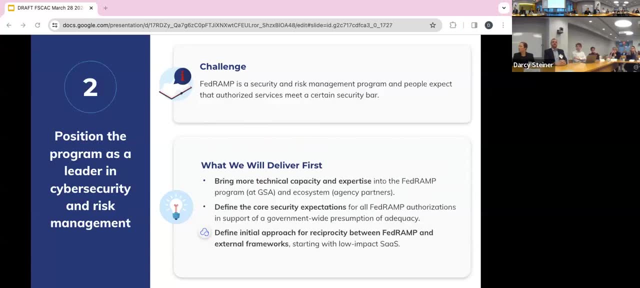 agencies using a service, but also cloud service providers who may be leveraging, you know, the sas solution as an external service next time. um, the other thing we're going to be looking at is being more of a trying to be more of a leadership role in cyber security and also taking, maybe in a more 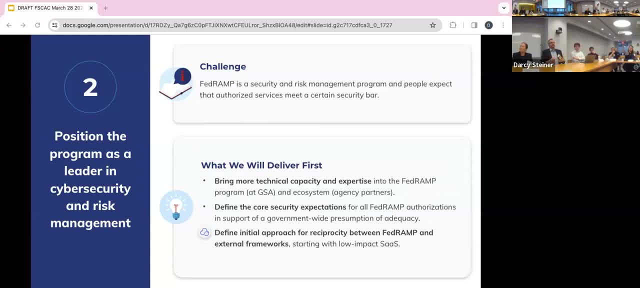 opinionated view. um, one thing we want to do is really make sure that bed ramp has a meeting within the marketplace. i know right now there's, I think there are a lot of companies that would want to have a meeting with a lot of people. so one of the key things that we're going to be working on is going to be the 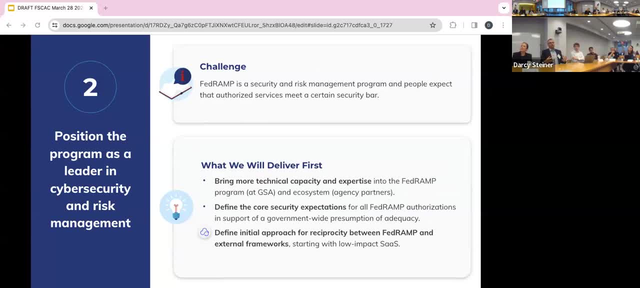 in-house employee. um, um, one of the first ways. one of the other things that we're working on is to create the expertise expaps right. so we're going to be investing in um, one of the first ways. one of the other things i think we're going to be working on is is ceremony. 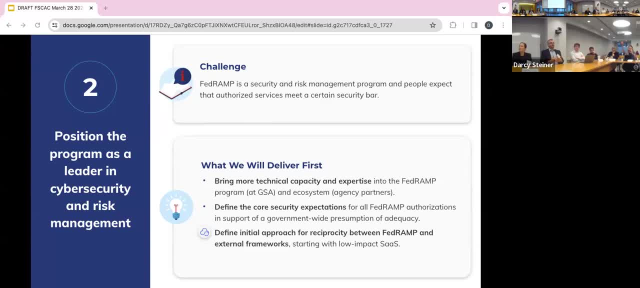 we're going to work on is reciprocity. We're going to start with something that we feel is achievable and that is reciprocity at the low baseline level of services already on, like that pass. or I ask very much, in line with what FOA with- sorry, GSA's process? So a lot of these. 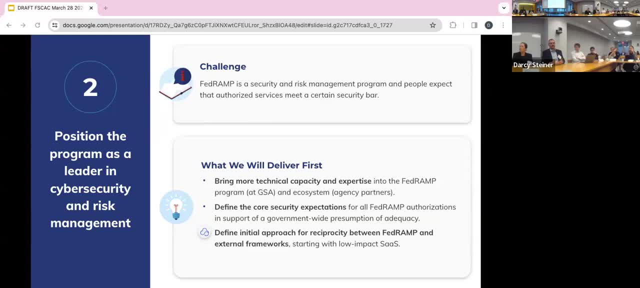 frameworks have similar assessment needs, right? If you've already done a pen test, can we use and leverage some of the artifacts? If you've already written how you're addressing some policy statements, how can we incorporate that work and potentially even assessment work, so we don't have 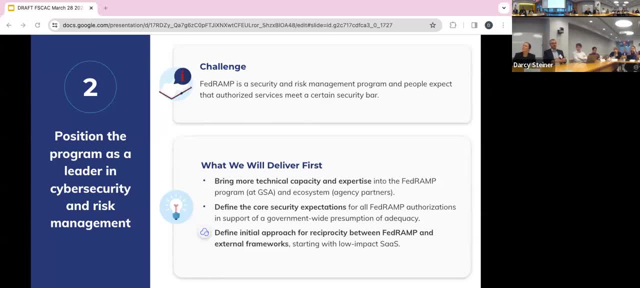 to do it again, especially if there's lower levels. I think there's a lot of opportunities to partner with, you know, other organizations to figure out how we can norm those baselines or maybe tailor those baselines to better reflect practices without lowering the bar of security. 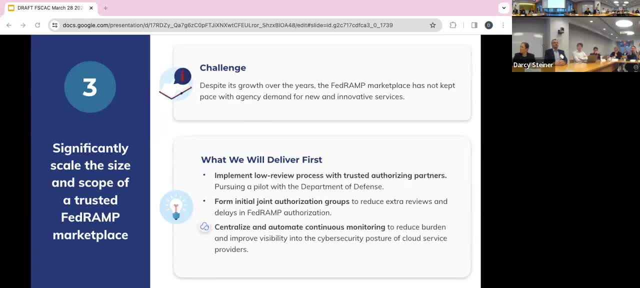 Next slide. We want to grow the size of the trusted marketplace. We had a lot of growth of, you know, all those different sorts of services, but the focus on SaaS and the a lot of products aren't really even available, sometimes in a 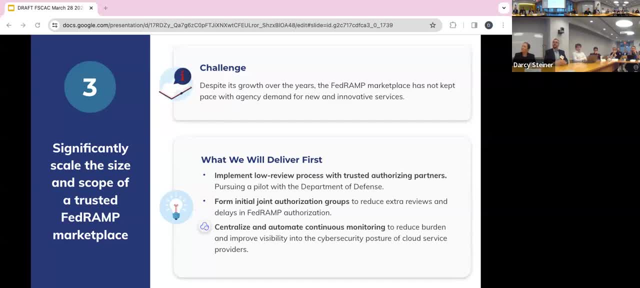 non-cloud offering database when we look at things like emerging technologies. One of the ways we are going to do that is work with trusted agency partners and also join authorization groups to kind of get more right. Our agency review process is something that takes time. We have more people who are producing those high quality outputs We can get. 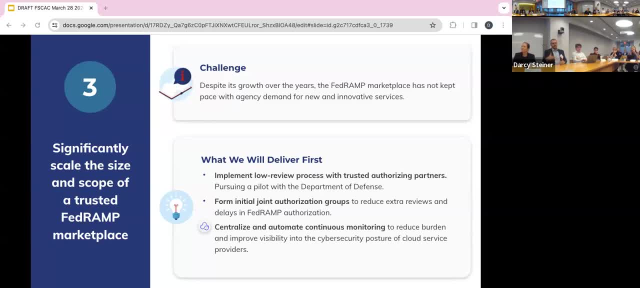 things from employees one to seven times a month. It's part of the process. We have a lot of growth of all the listed on the marketplace easier, which also means that your listed dressing that time to be able to market and sell in some cases should hopefully go down. the other thing we're going to look at: 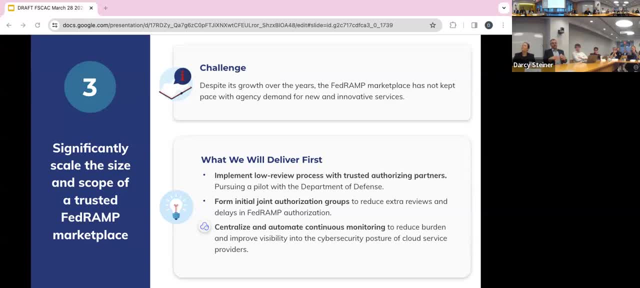 is trying to centralize continuous monitor. by centralizing that a it's a cost save across all these different agencies who are having to do that work a lot of times manually. like this is going to require automation. but also, you know we heard some comments from redhead earlier- how are we? 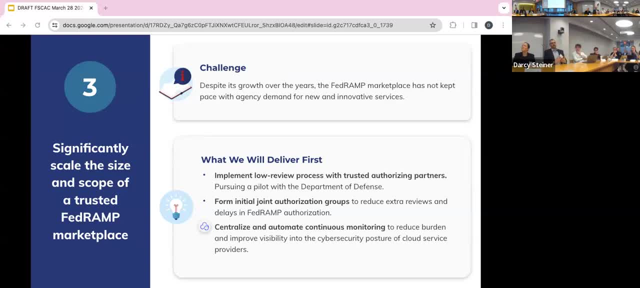 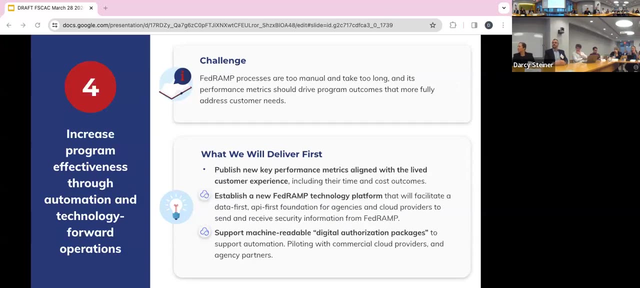 approaching vulnerabilities. if we start doing this centrally, we can probably take more innovative approaches to using that data and being more focused on the risks and real threats and maybe a little less focused on things that aren't really exploitable, because we will have a data format and the last slide- sorry, my last slide- you know, one of the big things we've heard is: 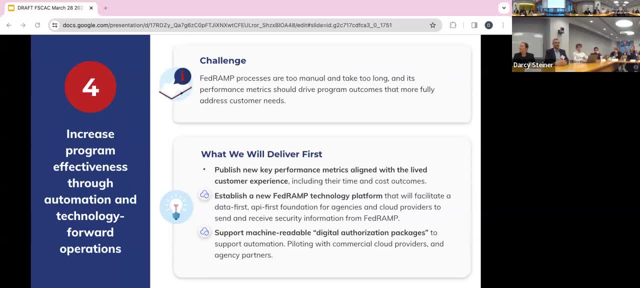 we need to automate. we haven't had a fed19 platform. that's going to be key- and a lot of these improvements. The other thing is performance metrics right, Making sure they're tied to the customers. We are going to be working. you know we've heard a lot of questions today about 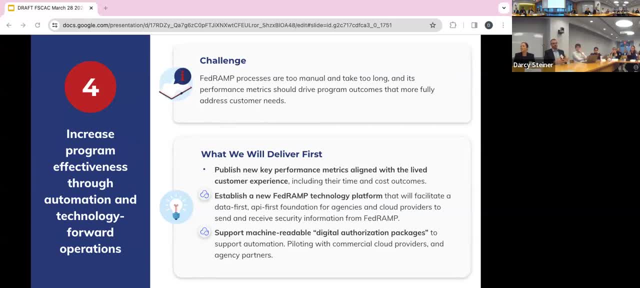 metrics, like what metrics are meaningful to different groups. We want to be make sure our metrics are aligned to our customers' experiences, whether that be agencies or CSPs who are entering the marketplace. We are going to be working to establish a new technology platform. This is 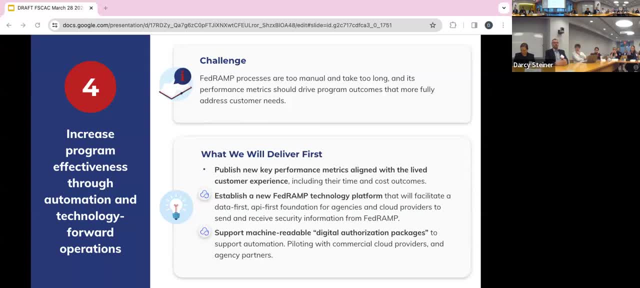 conventionally, I think, called a GRT tool. but we are going to- we're hope our goals for that are a lot more than just hey, we have your compliance documents. Like there's a lot of power in being. 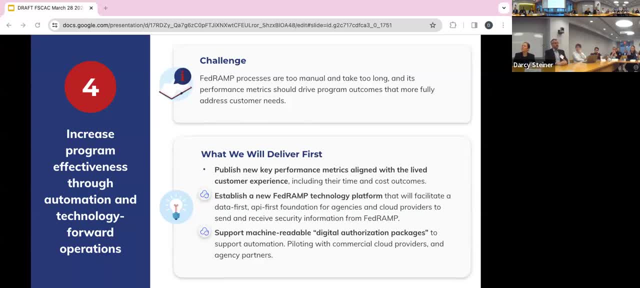 able to automate processes, being able to share data, being able to do things like inheritance, how to make it easier for a CSP that's built on, you know, an IaaS or PaaS? How can I inherit these controls? How do we make sure that these are clear? they don't have to be assessed again? 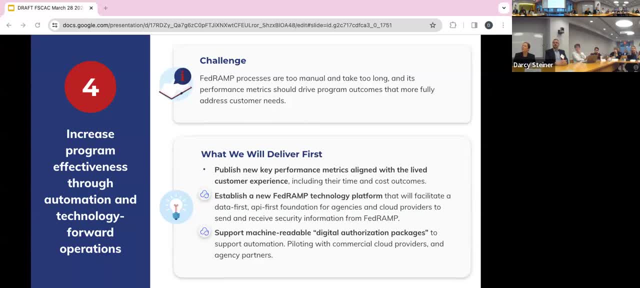 That lowers costs and will drive better outcomes. We're also going to be looking for transitioning to digital authorization packages. Those are going to be backed by the IaaS or PaaS. We're also going to be looking for transitioning to digital authorization packages. 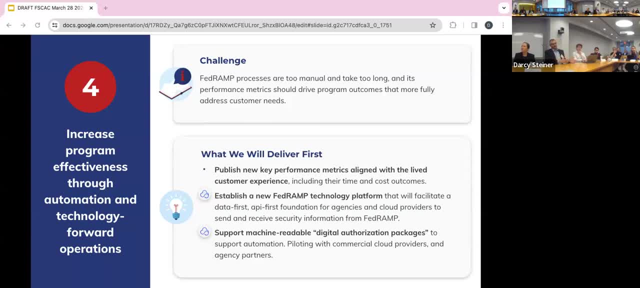 Those are going to be backed by the IaaS or PaaS. We're also going to be looking for transitioning to digital authorization packages. Those are going to be backed by the IaaS or PaaS. We're also going to be working with the community to figure out how to better do that. I think of it similar to 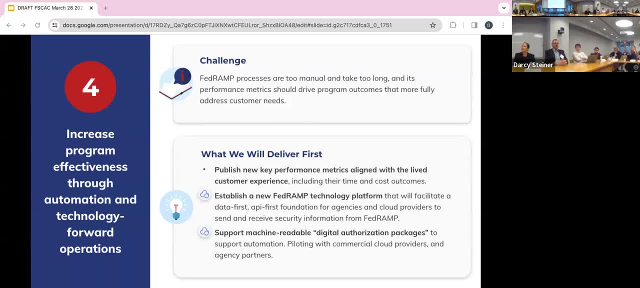 e-filing taxes. Right now a lot of stuff is mailed in. It's uploaded to a repository. People need access. They're having to do the manual processes and manual review work. We start getting those in a digital format. We unlock a lot of opportunities to improve our process. 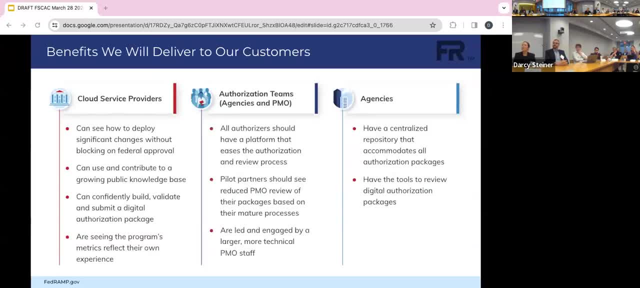 to improve our process. We start getting those in a digital format. We unlock a lot of opportunities to improve our process. We start getting those in a digital format. We unlock a lot of opportunities to improve our process. We spend a lot of time thinking about what the world will look like for FedRAMP as we go through. 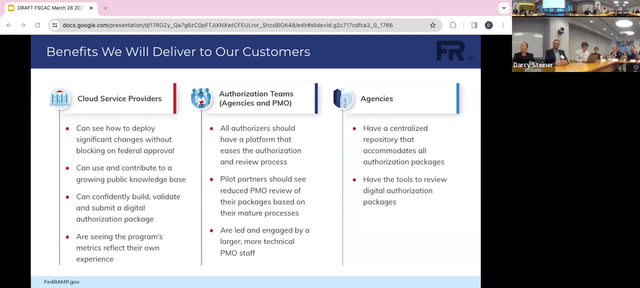 this work For our cloud providers. we expect that they can see how to deploy changes without being blocked on federal approval, that they can use and contribute to a growing public knowledge base that provides guidance on how to actually implement controls, with real examples, That they can confidently build, validate and submit a digital authorization package and are 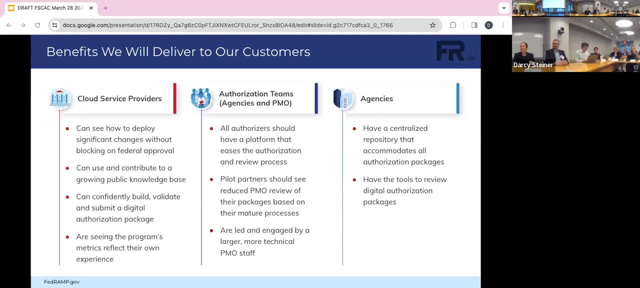 actually seeing their own experience reflected in our metrics and how the program is focused and operating. We expect that agencies will have a platform that will ease their overall authorization and review process. that, initially, our pilot partners should see a reduced burden in terms of our review of their authorization package. 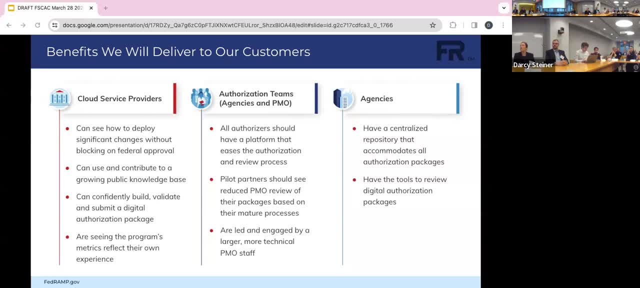 And then, of course, as that expands, more and more agencies seeing that as well And that there's more experienced technical staff. that's part of the organization helping to lead FedRAMP. And then we also, of course, expect there to be a central repository that accommodates all authorization packages. 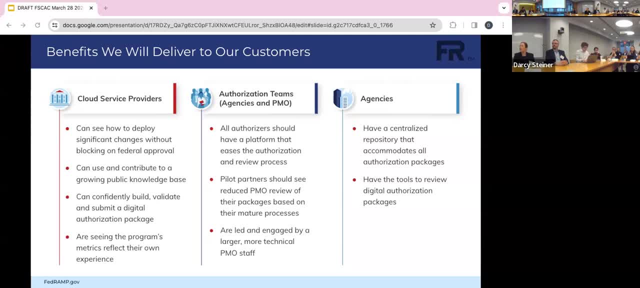 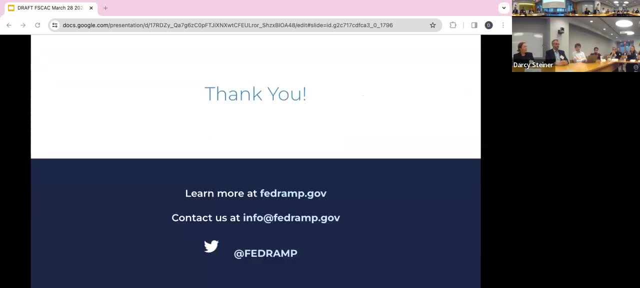 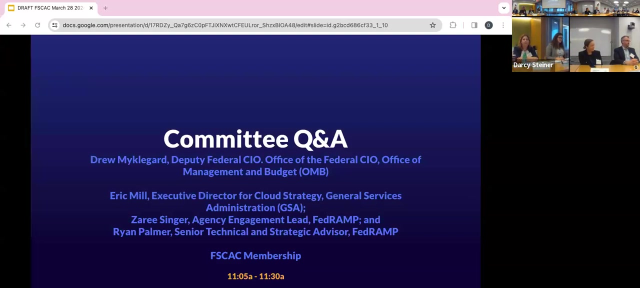 and that all agencies have the tools that they need to do their authorization reviews. And with that I think we'll open it up to any questions. Thank you, Karen, Sari and Ryan. I'd like to now open it up to the committee to ask any questions that you may have from the FedRAMP office presentation. 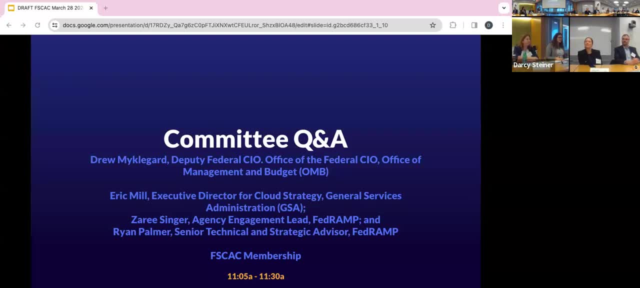 At this time. please go ahead and raise your hand if you have a question, and I'll call on you in the order that you have raised your hand. Sorry, anybody have any questions? Go ahead, Bill, While we still have OMB in the room, do you all have the necessary funding to do all of these wonderful things that you've described? 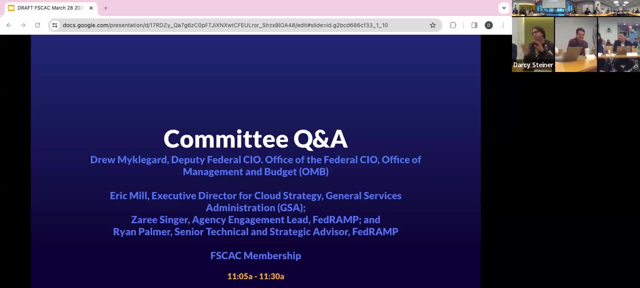 No, I know you have to give the GSA answer, but you can couch that Hal through a wink and a nod. You know, the interesting thing- part of what I alluded to at the beginning here- is that's basically the number one question that we get when we go out there. 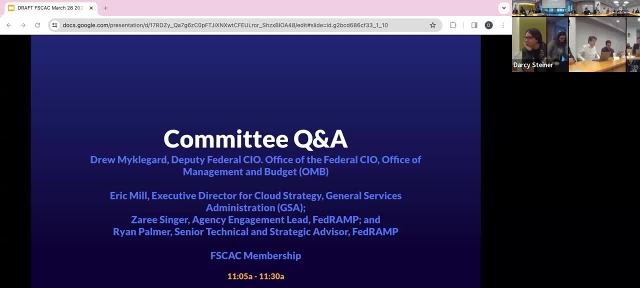 I got that in a public speaking event last week And you know we have a lot of questions. We have a lot of questions And what I said there as well, Sari, here- is that we're very focused right now on making sure that our machine is pointed in the right direction so that you know, as money is invested in the FedRAMP program, people know where it's going. 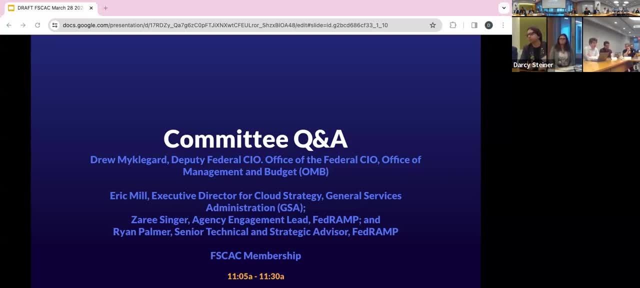 And they know that the outcomes that they're seeing are going to be the things that are accelerated and built on Right. And so I think the work- hopefully what you see in the work that's gone into this and what you'll see coming out of the team- is going to, you know, help to answer that question. 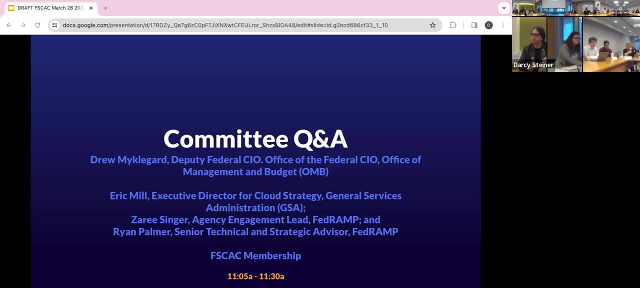 And so that's the GSA answer you'll get from us today. I'll keep a very close eye on the TTS hiring page then I would be remiss not to mention on that topic that we are in fact hiring a FedRAMP director and there will be some information sessions coming up next week with a posting going online later in April likely. 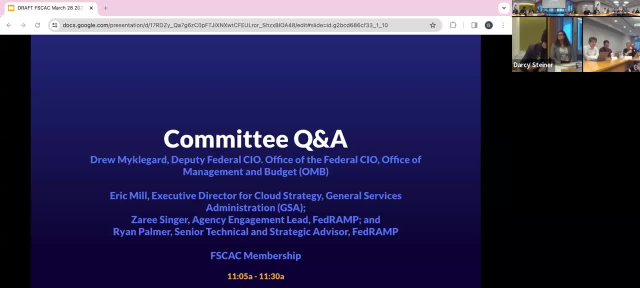 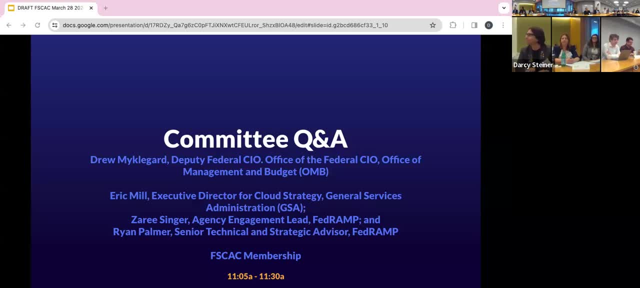 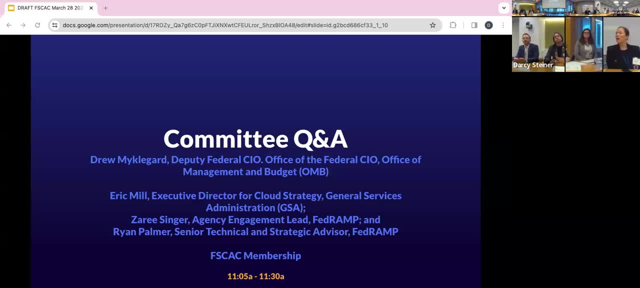 any sense of time lapse. We do, Actually, we have one. We can pull that up if people want to see. This is part of what will be in the public. Jarbessy, can you pull up the last slide? Yeah, right here. 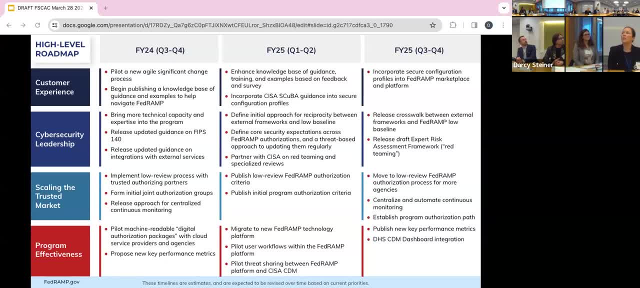 Perfect, Yeah, So sort of at a high level, the items in, of course, the ones that we are first up in priority. So we're working to pilot that SCR process. That's one of the first things we'll be doing And then also focused on kind of an MVP version. 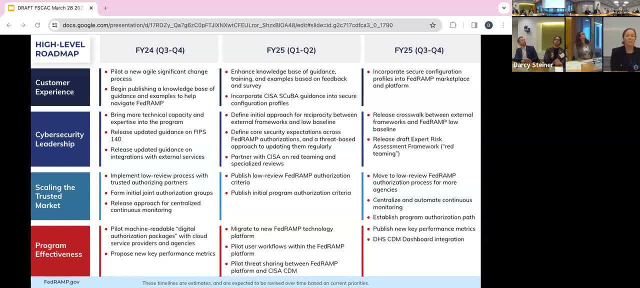 of the knowledge base. Of course, as Eric mentioned, a lot more expertise can be coming into the program. We have guidance updates that are coming. So everything that you see kind of here on the FY24 side is the nearer term things And the way we thought about kind of prioritizing. 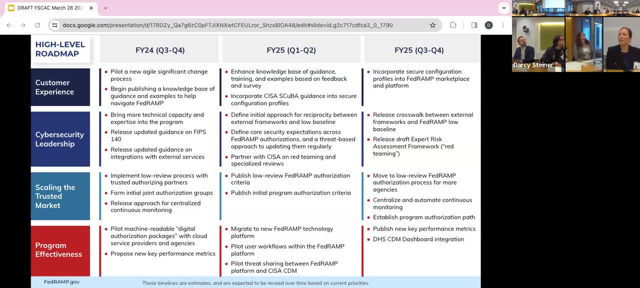 our work overall was things that will increase throughput and capacity. we're doing first, So that is our goal. Great, Jackie, go on. One of the things that I want to call your attention to is one of the customers that we continuously leave out, really, of this process is the authorizing official. 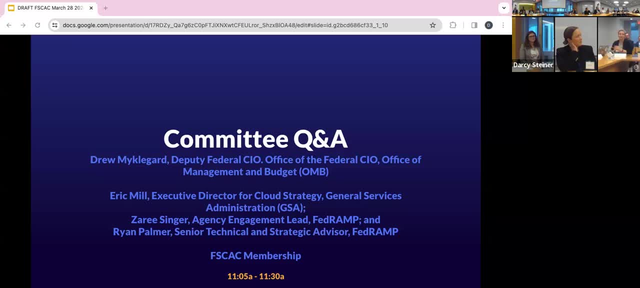 who's using the SAS or the capability right the cloud, And making sure that our GRC is available for them to inherit so that they can build their package, so that they have a shorter road to on-ramp to production. So I wear two hats And so making sure that I have real good availability to the 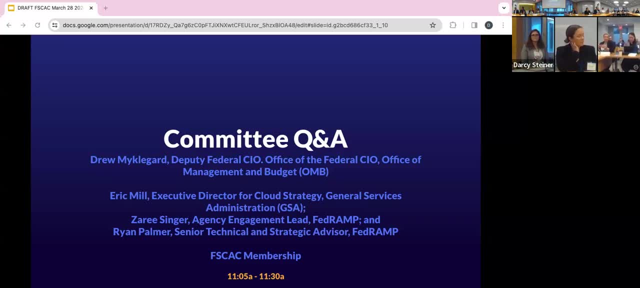 FedRAMP repository, which is not real strong today. Making sure that data is available in the GRC. making sure that I have a lot of data available in the GRC And then making sure that I have a lot of data available in the GRC And then making sure that I have a lot of data available in the GRC. 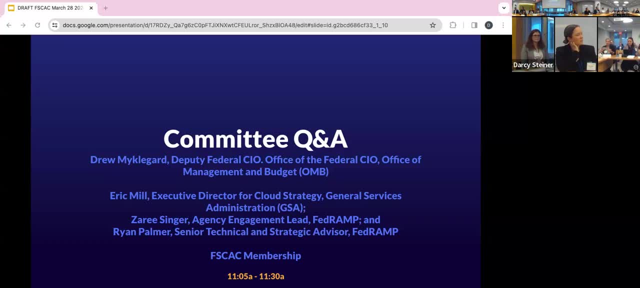 And then making sure I can inherit And if I can't directly do that, based on whatever GRC full, that I can at least get a package that can be loaded in. So I understand what the customer responsibility matrix is, what controls I have to take care of, those kind of things We've got to. 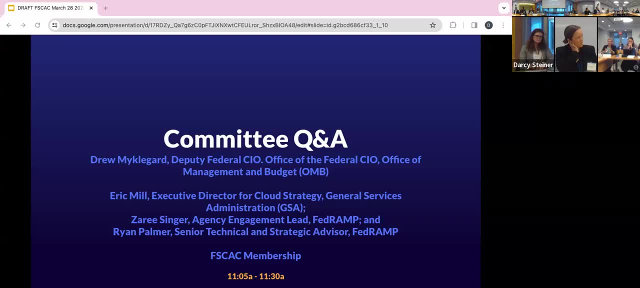 make sure that the end process to actually we've got to FedRAMP and then we've got to do the ATO at the end. So how do we, in my role, and so how do we get to that point where we recognize and part of 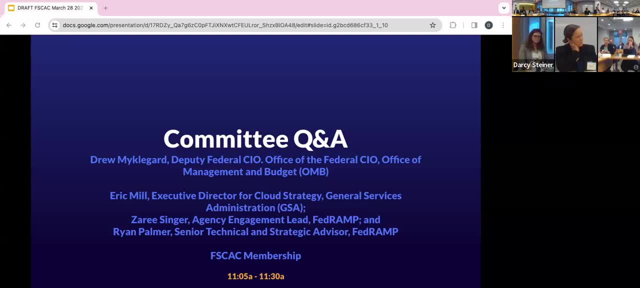 that is, how do we get to that point where we recognize, you know, and part of that is you know, our configuration, guidance that you talked about, which is really critical, But it's also being able to pull in all of those controls. And then my second comment is: as we look at our 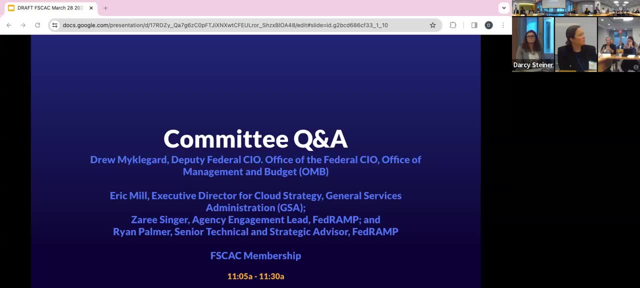 automation efforts. we really need to figure out in OSCAL- and it may be there- how we actually assess our technical controls on the system, put those into machine readable format and correlate those back to the 853 controls So that it informs compliance, so that we're not having to take a 3PAO's time for that 55, 60% that. 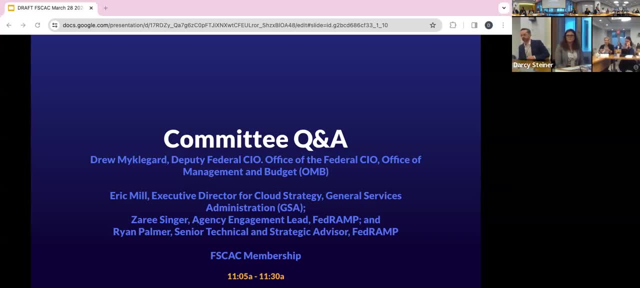 actually is automated through benchmarks. So how do I read my benchmark data? How do I incorporate that into my GRC? process it to inform the controls, so that I never have to look at a piece of paper. I don't have to do a manual assessment of the system. A lot of our cloud providers are. 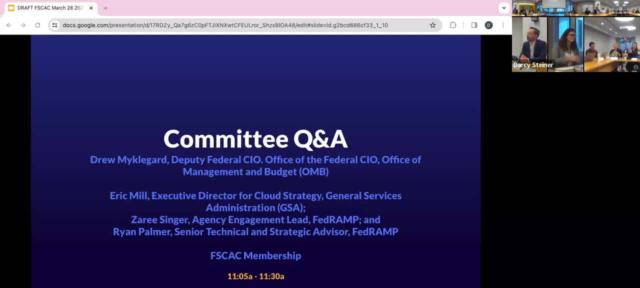 just so large, you can't do that at scale, And so how do we look at that for consistency across The cloud provider's infrastructure? So I offer that, And then, as we look at automation as well, I think we need to start looking at our SaaS providers and figuring out what a container 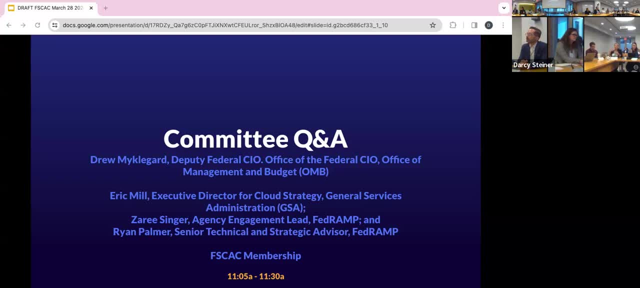 scan would look like what a code scan would look like. We've moved to that level again. we've moved from IaaS all the way to SaaS. So how do I assess the quality of the software? That's one of DoD's really big focuses right now is we're finding a lot of our vulnerabilities in. 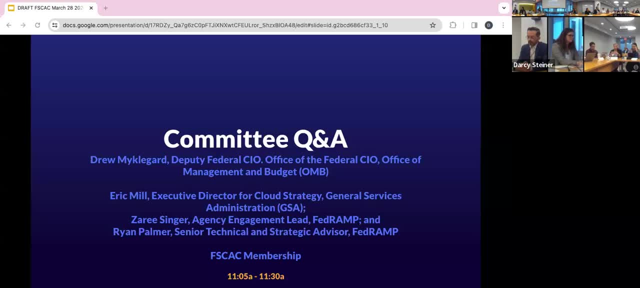 our exfil data is because of lack of solid data, And so I think we need to start looking at that. So how do I start to bring in my software efficacy testing as we move down the automation path, Just because you guys don't have enough work to do to do 25.. 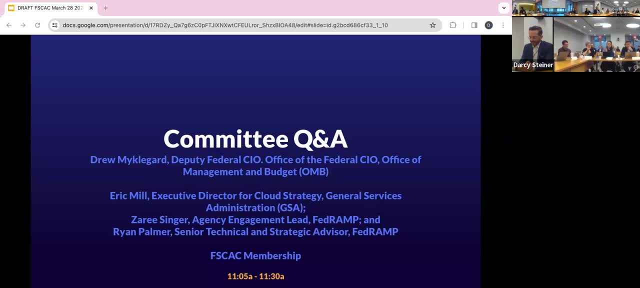 Just to echo a point that Jackie made, particularly around centralizing Kanban, I would argue a lot of agencies perhaps don't actively review the Kanban output corresponding to CSPs that they use And the current deliverables are CSP specific And, as we all know, 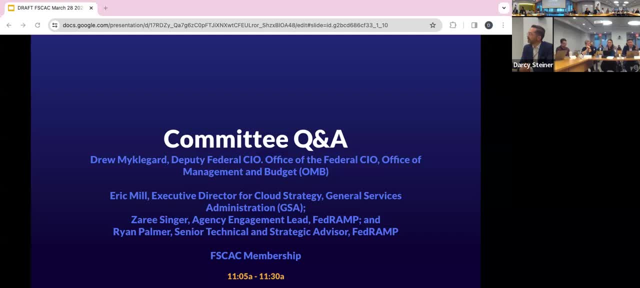 I mean from a cyber perspective. it's an aggregator right. We have a combination of CSP solutions that we use across each of our respective agencies, And one thing, if you're thinking about centralizing Kanban, would be to think about developing a central agency dashboard. 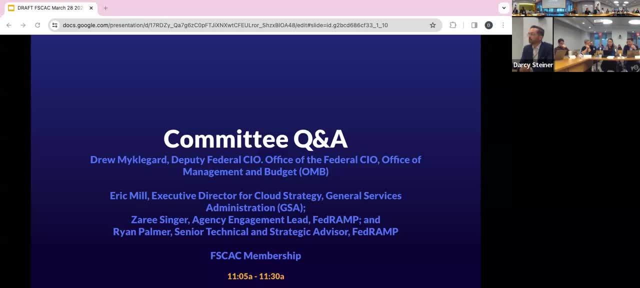 that provides an aggregated risk across the set of CSP solutions. So that's one of the things that we're looking at. And then the other thing is: if we're looking at a central agency dashboard, we're looking at a central agency dashboard that provides an aggregated risk across the set of 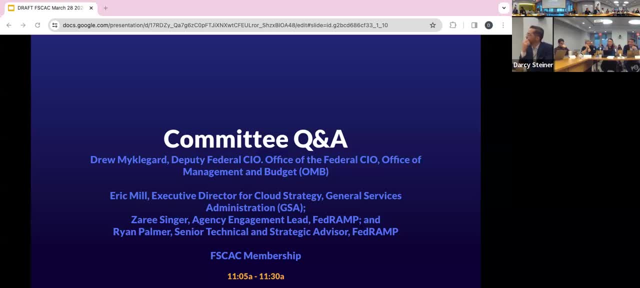 CSP solutions that are actively used. This would essentially help authorizing officials to understand their cloud security risk, their data risk, particularly relative to their cloud ecosystem that they use, versus having to go through and review individual CSP specific reports, which by itself is helpful, but it doesn't tell the full story right, Because 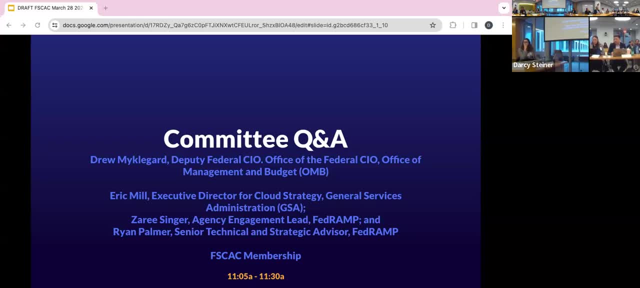 increasingly we're looking at supply chain related considerations and how all of these CSP solutions integrate with one another. I think tell a bigger story, And this could potentially go upwards, not just at an agency level but rather across government, in terms of what our overall national exposure might be individually to a SolarWinds type event. 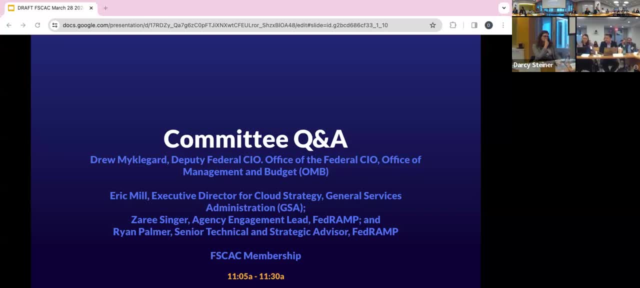 versus individually across the set of solutions that we're actually using, Something to think about. But as we're moving towards a database-driven type model, putting something like that together- I'm not saying it's easy, but it should be more readily achievable. Absolutely agree. Those are a very 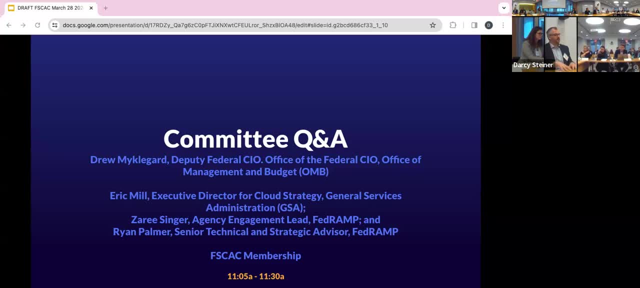 cognizant point. One of the things I don't think we talked about is we are planning on partnering with DHS to try to pipe certain data- not all the data, but enough data to power dash boards- through the CDM program. It doesn't mean we won't also have that sort of data or dashboards. 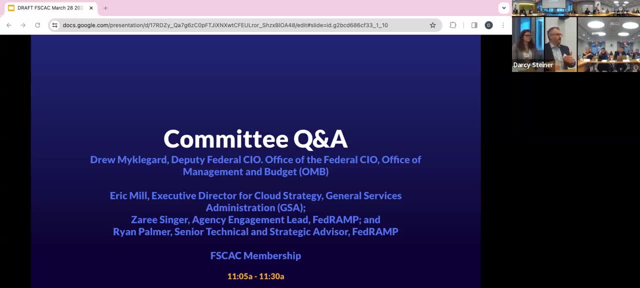 available in the tool, but we understand agencies may already have some tools. So we want to integrate with and leverage those experiences that agencies or authorizing officials may already be used to Through the GRC tool. it will allow us a lot of opportunities. We 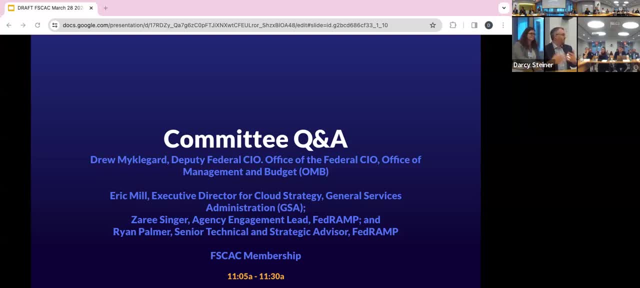 are looking for automation partners, All this stuff. we want to do pilots, We want to build partnerships so we can test these things early on and keep revising that. We need to integrate between systems and that's why we're working on OSPEL- And you didn't even see me up here. 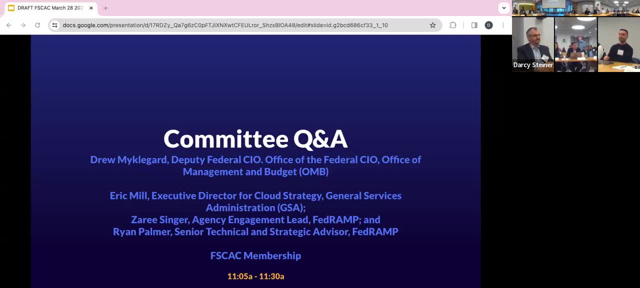 But I was going to offer this is my large CSPs. I have a lot of CSPs that are very interested in making veterans successful and being parts of these pilots. So anything we can do to offer pilots, resourcing public knowledge, please reach out to me and I'll get you connected. 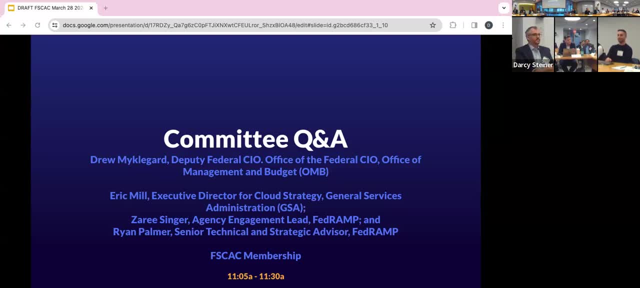 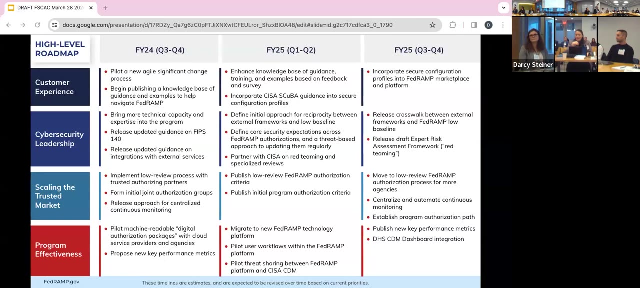 with all of the organizations that are lined up ready for this. Thank you so much, Marcy. go ahead. I was just looking at the timeline that was shared. So one thing as an assessment firm that we're- good or bad- really familiar with is integrations and relationships between various 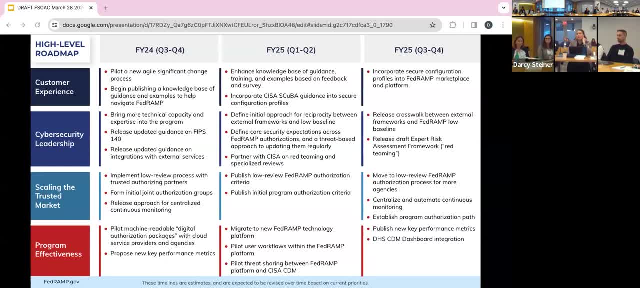 frameworks and how they map or don't map or relate to FedRAMP and the various baselines. Obviously, FedRAMP is very data-centric, It's system-centric, but data, parallel data, parallel, metadata- there are very few standards that follow the same. 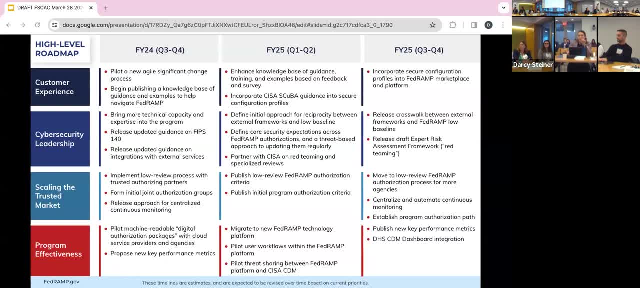 flow. So I guess my- when I see this- I saw it was focused on the FedRAMP flow baseline- Is that kind of the only target. Is there any anticipation that we would expect external frameworks to be mapped or get granted reciprocity with moderate or high? 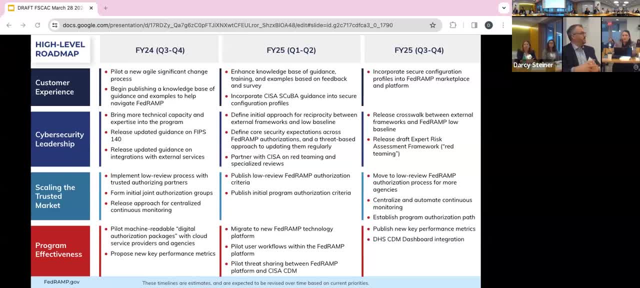 I think that's like an ongoing challenge. I think starting with low is a starting with low is an approachable thing. I think, as we, you know, get feedback from the community, which I think is really important, right Like this is a goal. We can start with low. 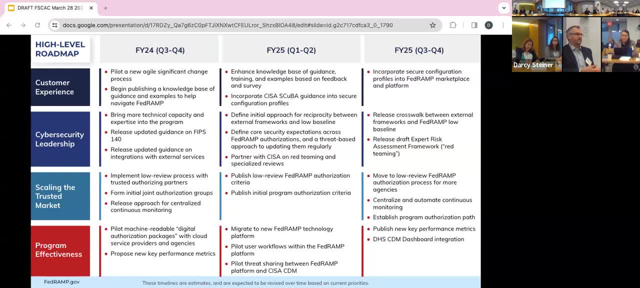 build that out, see how that's working and partner with like thought security alliance and these other framework people and say how can we kind of norm on something that does work? Reciprocity doesn't have to be 100%. We can cover 70 or 50% of those controls at least. That's still a cost reduction and a work in. 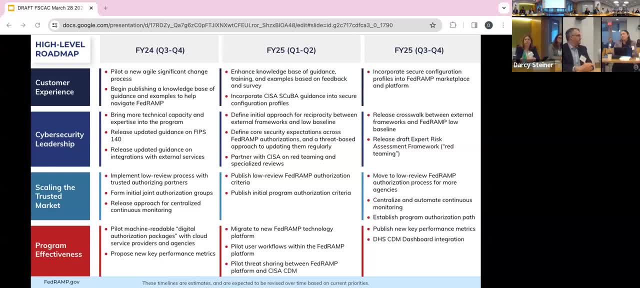 reduction in duplicative one. The simplest answer is that we want to be able to do something more than the low baseline. We see the same challenges that you're describing, and this is the best way to start by that. Do you have frameworks that you're targeting? 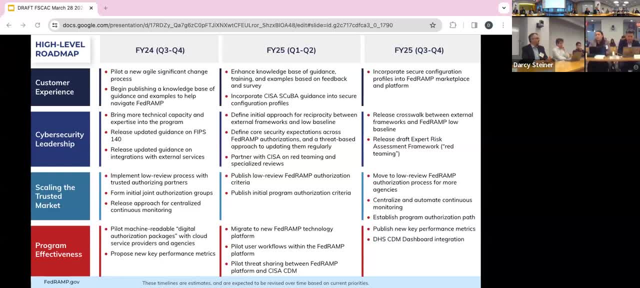 Right now I think we're looking at SOC 2 ISO like CSA. but we're certainly open and if we can map to it, especially with OSCAL and being able to look at these different data exchange, we should hopefully allow more flexibility to say like: hey, these across. 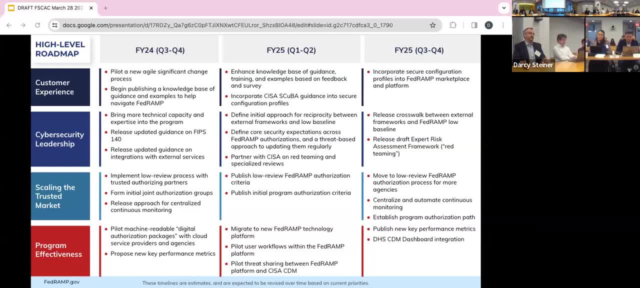 seven frameworks. these all map to the same control and we can do that through data. That'll also mean that if you have your own tool, that means you only have to write once, use many. That's already happening a lot of times with CSPs and probably 3PO's is my next suspicion. 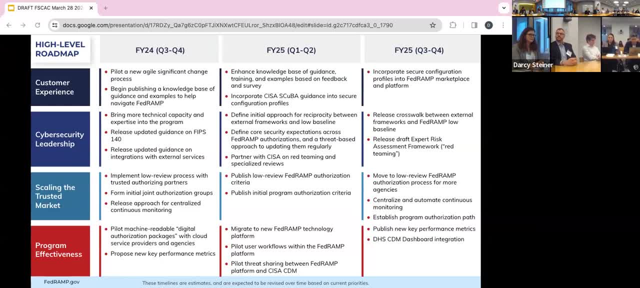 Great. We do have a question from Daniel Payne, who has had to join us virtually this week because he's in the middle of the loop. Daniel, go ahead. Thanks, I appreciate the clarification. Daniel Payne Databricks First off. 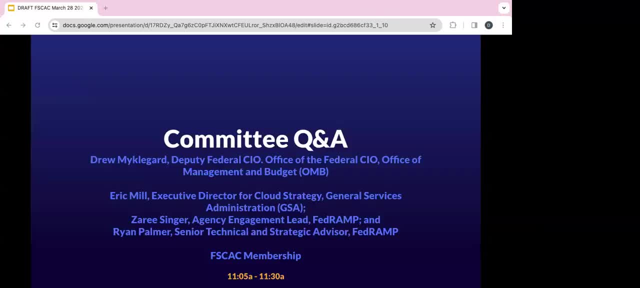 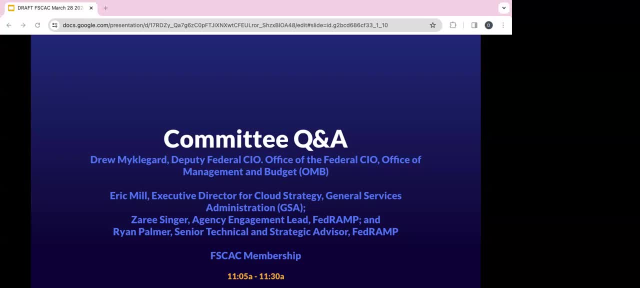 a lot of the conversations that we've had over the last kind of half year that I've been part of this have been around interpretations of controls, interpretations of requirements both from agencies, 3PO's and PMO, and sort of minimum standards, if you will. I'm curious if any of 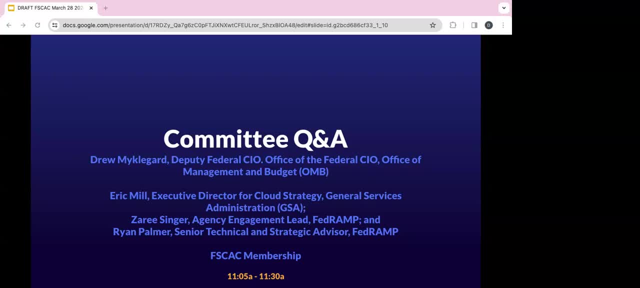 that kind of applies to things like minimum risk thresholds or mandatory implementations, ie FIPS 140-2, or just in general clarifying requirements across the board. FIPS 140-2, or just in general clarifying requirements across the board. 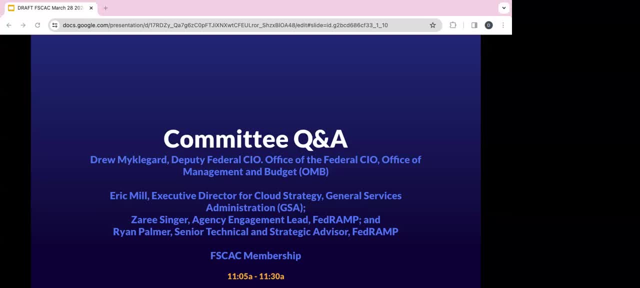 FIPS 140-2, or just in general, clarifying requirements across the board. When agencies are talking to CSPs, when CSPs are talking to the PMO, everybody's speaking the same language and we're all kind of on the same page. 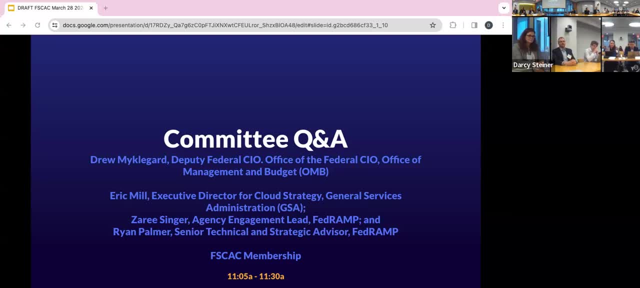 The knowledge: yes, that is a challenge and that's something we want to address. The knowledge base- one of the things around that why we want to provide technical examples in that is so we are clear in our communication to our different stakeholders. 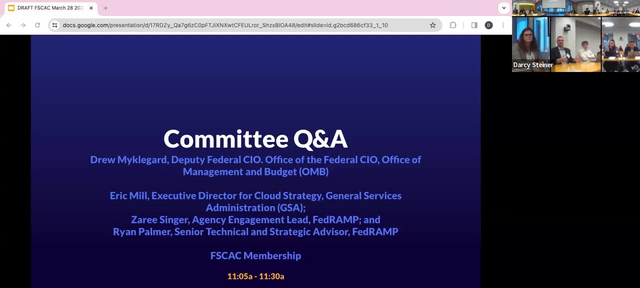 The other thing that knowledge base will allow is more visibility across those different roles. We understand that we're providing a response to the CSP and Info App. We're providing another response to a 3PO. These might be tangential questions or similar questions. 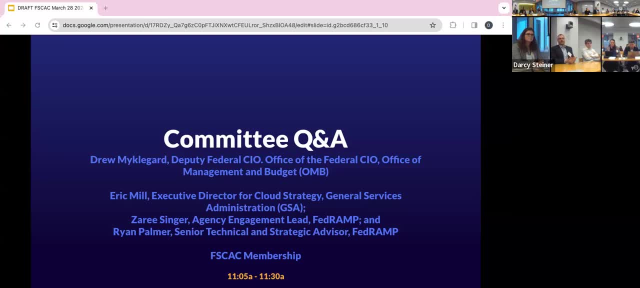 but we're not providing visibility to different stakeholder groups of the answers we're giving. We want to address that with the knowledge base. As far as navigating some of those challenges, we do need to do that, but we need to provide that guidance for all those different stakeholder. 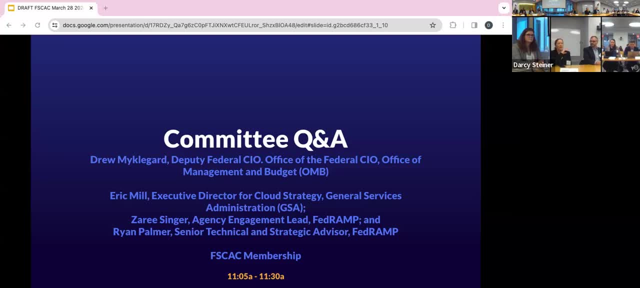 groups. Yeah, The entire agenda, Yeah, The entire objective is getting those kinds of things out of individual meetings and discussions and available to everybody. There's an implication there in the knowledge base, too. We talked about examples that I want to call out, which is that we want to put out real-world examples, examples of how. 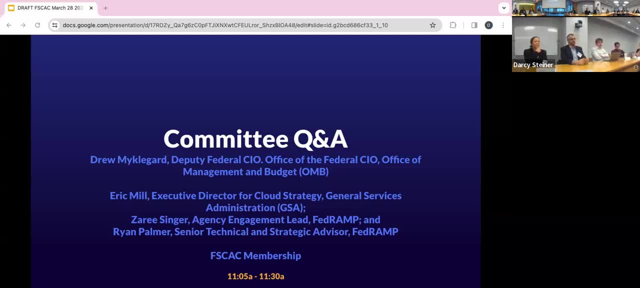 real companies have really made it through the FedRank process before. That means that it will likely be asking companies to be a little bit more comfortable sharing some version of what they may have done that could help other people. I think that's going to be important to the FedRank program and we'll be looking for a 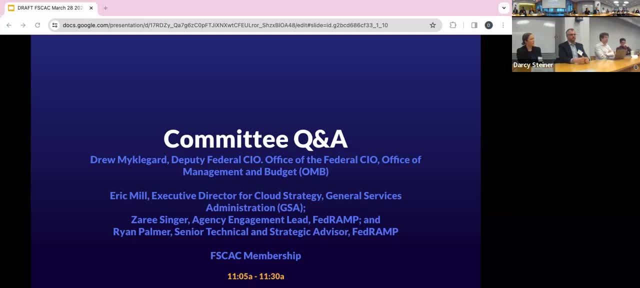 spirit of collaboration wherever possible. I have one more question. This is, Mike, The revision process itself. is that something you also are looking at in terms of how do we win this baseline or communication as things change, if we're going a little bit more agile now? 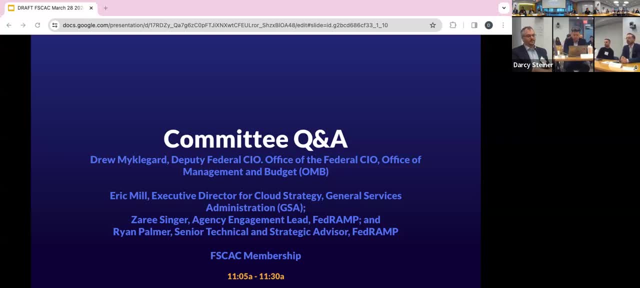 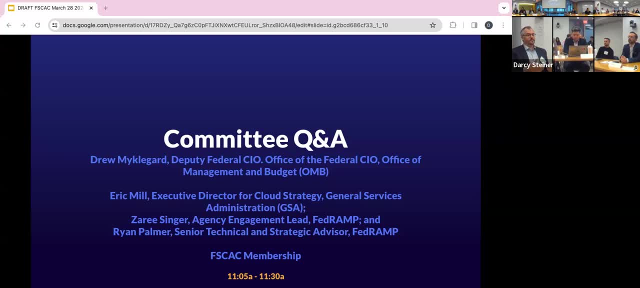 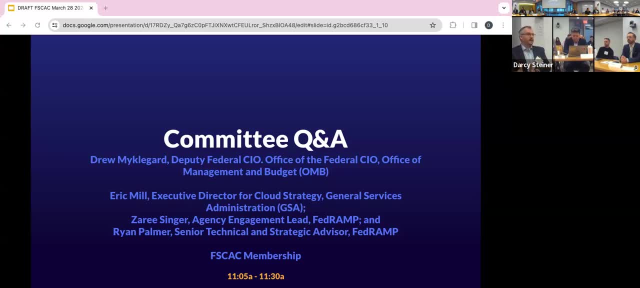 to these requirements today. they're going to be good for at least this amount of time. it is really important and we're practicing that challenge. We have talked about that a fair amount internally, and the idea, too, about the necessity of maybe having to distinguish what applies to our board, what applies going backwards. 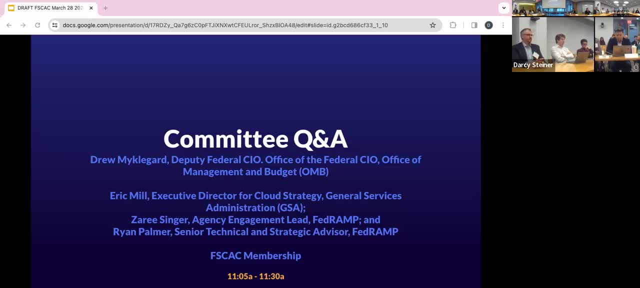 some periods of time, just from the change management perspective, But we don't want a concept of how daunting that is to stop us from making some progress on it. So yeah, we talked about that a lot. You should probably see that reflected at least a little, in what we published. 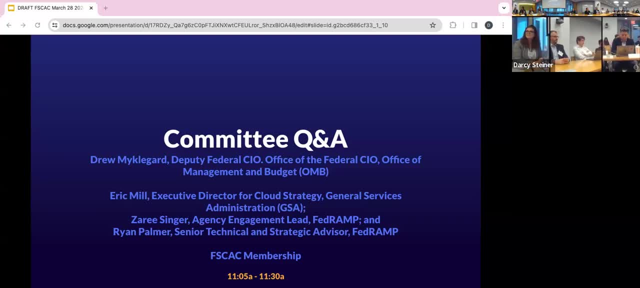 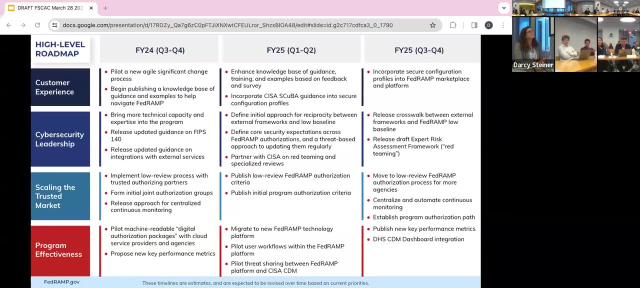 Any other questions? One more, If we could go back to the timeline. What is on the far right? release draft expert risk assessment framework, quote red teaming. What does that mean? So in the draft OMB memo there is some. 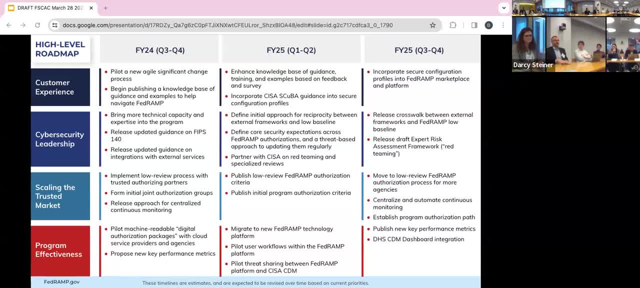 cases where we might want to look at expert risk assessment. I think there's a lot of different potential use cases. One thing I would be excited about is if we identify where there's an alternative implementation in place that couldn't be tested by a conventional assessment. 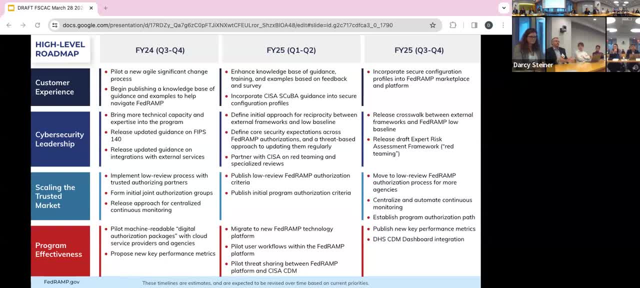 or team. we could look at ways where we could bring in a red team to validate that that technology is providing some sort of similar level of security and control. That's one potential use case. I think there could be other thresholds and criteria, One of the things we have talked about. 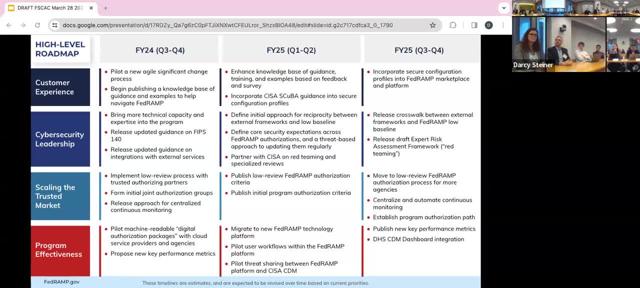 I think in earlier phases here, which is partnering with CISA, on when we would do those red teams and under what conditions. I think there's very, very positive opportunities there to use those red teams to validate what technology our new approach is to security. 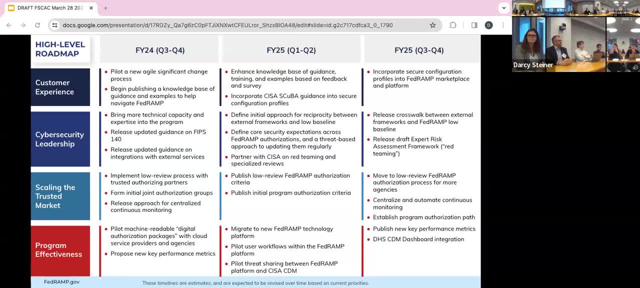 I can offer one piece of guidance. The terminology is triggering because of the new CAA2 requirements. I think there's an opportunity for a lot of confusion, So that could be potentially. Yeah, We've started to see some of that ourselves, honestly. 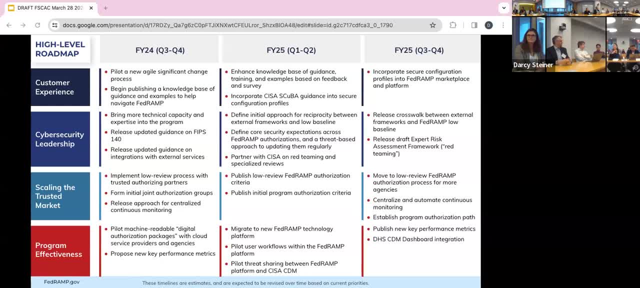 That makes sense. We've had to go out of our way to distinguish between those two things a lot, So definitely heard Cool. This is Mike from Total Again. The one thing I wanted to add, too, is a little bit of a challenge. I hear a lot of talking about 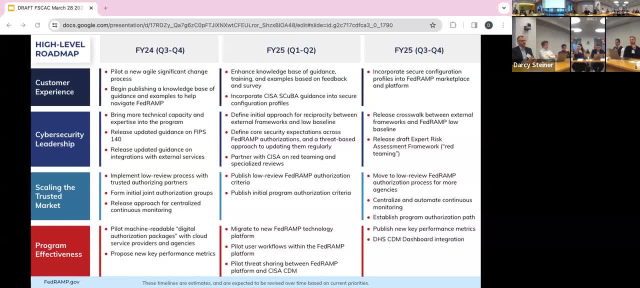 the cost benefit trade-off earlier. Low as a baseline has a very low return on investment. So a lot of companies really focus on moderate and high, especially as they get larger. Just keep that in mind. We should definitely be challenging you to push into moderate and high. 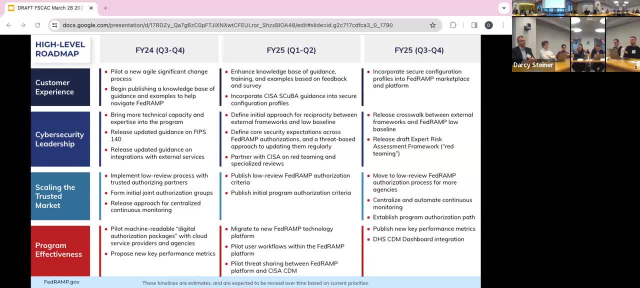 as fast as possible with some of these updates, because the return on investment makes more sense. Jackie, Just to tag onto that comment, we talked about the iterative type of ATO or agency evaluation. I would encourage to start at moderate, because that ends your CUI data. And if I had to guess, 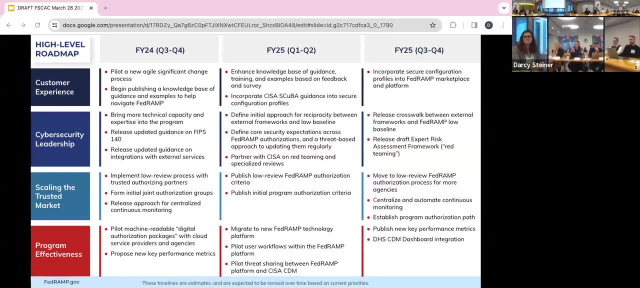 the majority of yours are going to be dealing with CUI data, And so starting at low really reduces the applicability of its use for systems that need a capability that are operating the CUI data Right. I would probably look at as someone described it is a moderate baseline with a set of the 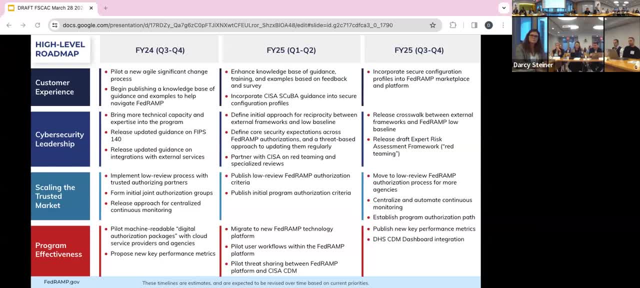 technical controls that are most critical to authorization. So in our system world we start with auditing and authentication as our critical cornerstones, And then that's the barrier to entry. you know that they have to meet privacy standards- auditing, authentication. 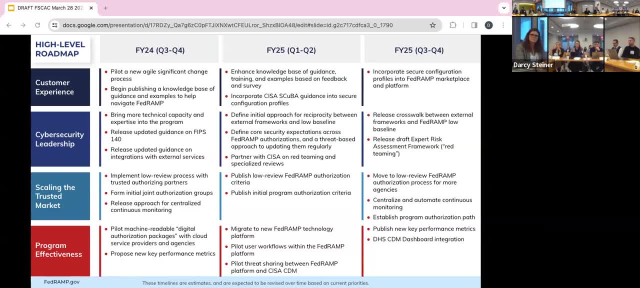 and choosing some of those boundary protection and those types of controls, And so we call it our subset of controls, just to get in the door right. But at least we know that we can process the type of data that's available to us, And so I would just caution you on the low-moderate issue. 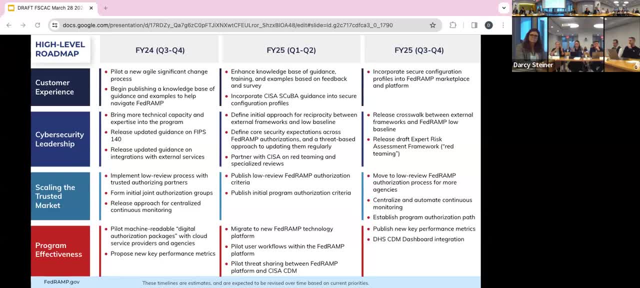 is to start with, moderate. but look at your control set and not focus as much on the impact level but on the controls around the level. Correct me if I'm wrong, but I think the reciprocity piece is the only place where we're. 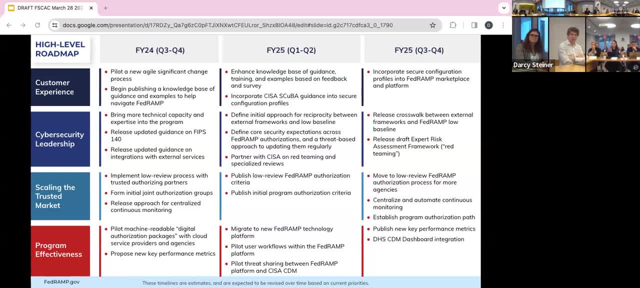 saying we're starting with low. Okay, More generally, I think a lot of the stuff is most applicable to moderate. Yeah, from a CSP perspective, I don't even think we've talked about low in years. Yeah, Real impact levels. Yeah, you have a lot of low things that are. 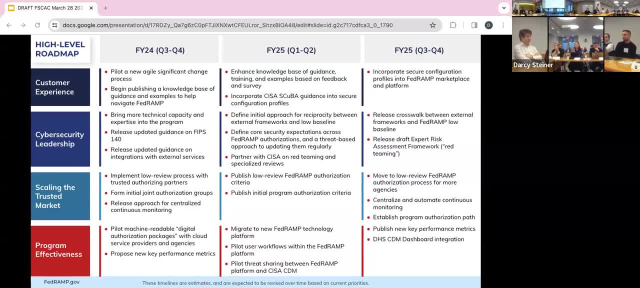 put in front, especially on the Taylor and Weiss side. but absolutely, yes, what you're saying is right. And, Josh, if you'd like, could you come up to the table. I'm sorry, just so that you. I just want to third the point about low working at an agency that has mostly small 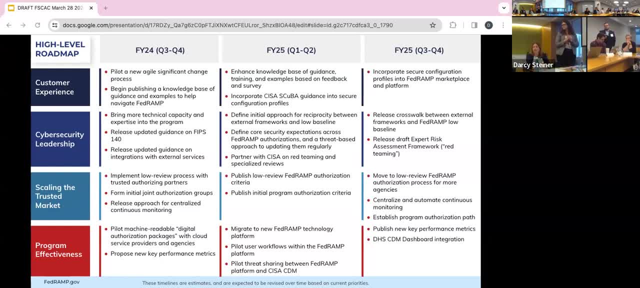 homes, Small homes, specifically Santa's products, pretty health-based. Low is just a critical sub-level. It's just how important it is to the community. Any other questions that we have? Does the committee have any questions for Drew? We can. 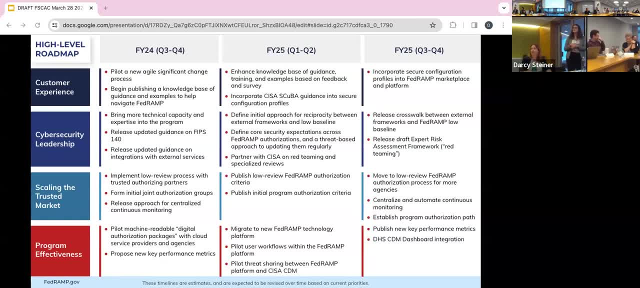 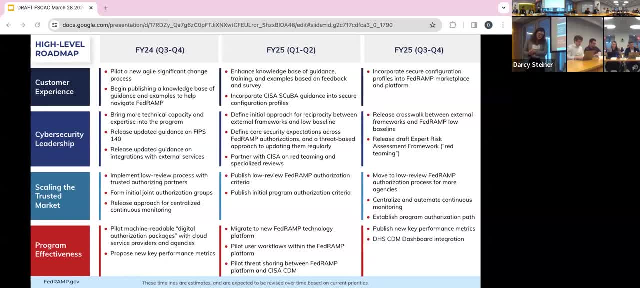 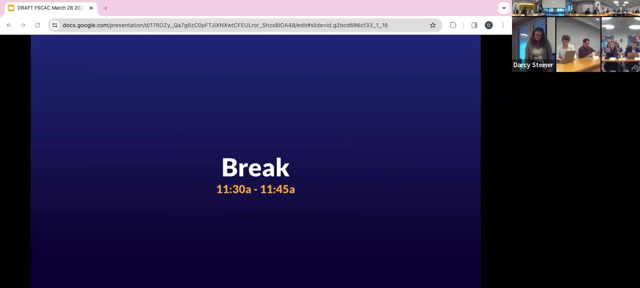 Thank you. Thank you, Good question. Thank you, Come on, Michelle, All right. Well, it sounds like everybody's ready for their break, So we'll go ahead and take a break, Please be. Thank you so much, Thank you. 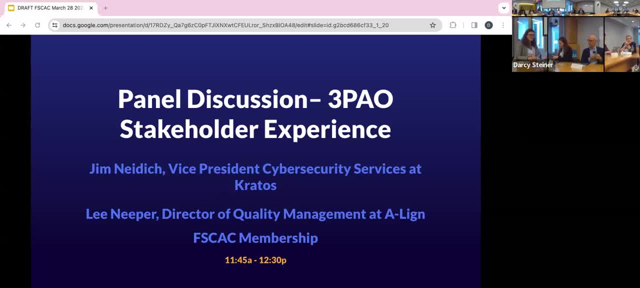 They will both be sharing their experience as VPAs in the FedRAMP process. This panel is designed to be less formal and more conversational. We've asked Jim and Lee to respond to several guiding questions about their experience working with FedRAMP. 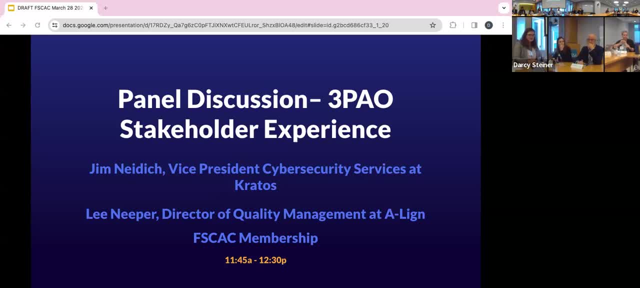 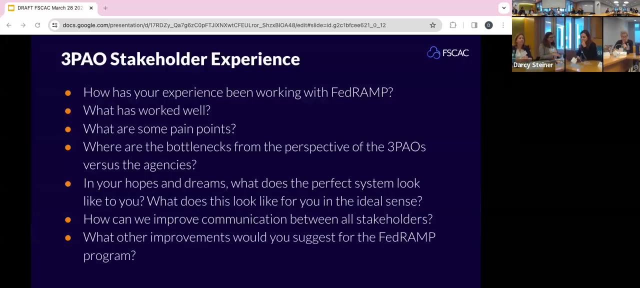 Committee members are invited to ask additional questions they may have for Jim or Lee during the conversation. Does anyone have any questions about the process? Okay, great With that. Jim and Luke, thank you for joining us today. Go ahead and share your experiences. 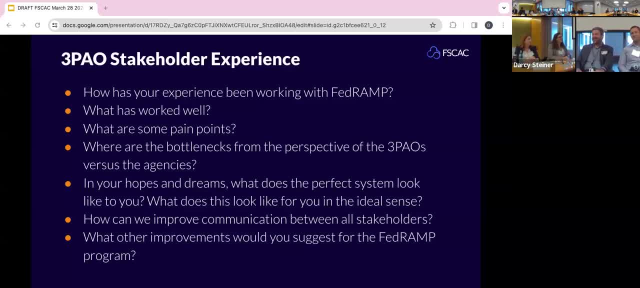 I feel like a lot of thunder has already been taken. I've seen a lot of my ideas up there. I think it's good progress. I think this is Jim Knight from Creator. I've been around the compliance game for my entire career. I started back in 2004 implementing FISMA programs at government agencies and did a decade of that and then came right into FENRIP because, you know, got to ride the wave. It's going cloud first and all that stuff came out. 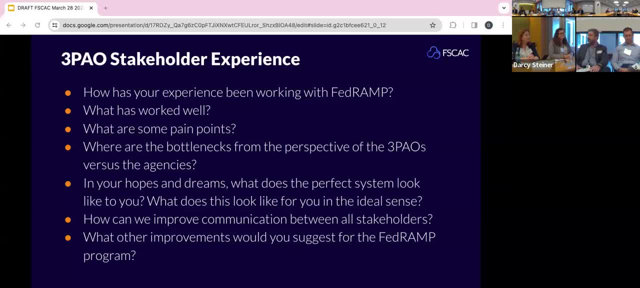 But I think we should be proud of what we've built here And I know when we have our challenges and things that are going on. we talk about the reciprocity thing and we talk about, you know, leveraging other frameworks. Well, you know what other frameworks want to leverage us. 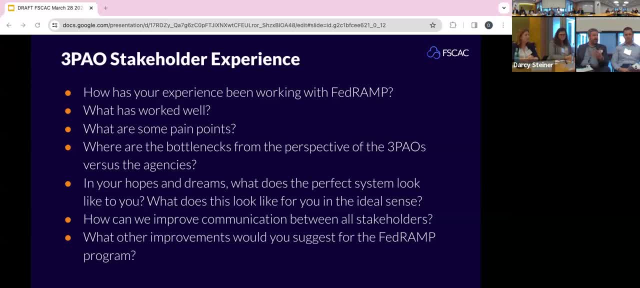 Because you know out in the economy. it's FENRIP first. It's like we have put in place the most rigorous, trusted framework to date that I've seen And it brings reliability and it's made some large improvements over what FISMA was. 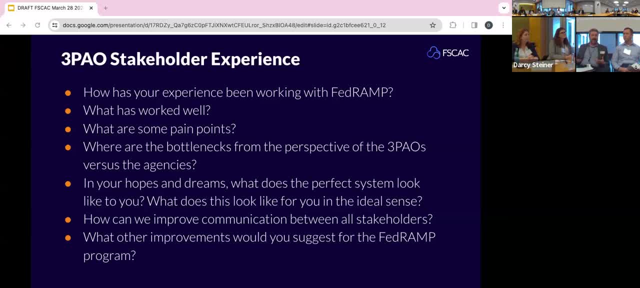 Just think of we were trying to apply FISMA in the cloud environment today. It's that use once, do once, use many times principle. That's important And that saves a lot of costs that are coming into this And you know it was interesting what I heard about the small business, whereas you know 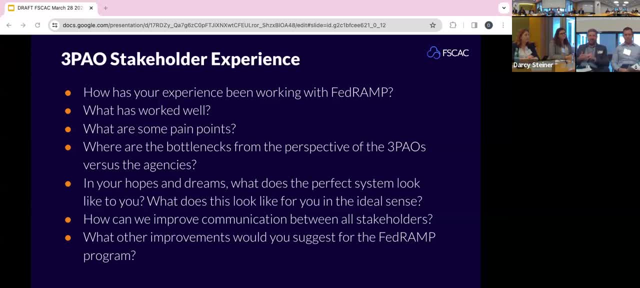 leveraging the IaaS and the PaaS to come through, And we have to be a little bit careful there because those small businesses may become capabilities or services on those platforms and IaaS too, So they can lose their identity at the same time. So that's a challenge that we're going to face when we kind of approach that. 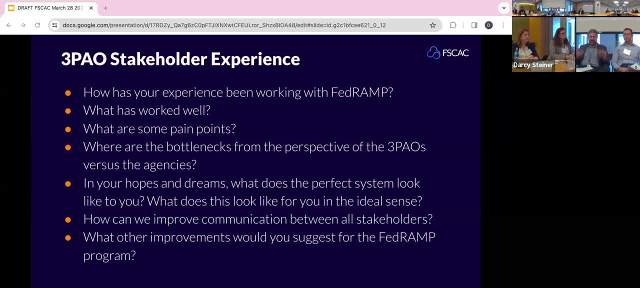 In terms of, you know, the most positive things that come out of this is, you know, just the foundation that we've built, the rigor we've put in, and then the consistency and reliability that we've harnessed from the 3PO perspective. 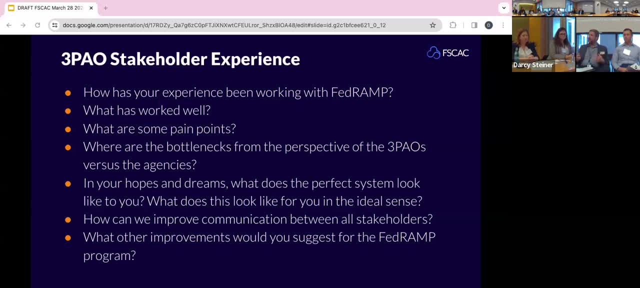 There's not a Q in the 3PO's. The 3PO's have been able to come on board. I know that there's. you know, Lee and I are sort of in the top five of 3PO's that have done- I don't know- 80% of the assessments out here. 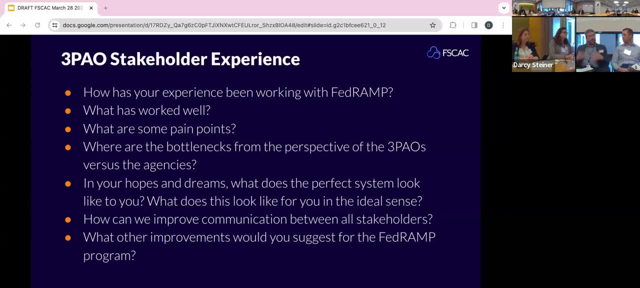 I think it's 88% The number, But you know, with that said, there's areas to improve and the challenges that we spoke about today. you know. I agree and I'm looking forward to working directly with the PMO, the CSP community, to help make the right decisions forward so that we can improve this process. 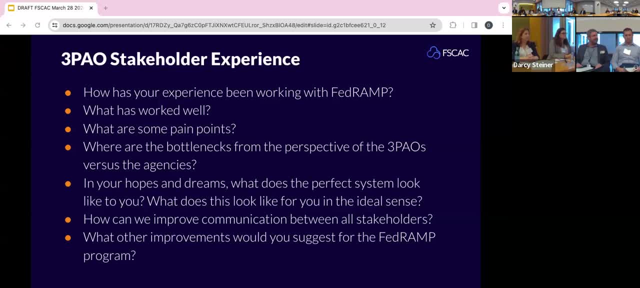 It's not going to be easy. Nothing is. Security is not absolute. It never is going to be absolute. It's almost good enough, right? We almost have to Look at it from a good enough perspective, because that's ultimately what we're going to face. 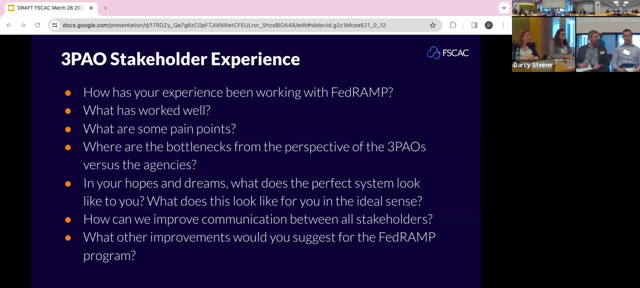 And so we need to set the litmus and work together to do that. But that's just my opening thoughts to leave. Yeah, it's growing pains is how I like to put it the best. When I came to align, we had only done one assessment, and now I think we're over 60.. 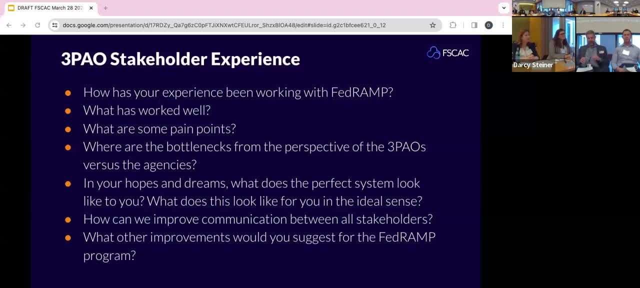 So I've had a part in every one of those assessments. basically that we've done And we do. we don't do the AWS is, we don't do the Microsoft's. We don't do a whole lot of that. So We have more one off smaller customers and clients and CSPs. 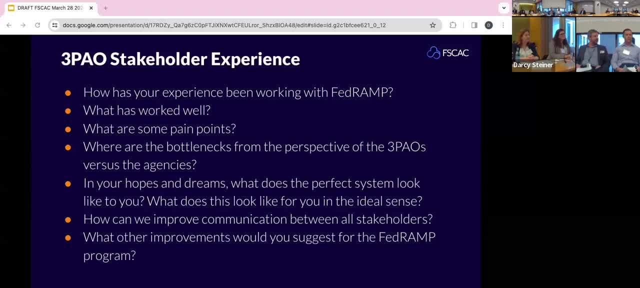 And those are the ones that we primarily work with And I think you know I've seen those groups struggle more than maybe some of the bigger companies like the AWS. So FedRAMP is adapted to that and we've had to adapt to that. 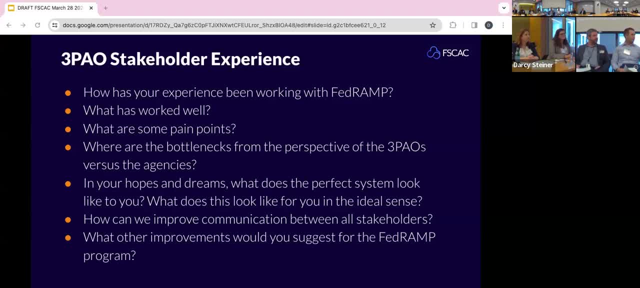 We don't have access to. you know a lot of those packages, like other three PAOs do, So it makes it more difficult for us as well. I You know, unless my customer gives it to me, I don't see the CRM, the CIS for Microsoft and Google and some of these AWS is they're difficult. 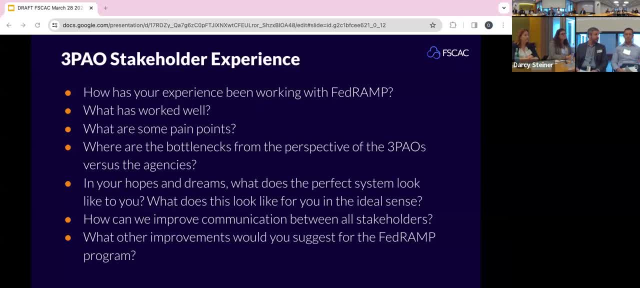 So they're difficult for me to get And then that makes my job more difficult. So FedRAMP has helped. you know that process. They've seen those struggles and they've adapted And I think there's still some minor growing pains that that everyone's going through on the CSP side, the three PAO side and FedRAMP side as well. 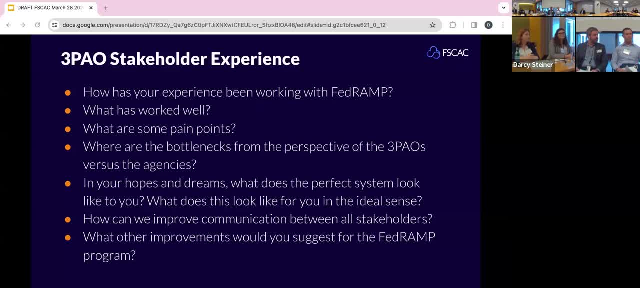 But everyone at FedRAMP has been more than willing, especially Recently with the REV5 stuff, to incorporate the three PAOs. we've set up groups ourselves to talk about how we can offer help and what we can do, And I've spoken to the CSPs as well and engaged their interests and how we can help them and what their struggles are. 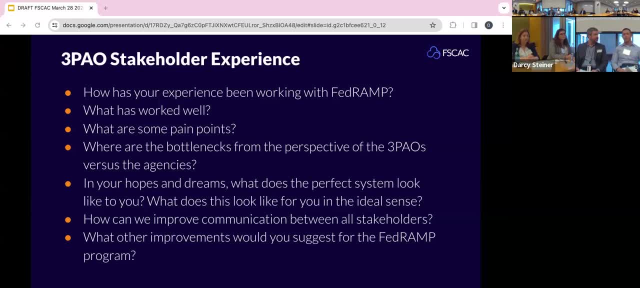 So I think we've brought all that stuff to the table and it's helped the process and helped FedRAMP overall. Any questions for us Based off of this? I mean, I can keep going if you'd like. I know that we had a couple of questions. you know what's what's your experience been working with FedRAMP? 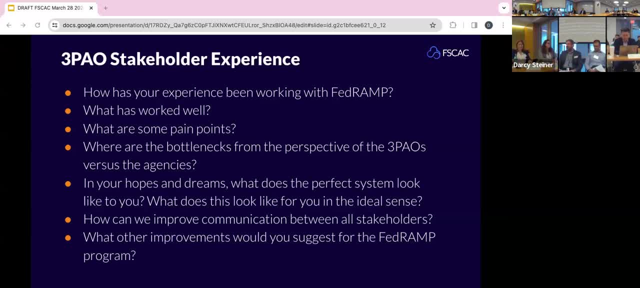 And you know, something I heard earlier- I'm glad I listened to it- was the metrics piece. I think the one metric that came to mind is: when is the timing right? Because, you know, think about it from a three PAO perspective. we can either serve as a consultant or an assessor. 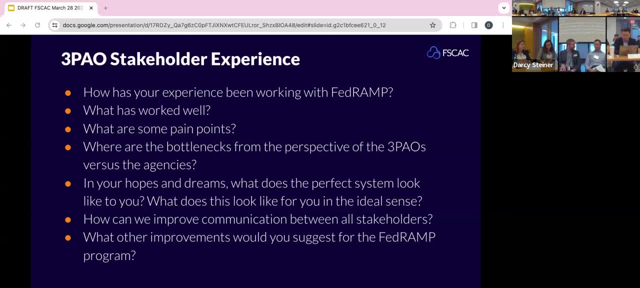 I don't know if your company performs both roles. Yeah, I'd say that we do more assessments than advisory, And I would say that we do too, but the consulting part is an area that we need to focus on too here. 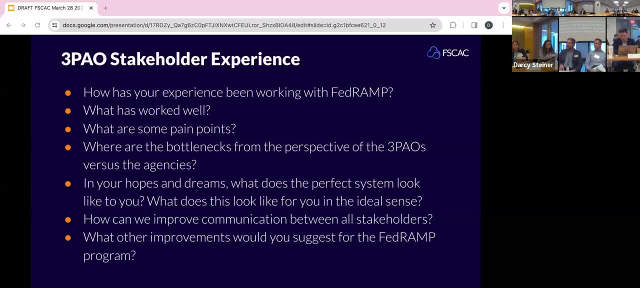 I know we're focused on the three PAO assessments. One of the biggest challenges from a three PAO serving in a consulting capacity is the expectation that they're going to bring us in and we're going to make it all up, write the SSP and give it back to them. 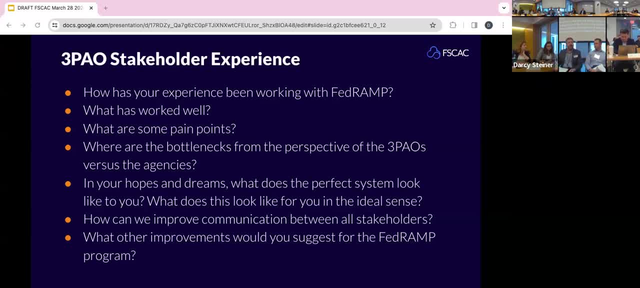 And that's not a reality. The reality is we need to become part of their team, And I think that's something that we need to be able to leverage, that we need to be able to build the team, to be able to put the detail into that documentation. 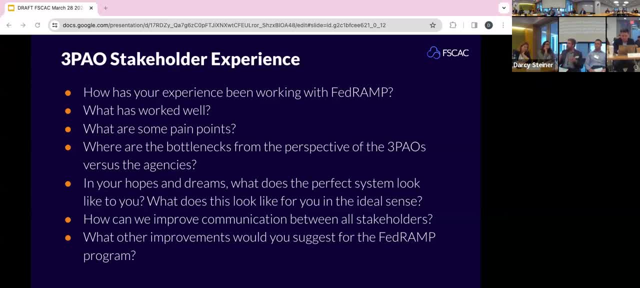 And we're not spending enough time sort of thinking about that, I think from the larger FedRAMP community. What are these consultants doing and how is that working? Well, it's not working very good because I would say my success rate on the consulting side is much worse than my success rate on the assessment side. 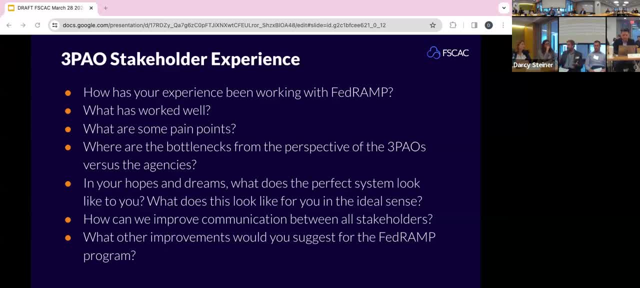 Customers get frustrated with us because we can't wave the magic wand and make those deliverables appear, And they realize that it's much more an investment- investment than they thought, than just from the consulting bringing the consultants in to make this happen. No, now I need my engineers, all these people, And that's where the costs go up. 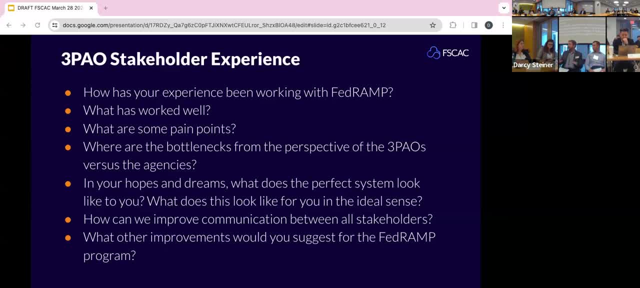 And they get frustrated like, oh, we're not even ready for you guys, We need to go back to our team. And meanwhile they've expended half of the contract value for the consulting engagement and they're frustrated and everybody's frustrated. So I think we need to kind of look at the 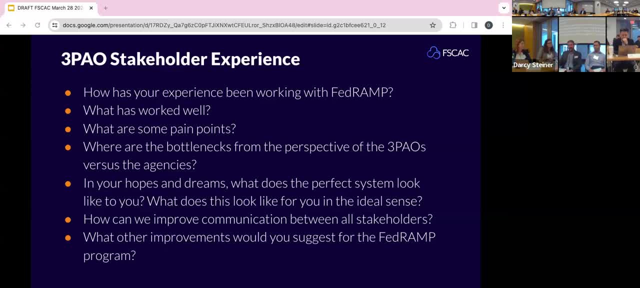 consulting side and see how we can make improvements there, because that leads into success on the assessment side. Many times we get into an assessment where a 3PAO hasn't performed the consulting and we go: oh guys, no, this is a non-starter, Like you have to go back to go. 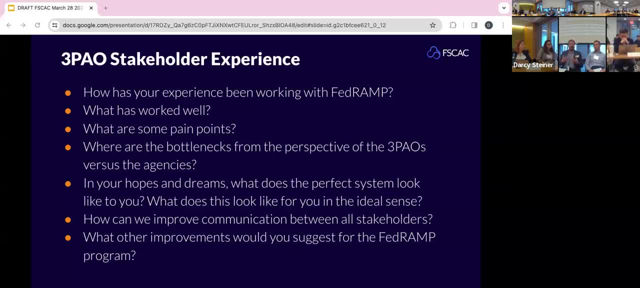 because you didn't get the right consultation or you got the wrong sort of consultation to move this path forward, And what I'm tying this back to is the FedRAMP cue. You know, we don't know what that is right. I think you're number something 50th or 20th in line, or I. 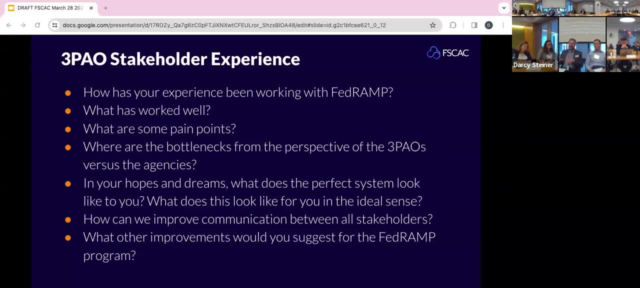 I don't know how they communicate that, but I think that's a metric that's important to understand to help unclog. that is, to allow that to inform the roadmap on the CSP side on when they're ready, because many times I get calls. 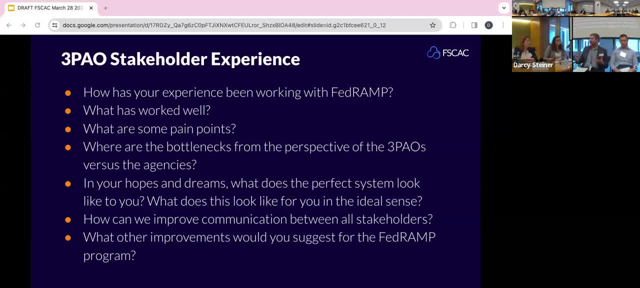 hey, can we start tomorrow? It's like we can, but we need to start with a plan. We're not gonna start the assessment tomorrow. We need to come in and learn and understand what's going on, And so that kind of feeds into my first question. 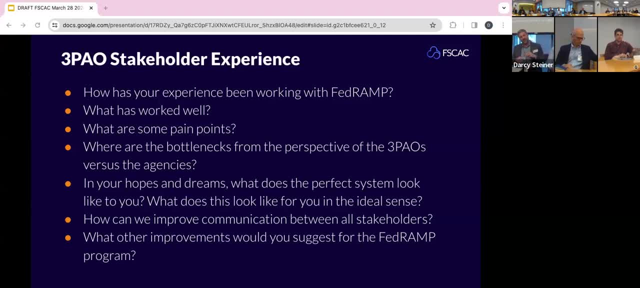 So you had mentioned that there's often a gap between assessment without consultation and assessment after a consultation has happened. Is that because of the lack of clarity or understanding of what the control expectations and deliverables are? What is not being communicated clearly and correctly to the CSPs when they seem to require a consultation? 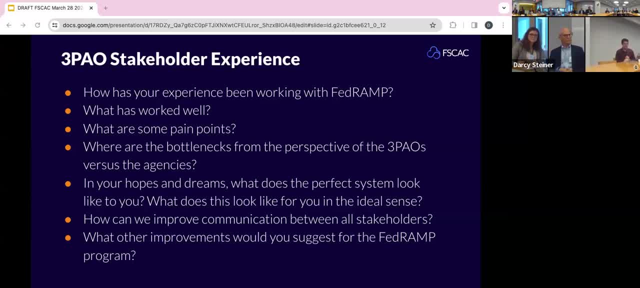 rather than to have them do this themselves and then be able to move to assessment. I think the templates is the first part, but it becomes a challenge as we now- and I think it's improved with Rev5.. SSP template, I think, is much more easy. 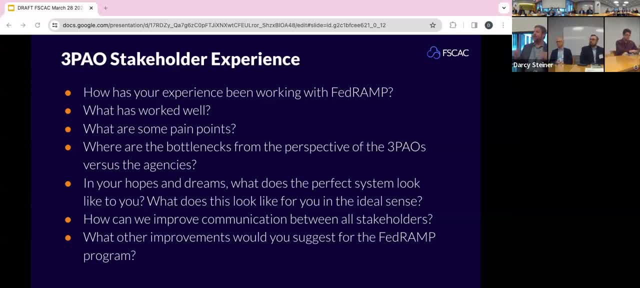 to roll our existing- from a CSP perspective, our existing- policies and processes into, because there's documentation out there but it wasn't focused on the federal framework when they built it and now they're backing into it And so it's translated. 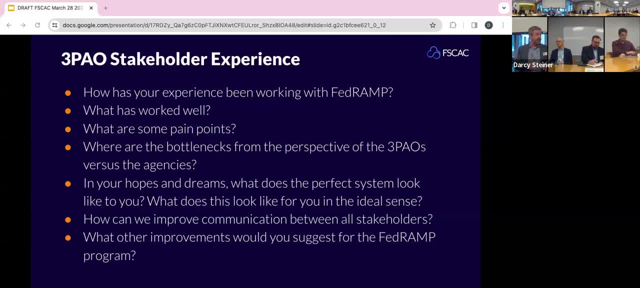 It's translating existing policies and procedures into the federal formats, And that's a lot of time to answer those questions correctly. the implementation statements: writing those up without actually doing a pre-audit- And that's why my most extensive consultations is we're there for the full ride. 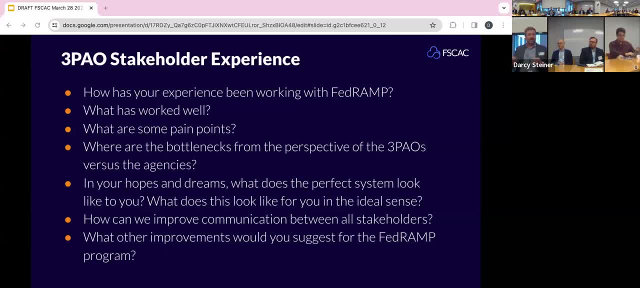 and we're actually prepping them for the audit, because we've now taken them full circle with the expectations of what the auditors are gonna have, And it's not just coming in, they're coming in, they're coming in line and say, oh, 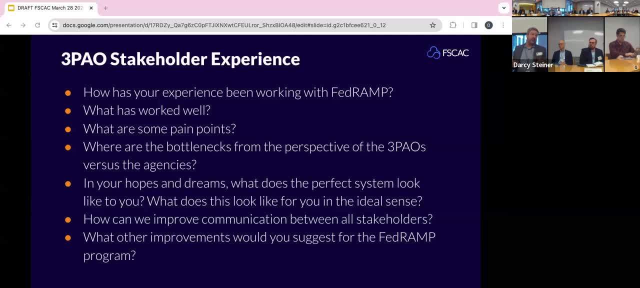 And so a lot of times we sit on a side call with them to ensure success to the assessment. But if that sort of investment from the CSP isn't made up front, they're gonna get their struggles where it's okay. now there's these showstoppers. 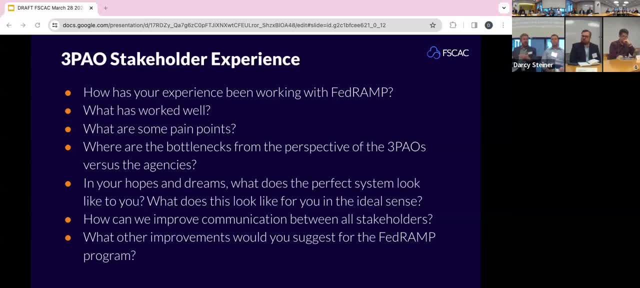 these deemed showstoppers that now we're clogging the FedRAMP pipeline itself because we progressed. we advanced too far without making sure that the road was paved correctly. There's also the issue with depending on who the advisor was. they may be one of these companies. 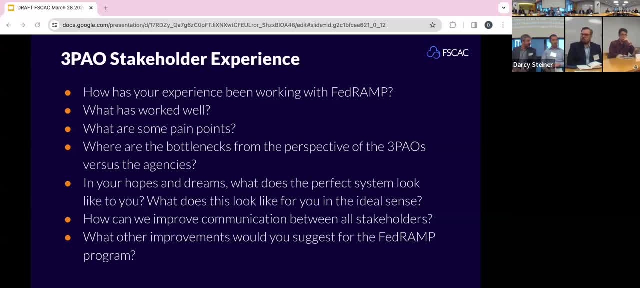 that they can either be a 3PAO or maybe they're not a 3PAO And they primarily do advisory work. The problem with that is they don't get as much feedback and as much direction as we. as somebody who does primarily all assessments, 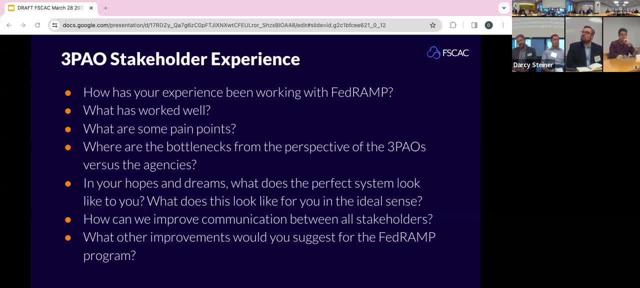 So we know that FedRAMP has issues with SC20 and SC21, and you have to have DNS set, But an advisory firm that primarily only does that. it takes them so long to do that, to do their advisory work, that they don't get 10 to 15 assessments a year. 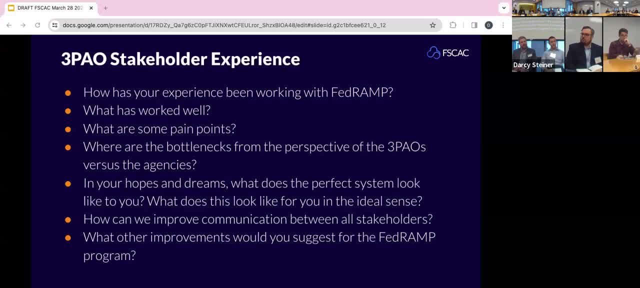 So they don't have this feedback And by the time they do get the feedback, we've changed the process or that's no longer a heavy hitter item. So there's a barrier there with who's doing the advisory and what is the quality of their work. 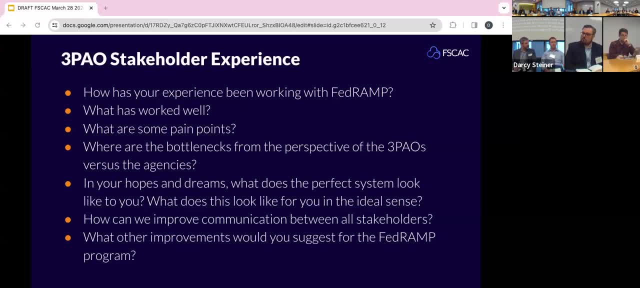 So this is where I think we play into the knowledge sharing that everyone's talked about with. we need some type of a portal. we need some type, whether we use USDA Connect, whether we have a link on the website to somehow share this guidance and share the direction out. 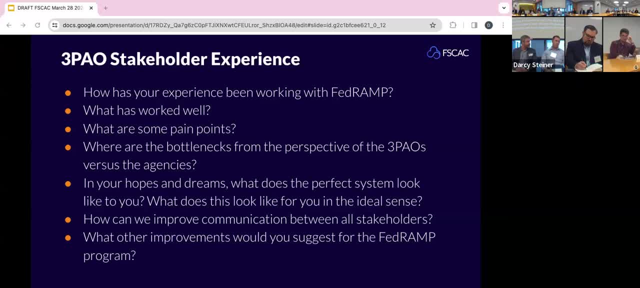 to everyone that needs it And that's where I don't know how to solve that problem. So the CSPs may need some type of guidance where the 3PAO needs another type of guidance, And do we share the two? Do we just make it a form for everyone? 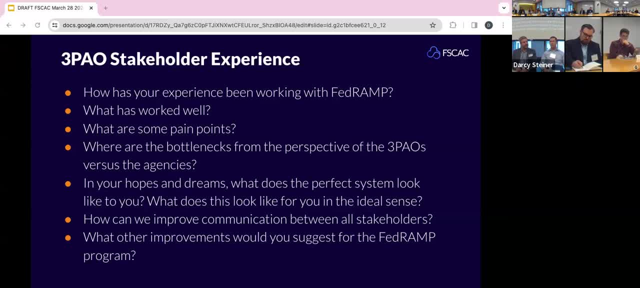 And I did see that on some of the slides earlier- that this is something that other people have thought about, and I think it's huge to share this guidance because it's gonna benefit everyone. It's not just: hey, this is gonna help a 3PAO. 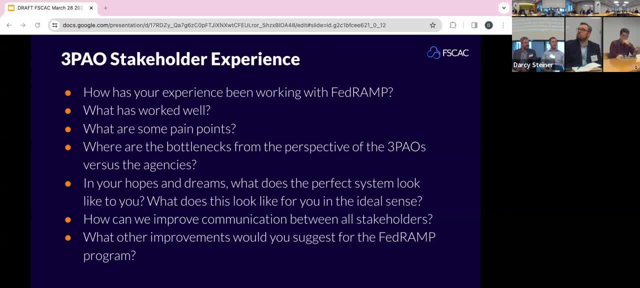 this is gonna help a CSP. We gotta get the guidance out there and it needs to be clear, concise and consistent, as federal employees to say for everybody, And that's gonna grow the program and put everybody in the right place. Yeah, Leah agrees with me. 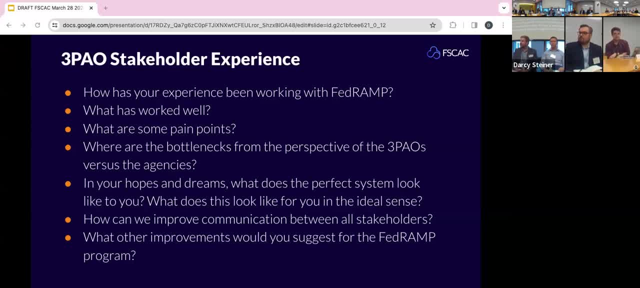 I think that the federal PMO has been more tactical with the 3PAOs than strategic. I think we need to take a step back and be more strategic And then we get back into the tactical pieces. But I think what you're saying is sort of like: 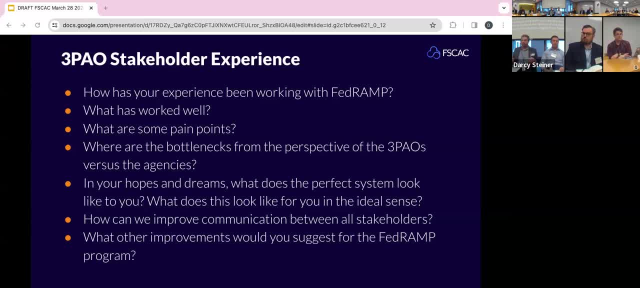 a knowledge base- maybe a 3PAO knowledge base- that 3PAOs have access to And we can decide. it doesn't make sense for the CSPs to also have access to this, But so when there's tactical discussions happen, we have a community where we can share. 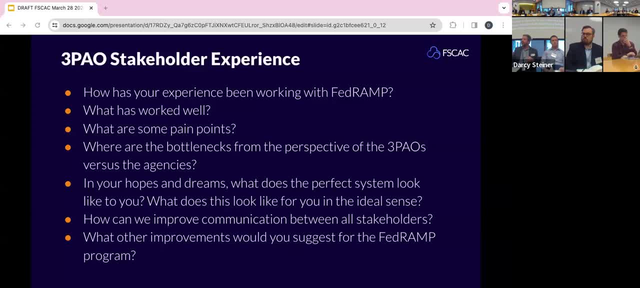 and collect feedback from the entire group of 3PAOs, not just the ones that are working with FedRAMP right now, And so that's where it gets really difficult, And the other thing that I think that would be helpful to me would be to have a challenge. 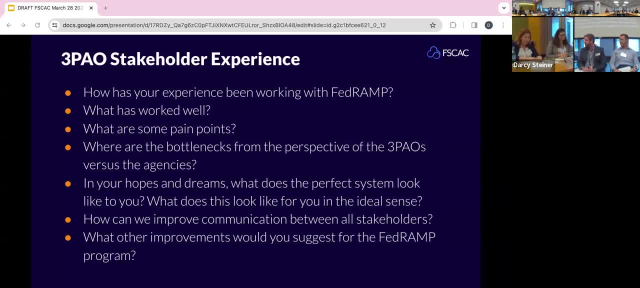 for the CSP to be able to say: look, we're not doing this on our own, We're gonna work together to make sure that there's no issue. But I think that there are a lot of challenges that we have to face with the CSP. 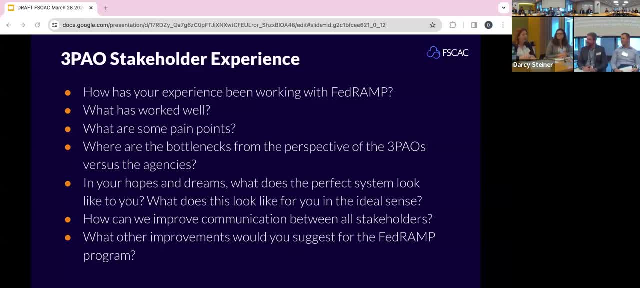 And so I think that that's a really important part of that, And I think we need to work together to get this done in a way that makes sense. I think that's a really important thing to work with the CSP, And then I'm gonna hand it over to you. 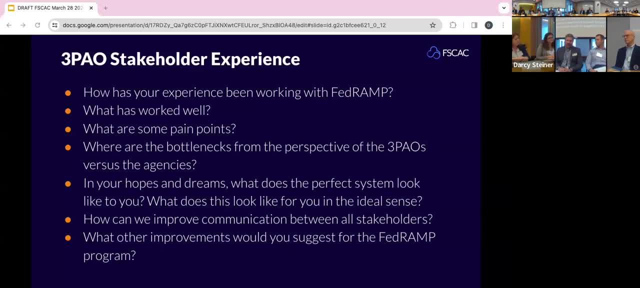 and we'll see you on the next panel. Thanks, Thanks, Leah. Thanks, Leah. Thanks for being here. I had a couple of questions. itself, and specifically the diagramming, has become a very big emphasis point with the FedRAMC reviews, especially through the RAR process, that I think we need to take a. 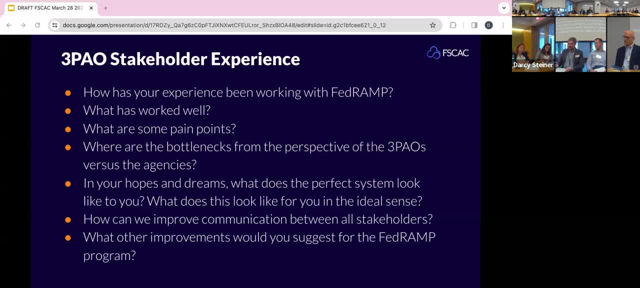 look back at. Yes, the diagram is important, but again, I was having a conversation on the break where at some point you bridge the gap. there's a gap or there's a collision between intellectual capital and transparency with cloud providers. That's always been something difficult for us to overcome. 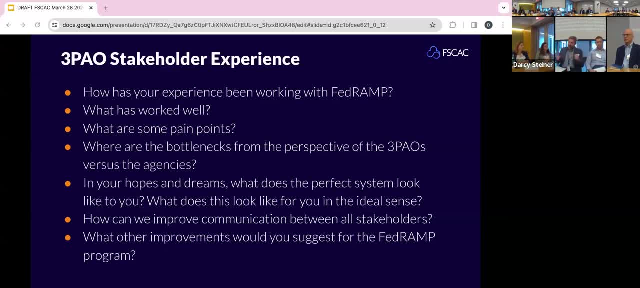 Even as three PAOs they're like: okay, we'll open it up a little bit to three PAOs, but don't you know NDAs? That's the nature of leveraging commercial cloud providers. It's not. this isn't a shared community. there's competition. there's an inherent sense that. 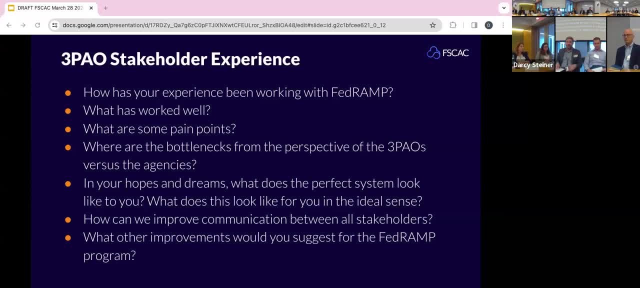 we need to protect our intellectual property here and not divulge too much as to give somebody a competitive advantage And you know, kind of cycling back To you know the point. I think we spend a lot of time mulling over diagrams and it. 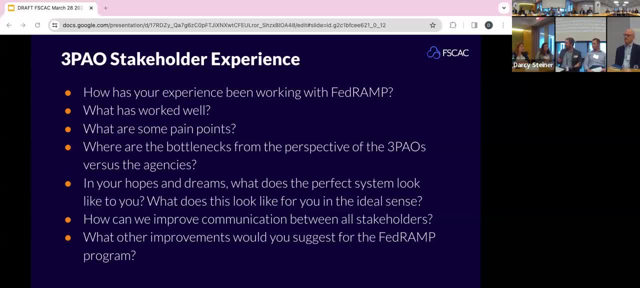 detracts us, maybe, from the operational processes that support them, which I feel are most important. You know, when it comes down to what's a perfect system, it's not. it's not no zero vulnerabilities, It's leadership, leadership, commitment. 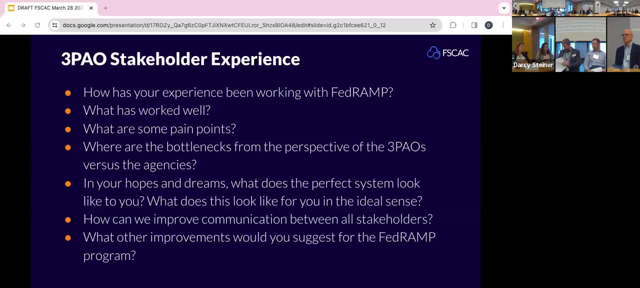 It's, you know, and I let me look at my notes here because I got- I got a couple other good points. Open communication is one, but then there's the challenge between how much communication does it take? And do we bridge without, you know, bringing our lawyers upset at us? 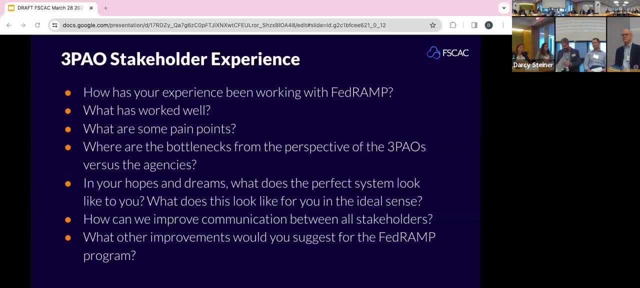 The draft boundary diagram, guidance that I mean, which I think it's still in draft form. but I mean that's something there that everyone can benefit from. if we release that document, get it, get it up to the current status of where it needs to be. 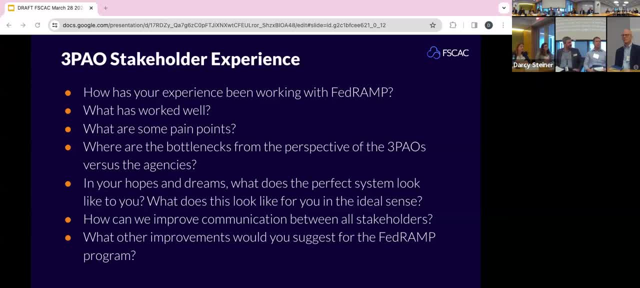 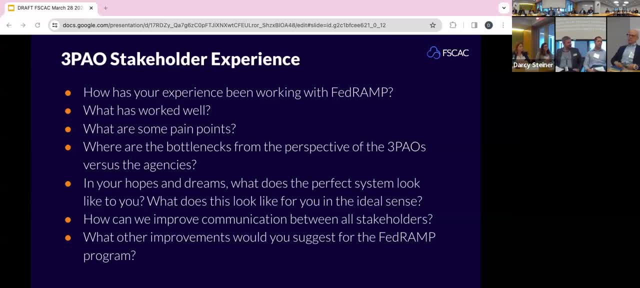 know the tools, they'll do a good job. It's not that they don't want to do a good job, It's they just don't have the direction. And if they don't work with an advisor- and sometimes when they do work with an advisor- 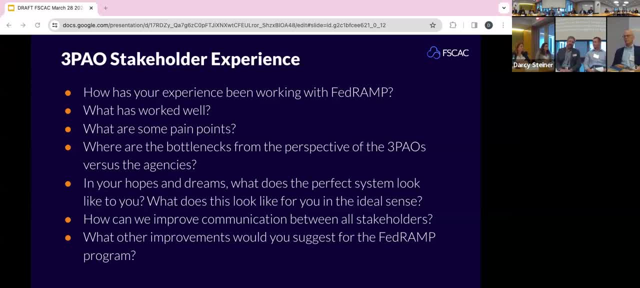 they get mixed information. Yeah, I think I think the large CSPs, obviously the large ISS platforms- have have more difficulty with the, with diagramming their their environment, than the small CSP. That makes sense Sometimes it's it's pretty easy to diagram if it's a relatively simple SAS, SAS solution. 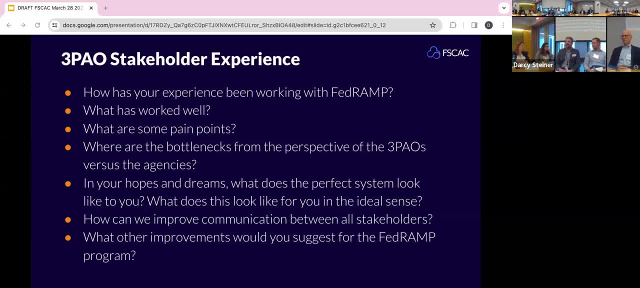 But once you start getting into the- you know, hyperscale cloud, It's like, oh my gosh, like this is going to take us a hundred pages to show you And that's that's really you know, comes back to you know one area too, that I think. 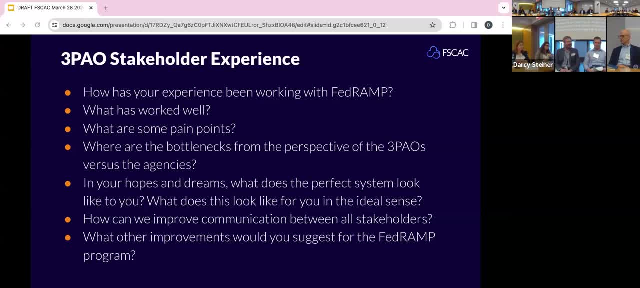 we need to collaborate a little bit better on is the authorization phase sort of. the way the authorization phase works now- And I'll speak from a from an agency sponsored perspective- is the three PAOs working with the agency and the CSP. you know the agency sort of sit there, they, they, they look at. 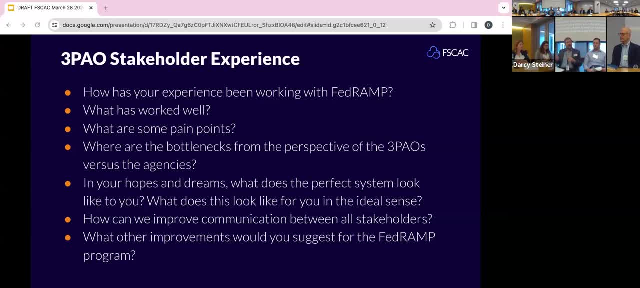 the SAP and And they get to see the SAR first And really that agency sign in an ATO is their ticket to enter the, the FedRAMP process review, which which can be dangerous at times because the risk tolerance between FedRAMP and the 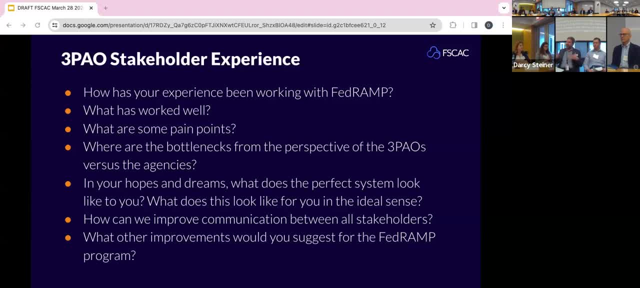 CSP may differ And that can become contentious, embarrassing, you know, punitive, you know, as, as the third party coming to review the package. And sometimes it's six months after those days, Yeah, Decisions, or maybe longer than than they've been made. 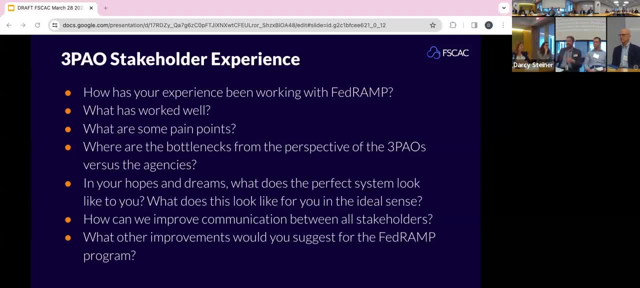 And so now it's like now we have to remember, recall why we did this. And you know there was six months of Kanban and usually, you know, sponsorship will will say Hey, yeah, And I know we're not allowed to put conditional ATOs, but the sponsors can put conditional. 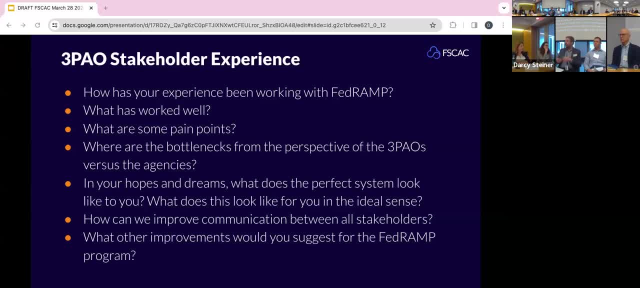 ATOs. We- okay, we're going to authorize this. We want to see three months of Kanban. It's sort of like a test period to make sure that it's usually due to high filings that they didn't, you know, risk reduce or whatever. 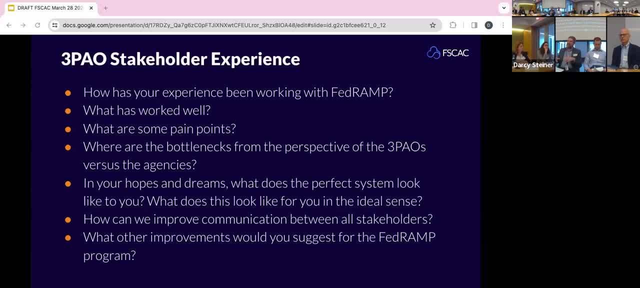 But what really is Important is is maybe we need to get the PMO and the sponsorship decision more closely aligned, or an alternative to that is: is is sort of like the RAR does maybe specify the, you know, the big rocks or the, the showstopper areas, to make sure that those are checked. 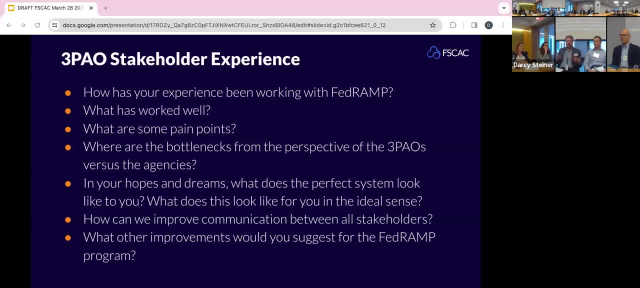 off. And then, yes, risk tolerance can vary between what the PMO wants to establish and then what the agency is going to accept, But I keep seeing A pattern of of inconsistency there that I think we need to address because, because of the timing of it, you know, six months later it's very difficult to like okay. 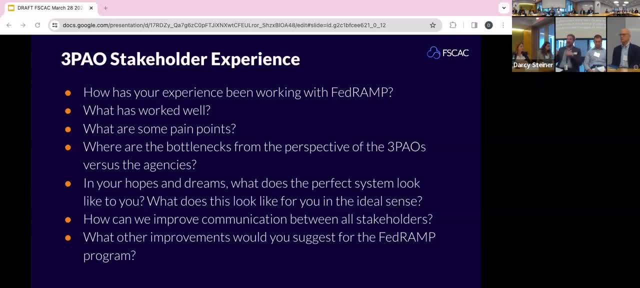 well, yeah, we've had these discussions with the sponsor and they they were comfortable with it. Now we're having those same conversations again. Sometimes we don't have the same people that actually worked on the assessment, And so it becomes a very difficult conversation to have, especially when you're asked what. 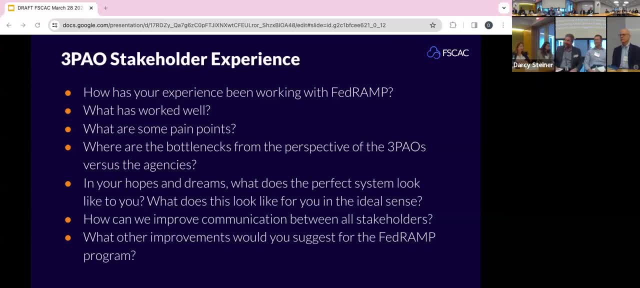 is it, Are you sure? Are you sure? I'm like, that was six months ago, I'm pretty damn sure. I was sure Back then, But now, now you're asking me, I'm not sure anymore. Any other questions? 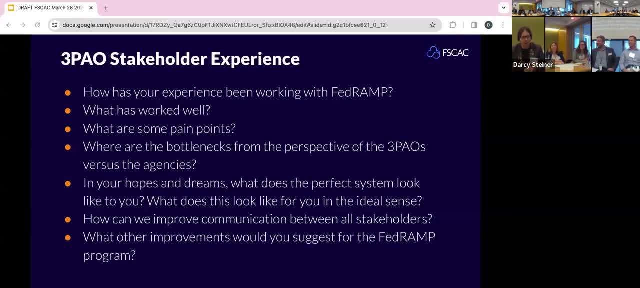 Oh, I'm sorry, Bill. Go ahead Close enough, Bill. I wanted to drill in a little bit more on where Ann was going and some of the conversations I think a bunch of us have brought up specifically around really focusing in on those small. 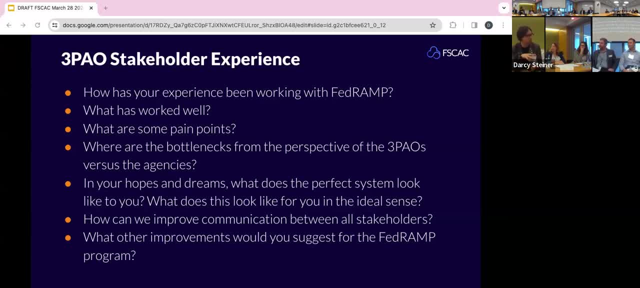 businesses. It sounds like between both of y'all's companies it's over a hundred assessments at least. I'm not going to put numbers in your mouth, But I'm just making up numbers. So focusing on those small businesses, not the hyperscale. 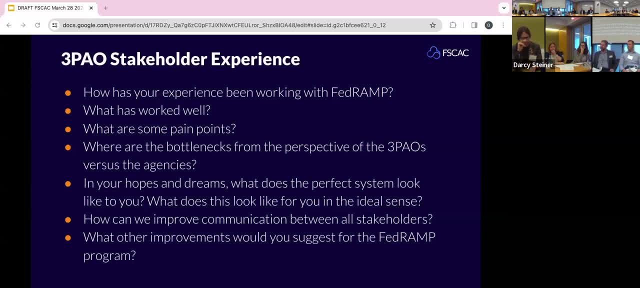 And Leah, you were hitting at this a little bit, you know, mentioning the SC family, Are there specific areas of these small businesses aside from the diagramming? are there specific families or things that we really should be focusing our automation or documentation, or 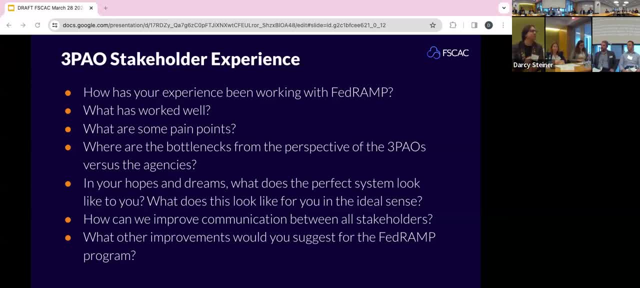 educational efforts around and specific families or areas that every time you see one of these come through, you know they're just going to, you know they're going to screw it up or that they're. you know there's going to be a. 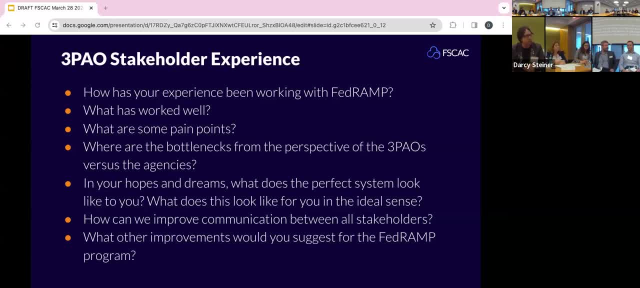 There's going to be a problem with it, because you see it over and over again, day in, day out: SC, a hundred percent. I mean the FIPS validation piece is literally killing every CSP there is. It's just, it's a. it's a giant black box that no one truly understands. 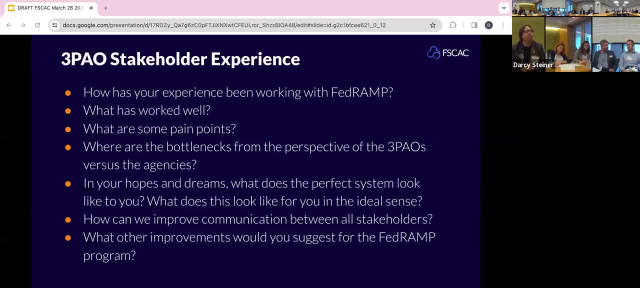 And then when you start saying that their endpoints have to be FIPS validated, well, their minds blown. where does this stop? How far does it go? And there was some direction given on, you know FIPS and there's a lot of historical. 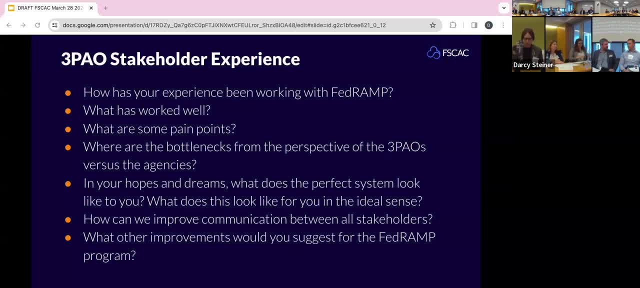 modules right now. Well, that that's some more direction that we don't really have. Is there any direction? What's okay And what's not okay? This one's in historical, but they're making progress towards updating it, So can we proceed with that? 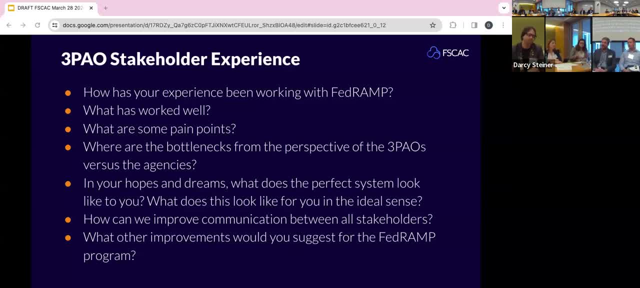 You need to see us. These are asking us and we're like: well, I got to ask FedRAMP. You may get some some mixed responses, But for the most part it's pretty consistent. but that's a document there that I think. 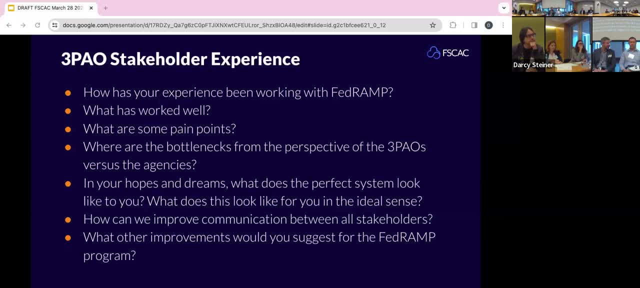 you know, the FedRAMP team could release and the agencies could even all get together on and say, Hey, FedRAMP, this is how we all want to address this. We're going to release that guidance And then CSPs know, going in, they don't waste a bunch of money. 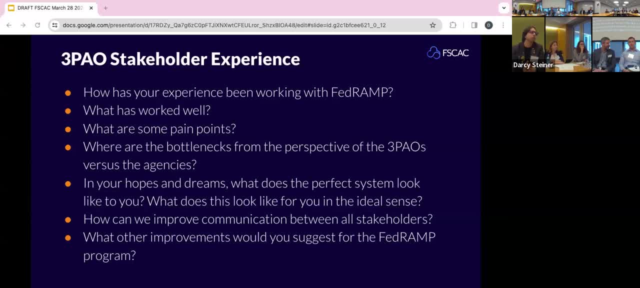 We don't waste a bunch of money with the assessment, And then when FedRAMP gets the package, they're not wasting their time and money reviewing that assessment. So that's a huge one for me. I'll carry on with. FIPS has been a bit of a pickle because early adopters got past it. 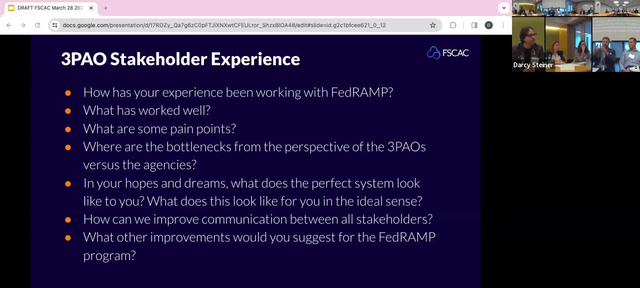 And then it's like, oh damn, this is a, this is a big deal, We need to really pay attention to FIPS. And then we kind of shut the door on it. You must do this. And then now we've sort of come back to: well, there's some risks. 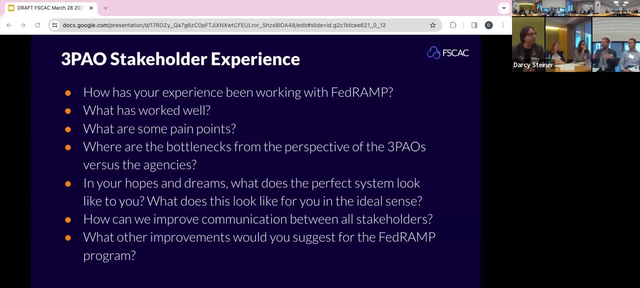 Yeah, There's some risk exceptions around FIPS that we can now make it. So, yeah, that's an area that we really need to put our heads around and get some clear, solid guidance moving forward to that allow folks that maybe were grandfathered like. 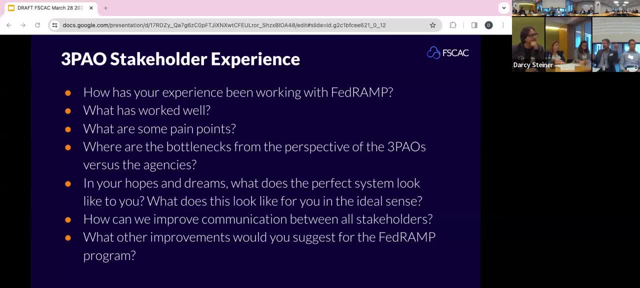 now, now in the annual, like you guys need to start working this, because this is now. you know, you don't get grandfathered into this anymore. This is the new rule and it's fair And one of the one of the constant. you know. excuses- not excuses, but the responses to 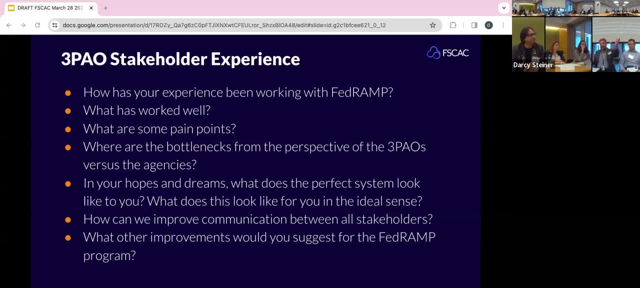 FIPS is like: well, FIPS can't keep up with us. You know, this module is years away from getting. We're almost, we're, we're, we're, we're, we're, we're- restraining ingenuity and advancement. 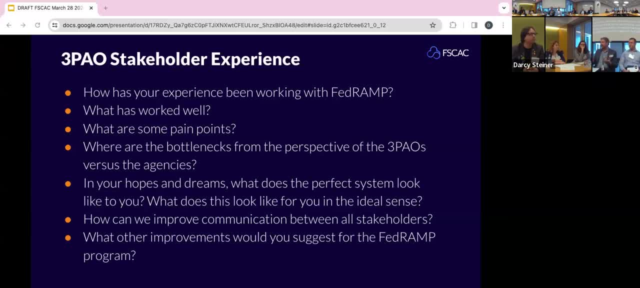 based off a law that you know. maybe we need to figure out how to better employ people in our risk acceptance process. I think that's how we can manage it. but, you know, put some, put some ideas behind how FIPS validation isn't an absolute. I figured that was going to be your number one. 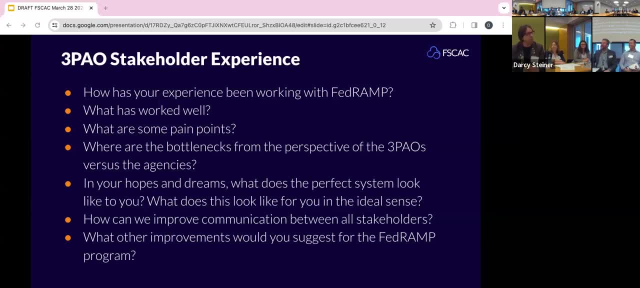 Yeah, I think most of us know. but while we're on the topic, not to take up the whole meeting again, as I do, But do you have a number two and number three, briefly, that you add to that list as well, I would have to say the AC family with a lot of MFA concerns? 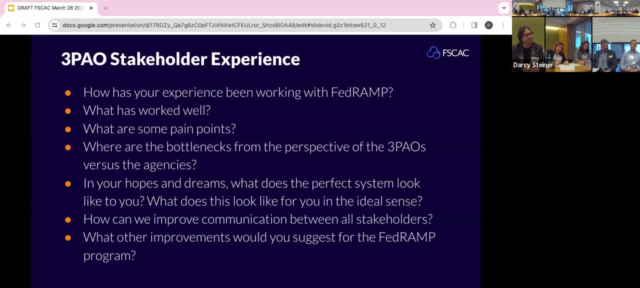 What is okay, What is not okay, Yuma keys- I mean this could go on again- not a whole lot of clear guidance and consistent guidance from Hey, you can use push, But you can't use this, And I know for FedRAMP's perspective. this changes, it changes every day, it changes. 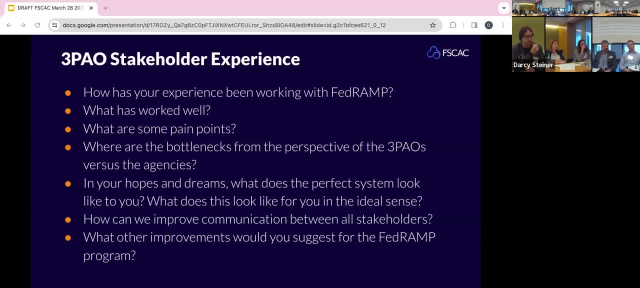 for us And, and every time I get an assessment where I've seen something that I haven't seen, I kind of have to reach out to FedRAMP and say, Hey, what's the latest guidance? Is this okay? And if it's not okay, what other methods do we have to use? 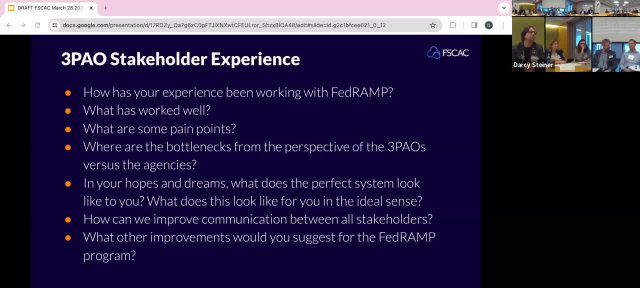 So and then you know you get into Microsoft. they've got multiple different technologies for MFA as well. So again, this could all go back to that portal, But you're going to get three PAOs. that says Hey, and it's updated. 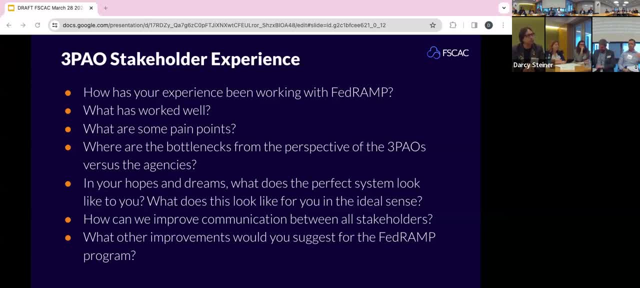 When something's no longer valid, it goes away. It's not on the list anymore And you can go to this portal and log in and say: Hey, I can use Entra. I can use Yuma key five, whatever it may be. 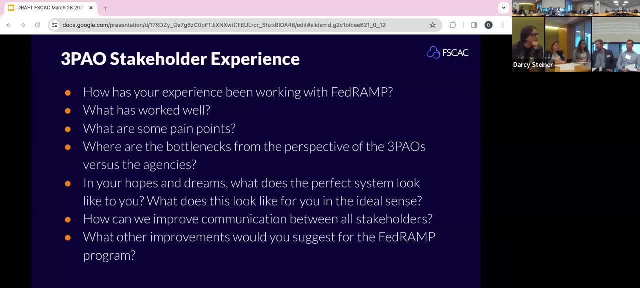 So I think that's where it's going to play. If I had to pick a third one, I'd probably come back to the risk exposure table, because that's what everybody looks at: Operational requirements, you know, vendor dependencies, risks. 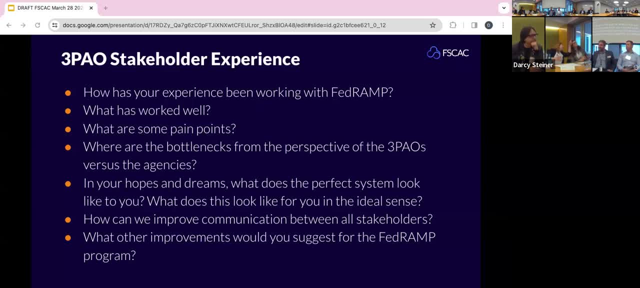 Yeah, Yeah. Risk deviation requests, risk adjustment: that's where the trust gets built or lost. It's like, okay, they've reduced this risk, but you know what's that telling me? And so I think we need to come back and look at how those things are done. you know what? 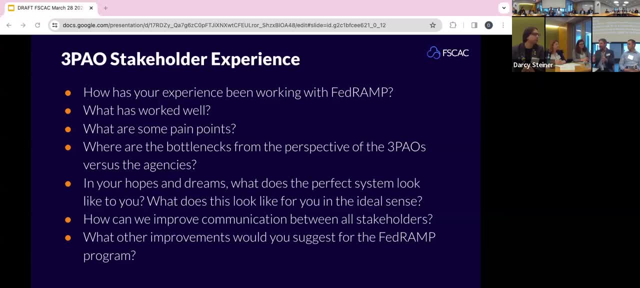 is a high vulnerability. What keeps it a high vulnerability? Because we're tied to the tools that are, you know, assuming that this is a public facing vulnerability And there's layers of protection down there, And so we kind of need to look at how we handle the deviation requests, because those come. 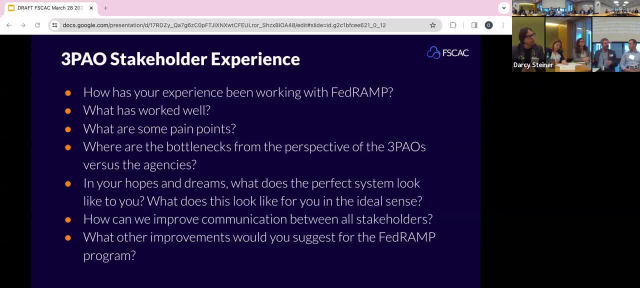 into play on the annuals. One of the most challenging things as a 3PAO is when another 3PAO did the initial and we're coming back from for the annual, And the first thing that has always blows my mind is the continuous monitoring. 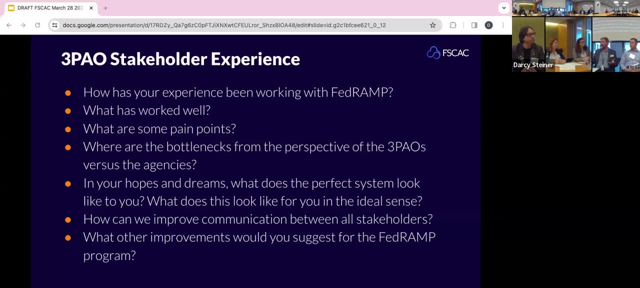 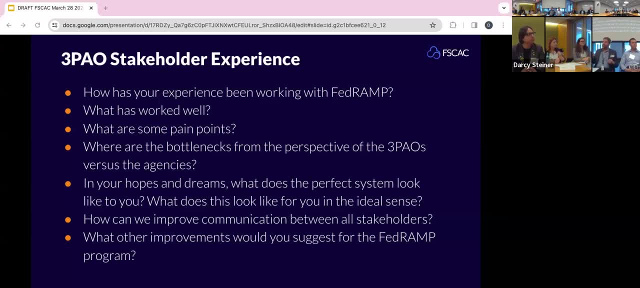 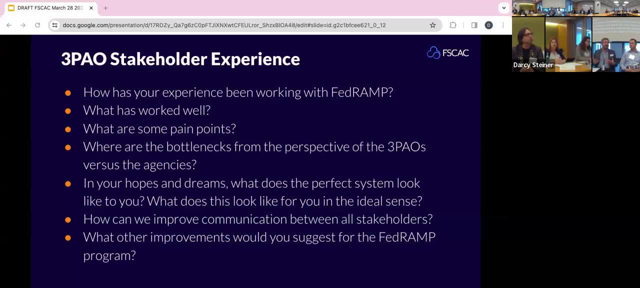 here we need to look at: Let's get the sponsor involved, Like a CSP is not because we talk about the investment that CSP they're making. they make it up front And then it's continuous monitoring. Once they get through ATO there's people walk away to other projects. 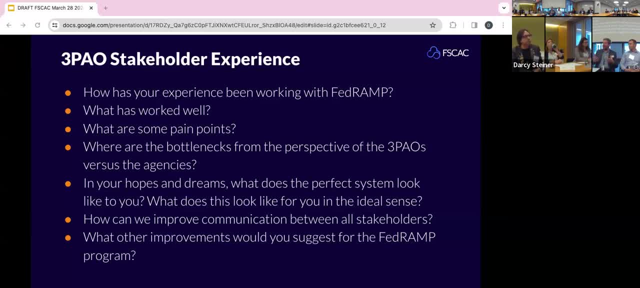 And it's about- it's that leadership commitment that I was talking about earlier- to make sure that they're continually improving security. Continuous monitoring should be about improving security, security, not letting security get diluted. Thank you, And we do have a virtual question from Daniel. 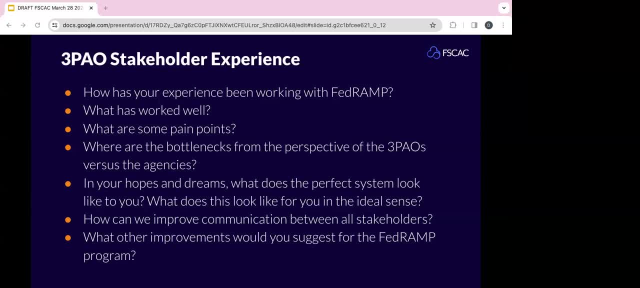 Go ahead, Daniel Hi, thanks, One of the things you know just in your experience. obviously you work with a lot of different CSPs. you know at various stages of maturity, And you know- I think one of the elephants in the room is the- you know the PMOQ right. What do you think is? 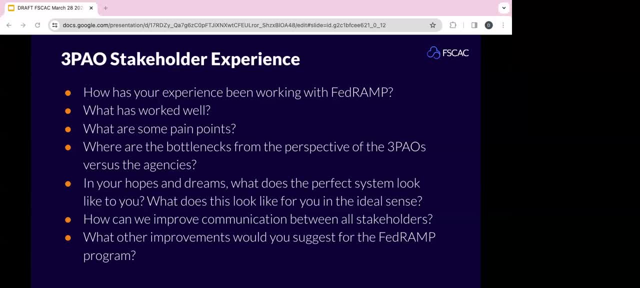 you know in terms of package quality. what are some of the things that you think can be done to help new CSPs get through the process cleaner than they currently do, And what can be done for existing CSPs to make sure that you know package quality is not a contributing factor to 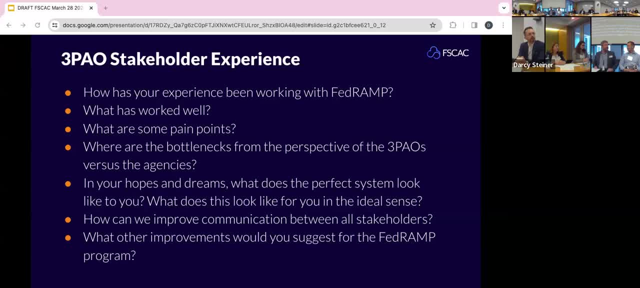 an extended queue. Yeah, I think I have a good idea. So I want to have some type of a quick check system which they can upload their SSP to. We can upload our system to their SSP. We can upload our system to their SSP. We can upload our system to their. 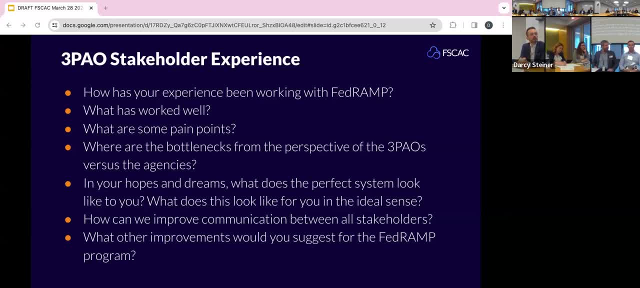 system. We can upload our system to their SSP. We can upload our system to their SSP. We can upload our system to their SSR, to the RAR, whatever it is, And it does simple validation checks. It's a check mark, a green check mark, you're good, And it runs. the FedRAMP set parameters. So if it's, 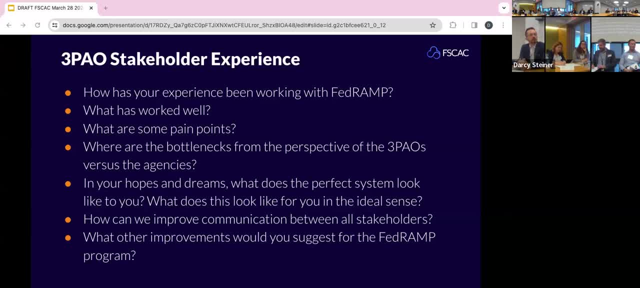 supposed to be 15 minutes and you have it for three hours. there's a red check mark. You need to fix that before you go to the next stage of validation. This tool can be fairly simple. I know there would have to be some changes to the templates along the way, but it would allow the 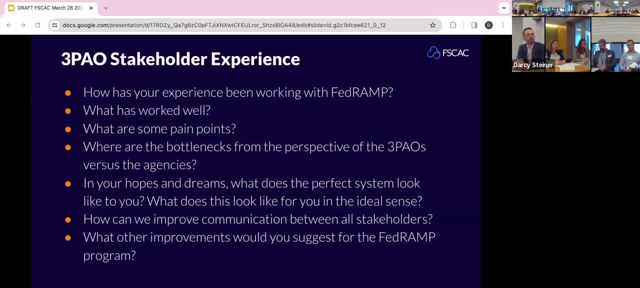 CSPs to do their own due diligence. They could upload their SSP once it's done, Do the checks on it, And they shouldn't engage with the 3PAO until they have that thing- all green check marks- And then the same with our SAR. Once our SAR is done, we upload it, whether it's a 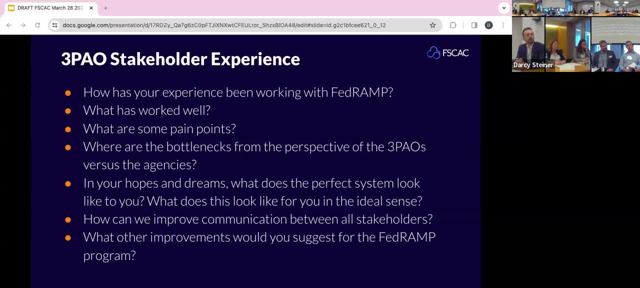 tool that's in USDA, Connect or whatever it may be. Until we get all the green check marks, that doesn't go to PMO review or the agency's review. Let's not waste their time. If we can't get our part right, there's no sense in wasting anyone else's time. So I think if we could build a system, 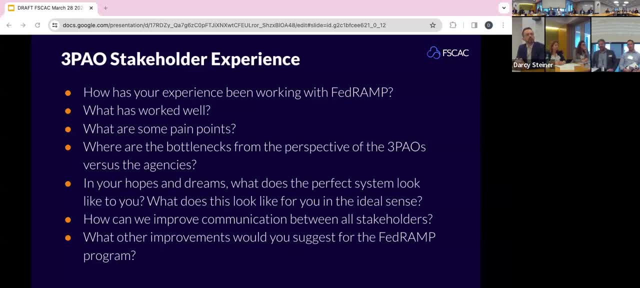 like that, you would cut that queue down to a third. I guarantee it because I know some of the comments that FedRAMP's getting that they're packages and it's not by any one person's doing, but there's simple mistakes that should have been. 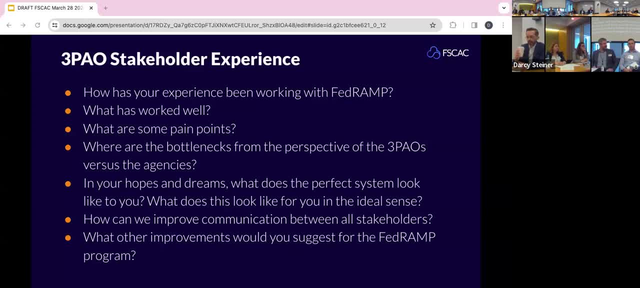 caught and for whatever reason they weren't. So let's automate that process and let's take the human factor out of that, those simple mistakes. The review queue is getting clouded with non-security impact-related deficiencies or errors. Mike from CSPs, I just had a question. 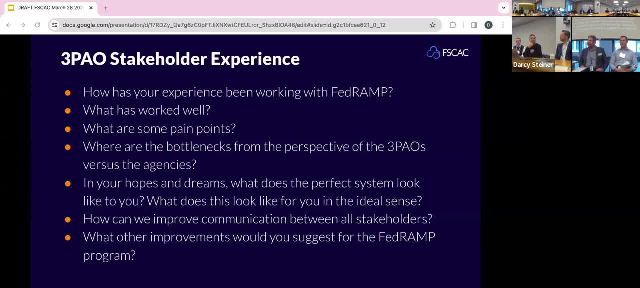 around, minus the simple things. So if we've got those off the table for you, do you see any interpretation issues in guidance between different reviewers? Absolutely, And that goes back to the strategic part and building the trust in the 3PAO through. 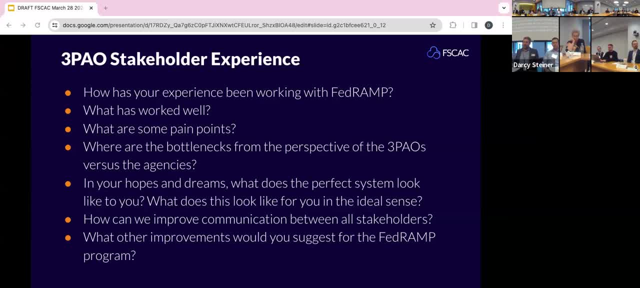 more interactions with the PMO. I couldn't tell you if the PMO reviewers how many FedRAMP assessments they actually worked on, but what they don't get, they don't get the value of actually performing the review. So I think that's a good question. 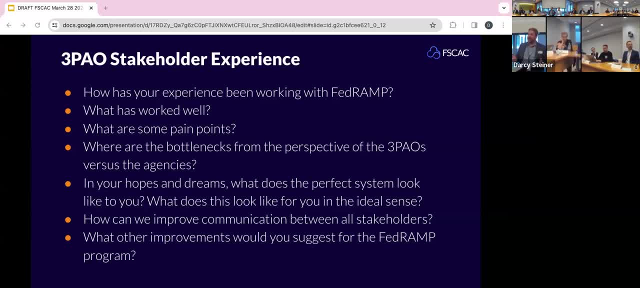 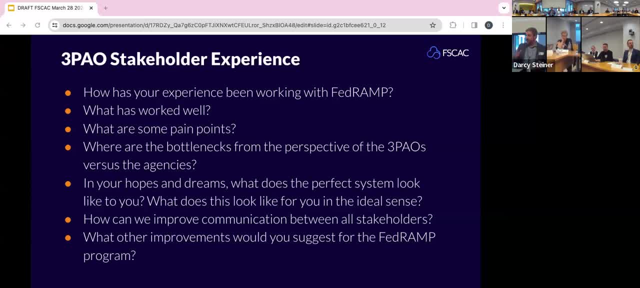 passed because we looked at this and we validated that and it includes all the information in there to hopefully give a reviewer, a government agency that wants to leverage the package, enough to say, yeah, I trust that this was done fully. It's not going to answer every question because it's impossible to repeat, Otherwise they were. 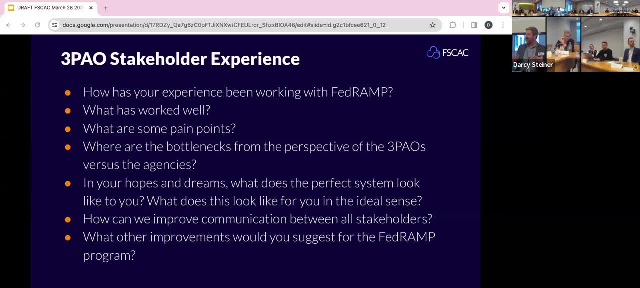 actually performing another audit to gain understanding of the system so that it answers all their questions. And so I think we need to bridge the gap of what the 3PAO authorization recommendation means and make sure that that's agreed upon by the community, Because what it 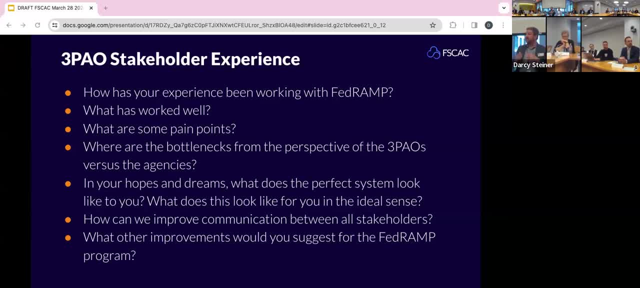 means today is it means it's going to pass FedRAMP PMO's litmus, not the. you know what the tolerance of a particular agency is. And that's when we get into those disconnects where it's like, ooh, should I have maybe? ooh, I didn't think of that, But I mean that's from my perspective. 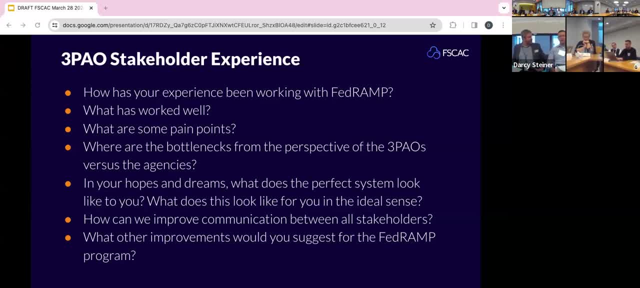 On a positive note, I will say the reviews that I've been in as of late, the actual reviewer that reviewed a family or a set of families joins the review call with the agency and the CSP and they go through their comments and talk to them. So it's not hey. Bill reviewed this. 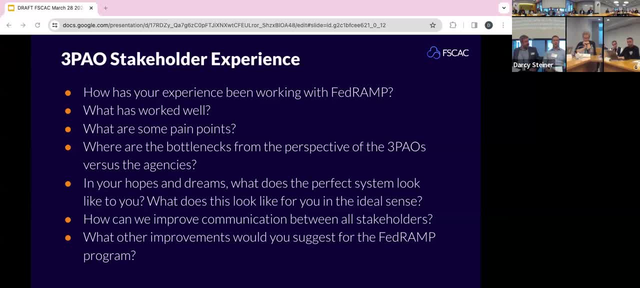 family. It's not, hey, Bill reviewed this family. It's not, hey, Bill reviewed this family. Cindy reviewed this family. They're actually on the call with us, So if we have questions in their comments, you know it used to be well the person that reviewed that's not here. It was. 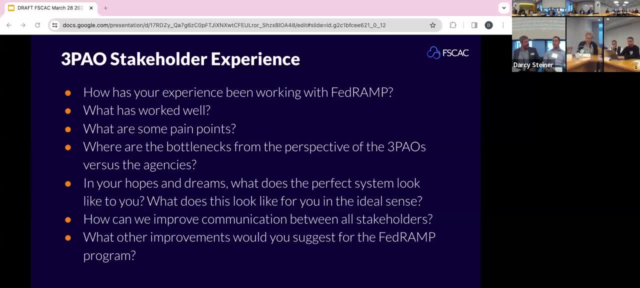 reviewed by. they're on the call now So they can answer a lot of those comments and those questions and help us update accordingly and get to a positive reputation. And be honest, these are humans, We're humans doing this. The assessor is a human being. They have their 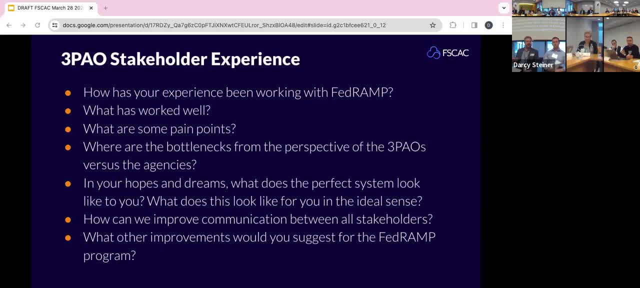 interpretation. They have what they've seen before. You know, an experienced assessor has seen controls implemented a myriad of different ways, And so I think it's important that we make some great consultants from seeing how new implementations are done And it becomes an. 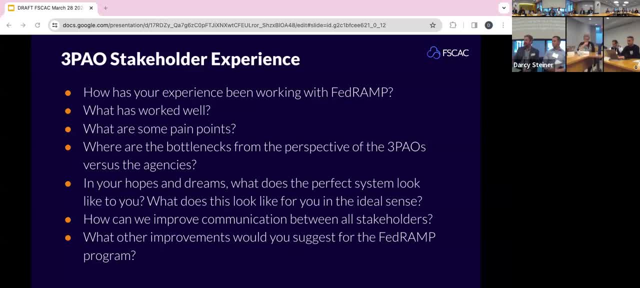 interpretation And sometimes you lose that If that individual isn't around to answer the question from the PMO. we've lost that because you know they've written it down. But we can't recreate that moment because when we do an assessment we're sitting with the engineers. 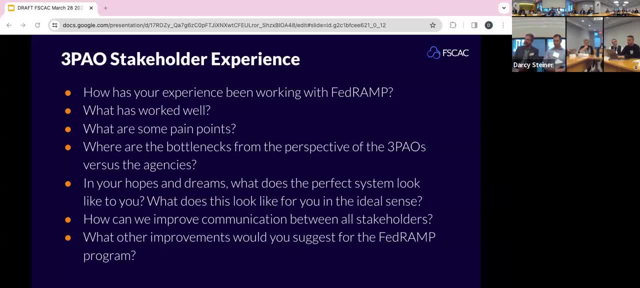 Our process is to drive to the evidence we need and capture it then, And so it becomes. it's a journey. An audit is a journey, It's not. it's not anything else, It's. we're leading down to answer that question. I'll go back to. 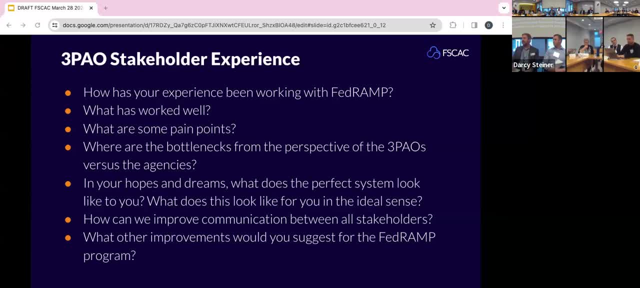 this is good enough, They got it. This passes the control, And then you move on to the next one, because there's 400, now right, And some of them intertwine too. So we could probably work on how we can look at efficiencies across the control families. Absolutely. 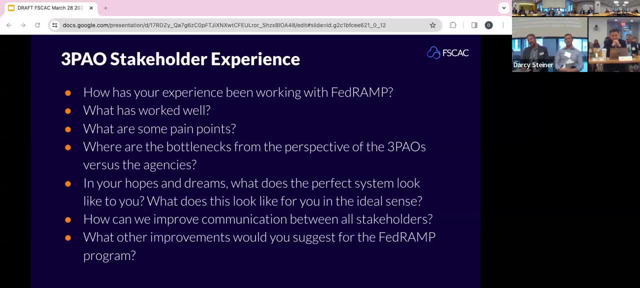 Hey, real quick guys. Bo GSA, I'm curious: have you found a particular set of conditions that would drive one CSP over another to want to go through and develop and build out a Gov-only cloud environment, vis-a-vis essentially building something into their existing commercial offering? 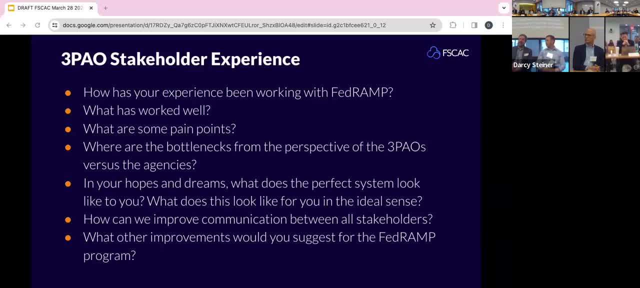 This comes to mind. but I mean if they have, if they have the ROI, you know, the return on investment, or it makes sense that they, because they're essentially creating a replicating, a commercial cloud just for government, And some, some, some CSPs, have done that right, Is that? 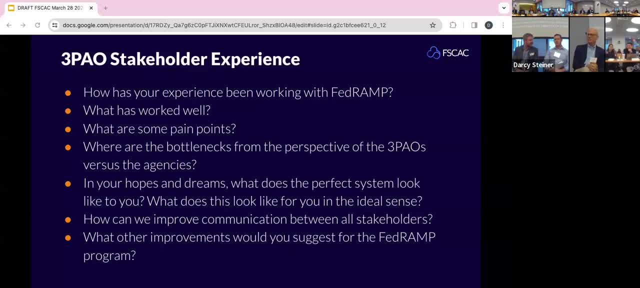 is that I'd say the reason that I see it is because of the external services requirement and they have to use FedRAMP authorized services. So they build out a separate environment from their commercial offering strictly because of the additional cost of having to use tools, external services that are FedRAMP. 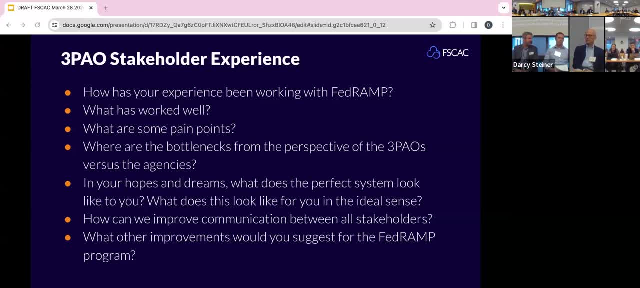 authorized, Because if they don't, they get into all kinds of issues which will likely prevent them from getting authorized Or employing controls to other commercial entities that don't require the level of rigor. right, And so it becomes: oh, if we, if we. 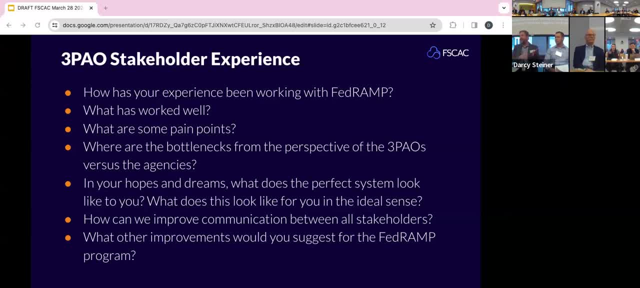 put these controls now we're harnessing and irritating our, our other non-government communities, So I think that's when it makes the bridge to. we need a government-only cloud And oh, by the way, there's enough interest in it that we're going to get the return on investment because they're going to. 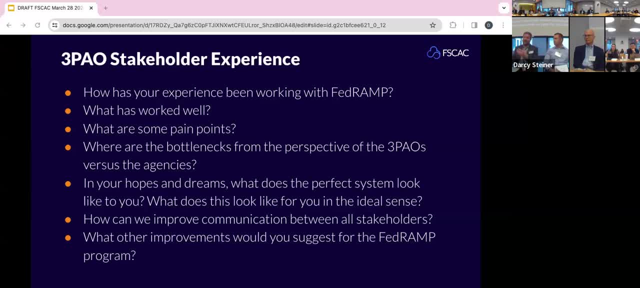 charge more for it. It's going to be a government decision. The commercial cloud is cheaper than the government cloud. It always will be. Yeah, I think the emphasis is that if it's good for government, it's good for everybody, right. 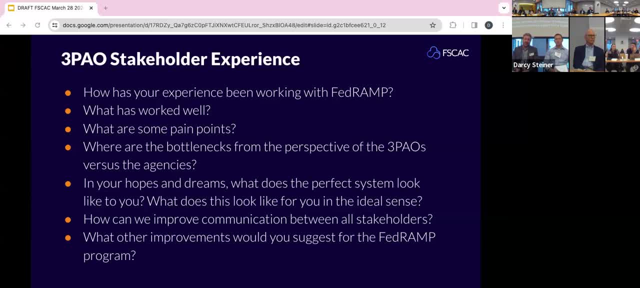 And you know, good security is good security right, And if there are a specific set of conditions that are driving decisions to be made around, build something unique for government that is separate and distinct from what is the base offering for everybody else. So the external services: 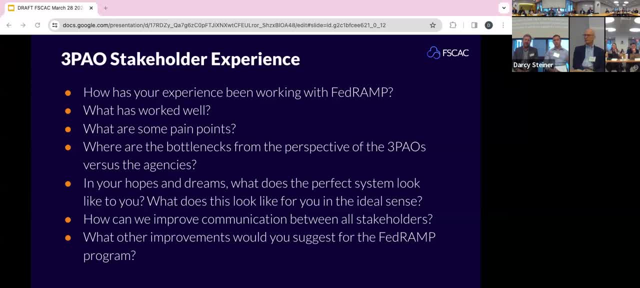 I think Lee said it right there. That's an important one, And there's there's tools out there that everybody knows that are excellent: Jira, for instance, Everyone wants to use it, but it's not FedRAMP authorized. So 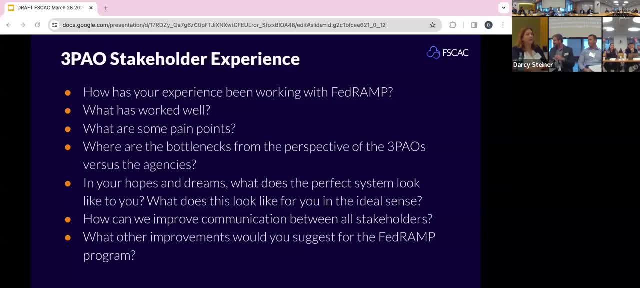 Hey, can you share some examples So like I can imagine that, like if there was an infrastructure or a service provider that was not FedRAMPed, that like a CSP was deployed to, then that that could lead to this sort of like. 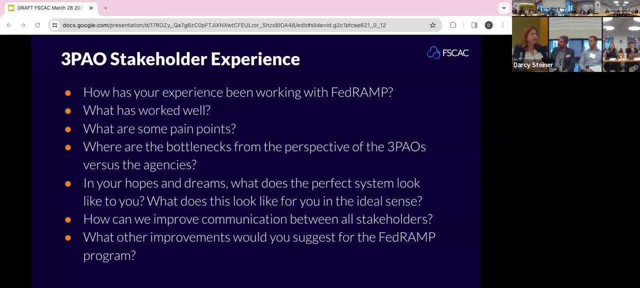 inference that you need to make a version of something, But I think all the infrastructures and service providers have been FedRAMPed at this point. So is there like a specific example right now that you could share about when the external services requirement- like recently growing the CSP- to sort of fork and make a government version? 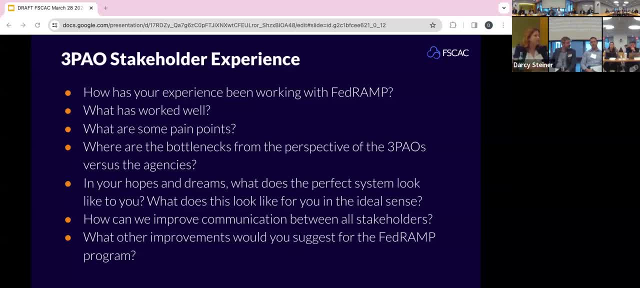 Yeah, I mean I can think of a couple, but typically it's not the big services that they need that aren't authorized, It's the smaller sub-services. Like everyone wants to use PagerDuty, That was one that we beat. 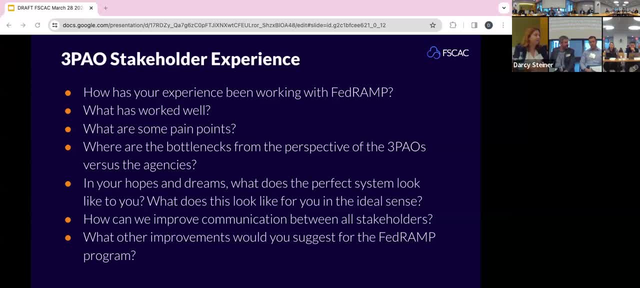 to death, but they couldn't use it. or they could use it, but they had to dumb it down to the point where it was absolutely useless to use, where, hey, there's been an incident login to look at. That's basically all you could get out of PagerDuty. 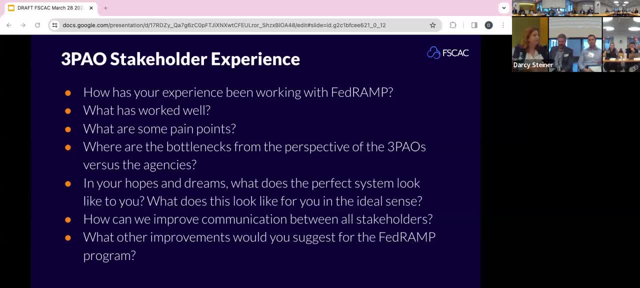 which is not what the tool is really designed for, And it doesn't really help anybody. You don't know if this is a serious incident or a false positive or what it may have been. So that's an example, And the JIRA one we used to be able to get away with. 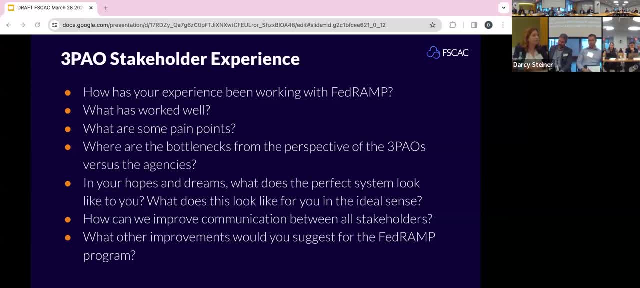 They could move JIRA into their boundary so they could use the in-boundary version of JIRA, And that was OK. Well, JIRA is allegedly stopping support on that And FedRAMP doesn't really like anyone using it because they know that the support is going to stop. 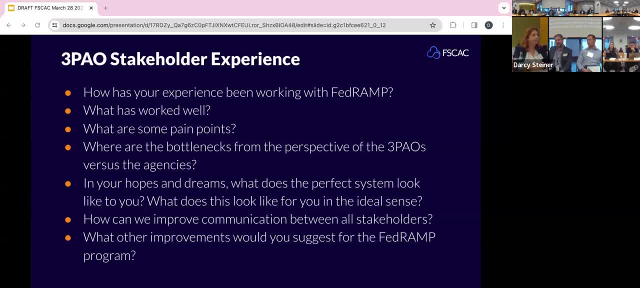 So you can't use the cloud version because you've got sensitive federal metadata or data going into that, which is leaving your boundary causing concern, which is 100% valid. So for those CSPs, it leads companies to do a self-hosted version that increase their maintenance costs and their security. 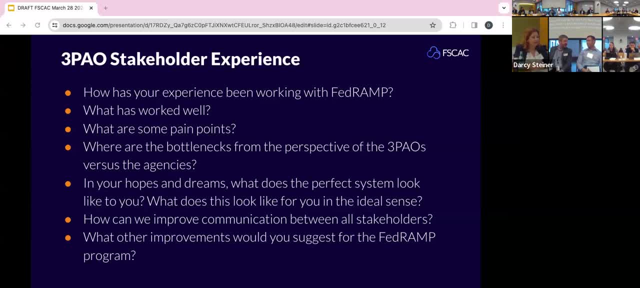 Or they've got to re-organize Right, Or they've got to re-organize Right, Or they've got to re-organize Right, Or they've got to re-organize, Or they've got to re-architect their commercial version away from. 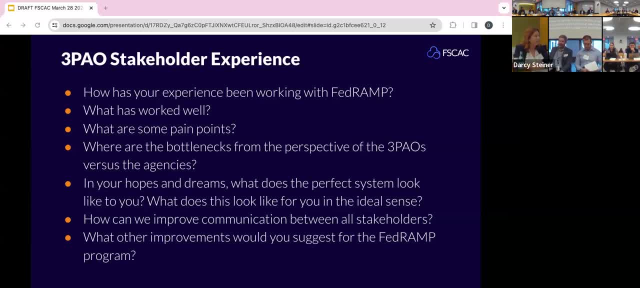 It's bringing stuff into boundaries. So it's corporate services too, not just third party. These CSPs have developed all these developer processes and everything else. Their SDLC is reliant on their corporate. Now it's like: oh how, then the metadata is what causes the problems. 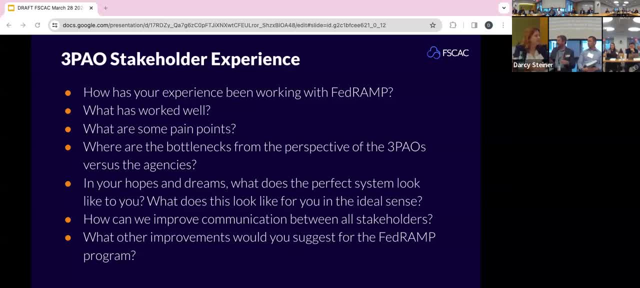 It's like, oh well, we can't draw the boundary on corporate because we're not going to pass, So now we have to either figure out how to handle the metadata that goes into corporate sensitive metadata, or we need to actually stand up an instance in our boundary. 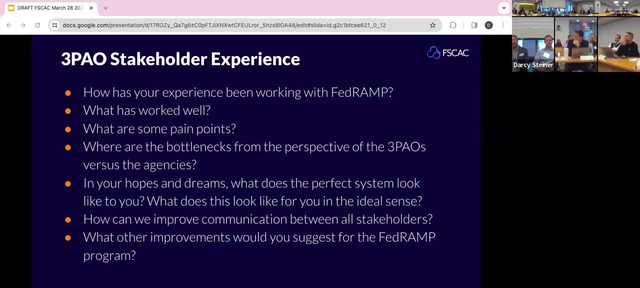 Any other questions, If I may, Jackie? I mean for DOD. do you guys require CMMC for the set of service providers that you leverage? grant authorizations from CMMC is not quite there yet, And so that's really not my area of expertise. 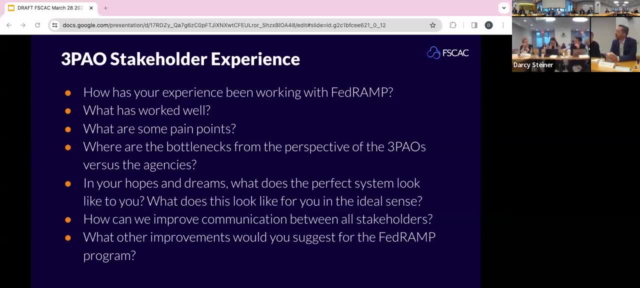 But you know, I don't know how they're going to handle it. I don't know how they're going to handle CMMC relative to FedRAMP, And I think there's the intent early on with reciprocity, but I don't know where it is. 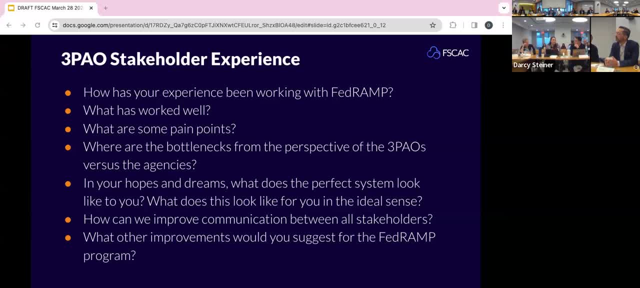 But I can get the answer to it. That'd be interesting. So for CMMC, the proposal was released on December 26th, But one of the things that was in there is it follows basically what's set in DFAR 712, which bifurcates: if you're cloud, go do FedRAMP. 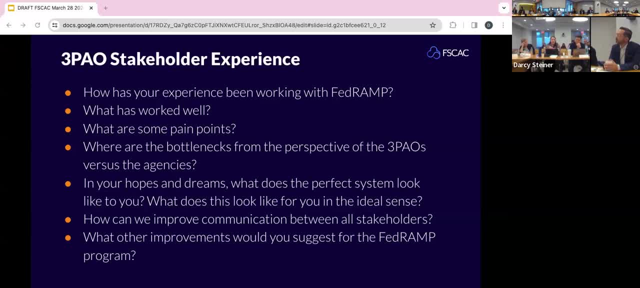 If you're not do 171, all the subsequent clauses. That has been true And that is essentially what the proposed CMMC will allow for. So, as an external service provider in the context of CMMC, So any of those external service providers handling CUI, if you're a managed service provider, then you have to do 171 and CMMC. 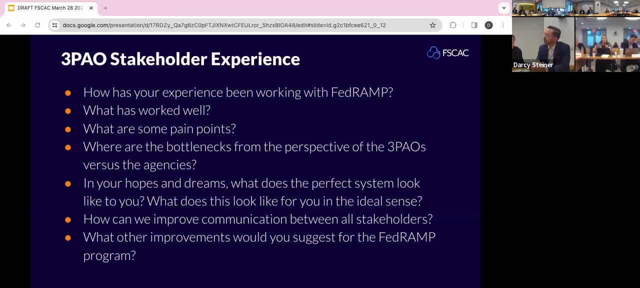 But if you're cloud, the requirement for FedRAMP still stands, which is very interesting in the larger context, And I wish I had thought of that when the OMB folks were here, because there's also the FedRAMP, the FedRAMP equivalency memo that DoD released. that basically said: hey, if you're not FedRAMP authorized, you have to be equivalent. 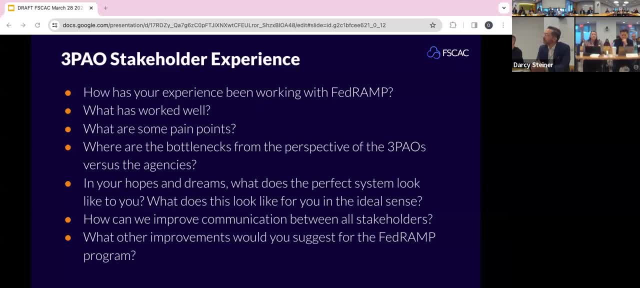 But that is a higher bar for a variety of reasons, And it also highlights just the lack of authorization paths that are available to CSPs right now. So my understanding on CMMC draws a larger boundary than FedRAMP does. FedRAMP is for cloud systems, CMMC is for business processes that incorporate cloud systems. 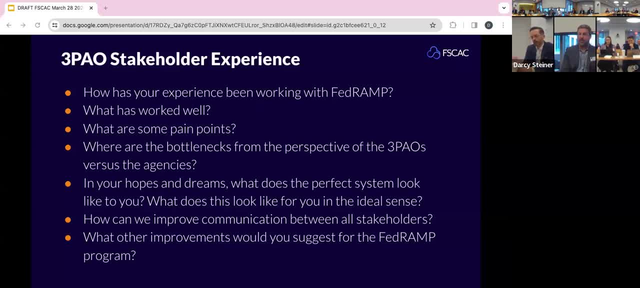 So you're drawing a larger boundary. So you know, the FedRAMP first makes sense because, OK, now if we get FedRAMP on that cloud service now we can focus on the other elements of this boundary, you know, and we can maybe inherit that piece from FedRAMP. 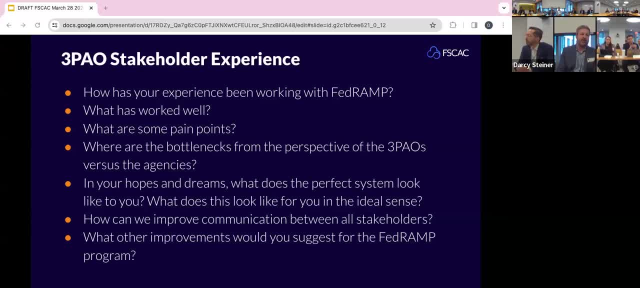 Now we focus on the business processes that CMMC also encompasses, And so I look at CMMC a little bit different. IAPRI is another emerging framework that's out there. that's more. you know, product-less focused, right, You know. so you know we have to look at. 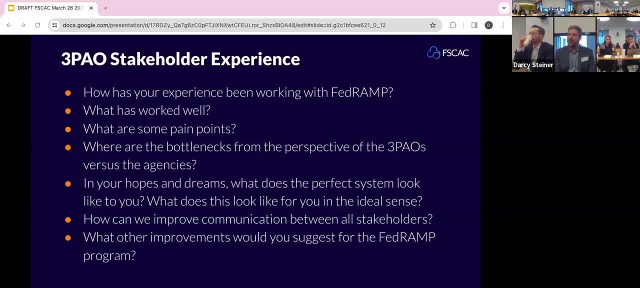 how the scoping draws around these, these requirements. It's a little bit different for each framework, but they can benefit from each other. I raise that because you know CMMC is really focused on ancillary data, CUI data that would essentially be in the context of a new organization's corporate network and further in support of a tech-related element. 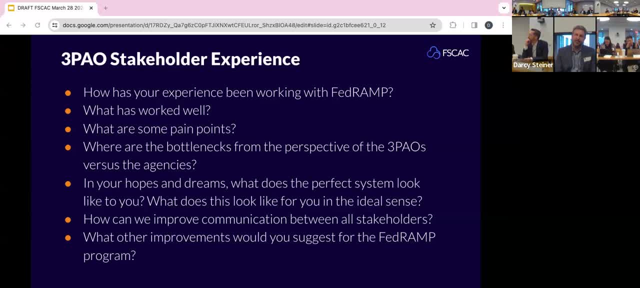 So, you know, particularly when we're having this boundary scope discussion, there might be an opportunity around, you know, as opposed to saying, extend FedRAMP all the way into the corporate interests of an organization, perhaps looking at the interplay between one and the other. 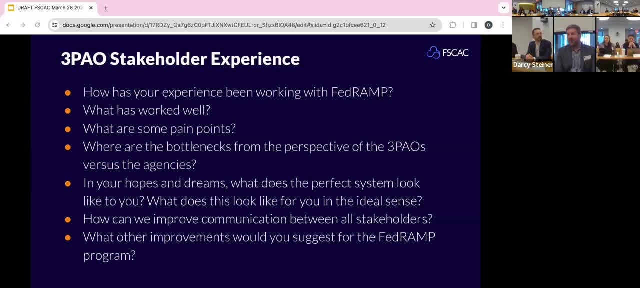 That would be great If CMMC was operational today. then we could be gaining some efficiencies from those assessments that have been done on the services, because, yes, now you're creeping more into the corporate side of the boundaries, Jackie, One of the things that 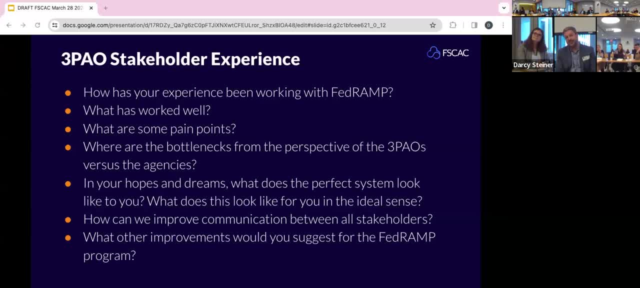 that we're trying to work for is what is our next year's priorities, And one of them that I took from y'all's discussion was that how do we get FedRAMP guidance out quickly for how it affects the agencies doing authorization, the three PAOs and the review process? 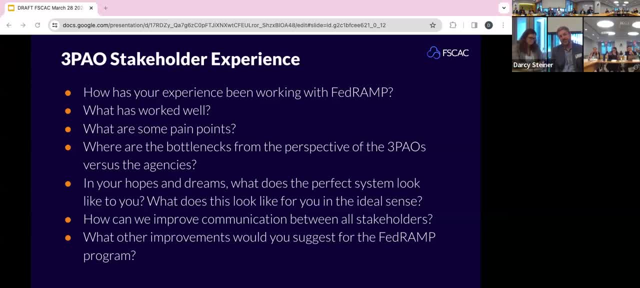 And so I would be interested. you know, I heard you know, FIPS is one that's near and dear to my heart. You know, one of the ones that you talked about was, um, uh, operational requirements- deviation requests. 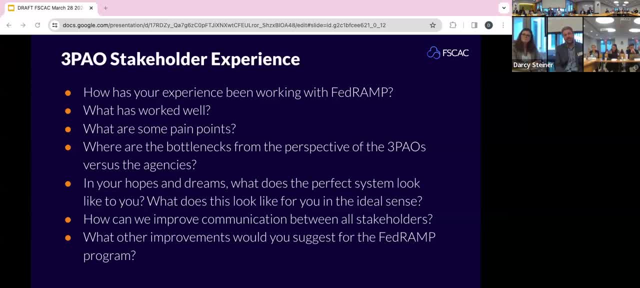 And I have to be honest for an authorizing official, it drives me crazy. Um, I get um authorization recommendations, um that have, um. I'd like you to accept this operational requirement. There are no mitigations listed. 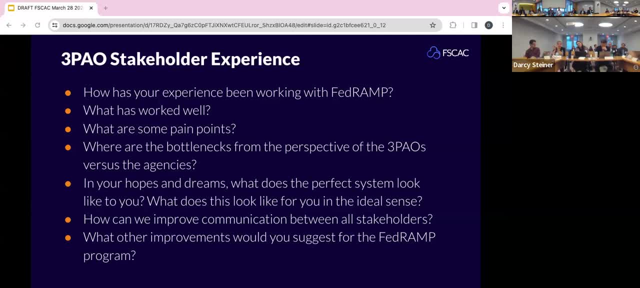 Um, sometimes they're patches, and never should a patch be an operational requirement, um, unless it really just breaks something, right? But, um, and so it having those standards and and things to really tell me how everybody's considering these. 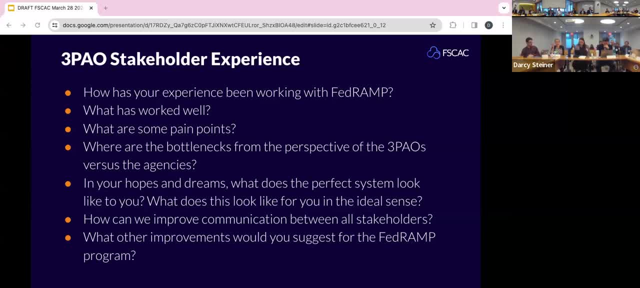 um, I think it's critical. So I'd be interested to hear you know if you had a top five list that FedRAMP could push out. quick guidance, you know? and how do we do that in an agile way, You know? 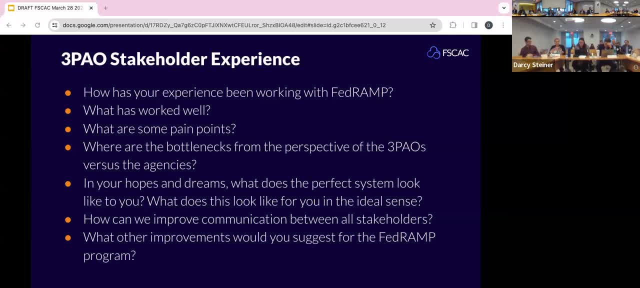 what are those things that you see the largest issues around that FedRAMP could assist the whole community with? Yeah, I think around those, specifically around the deviation request, which includes the risk assessments, operational requirements, vendor dependencies- we need to take a closer look at that because, honestly, 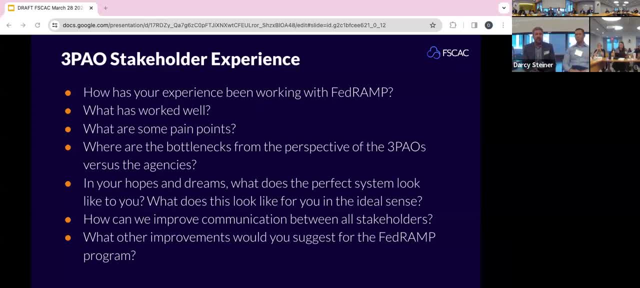 you're absolutely right. If they spend some more time, they can reduce some of this risk. And what we're based from a 3PO perspective is: well, is it good enough? Is it going to pass? You know this is. 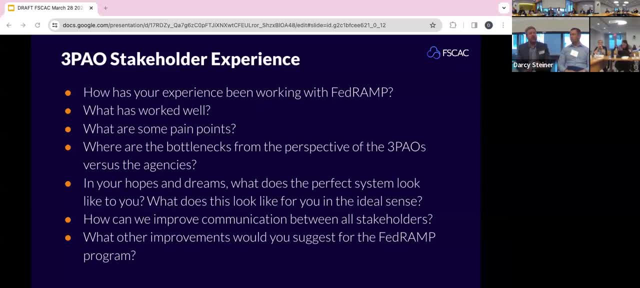 this. we'll- we'll address this later. Is this enough to get us our ATO? And so they? they want to rush. they're rushing to get their ATO so that they can celebrate, And it's like selling their product. 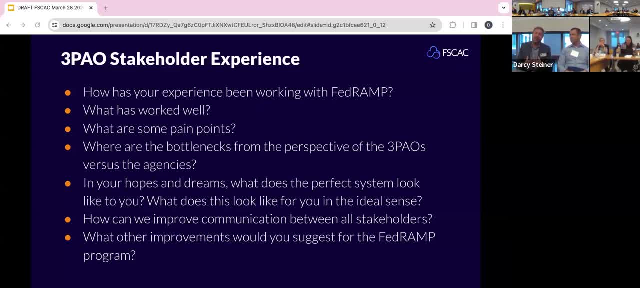 And so if we establish some sort of criteria- you know how I address it personally. when I go into contract with the CSP I- I say it all. it doesn't include risk- adjust the deviation requests to get them to fix it. And if they, 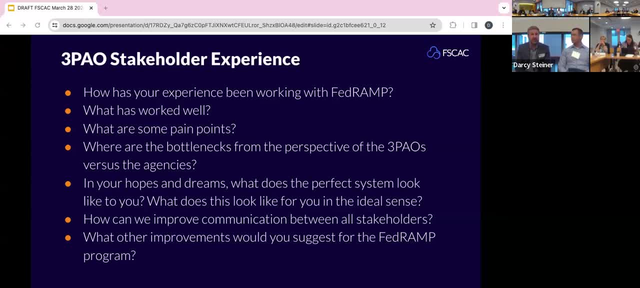 they try to do deviation requests, it's going to we're going to charge them more for it, And so that's that's a tactic that we use to get them to fix it and not try to pass forward unnecessary risk. But I think we can do a better job. 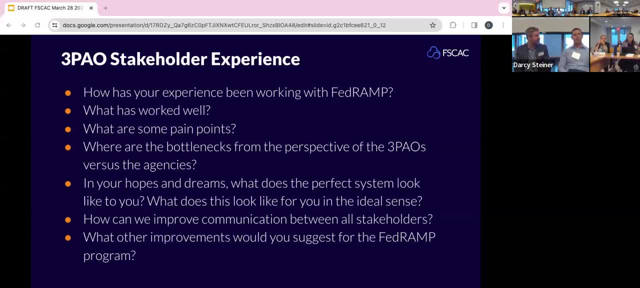 Better job addressing it as a whole to put some guidance out. Usually you hear all we'll address with the agency later. Let's just get through this. That's the typical CSP response, which we know is not valid, Coming at a lot of this from a position of ignorance. 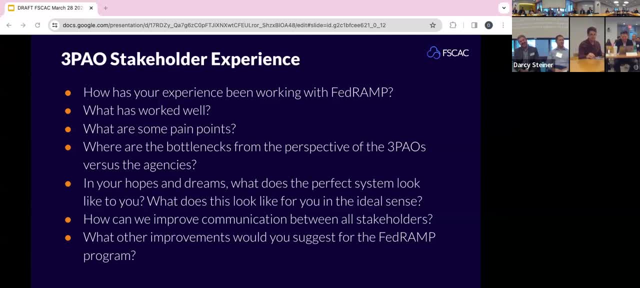 So that's my caveat. There's a lot of talk this morning about metrics and and and data. The three PAOs are a great source of metrics And and data around the pre FedRAMP security state of the potential CSPs and the post and the potential Delta that has occurred versus then what comes into the government marketplace. 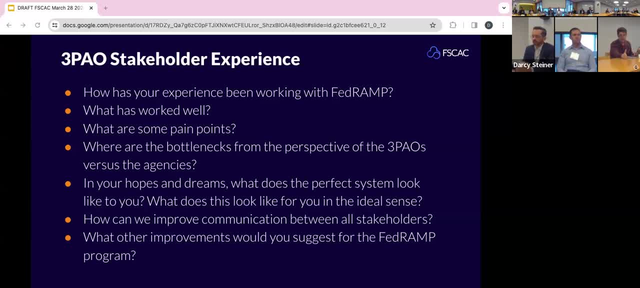 That, though, puts you in a weird position if the government is going to try to potentially collect that from you with respect to your customers, right? We have NDAs with all our customers, right? So how do you anonymize? Could you envision a method to anonymize? 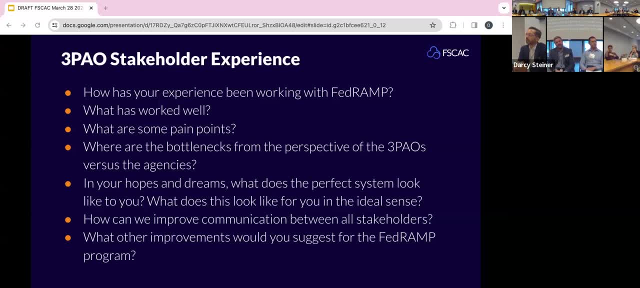 Not just who the information is about, but also whom is delivering it. So not only do we not know necessarily who the CSP is, we want to know who the three PAOs is as well, So that at least some Delta measurements over time could be looked at. for is the program actually improving the secure state of the CSPs? 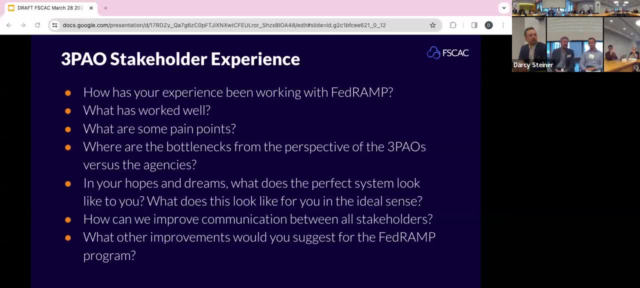 Does that make sense? I think that's a responsibility that the three PAO community has to take on. That's a responsibility that the three PAO community needs to all get together and meet on and discuss to see what, what type of relevant metrics can we get and how can we de-identify them to make them useful for the community. 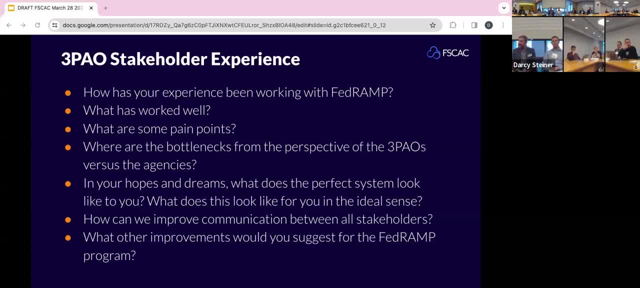 Yeah, I think we could do that. But CSPs, I'm curious too, since you have that aggregate view, like would we be able to get which controls are coming back tonight more often? Like which controls are CSPs pushing you on? 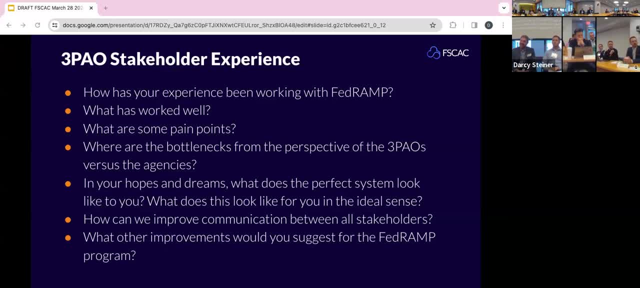 maybe right To try to and we see failure or we see, you know, cycles that are burning time. There's lots of there's lots of stories and similarities that we can share. I have checklists that I obviously you know. 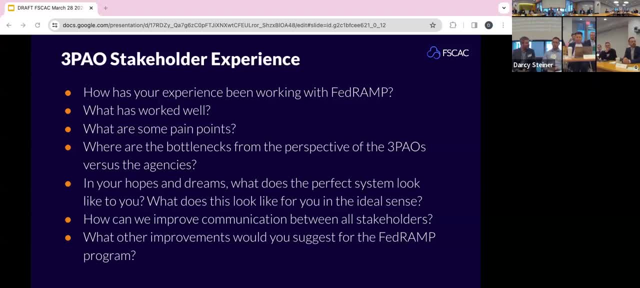 as being the quality director I look at. you know every report before it goes out, So there's ones that I zone in on more because I know that it's going to be under scrutiny from the FedRAMP reviewers. So you know. 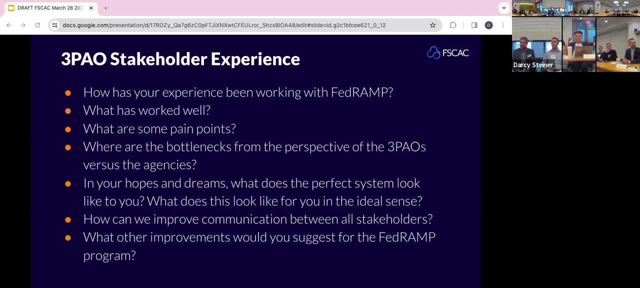 I have a lot of those metrics and I've worked a lot of that stuff for quite a while And we're, Lee and I are frenemies But we are friends. I think if we can connect that with the GRC tool that's coming up, 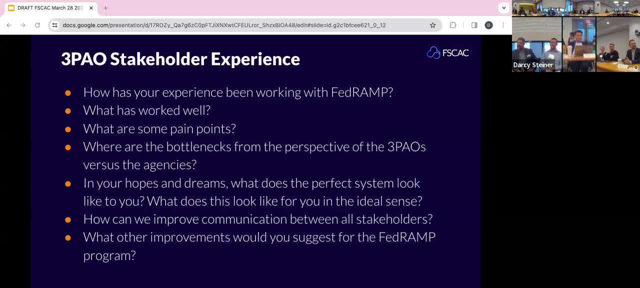 Absolutely Like having that level of visibility, that because then in CSPs perspective, right, we can start to say, all right, we're AC1.. I'll just pick on that Like if it's AC1 that's constantly failing and causing 60% of our failures. 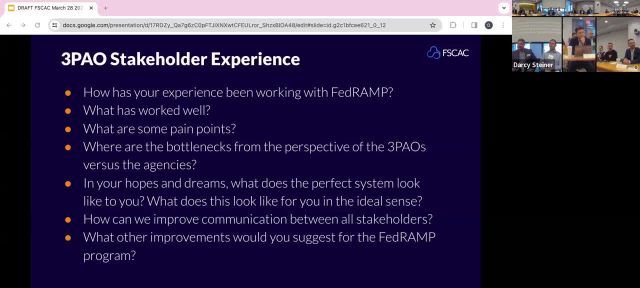 like we have to go back and look at that across the industry and say we're approaching this intellectually. That's a good exercise. It's a bottoms up to figure out: what do we need more guidance on? So just ask ourselves: that question pulls out. 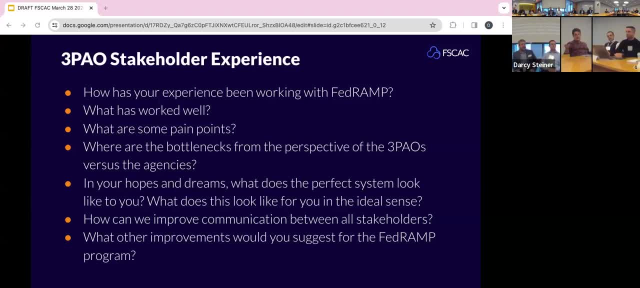 These are the areas we need to focus on. So I think it's a focus on Right, And I'd be more concerned if it was DNSSEC versus the quality of the paper package, for example, which you mentioned both, And there's the review reports that FedRAMP uses as well. 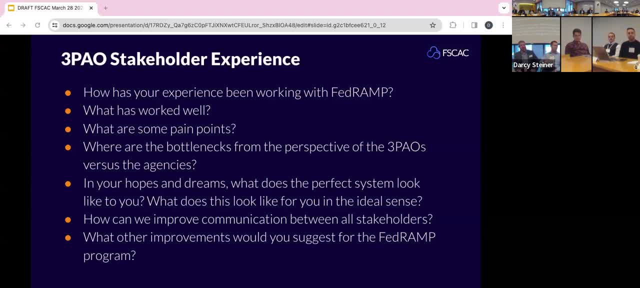 And you know they have about 40 controls that they really hone in on as part of those reviews. You know that would be obviously the best place to start, because they've picked up these ones that are typically major failures And they've adapted that list for REV5 as well. 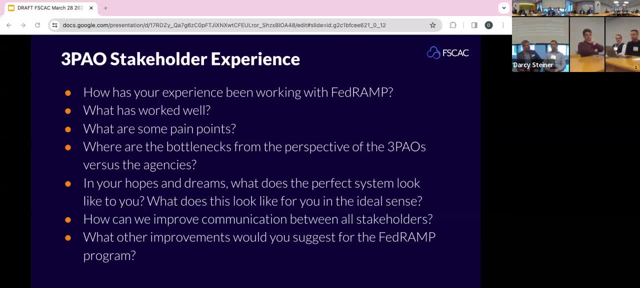 So they've almost established their own top 40 critical controls, Right, Yeah, And everybody? I mean I don't want to speak for everybody, but I think we all look at those ones with the most quality. He wants to call it. 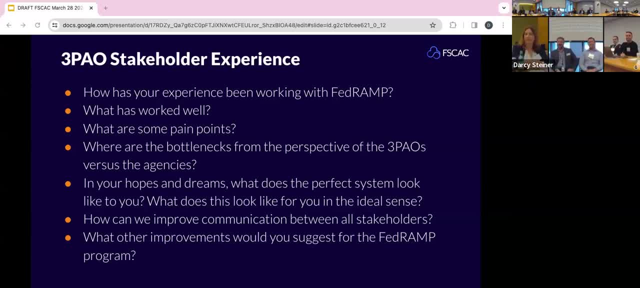 But yeah, I'm sure my quality is pretty good. We are scheduled for lunch now, So if you face to, So let's be brief in your, in your questions. How is Jackie Stonkworth who just said: how are you all, or are you incorporating size of bots? 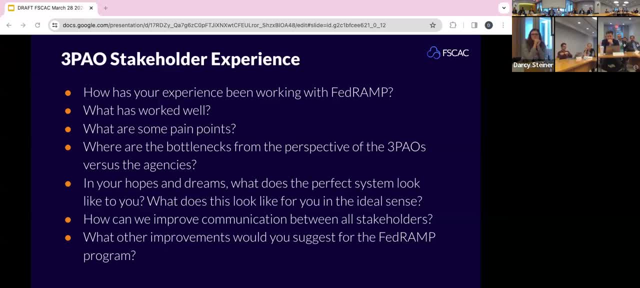 and any of the other emergency directives into your assessments for validating compliance. Yeah, that's, that's a good. that's a good question because you know we're probably not doing a good job at it And we see those come out. And we talked through it with the CSPs. 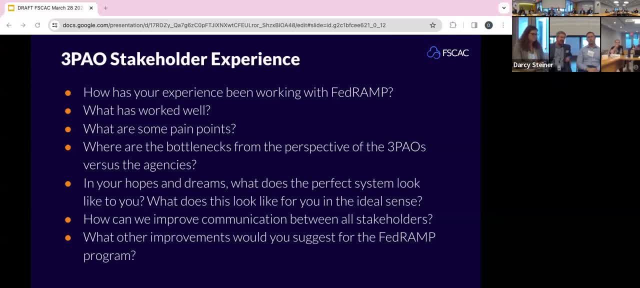 Like, what does this mean to us? And you know it doesn't become a measurable thing because you know, I think there is for 1801, which is the spam protection one, That's the one that FedRAMP really harps on early. 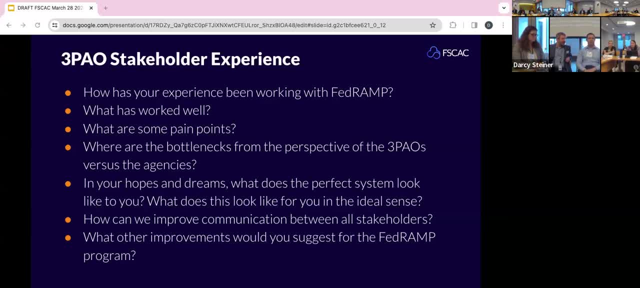 I mean that's probably the main one. I think that's looked at the most. I mean, Marcy, the FedRAMP doesn't integrate it into the requirements. So I mean, this is part of this like cyclical: Identify an issue, talk about an issue and it becomes an issue at the end. 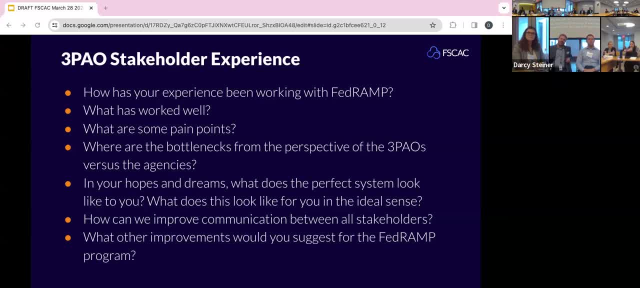 but if we put it in the templates, we put it in the documentation then, But, like right now, there's there's no way for us to validate odds. Yeah, And so this is a concern from the DODIG perspective And I'm having to. I have a finding against me that I have to work with FedRAMP to implement it. 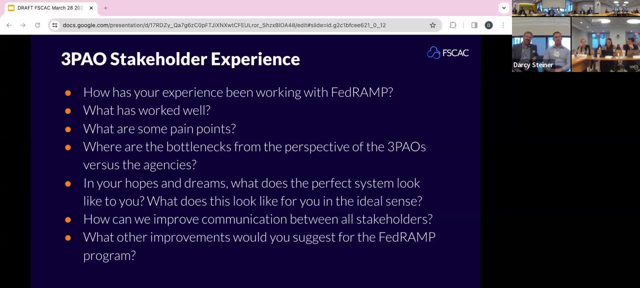 But yeah, it's been an interesting one And so. but so from my perspective, I mean, we clearly have right now a lot of significant activity against our cloud infrastructure And we've issued bots on F5s and we've issued just Cisco devices, ASAs. 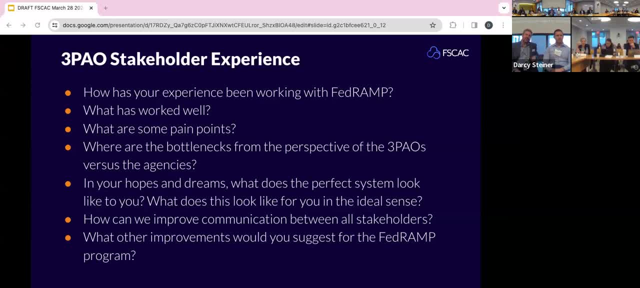 And so the question becomes is: how do we leverage our three PAOs, How do we get guidance out to our CSPs that require compliance and Kanban to answer up to these, to make sure that we are compliant? And I just think that in our annual assessments, our initial assessments, in our Kanban, 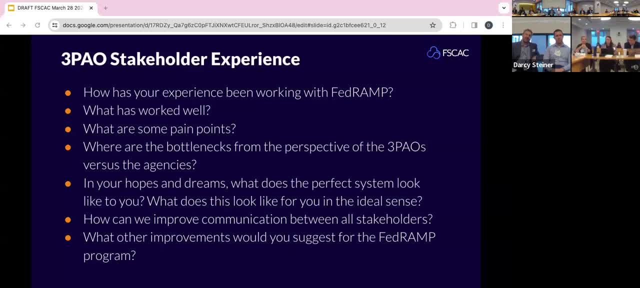 we've got to figure out how to address These because they're coming after I think. I think you make a good point and is is annual. soon enough, right, The next annual assessment, because you know you could do it that way where it's like: OK, these are the, these are the bots that have come out. 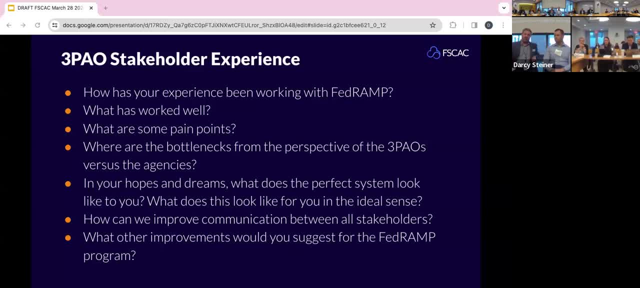 This is now. we incorporate these- whatever, whatever the requirement is to validate that this isn't present- into the FedRAMP SAP And then then you get the outcome of those results as part of an appendix or just included in, And the scope of Of the test case workbook. 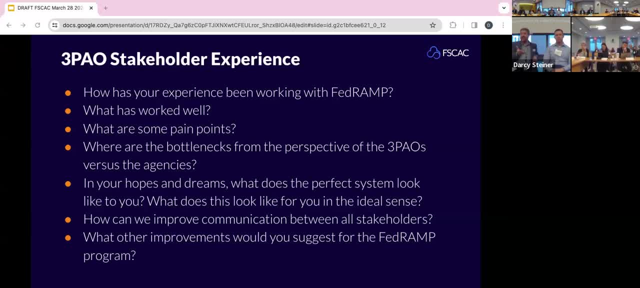 But if it's something that needs to be more proactive- like that's like us. you know we talked about system, you know significant change requests- like we need to. We need to now go back to all of our. if we're assessing any of these customers now it's basically an all call for me like hey, hey, customer base, we all need to come back and we need to validate this. 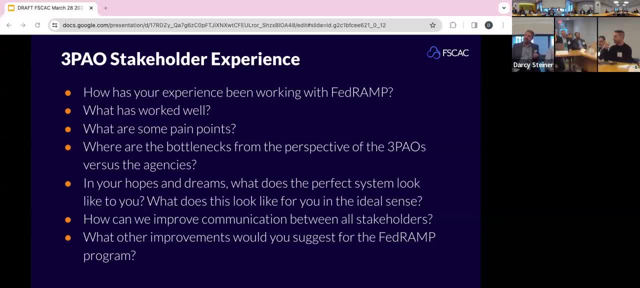 I just wanted to add in on that- I think that was my question earlier around baseline and change as well, Because I think The sort of huge revisions are good, but we need to be able to manage, like you know, the next digit between and how do we make sure that I think we put it into the common program somehow, where it becomes something that we that- OK, this came out this month that we have to, we have to report on this to come on. 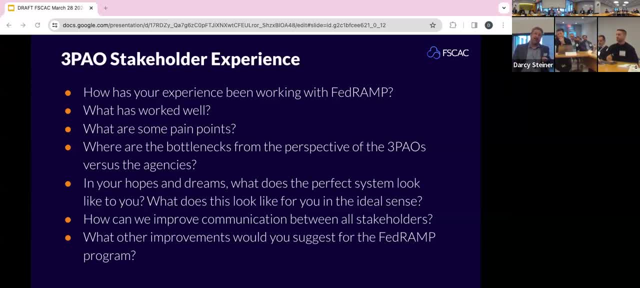 And if you need to pay a validation on that, then that becomes part of that element and you know directive that comes out of it And I mean jumping on that. any chatter, Yeah, I mean it's so people are starting to think about it. 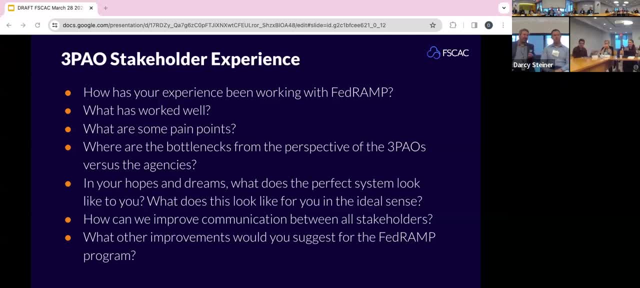 Absolutely. Yeah. Yeah, we some of our customers, we attest to so many of them, but it does a great job And that's that's one of the pluses of it is it allows for a lot of attestations for for smaller type things. 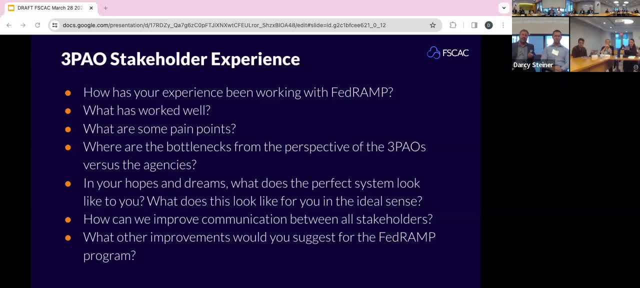 But we need to consider the emerging things, not just the things that have been around. Yeah, I think you know you're You know, I think you know, I think part of the reason that we're here, this is a discussion point that we've had with both CISA as well as OMB. 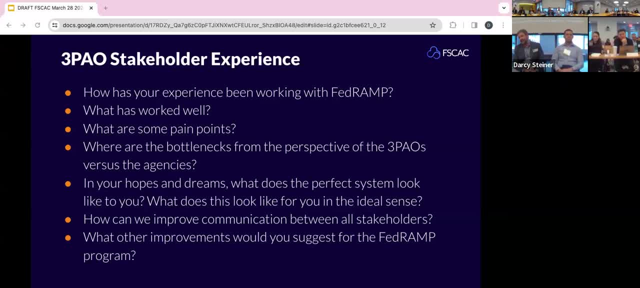 particularly associated with M's BODs and EDs and incorporation into the FedRAMP requirements, That part of the problem is that these BODs, EDs and M's themselves are not very clear in terms of who it applies to. 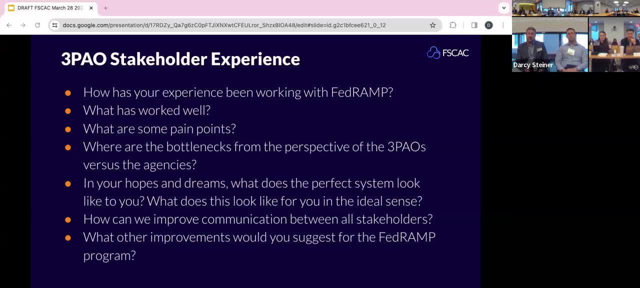 Right. Some requirements are at the system level, some are at the organizational level, some are at the CSP level, And so I think it's really important for us as a government, having a consistency in terms of applicability is super important. that way, then, it creates a direct line path for incorporation of a requirement into a FedRAMP baseline. 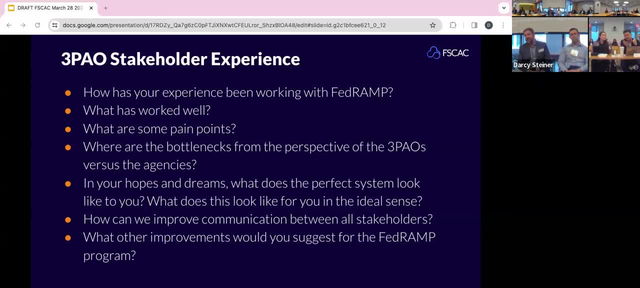 And I think part of the challenge where you might get one answer one day and another answer another day is because folks just don't know. Information exchange within the government still remains a problem today. You know, come on, I mean, you know, if you don't get the full story, you get, you get a piece of it. 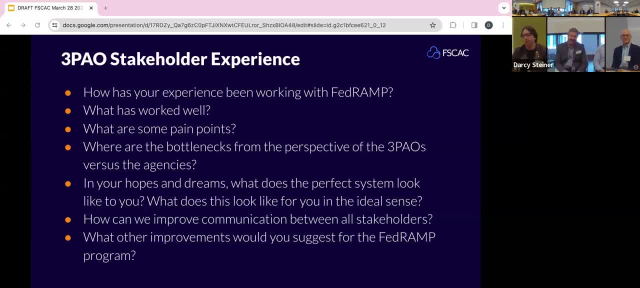 But the new version of Max will fix all of this. I think that's also a requirement from the GRC is the GRC we use today. I can put all of the BODs and M's and I can dissect it into the specific actions that our system owners have to have or our cloud service providers have to have. 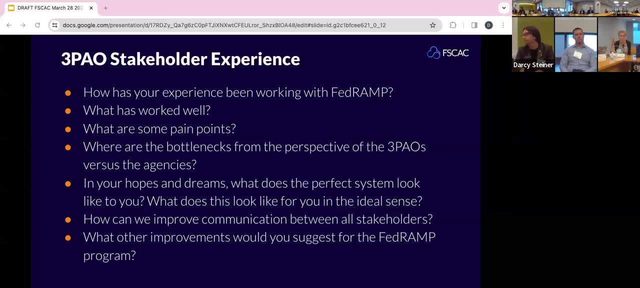 And so that's something we need to think about as we're developing our requirements for our GRC, so that I can publish something. If we go out to our cloud service providers, they can actually answer inside of the GRC. They can become part of validation. 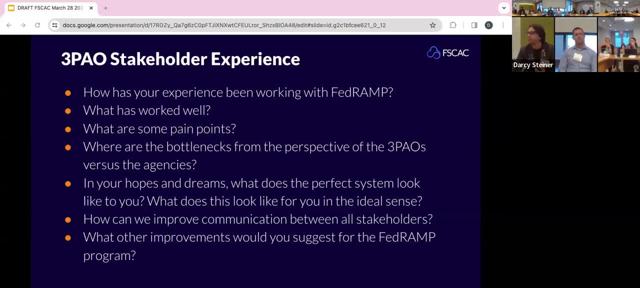 And so it's just a matter of how we incorporate those requirements on a quarterly basis or an annual assessment, that type of thing. But we've just got to figure out how we incorporate them into your point. I always take apart the EDIs and the BODs and then say, OK, now what of that is technical? 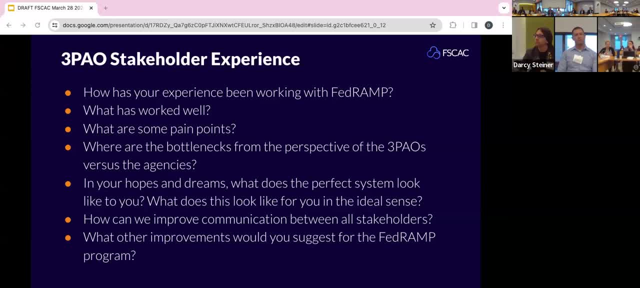 And how do I what's required here, as opposed to from an organizational perspective, And so that's. that's probably guidance we just need to share across the community. I think there's a lot of synergies between FedRAMP and DISA that we need to realize. 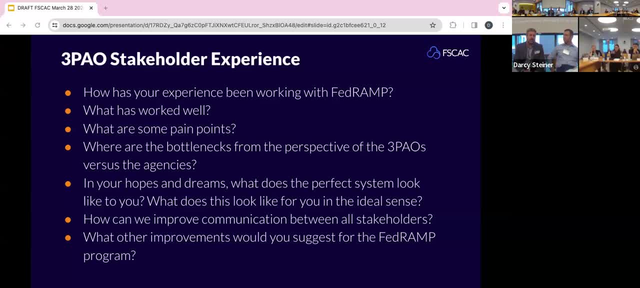 You know I've worked quite a bit in that field. I've worked quite a bit in that field bit on the DISA side, whether in the impact level assessments, you know where well, they're either going that, going that out first, or it's the federal first. I think there's some, some, some. 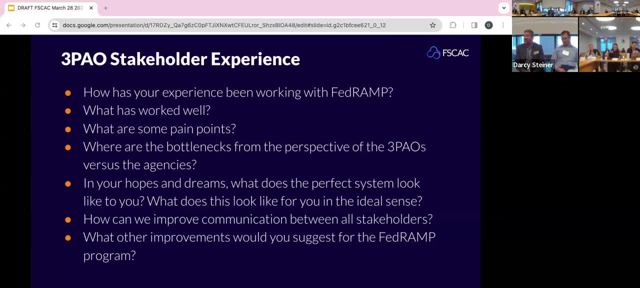 good things that we can, you know, help help each other out in terms of, you know, meeting the expectations for for both parties, knowing that, going in rather, you know, we can condense the process and make it better at the same time. Have you seen CSVs actively using like generative? 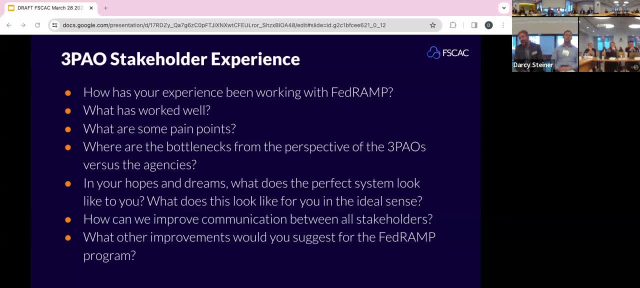 LLMs to facilitate the actual development or creation of their security plan responses: No, yeah, no, I haven't, honestly, And I don't know. I'm going to tell you that, unless they have a proprietary one that is local to their network, they're not going to because the 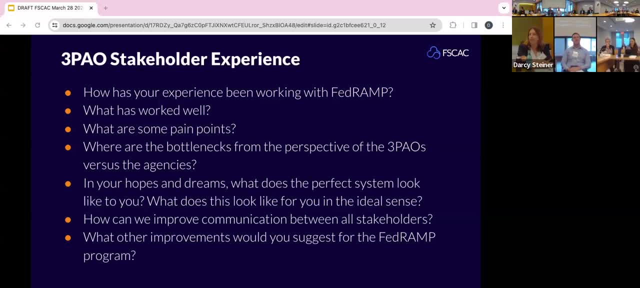 the intellectual property and it becoming a part of a larger model. So if they've got one that's for themselves, they would. It could work. Otherwise you snip it out pretty quick, but this is too general. There's no way, unless they don't want to feed their data into that engine. but they have to. 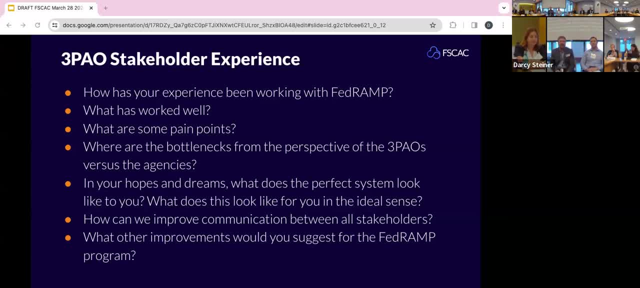 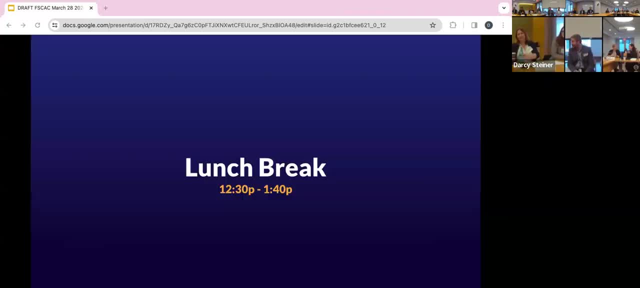 get their own, But that might be. that might be. that's good, right. We can't resist AI. We have to look to see how it can help us. We do probably need to go ahead and close for lunch, because there's not a lot of restaurants that have been like super close to the building, So I do want to. 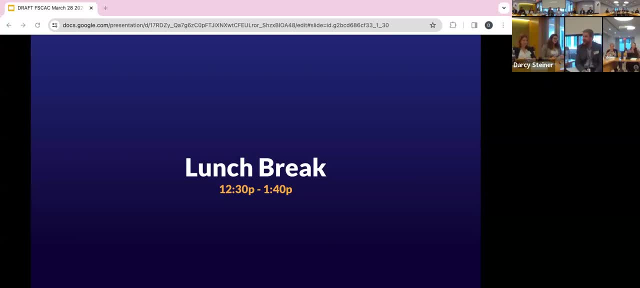 thank both Jen and me for joining us today. If you do, if we do have more questions, are you guys going to be free After after lunch? if you guys want to continue this discussion, we can have some more discussion after, after we're ready for lunch. 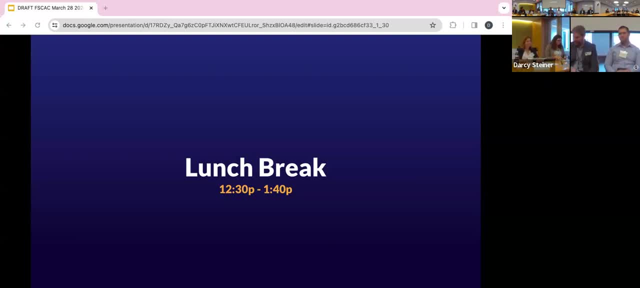 Yeah, sure, All right, great, We will be back. It's Gary. Yeah, We got this, But the soup works All right. That's what you want And we have to go on. I don't want to put you on. 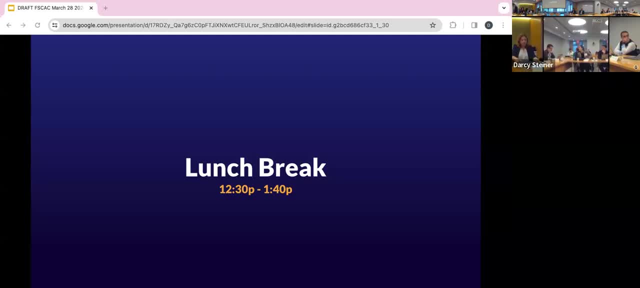 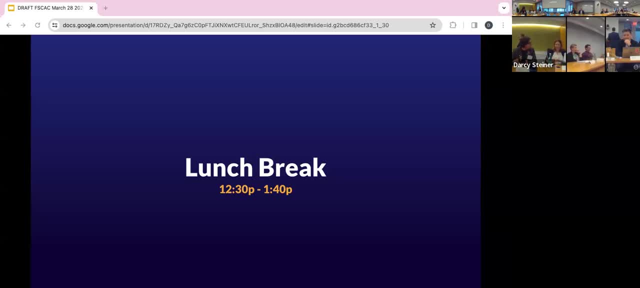 So definitely some home for you now, And then you can get online and find us Seeing it. Yeah, I got that. We're on the way to work. I'm cutting down today It's on travel. I'm So excited. 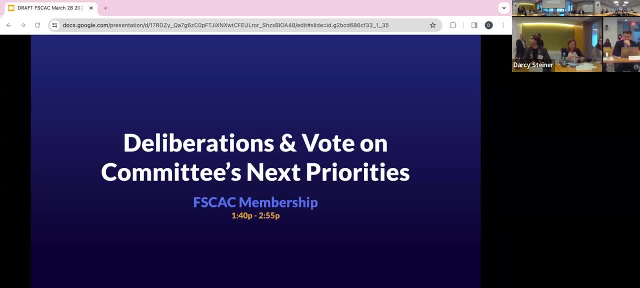 So he is like right back in the moment. I think there's wrong. You're here. If you get Yeah, See, we can go ahead and get started. We are, We already need, We got Yeah. I feel like I didn't predict that one, but I'm here. 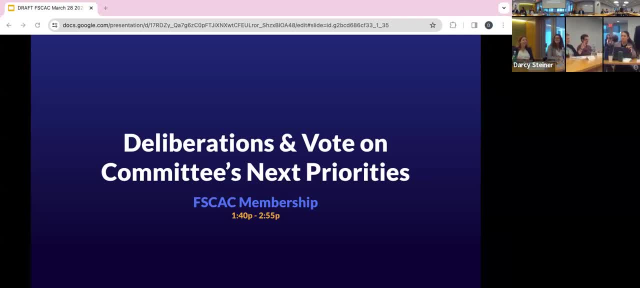 I feel like I came about Forms It's about. Then I started making a Four. That's actually I can't Answer place. welcome back everybody. um, do we want to have uh jim and lee come back to continue our discussion on the 3pao? 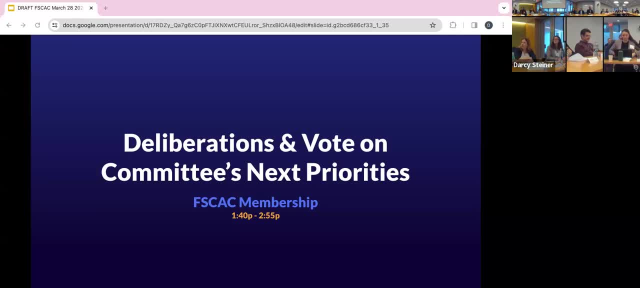 i know exactly. um, i don't see jim anymore. he just he just stepped out. oh, okay, um, do committee members? uh, do you have any more questions or engagement that you would like? i just was going to ask just a follow-on question, particularly relative to the last topic. 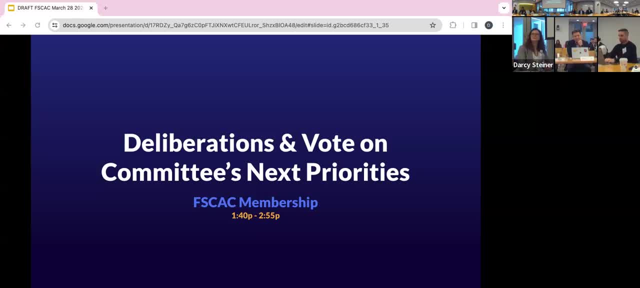 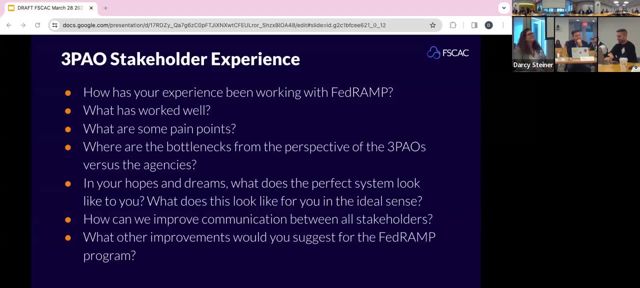 ai, please come on up and hopefully you can join us. sorry about the tight support, oh no, worries, all right, sorry to bring you up here, so just curious. you know, we're all like, uh, you know, talking ai at every meeting, it seems, and i think one of the consideration points that we have, that's been brought up in committee meetings. 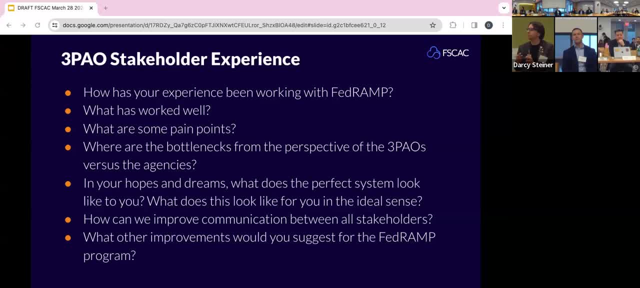 previously is: are the current set of people who mentored, with the corresponding set of risks associated with ai services? right, and i think you know some folks say, yeah, some folks they know i know this is doing a lot of work, particularly around the- uh, the ai rough map 2.0 to come up with some corresponding controls. so when you're 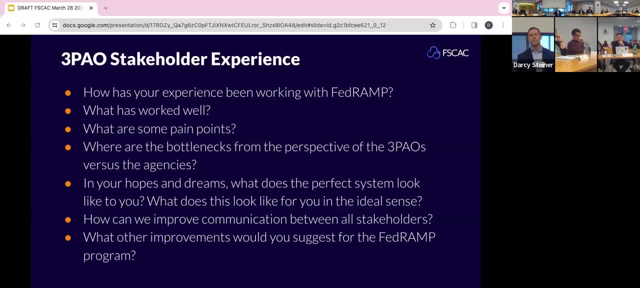 looking at this just experientially, right from uh three-part perspective, uh, i'm i'm interested in, like your views and what you guys are seeing on the ground, particularly when you're engaging in assessments, like, are the set of controls, are the set of assessment actions, you know, are they sufficiently robustly able to go through and provide confidence? 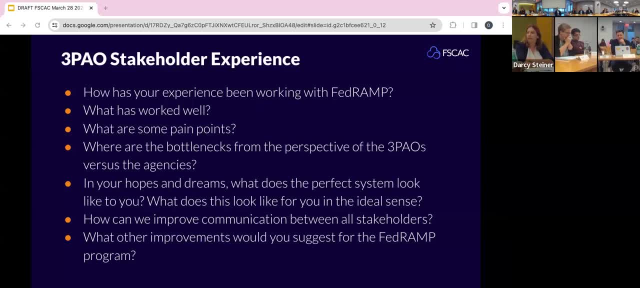 and then a fedramp authorized ai range screenrictors that all the actions are the same. can service provides adequate security using the existing base control set. Yeah, that's tough. I would say probably 75% of the way there. 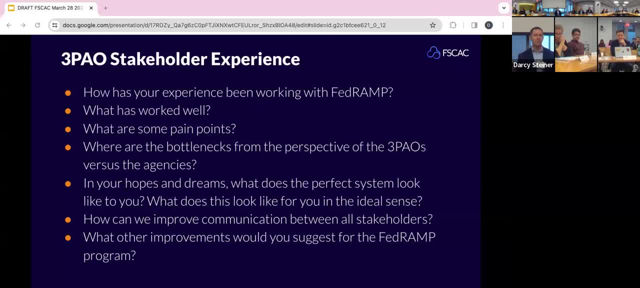 I don't think there's going to have to be a huge lot of changes in my perspective, Like the external services, I mean that's going to be an issue. So your CA3SA9 type controls, because there's going to be a lot of outsourcing of that technology. 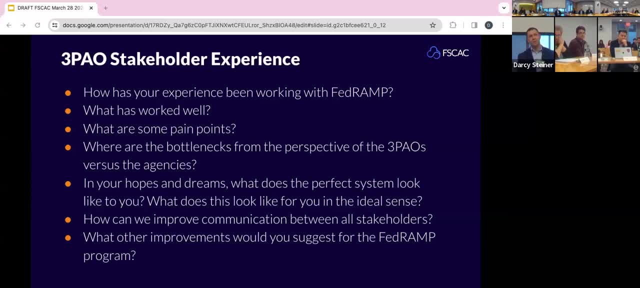 And how does the first person get authorized and not have external services type of situation, Like a chicken for the egg, is what I think of. So for that initial AI type CSB, I think they're going to get some special privileges. They're going to be able to get away with some things. 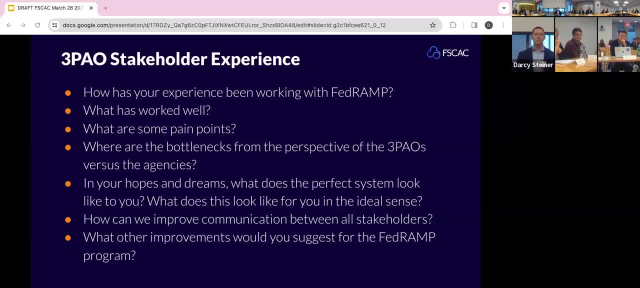 So build up to the next one, and the next one, and the next one. So that's kind of how I've thought about it is because this is uncharted waters, There's probably services used in the background for this AI that's not going to have a FedRAMP authorization. 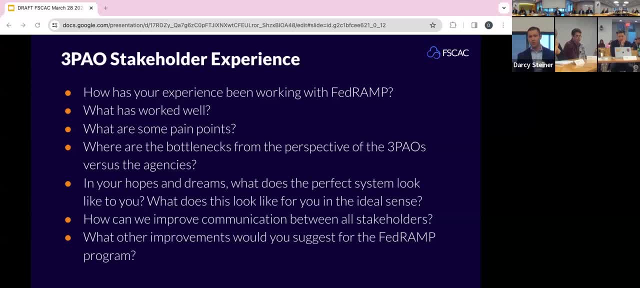 And, let's be honest, it's going to be processing federal data and metadata, Or it could be, because you can ask anything. How do you keep from inputting sensitive data and metadata into an AI type of platform? Have you guys played? 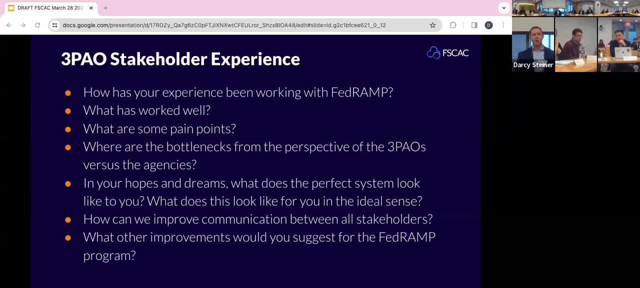 Both the advisory role as well as an assessment role. Primarily we do assessments. I would say one to two advisory roles a year. I prefer the assessment side of things just because I feel like we're more accustomed, the way we're set up, to do that type of work. 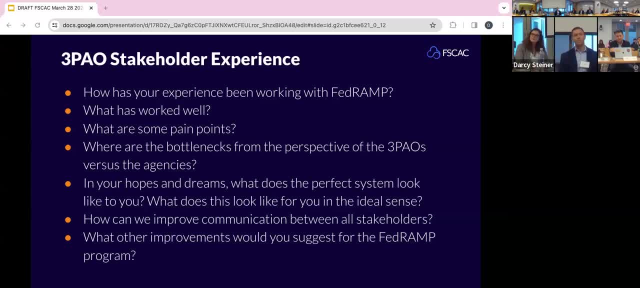 I appreciate that Absolutely. Any other questions for Lee? You had talked about guidance from the BMO around assessments And the assessments, Assessment expectations or evidence. that could be helpful. How often do you communicate back with the BMO And is there like a structured mechanism? 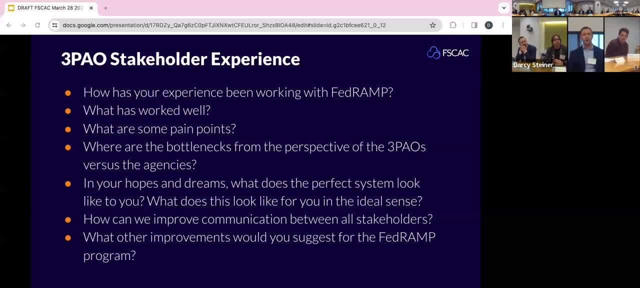 You know you guys have the monthly coffee, Yeah. So this exchange. I've been doing this for like nine years now, So I know all the reviewers, I know most. I have their cell phone numbers. I can call them and contact. 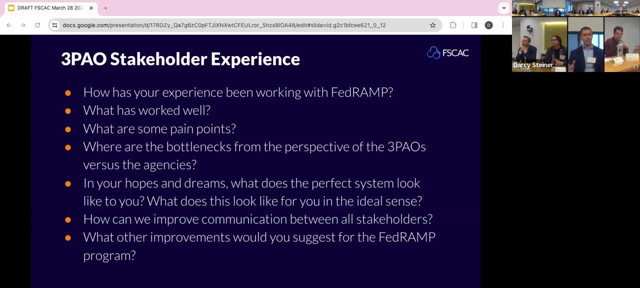 And that's from a personal Right. And that's where we have issues with clear, concise guidance. Because what about a new 3PO coming in? They don't have this type of relationship, So it's difficult for them, And it's difficult for new assessors coming in as well. 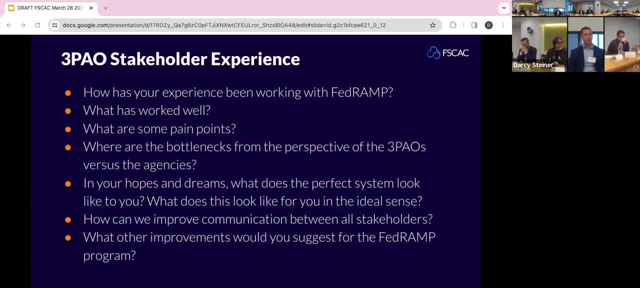 So there's obviously info app. You can send a question there. I mean, it used to take two to three days to get an answer, But they've drastically cut that down. I mean, I usually get an answer Same day now with fairly structured, good guidance. 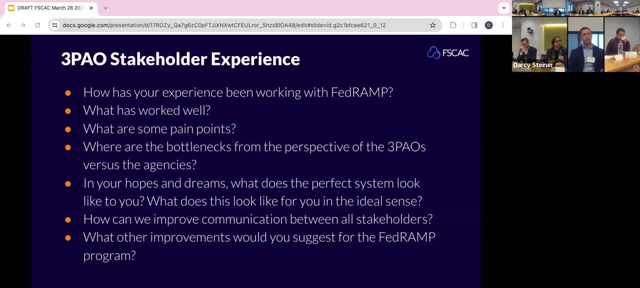 So anytime a CSP wants to see a response, I go to info app Because they're not going to want to see one of my- you know- backdoor conversations with one of the reviewers. They want it coming from a reliable, credible source. 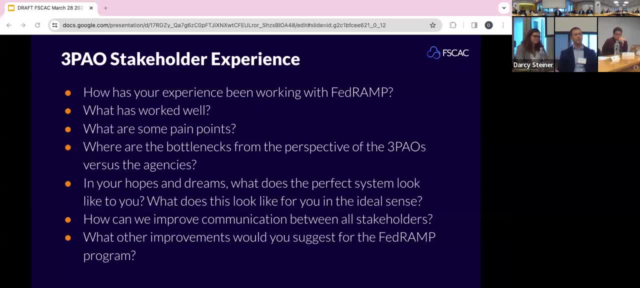 So that's kind of where again I think this- Can you get access to other assessors questions that come in as well? No, not really. Occasionally. they'll post some stuff On the FedRAMP website- I don't know, Marcy, if you remember the name of it- where there's like 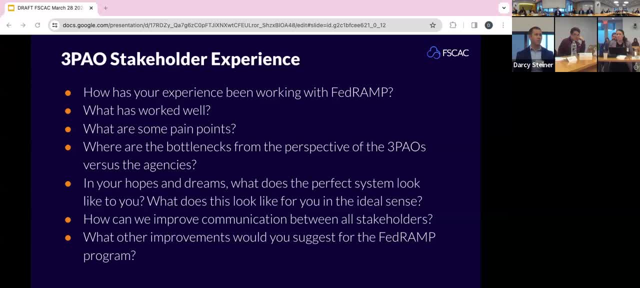 Tips and cues. Tips and cues- Yeah, that's what it is. So that is a resource. There's the blog posts. I mean, I think if you put one of those out every Friday, that's even a good start to one of the blog posts, to sharing some guidance. 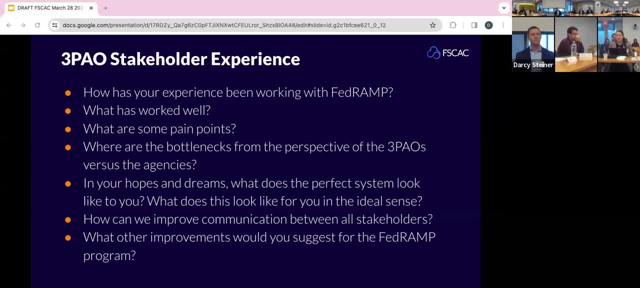 I have a question: Have you found that there's some, Particularly with the rep, five transition, kind of like cart before the horse scenarios with some of the things? And I think you mentioned it earlier- red team, the CAA- There was the requirement put in there and we saw so much panic from that. 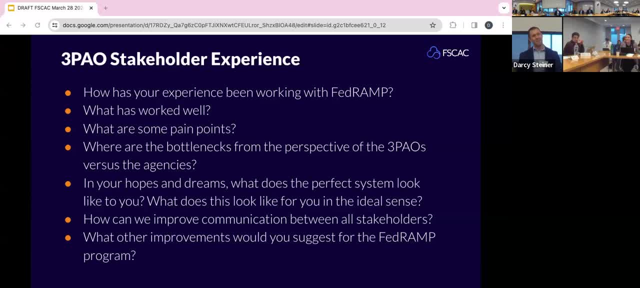 I can't even explain it. We're still getting it. So now everyone's saying, well, it's only draft guidance, I don't have to do it type of situation. So and that's what we ran into with the authorization boundary diagram guidance as well. 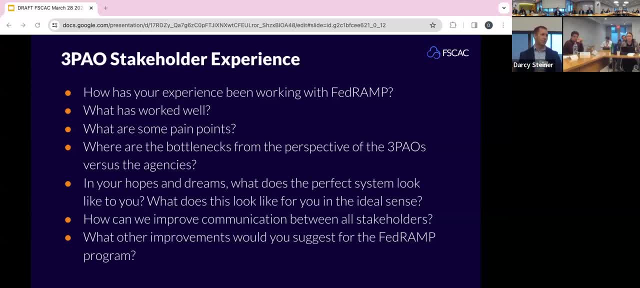 It was never really finalized. It was always in draft. So I don't have to follow That because it's not official. but we all know, as three POs and our relationship, that if it comes out in draft you're expected to fall. 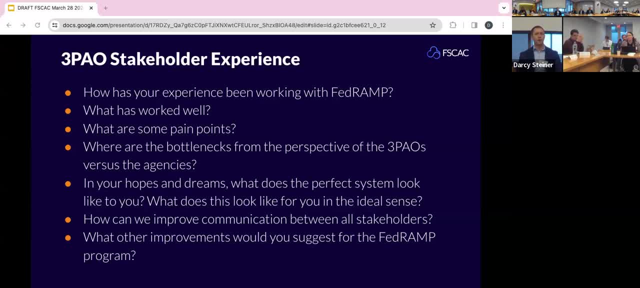 So that's, that's kind of an example there, but overall I thought the road five transition were very well as compared to the red floor transition. I think it was very well detailed. The website was set up- Perfect. I was surprised at how little questions I actually had from CSPs on: Hey, how do I get to rep five? 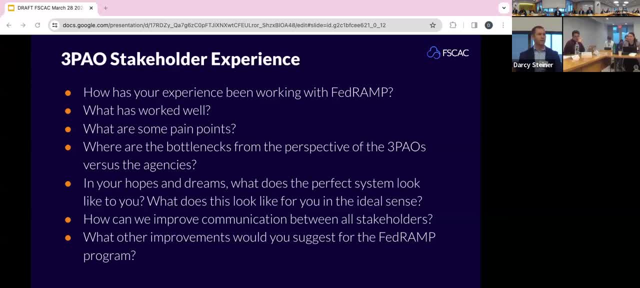 So I think there was a very good job done there. You mentioned, though I think, that the templates had not been updated like the SSP. So have have all of the templates been updated, and do is everything there to accompany red five? that's needed. 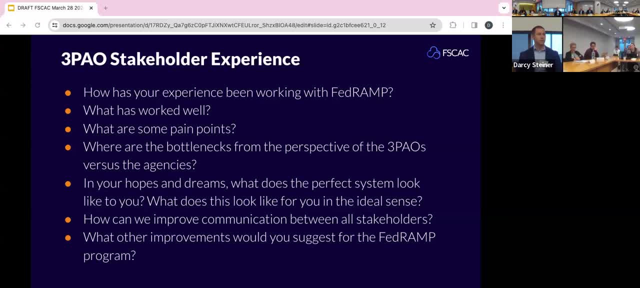 That might've been Jim. As far as I know, everything was good with the templates. We had a hand in helping with some of those as well. FedRAMP, which I love, reached out to us as three POs and said: Hey, what's you guys' thoughts and opinions. 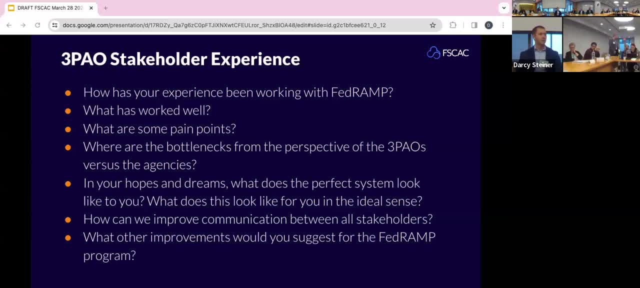 And would you help collaborate with us on creating these. And that's what we did, So that was very well done. Again, I'm the, I'm the ignorant person in the room. Red five, the 53 red five, Yeah. 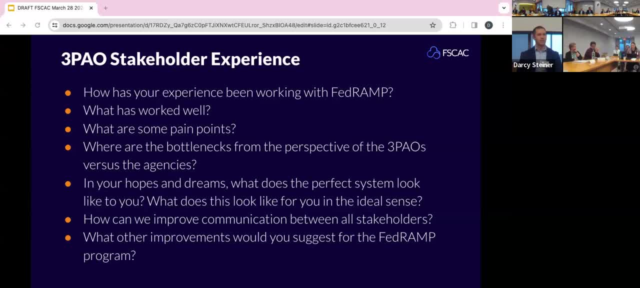 So going forward in the future- I'm not sure if nest and I don't want to speak for them- Um, we'll be doing like full rev updates to 53 rather than individual control changes in the catalogs going forward. So there is a very real future. 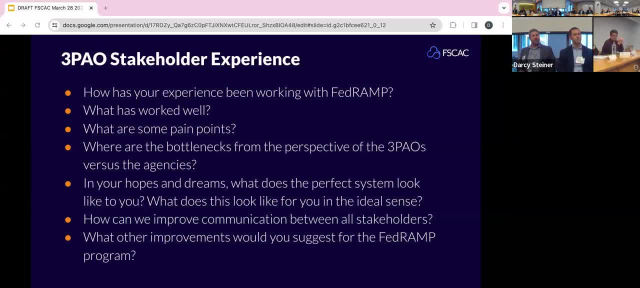 Okay, So there is a future of uh control updates absent of full rev roll doing what they belong. Interesting- Yeah, That's excellent It's, but it also changes the way that change is managed. this situation: Yeah, We'd probably have to address that, as Hey. is that going to be? here's the guidance during your next annual assessment. 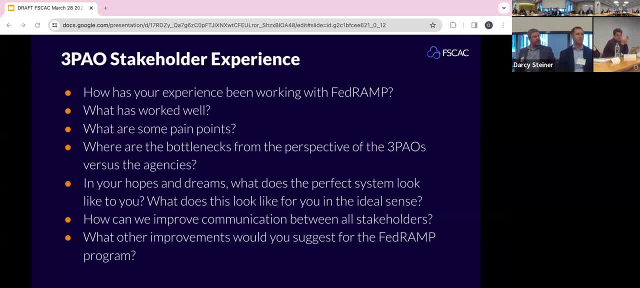 You have to review these controls, including in your documentation type of situation. I think that can work. I think, with everything else that you know, requirements are going to be emerging So we need to be able to address it in a more expedient fashion, and maybe annual was soon enough. 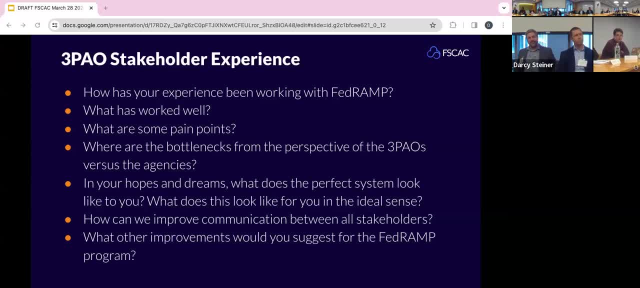 Maybe it's not, which is why the big red roll cycle was not adequate, but it's just the time to catch up. Yeah, Any other questions for the urgent? So uh, Now that we have more time, I just wanted to drill down uh more into. Jackie had a question about compliance with uh. says uh emergency director will buy an application record to any specific examples. 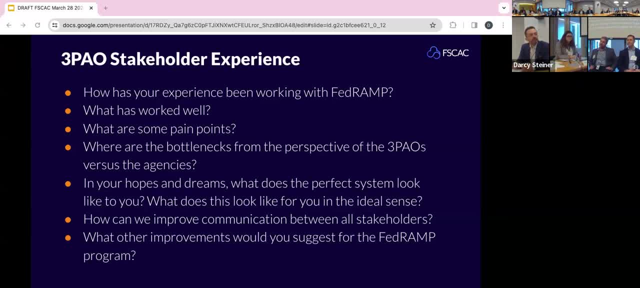 So I mean there are issues or pushbacks that you've received from CSPs that you ran into without naming any names that were specific to a bot or an emergency director. I would say for 1801, we always get the well, we don't really manage the email. 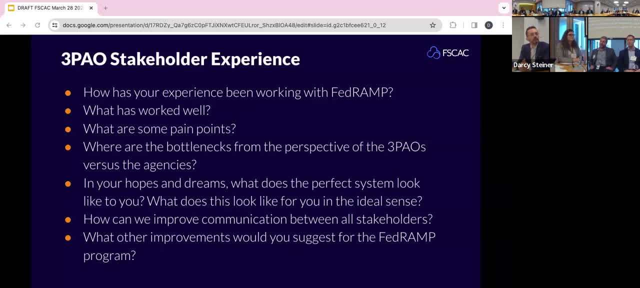 I would say for 1801, we always get the well. we don't really manage the email That's being sent on behalf of the government, So we should not be responsible for that DHS bot, but yet they're providing the avenue for it for the government. 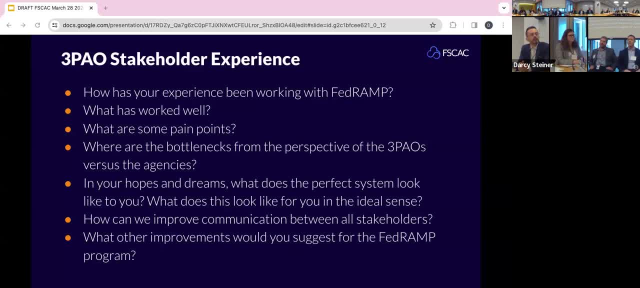 So, therefore, they should be responsible and they should have the technology in place. That's just one. Again, that's the big one that I always run into- is, you know, providing the spam protection for sending emails on behalf of the government? If you have any part in that in your cloud service, then you have to to abide by that. 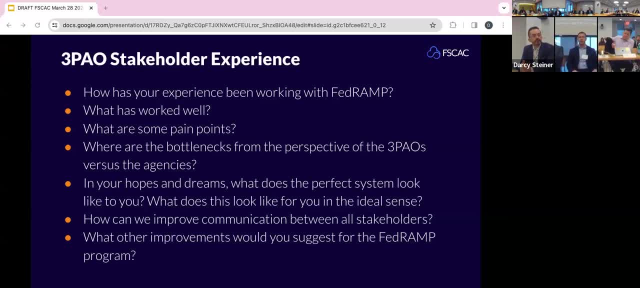 Your part. You're talking about the DMARC thing, the DMARC 01?? Yeah, the DMARC, I believe it's 1801.. Yeah, I don't have any specific examples, but I could see it very easily: the CSP challenging us: what's your authority? 3PAO- like we need some teeth behind it because we could enforce that, because it's which is a good question. 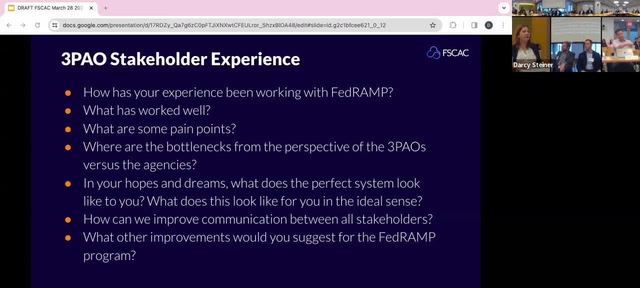 That's such an interesting example because, like they're asking: well, hey, why do I own this? If they were doing regular red teaming, they would understand exactly why they would abuse it and how. So, Like that kind of brings me back to the I think folks were talking about like adding, adding red teaming as a, as a control or attesting to having done red teaming. 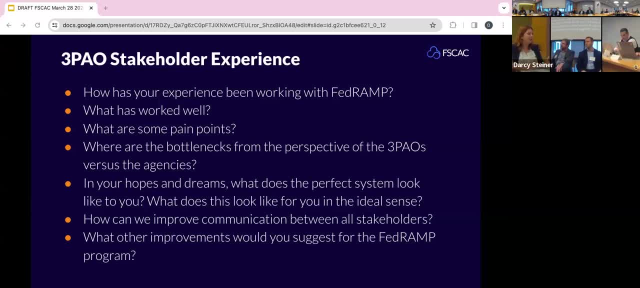 It just it seems like it emphasizes the importance of making companies develop that capacity. We're going to get some interesting results out of red teaming because it's- it's not a 3PAO required service. We can validate what the companies are doing. 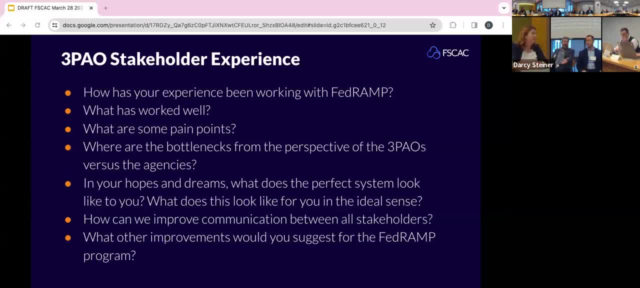 And so the guidance that came out was very timely, because we're in this. We needed that supporting guidance, because 3PAO is always questioned on the rigor that we're taking things and how we're interpreting it, And if we don't have that guidance to point to behind it, we get pushed around and bullied. in essence. 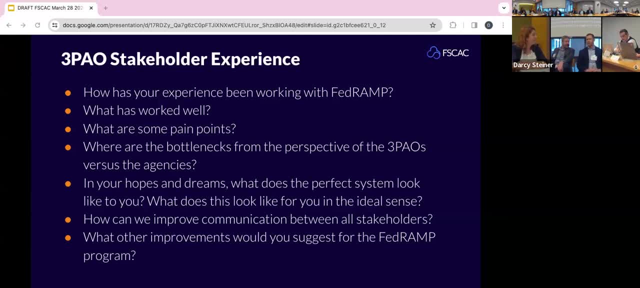 And that was a comment I left on the red team. The draft that was out there is. there needs to be some type of a structure to it, Otherwise you're going to have people underselling the red team exercise just to satisfy. where you know, a non 3PAO may be doing that for a $5,000. 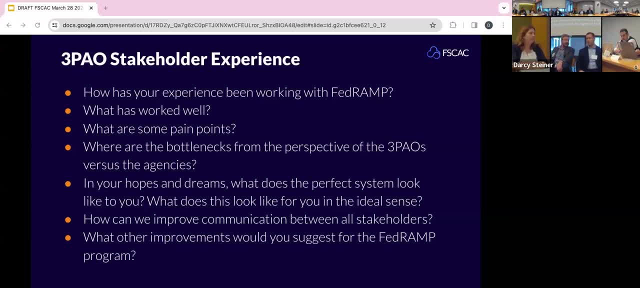 exercise. Well, there's no guidance to telling them that that's not sufficient, Whereas as a 3PAO we'll probably have a little more idea of what should be in it. We may sell it as a $50,000 engagement. 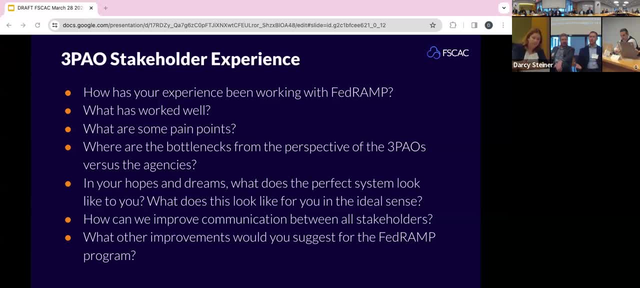 Well, that's a huge difference there. And then when I come in to do the assessment, I'm on the hook to validate that that red team exercise that said company did for a very low price that. how can I prove whether it was sufficient or not? but yet I have to sign off on. 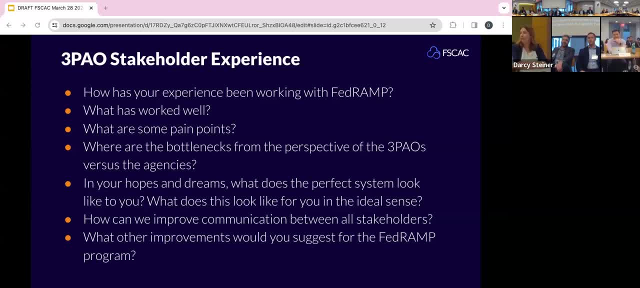 This harkens back to the first days where a web scan was rendered as a pen test. Yeah, So you really need to go through and find some of the rules of the road or some of the basic guidelines around what constitutes a red team. 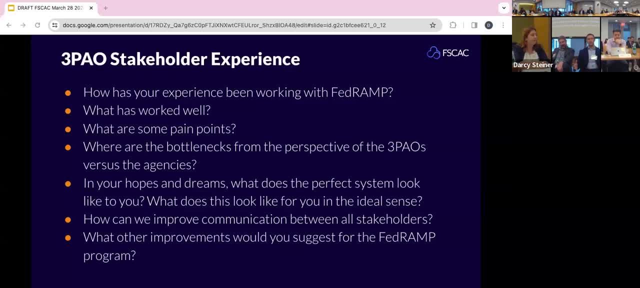 Absolutely. I mean, I like to, I like to leave things open and, you know, have ingenuity, but at the same sense, if you're just there's people out there that just want to check the box. they don't care about security. 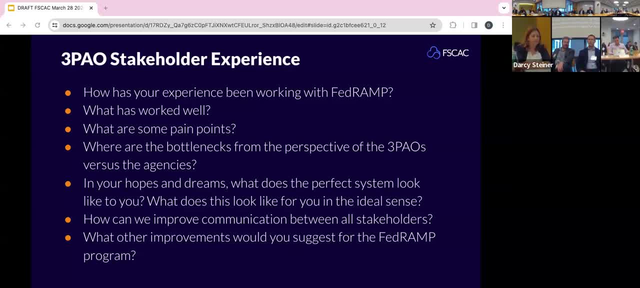 Unfortunately, that's where we are And that's what scares Me. controls, assessment isn't so much, but when you get into to rent, teaming, penetration, testing in general, it's not about what we're done, It's about: did we run out of time, right? 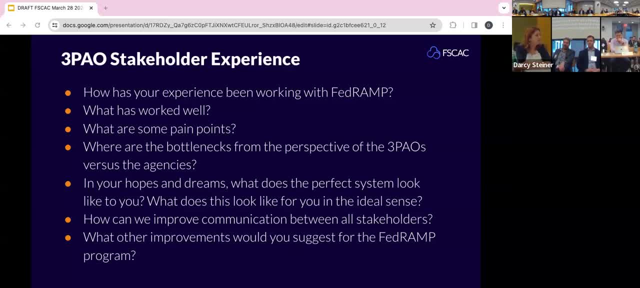 Because the pen testers never want to stop. you know they they constantly dig and then, but they have to, they have to pull back at some point and say: all right, this is what we got, And then they pick up next year. 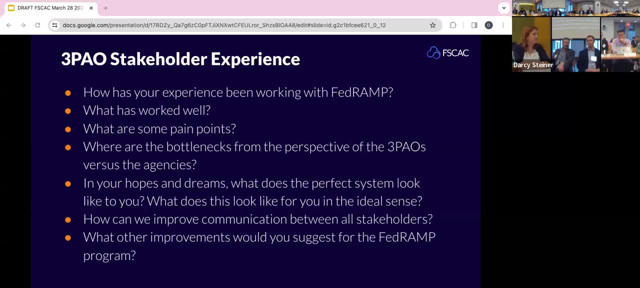 Right, So it's, and that's what's, that's a benefit of you know continuing, you know consistent three PAOs is you bring back to people. We take our lessons learned and applied in the penetration testing exercise. 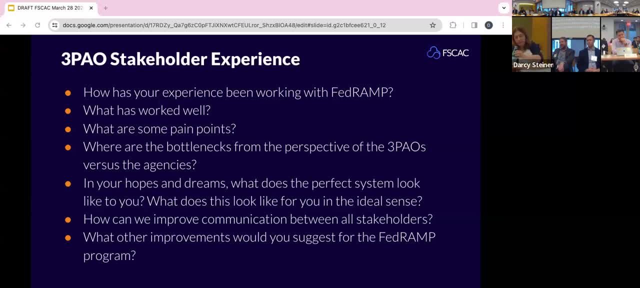 Is are, are really the the most valuable in terms of identifying things that you don't know. that could be the next thing that gets you know you a headline right, That's, we find some critical and valuable information to correct system security within those engagements, as opposed to the control assessment, which relies on an operational process that it was carried out. 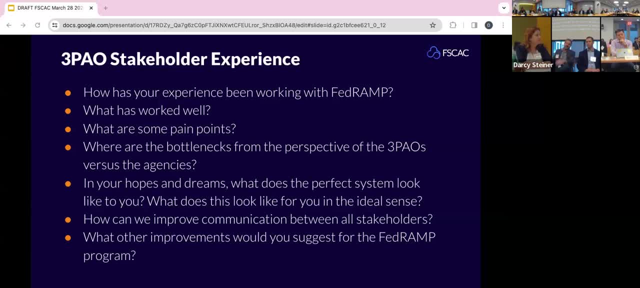 It was documented right. It should have been followed, but somebody didn't And and that's I don't know, I can't remember exactly. Yeah, And that's just part of it. It's, that's just part of it. 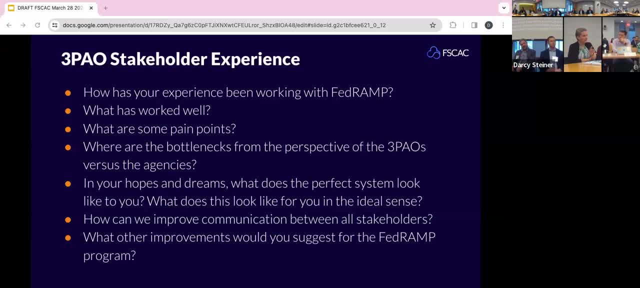 In terms of internal data that they think might be an internal ticket, or Why? because, right Just to to your point, I really think that that's part of this guidance that we need to look at because I've been getting lately. well, the pen tests said it was external and it didn't have this and it didn't have that. 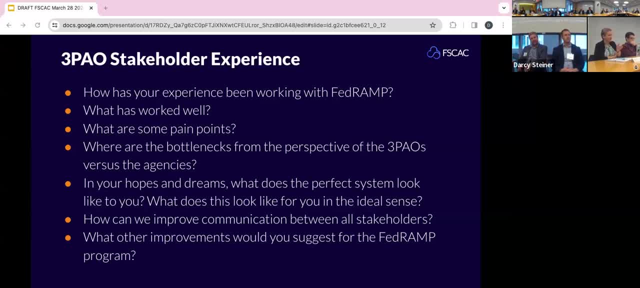 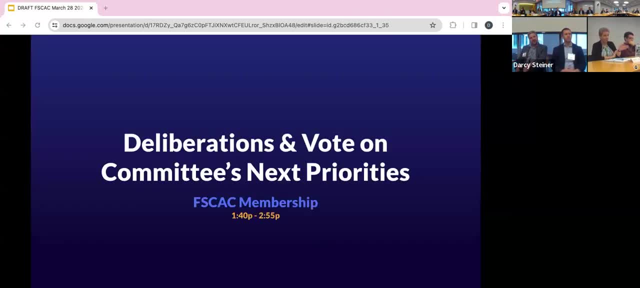 And I'm thinking, you know, shouldn't this be an internal pen test? Should we not assume reach? you know, should we be ranking for? you know good places for lateral movement should be executing, and whether different three PAOs do something different. you know, I don't. 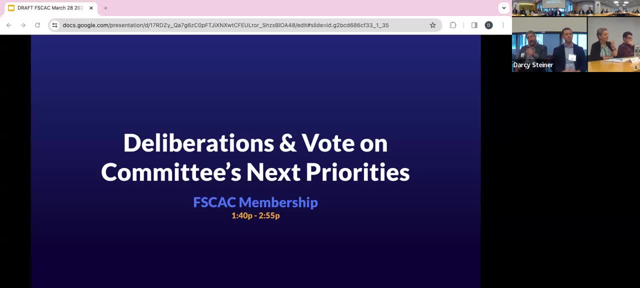 know, but it's an interesting question and what I see really varies vastly depending on which three PAO actually does the test. There's going to be a disparity between, because we develop our own methodology. Yeah, and I would like to remind the committee that we only are flying to 255 today. 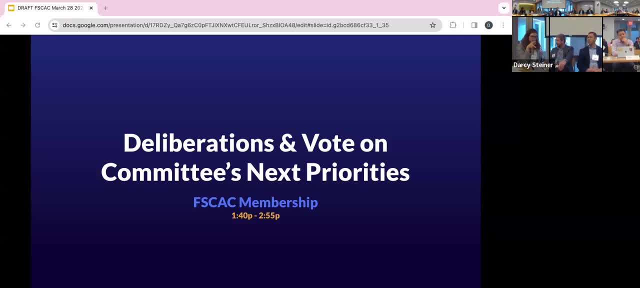 so we have just about an hour left to do our deliberations and discuss what we would like to work on for the upcoming year. We can keep going with Lee and Jim if you prefer, or we can move into the deliberations. Can I make one more comment? I'm going to go over to Bronco, to your 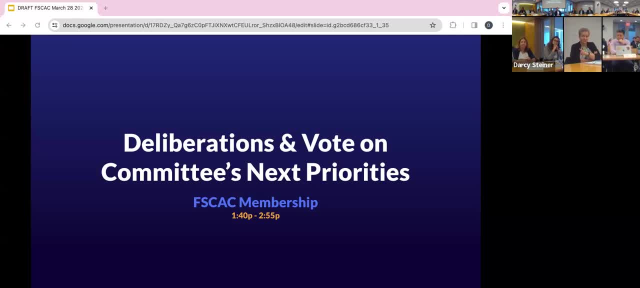 question to them, which is on the side of the box and it sounded like, from what you all indicated, the only one y'all actually really look at is the 1801.. Oh, that's fair for me. Yeah, and so you know. that's where I think we need to get guidance out and how we actually 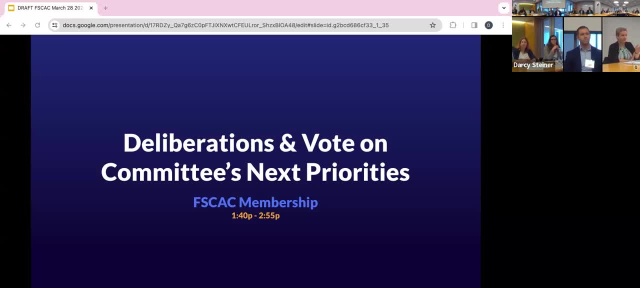 address current FODs and current activities and emerging requirements. and you know, just tell Marcia, does the AO issue the authorization to cloud providers? Is it their responsibility to go out? Is it FedRAMP to all the cloud providers on the marketplace? You know how do we track. 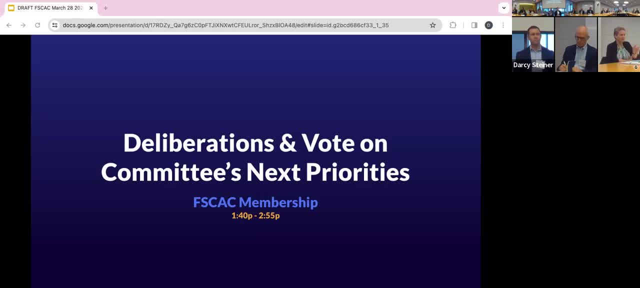 the compliance You know. so I think that's an area we really need to wrap our arms around with APTs out there. It is a really significant issue to get after with our cloud providers. They're part of our infrastructure, part of our day-to-day business now and we really need to make sure. 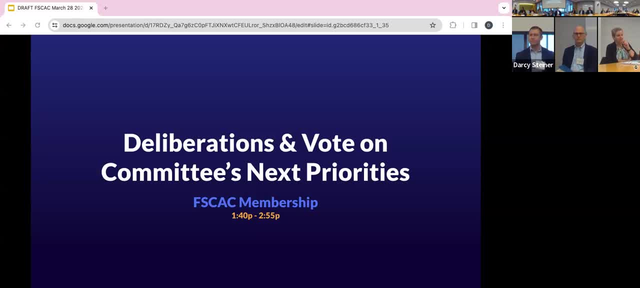 they're taking care of emerging requirements. They don't necessarily have the information about the threats that we do and we just need to get that stuff out. And I agree- and again, we worked with FedRAMP in the past to provide some guidance, but clearly we need more. 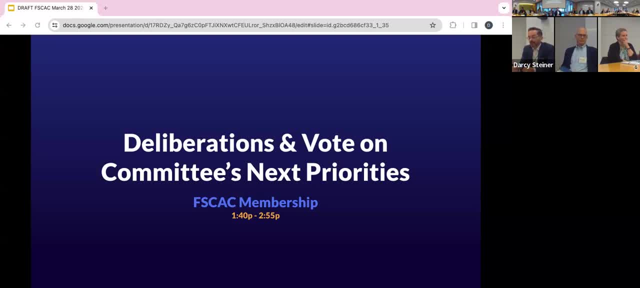 and now I need to comment that my question was somewhat loaded. There's also a question of authorities, because obviously our directives, we only have authorities over federal civilian executive branch. We can't direct cloud providers what to do. and then there's also applicability. 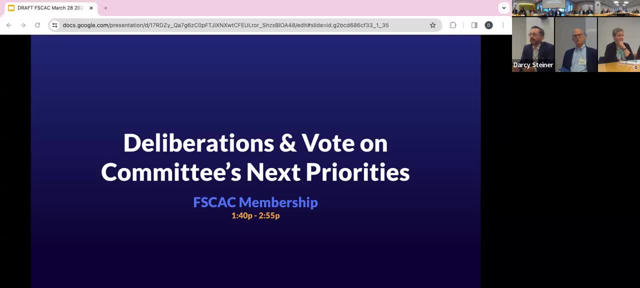 Unfortunately we can't. and then there's the applicability issue, where FODs and emergency directives apply to federal information systems only. and where's that boundary now that that one's passed? That's not an easy, that's not clear, straightforward answer, but we definitely need to work on that. 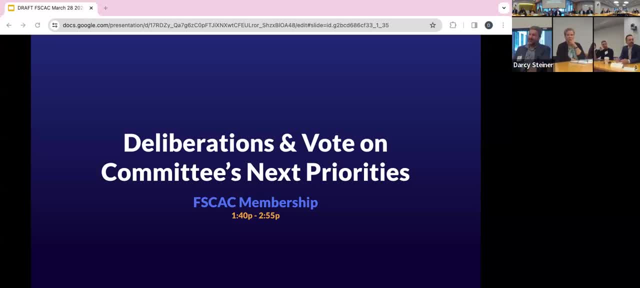 It tracks with how it's viewed and the resistance that we've received. And again, being someone who co-authored most of those directives, I've been intimately involved not just in developing them but also working on the deployment side and both the deployment agency, So it's not an easy thing. 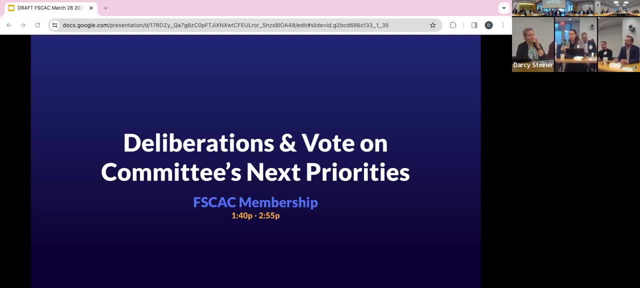 because we, obviously you guys have the same thing, as if we have a vulnerability disclosure program right, and so we have, you know, currently hackers that attempt to compromise our public facing websites, and so those are directive actions to that. we're actually penetrating the cloud providers and the hackers report in the vulnerabilities that they find and we are tracking those to. 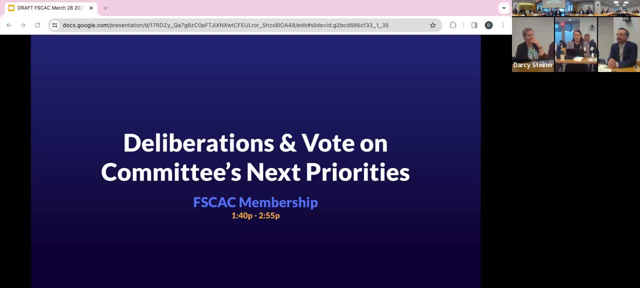 closure and there's no question of authority, you know. so you know, in this whole space, we've really got to figure out that we're partners and how we approach securing all of our infrastructure. yeah, i guess i was just going to add. there's probably two nuances to one is from a cloud. 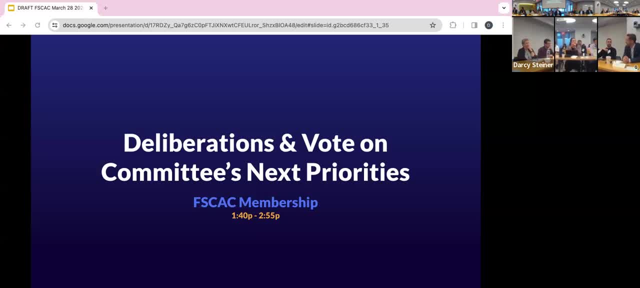 service provider's infrastructure specifically right is. that's what we're focused on, and then there's your actual efficient workloads running on our infrastructure. so you're going to have like a kind of a bifurcation there. the other one is how fast, late, like what's your? 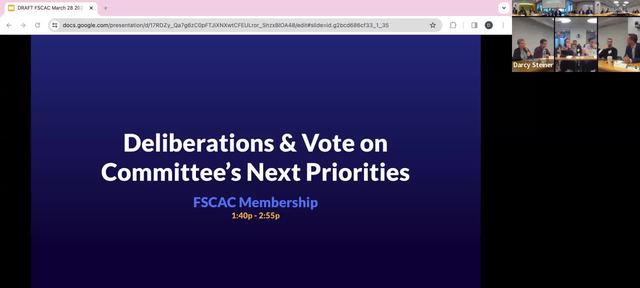 what of of this vulnerability is going to be a big question mark, Similar to like the. it's like 30,, 60,, 90. Or are we looking at a year? That's why I'm saying, with APTs, it's today. 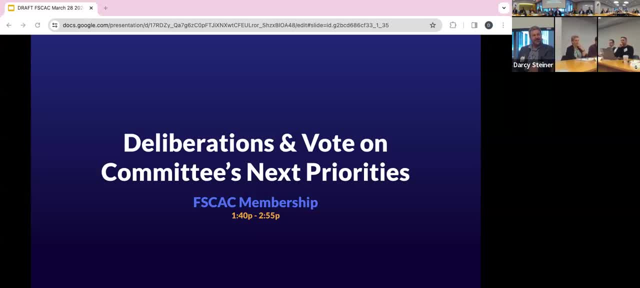 And that's the one I'm really concerned about. It's more than the CDGs that we're picking up on standards. It's the. we have an immediate threat and we need to close this gap. And so it really is about the mission systems. 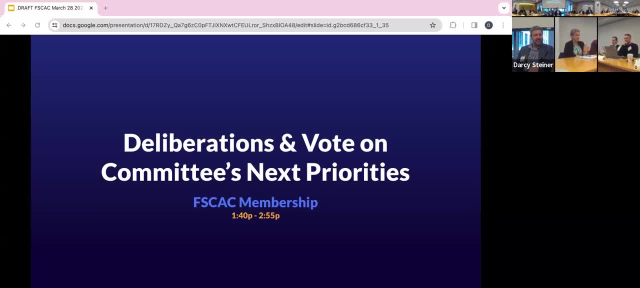 And we tackle that side even in, but also those that are on the cloud infrastructure side of the house. Yeah, I think there's a lot we could do to share. Yeah, What a good transition, Thank you, Thank you both for your insight today. 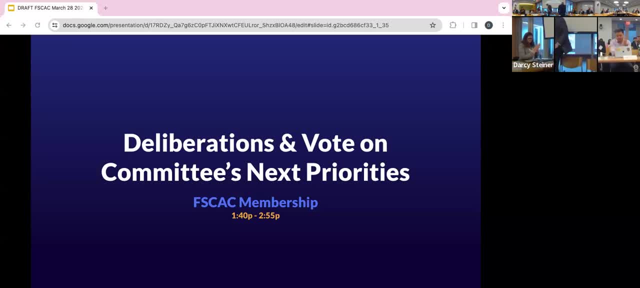 Yes, thank you so much For sure. I would like to now invite the committee to begin their discussion And deliberation to determine the next priority or priorities you would like to work on. If you're ready today to vote, we can also do that. 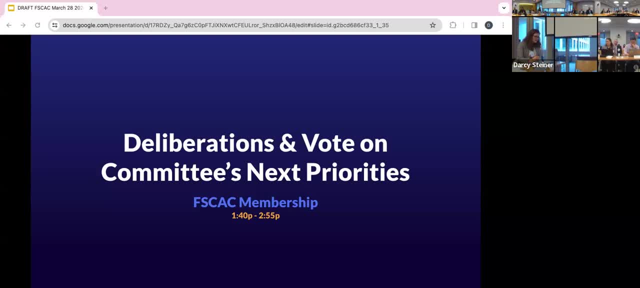 One more note. if the committee cannot decide what they would like to work on this year or feels that they need additional presentations or information to proceed, we can still hold a vote today, But the vote can be, for example, to delay determining the committee's next priorities. 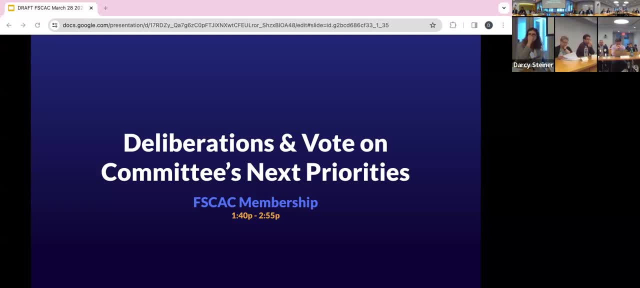 until the next steps are achieved. Are there any questions? All right, great As always. please remember to restate your name prior to speaking to ensure that those on the webcast and the people reading the minutes will know who is making what comment. 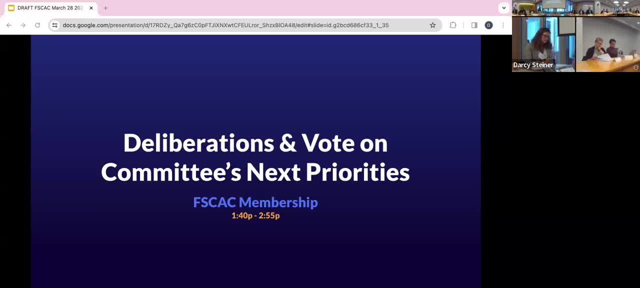 With that, I will now open the floor to members to deliberate what they believe is the most important priority the committee should be working on. Anne, would you like to start us off with your thoughts? Thanks, Michelle. I just wanted to say thank you to all of our speakers. 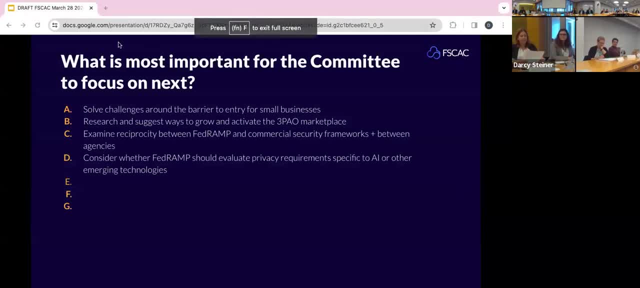 and presenters today for sharing A lot of great information and then teeing up a lot of great discussions. Based on these presentations and what I've heard from the group so far, I think there are a couple of priorities this committee could consider. 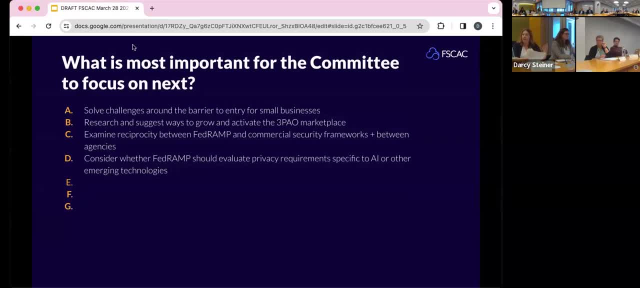 And of course we're open to whatever the committee comes up with here. But just to get the discussion started, it seems like one big theme is how can we help FedRAMP solve challenges around barrier entry, specifically for small businesses? So we've heard about cost authorization timelines just. 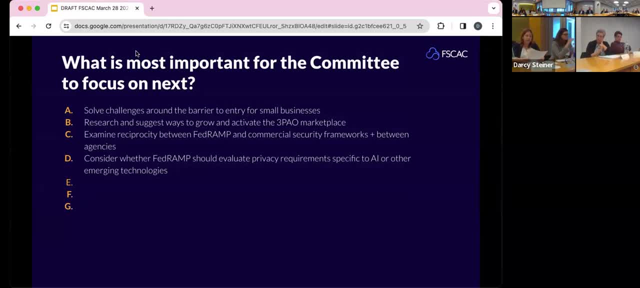 this. We've also heard that there's a lot of tasks made of small businesses at different levels of maturity. That could be a whole category. We could also talk more about the discussion that we just had about what are some ways to grow and activate. 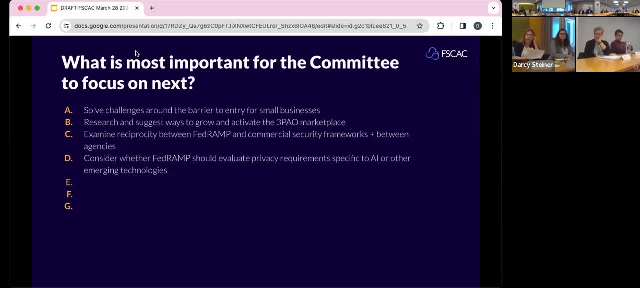 the 3PO marketplace. So we've heard from some 3PO's. You all have had experiences working with 3PO's. We know that the marketplace is about 40 companies, 10 of which handle about 80% of the business. 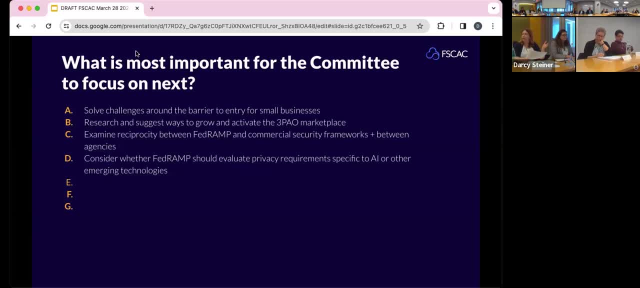 We know that the ecosystem, especially for SaaS products, is about 50% of the business, And so the FedRAMP program is going to be scaling up in a variety of ways to meet the demand from the marketplace and also agency needs. 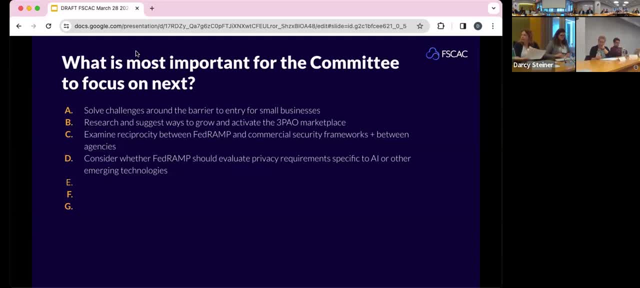 How, if any anyway, does the 3PO ecosystem need to evolve And are there ways the FedRAMP program can be more directly supporting them, strategically engaging with them, as folks have mentioned? So it's a second priority area. 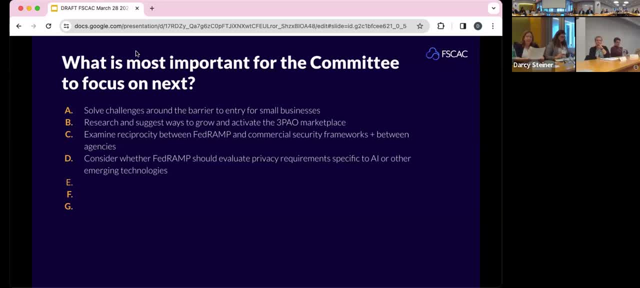 A third priority area that's come up a lot is doing a deep dive into reciprocity Between FedRAMP and commercial security frameworks, potentially also between agencies, combination of these, And if there are specific types of companies or authorization levels that would benefit from prototyping reciprocity. 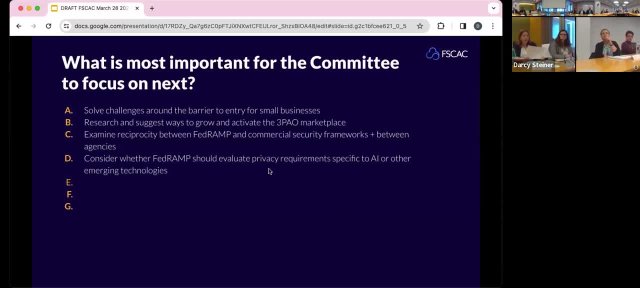 frameworks, for example? And a fourth area that's come up is: should the FedRAMP team evaluate privacy requirements specific to generative AI and other emerging technologies? Bo brought up a couple examples. We've talked about this a little bit. The space is moving very quickly here. 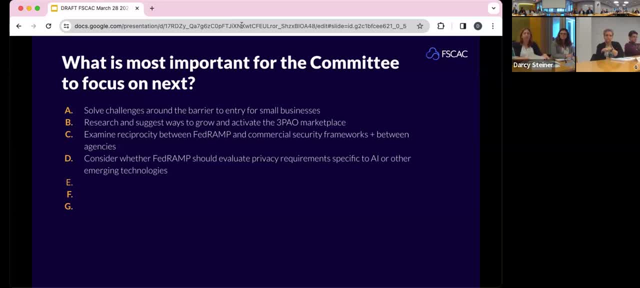 So I think this conversation will be less about specific point in time benchmarks and more about how do we evolve our government and FedRAMP idea of threat model to accommodate the idea of how generative AI, large language models, other kinds of emerging technologies? 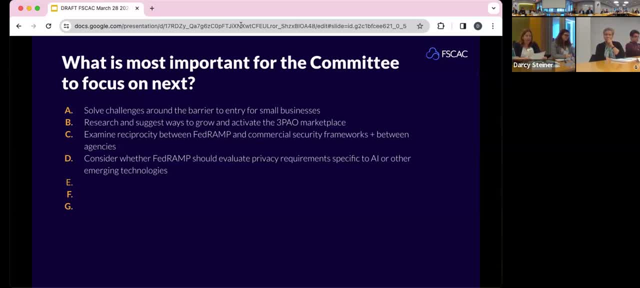 affect how we think about data privacy and security boundaries. So I think any of these Areas are probably media enough for us to spend a lot of meaningful time on. Maybe there's a combination of them that resonates with this group. Maybe there are other prairie areas as well. 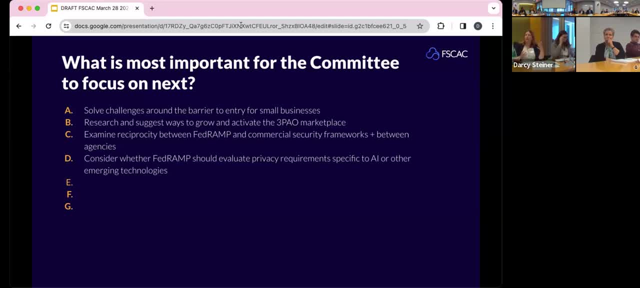 I think we saw from the last year's worth of engagement that we were able to tackle some substantial topics and provide feedback that was meaningful and actionable to the FedRAMP team. So I think we have the opportunity to do that again, But also learning from the prioritization conversations. 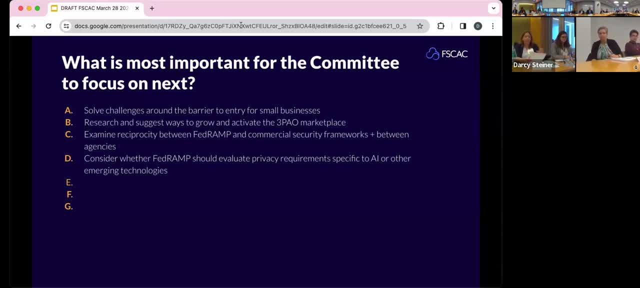 we've had in the past. I think we do need to focus to be able to make the best use of this committee's time. Thank you, Thank you. So I can get into more details here, But I'd just love to just pause there and hear. 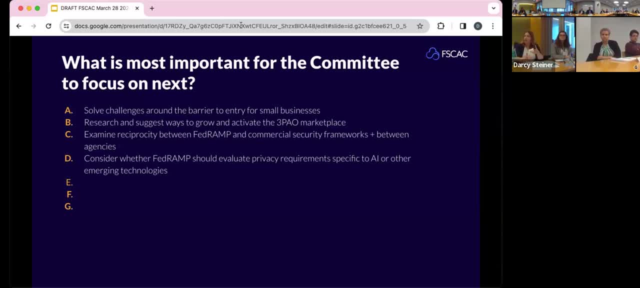 whether any of those areas or a combination thereof or other areas, are resonating with this group as priorities. You don't mind me starting So some of these areas. I'm not sure they should be our priorities. They should be the drivers behind what we do. 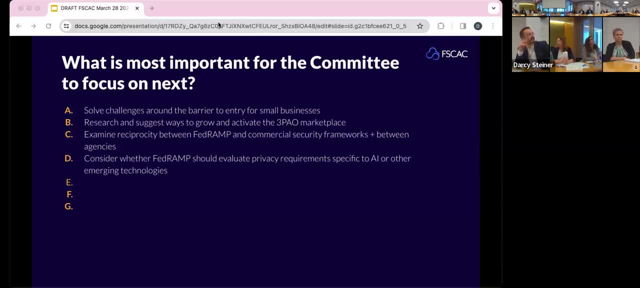 But there's an S in FISCAC or security, And I think security should be our priority. And again, this comes from the agency I work for And also that's one of the priorities for the FedRAMP: security of cloud offerings. 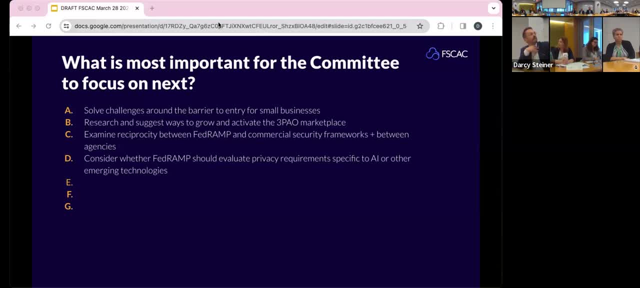 So I think that needs to be out of focus. So as we think about potential priorities, I just want us to refocus and think about security as a response. I'm I obviously come at it more from hey, so I understand. 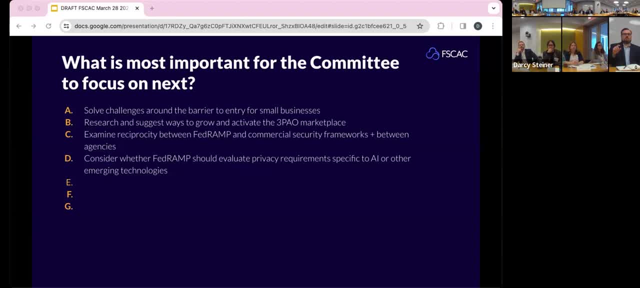 The one thing I wanted to point out relative to security is there's security for the things we buy, which, of course, is not my lane, And I obviously agree with everything you're saying. I think there's also modernizing unsecure old things. that also 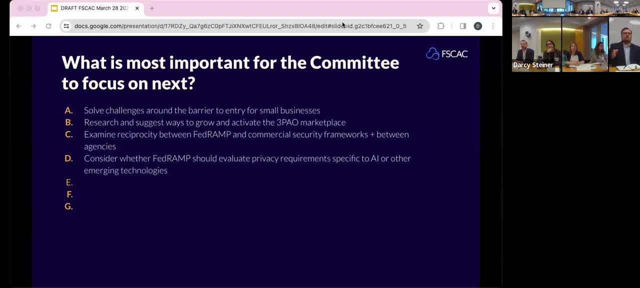 has a security which is less about meaning there's still some balance towards the perfectly secure product that you buy and something better than what you have, And it's very challenging. It's very challenging for agencies that are asked to do both things. It's a balance, is my point. 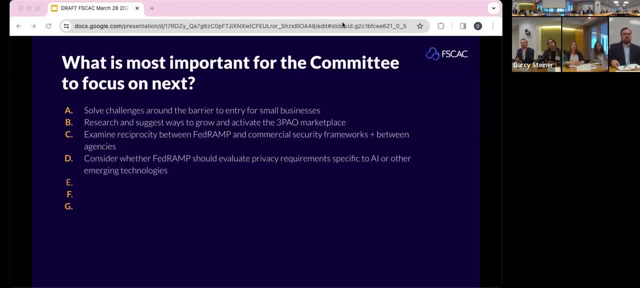 And I think it should be. the focus of this is security, but that we look at the process by which we bring those new things in and the timeline for those things and how insecure something may be while that's going on, balanced out with just very specific 853 controls. 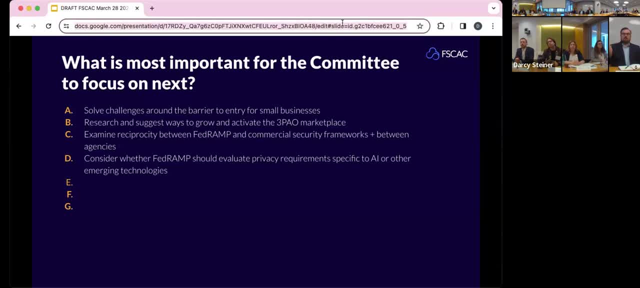 and all of that stuff. So I think they're both security focuses. I guess my point. I would argue that A to some extent they're both security. I would argue that B to some extent feeds into a security discussion as well. at least, 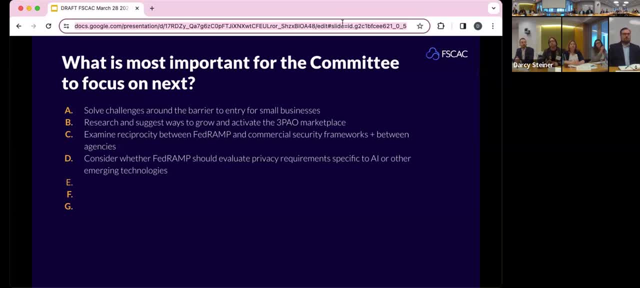 from the agency. My perspective would be that doing both is maybe, And I think A supports everything we do. We definitely have everything With security in mind. we have to make sure that we don't create barriers for entry, And then obviously it just has a cost to it. 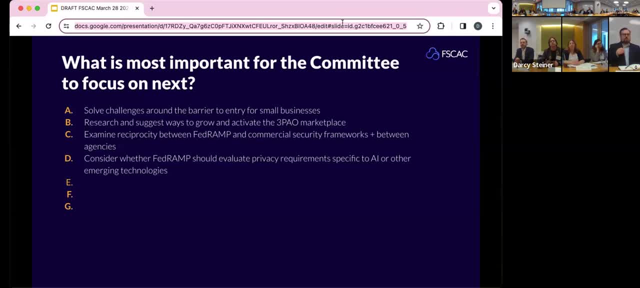 It makes that much harder from a budgetary standpoint for me, who has to pay for it and then to talk a vendor into actually go And there's some risk, as we've seen with the consulting and the consolidation of many small companies into a few large companies over the last- excuse me- 10 years. 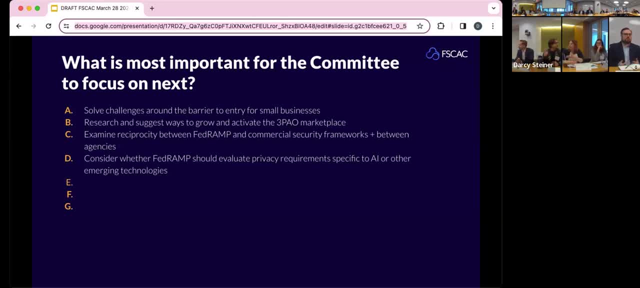 So, anyway, balance points Bill, and then Mike. I also have security in my agency's name, But my perspective is a little different on this one. I concur with the obviously small businesses. I think that that is the key. 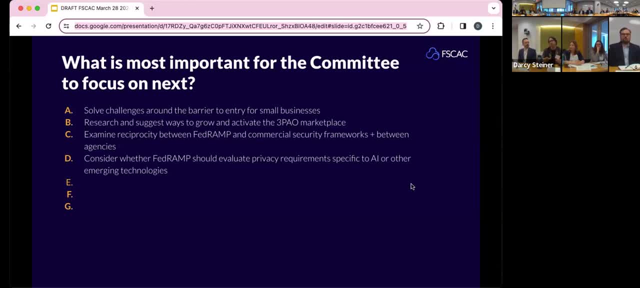 I mean small businesses- is a way that hackers can get in. That is a clear point. It's a clear thing. That being said, I feel like a lot of the discussion we've had around small business, a lot of those levers. 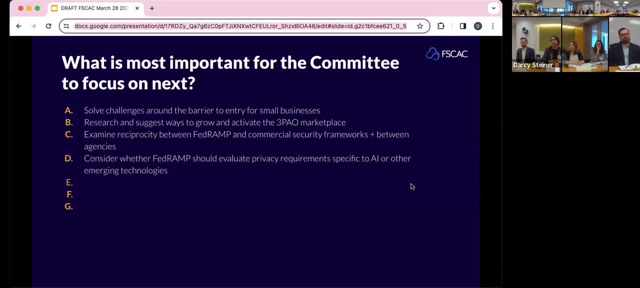 that we are concerned about might not necessarily be in the FedRAMP box, And a lot of that seems to be in some of the other boxes- not to put SBA on the spot- or will be on the spot, But I think there's a lot of other things. 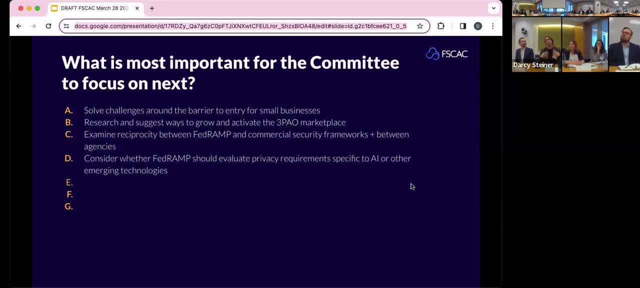 in there that go into it. I'm much more concerned personally. I'm in a small agency now, So my concerns have shifted pretty much 180 from where they used to be. And when we're looking towards D and broadening to the conversation, 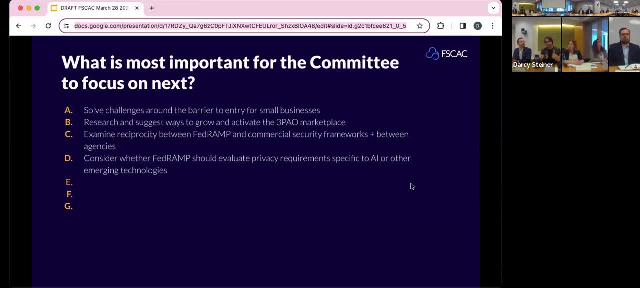 We're having about the bods. My biggest concern at the end of the day, sitting in a small agency, is: I got all this stuff. OMB is throwing all these unfunded mandates at me. I don't have the resources to keep up with this. 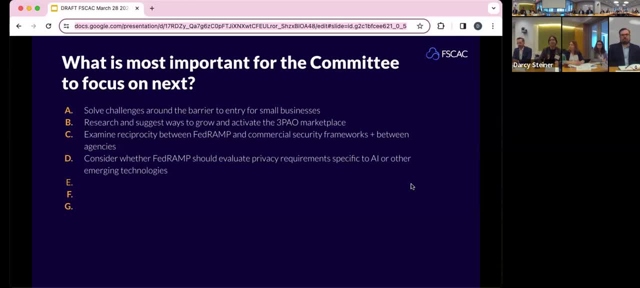 And we need a government-wide approach to dealing with these with all of the vendors. So that is my pain point day in and day out is: how are we dealing with all these requirements? So I would broaden D away from just the privacy specific requirements of AI. 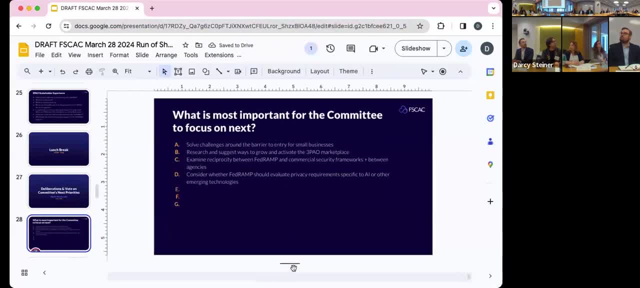 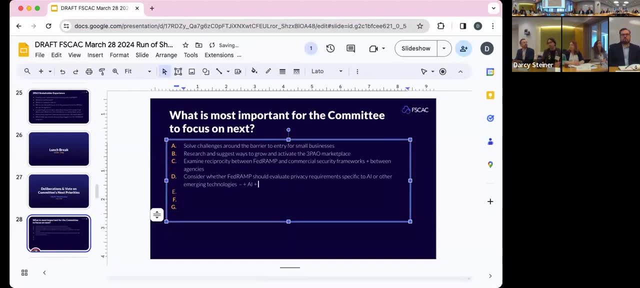 I mean everything that's in that new AI memo that just dropped last night, And all of those areas are things to be looking at, as well as the bods, as well as all of these other requirements that are coming out and think about broadening the program. 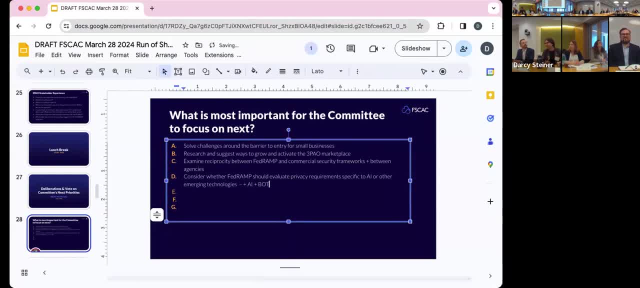 And I understand that there's 183 difference from what I said a year ago on this topic, That we should only be focusing on the 853 stuff. This is where my pain lives, personally: D instead of a T. We're worried about that too. 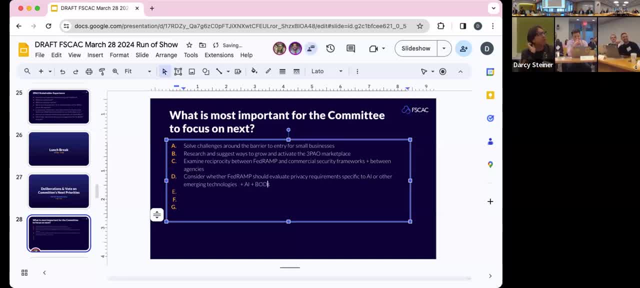 Bods are a problem. It's not going to be my size. Thank you, Sorry. What does bod mean? Find an operating, So maybe it's a different line. I mean, it's an important thing to be focusing on, But it's not the same as AI. 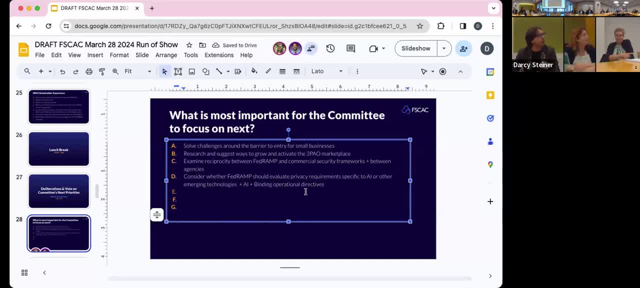 Yeah, I'm proposing a modification to D. It could be a D, part B or part one or whatever, But basically saying we should consider the variety of other requirements that have been introduced that are current and ongoing and persistent, of which privacy requirements of AI is one. 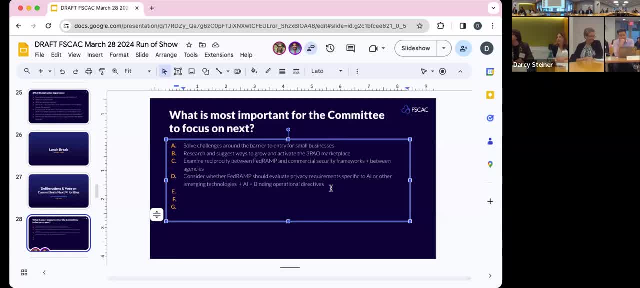 I think there is a question, Please. Well, we have Daniel. All right, Daniel. I'm sorry, Michelle, did you want to follow up on that? Well, I thought we had the first, So I just have two quick ones. 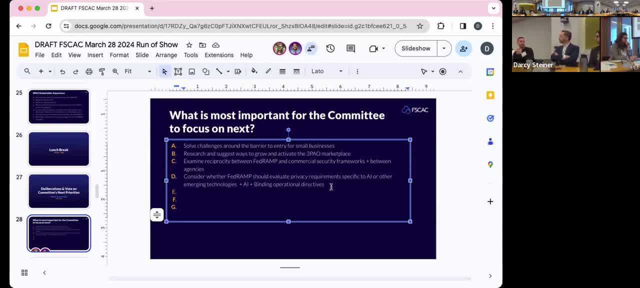 One. I think we need monitoring of the 2023 initiatives and landing of those, So everything that we had in 2023 will not actually follow through on. And then the second piece that I wanted to just hit on is: I just got out of my head. 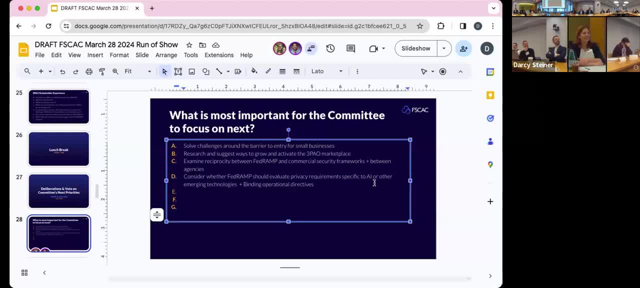 So I'll let Daniel go. Daniel go ahead. Thanks all. Data pain. data breaks Again. I think I agree with all the points that are being made here. It'd be really hard to argue against any of the lettered. 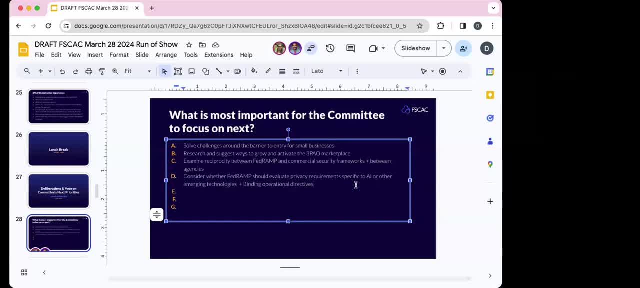 points that are up here. I think my one concern is that when I came on board a year ago as kind of quiet and trying to listen in and see what everyone was thinking, and as we move through the initiatives, I still feel like we have a lot of the same problems, that we're not. 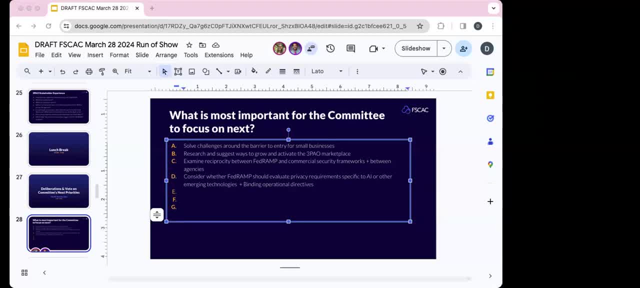 quite addressing PMOQ, lack of clarity with FedRAMP requirements, lack of cohesion between agency review teams and PMO interpretations and CSP interpretations. lack of volunteer agencies for sponsorships and, as someone mentioned, the resources for the day-to-day. 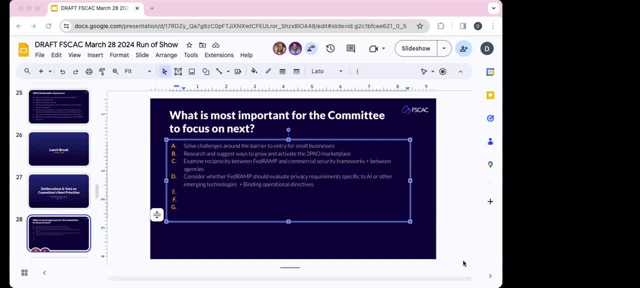 things. And then there's the emerging technologies. Some of these are kind of baseline issues that I think we've all seen and heard and dealt with. But Yeah, Until we kind of see what the PMO has to roll out, I still feel that a lot of those baseline activities and issues 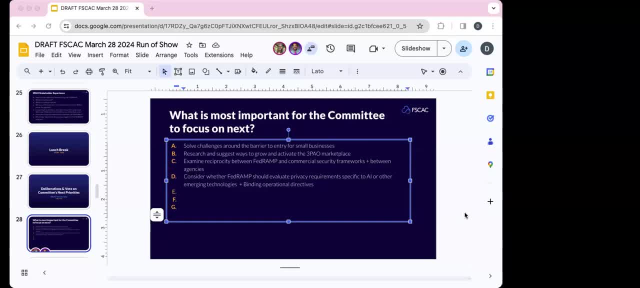 are still there And I'm not sure that any of our current initiatives are sort of hitting on that. So those are kind of my areas I think, that I'd like to tackle, as someone who's on the CSP side now and who has been on the audit side before. 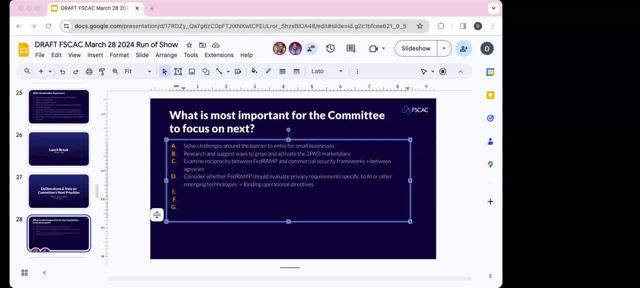 and on the agency side as well, A lot of these baseline issues are the main cause, And some of the symptoms that we're trying to fix as well are going to be the whack-a-mole kind of things. So I guess that's why I'm really concerned that we're kind of straying. 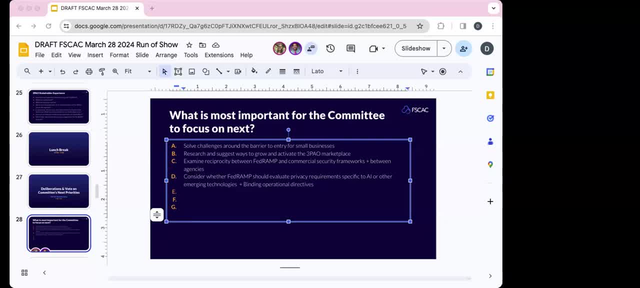 from what are the problems that FedRAMP currently has? And obviously we can move into future activities and future goals and future technologies, And that's all well and good, But I'm still trying to think of the little agencies that are struggling. they don't have resources. 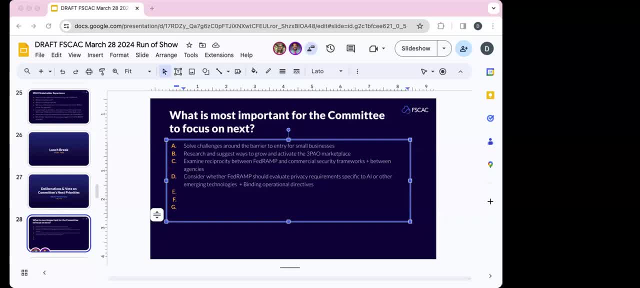 they still don't get this kind of stuff And we're all kind of breaking the sound barrier into the next wave of things to do. But I'm still trying to be cognizant of who's really struggling with the problem, And that's what's happening. 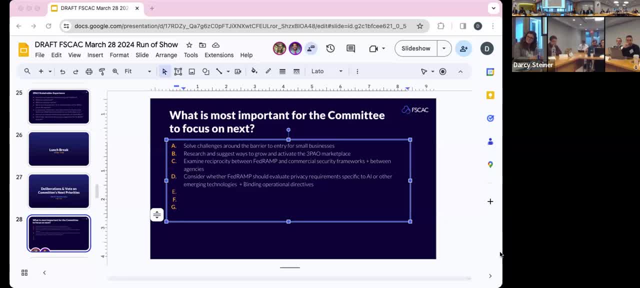 And I think that's what's going to be a big issue in the future with the process. So, Daniel, I fully agree. That's exactly what I was talking about with the landing and monitoring of our 2023 initiatives. We have to make sure that all of those things land. 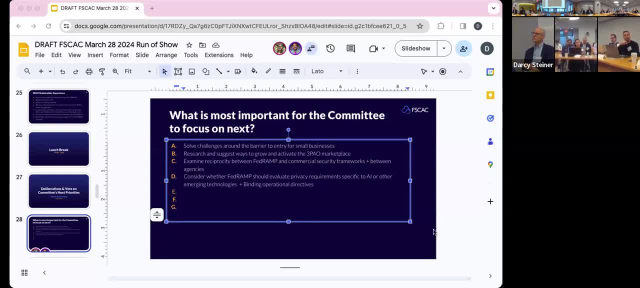 because they're kind of the table stakes for making sure that this is a successful program across the board. And then the other thing that I think we still need to focus on, or we shouldn't just focus on, is just cost reductions overall. 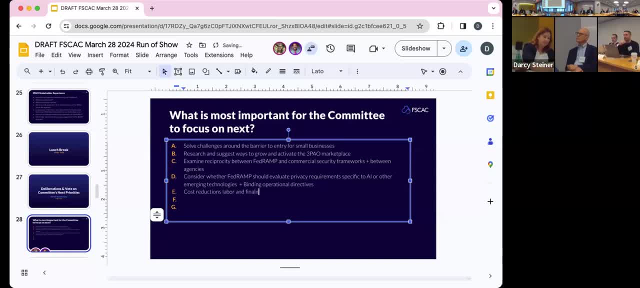 financial. so making sure that we're keeping that in mind, as at the community, and making sure we're focused on how do we continue to remove, you know, cost, drive down efficiencies, find those really low-hanging fruits that are hanging out there for us, and driving those out of the system. 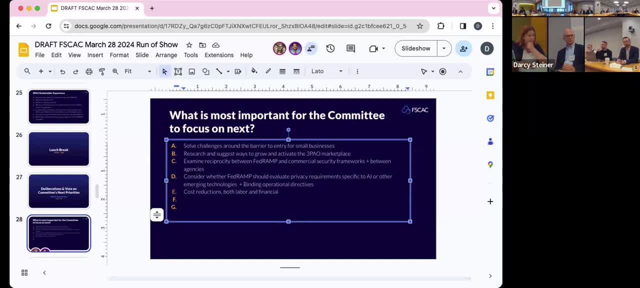 right and then we can start to really focus on how do we then improve it and catapult from that position. jackie, um, jackie's not for this um. item c, i believe, is already on the road map, so i would probably remove this from our focus because i think it already is a priority. 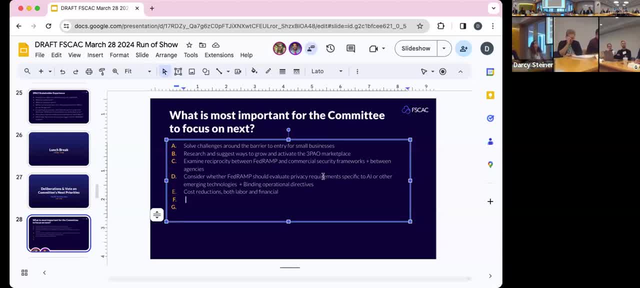 um, and the other one that i i'd like to see out of this kind of goes along with the landing of the 2023 initiatives, is the implications from the omb memo on fed ram. i think there's a lot of churn right now. um, i have churn, uh, just from specific little section of it, but i don't know. 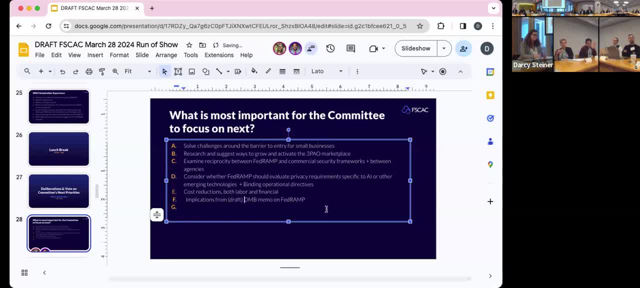 what it means that the jab's not doing authorizations anymore. do people know that the csps are turning out? they're going well, what's happening there? um, who's going to do con mod? how are we moving forward with these multi-agency things? you know, if the jab wasn't effective, 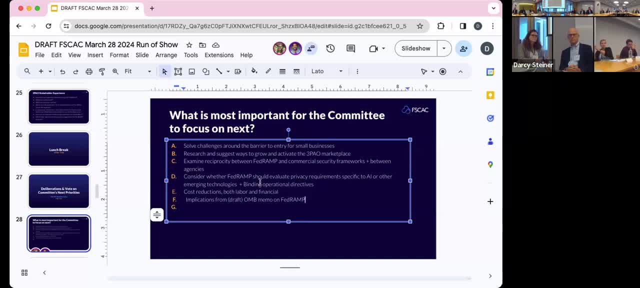 you know it turning out stuff. how are we going to just join up, you know this agency and this agency to do something? what does it mean to reach out to an agency for process improvement? um, so i think that it's to me, it's it really. i, i don't know. we heard this morning a lot of their roadmap- right, 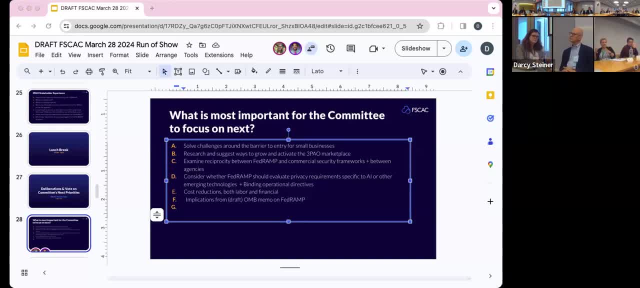 but i didn't know how they're going to implement a lot of the requirements and where that is going. so me, from a labor perspective, currently supporting the jab that doesn't exist anymore. what does that mean, you know? and, and what do you know? what is where my cost figure is going to be? what? what do i have to adjust? and so it's not. 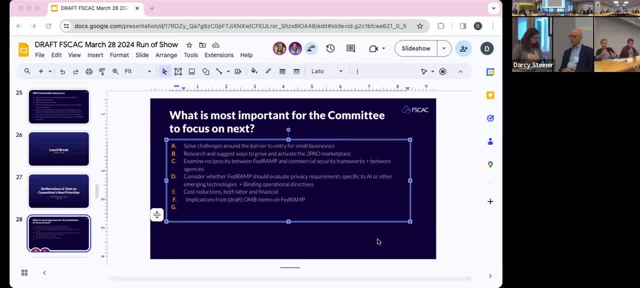 just the cloud providers, it's going to affect the three paos, it's going to affect the entire workforce and i'm not sure how that actually gets announced or codified. and so that is. i mean that to me is a real immediate concern, because the essentially when something comes out of draft. 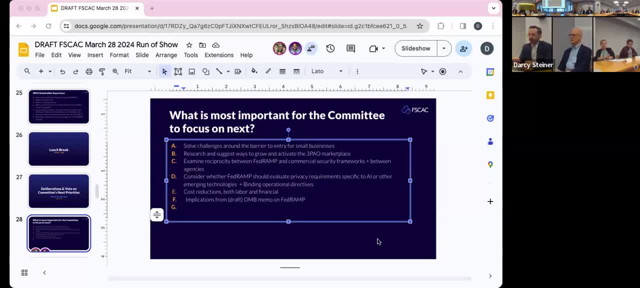 fedramp today reacts, and so certain actions have been taken, but do people clearly know what those mean to them in their workspace? okay, i thought too. i think that, marcy richardman, i think that's really important because you know, we've talked, we've heard today just from the folks in the room about no one really wants to. 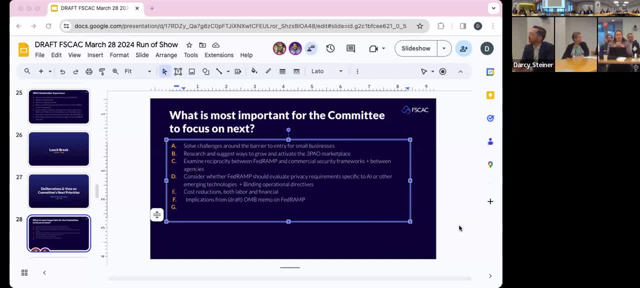 be an agency sponsor, because there's a labor and there's all the time and hours it goes into that. um, but if jobs aren't authorizing and we don't have the new program authorization, that's the only path right now and so we're we're going to be at this at this point. 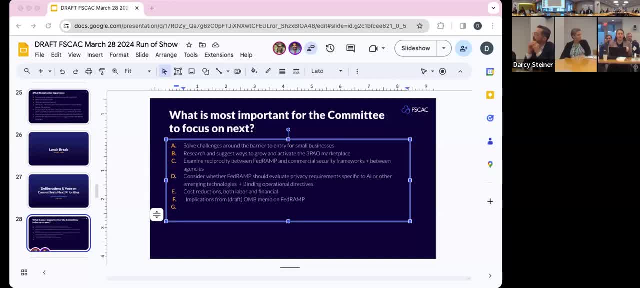 where there are no new off, like there are very few ways to get authorized and so we're continuing to build and create additional bottlenecks. so, like the additional authorization paths that were outlined in the memo, um, we didn't spend much time on that this morning but um with the omb folks. but 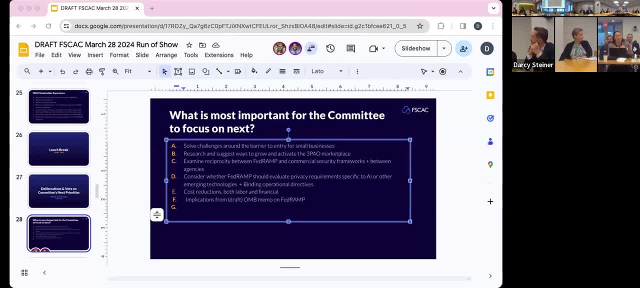 i, i think that that should. i don't know how that affects us, but i think that should be a point of concern because it's going to affect the overall number of authorizations. i think it's a really good point and it's table stakes and, um, i don't know if this is a lot you. 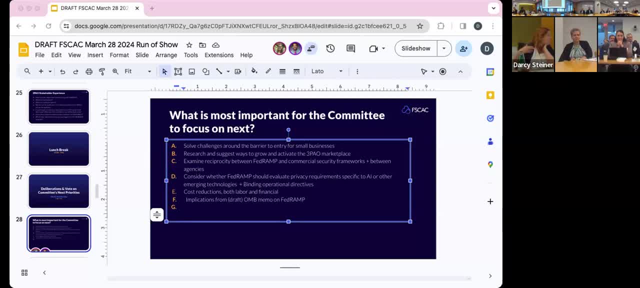 can tell me if it's not, but i, um, can we ask the federal app folks who are in the room to respond to? actually, there is a communication plan that is happening but, um, in terms of like, is there anything that you guys would like to say that would address some of the concerns here about? 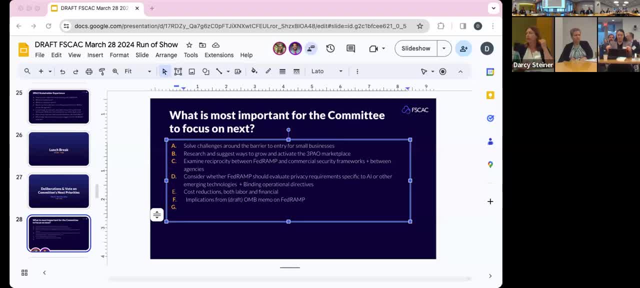 how? how does the post, job or world actually going to work? we can't do that, but if you, please come up to the, l can hear you. it's okay. you're staying in front of the team, just just. uh, you have to be close enough where to pick up your the mic. so the pmo authorization is absolutely something we want to do and deliver. 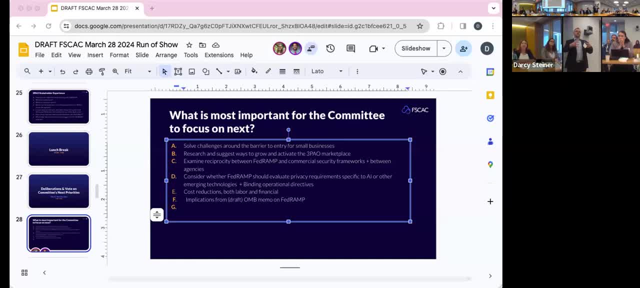 on a lot of those prioritized activities you're seeing, are really making sure we're building the capacity so that we take on this new work, we're able to execute that efficiently. so that's one of the reasons why you're not seeing it as an immediate amount of roadmap, but it is something. 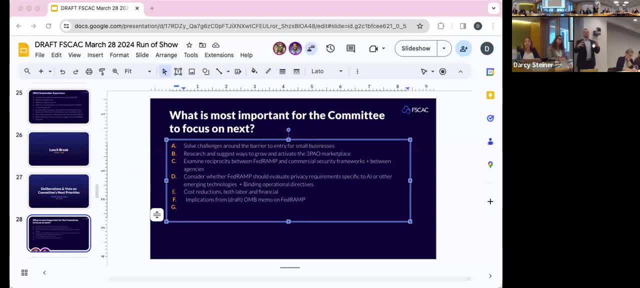 that is a priority because it's important to build a marketplace and the potential gaps in the marketplace as well. so this is jackie. so does that mean the pmo is as a almost as an agency you're going to issue authorizations with just you? are you going to partner or have? how does that work, or do you know? 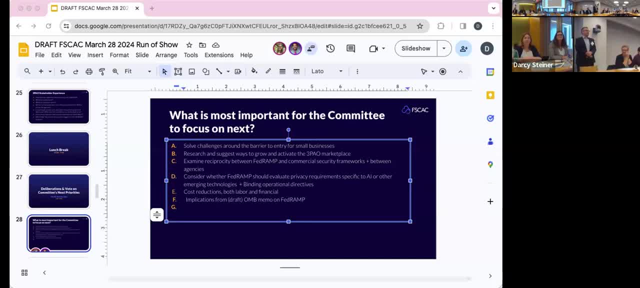 you may not know. i think that final on the memo is going to probably determine what that looks like and how the pmo authorization is used. uh, i just think there's certainly a prioritization element: filling things in the marketplace. csps also need services as well, so there could be other demand signals we could look at and evaluate. 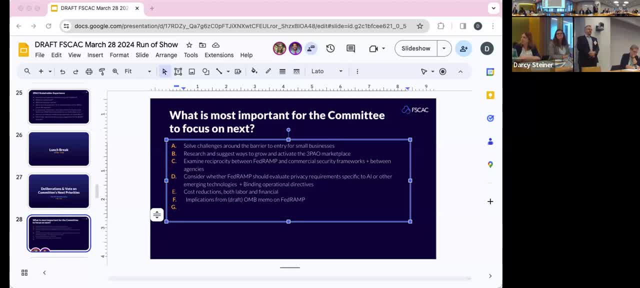 when that type of authorization would be issued. uh, mike, just a quick question on the jab sun setting. is that going to happen prior to this setup or is like: is there a plan? yeah, yeah, yeah, i think it's already sunset, it has, the jab has has really sunsetted at this point as- and it will not be, you know, convening. 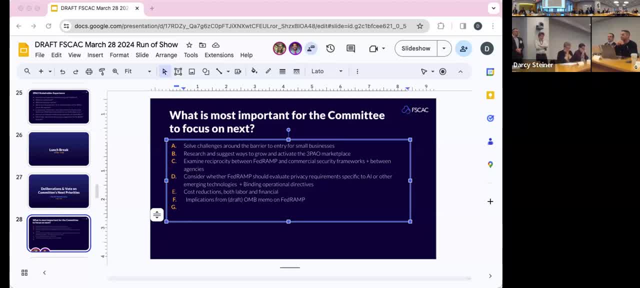 again as the jab um. the next thing i think you will likely see, as you know, really more on own being a speed for this detail, right, but will be the assembly of the veteran board and some of the some of the threads that i see in this discussion are also. you know, that's what i think you will. 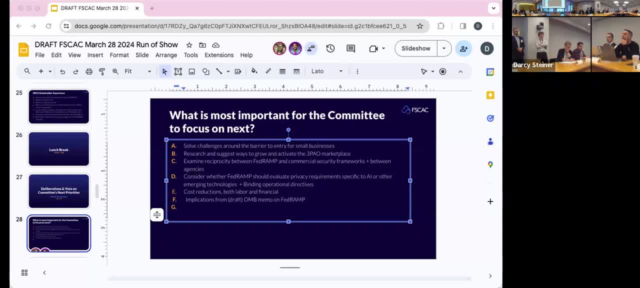 likely see those bodies taking a? uh, it'll be some of the first real things they have to sort out, but there's a limit to what gsa and the program can say definitively about how agencies are being organized and how their work will be performed. um, but that is definitely we. we've been observing it. 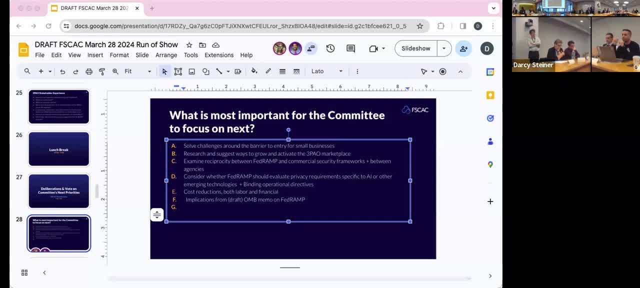 as a pretty active line of work on that part. just a quick follow-up on that one: do we know who owns that roadmap and can we get that roadmap presented at our next view and that might not be able. that might be a more general question. yeah, i, i mean, i think that is is likely. 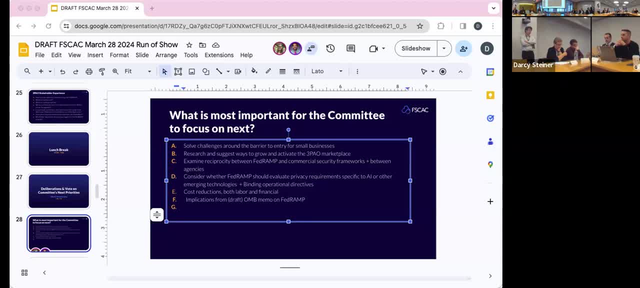 be something that we channel towards that would be- and to enter the board once it's brought together. i mean, it sounds like we're reducing the pathways to authorization current in current state to get to a broader state leader like we've jab is not giving any initial authorizations right. 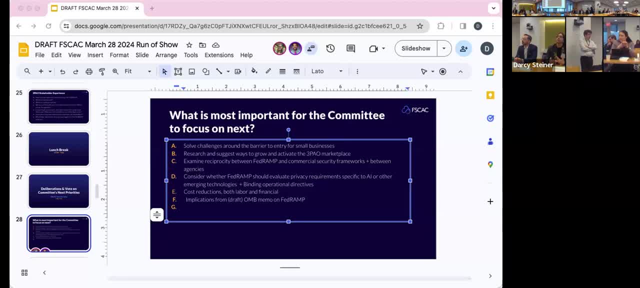 now there's no additional patos being granted by jab, so it's agency or nothing currency, is that right? i mean those, i think right now i mean there are, uh, in terms of what's being actioned, i think right now, agency authorizations are the ones that are the most active periods. 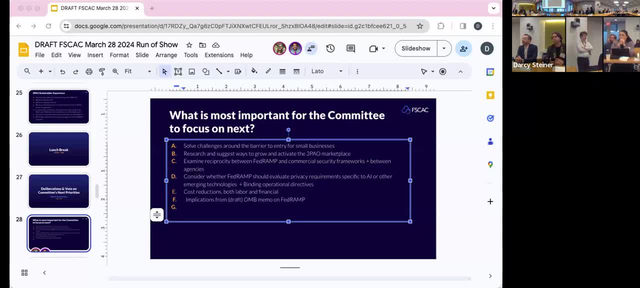 that we've just described. but the um, you know, what i think folks are trying to bring together here from both sides are more pathways than existed before. um, i think folks are noting the pain of the transition. okay, and would that be something that you could take up as like an action? 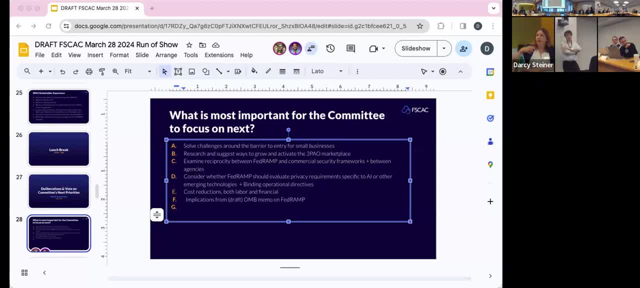 to see who owns this. yeah, i think you're. you're drawing out an important um point, which is that, during the transition, we're going to see a dip in authorizations and pent-up demand and then, as the pmo wraps up its capacity to do authorizations, they'll be- you know, it'll- be an uncomfortable. 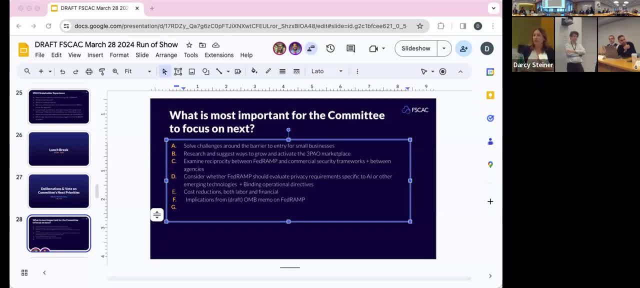 transition. so i think we could certainly um get more information on the, the communication plan, the timeline and the roadmap for that, and also communicate the concerns you've just articulated here in this room too. all right, thank you so much for joining us today, and we'll see you next time. 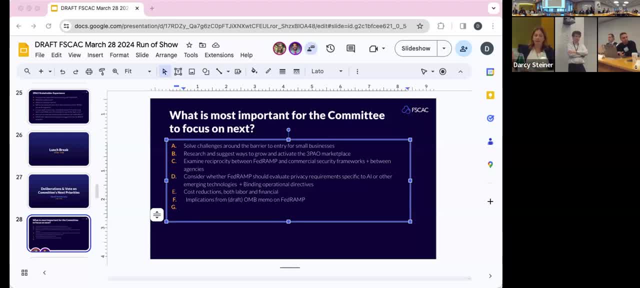 all right, thank you so much for joining us today and we'll see you next time. so that we're all aware that, um that we're, we're entering into a state where, um there will be some negative impacts before there's a long-term positive impact, so we should 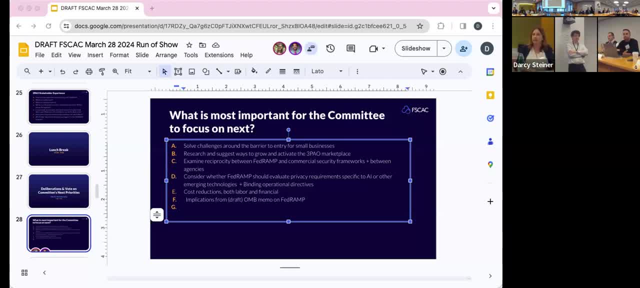 just be clear and transparent about that as much as we can, and omb, gsa, etc. should be able to communicate to this group um effectively about what to expect. you better be on the phone, hi. uh, yeah, this is carol bells. um, i just wanted to add that. um, you know, because 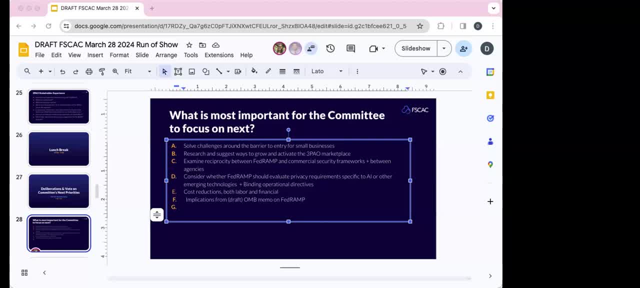 omb is in the process of establishing the fed ramp board. um. i wasn't on the call this morning, i'm sure drew probably mentioned that maybe. um, so in in as far as the concerns about um authorizations and the board doing authorizations, there would be nothing stopping the new board from 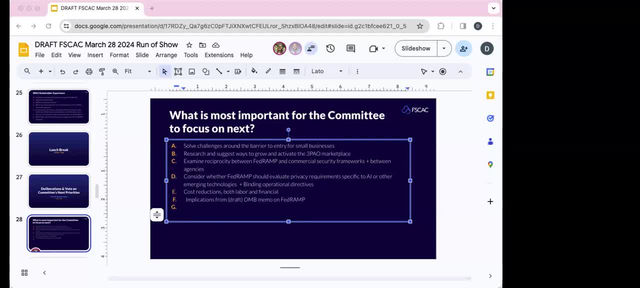 doing authorizations. um, it is in the statute that they can perform authorizations, but we are wanting to rely more on the agencies, more so than we've done in the past, just because of the vast number of uh cloud service offerings that are out there and we need to dramatically, like, increase uh. 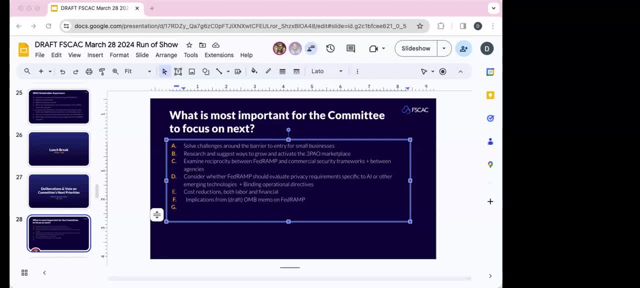 the number of products and services that are in the marketplace, um. so that's why we're just looking at all of the different options for um, how we may be able to increase uh capacity. carol does omb currently have in the materials that plan to communicate the future? 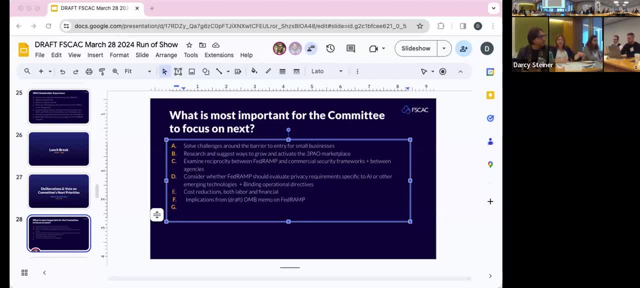 understanding or estimation of the volume of authorizations that would be affected by the transition and what our goals would be around either preserving the volume of authorizations or increasing, because it stating that we want agencies to do more authorizations. that's it. that's an intention we could also like aggressively bring agencies to the table and say: 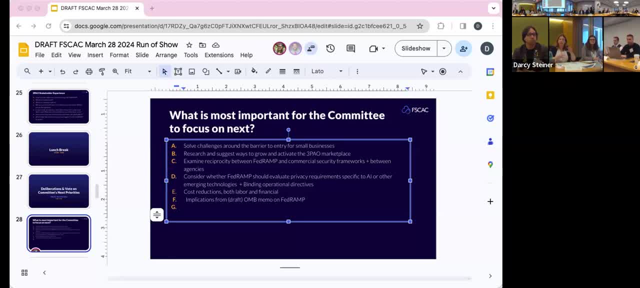 we've got 150 pending authorizations going to pick them up, you know. so I'm just, I think, what we're. there's some anxiety in the room right now that I'm sure we can resolve with communication around. what do we do for folks who are waiting now? 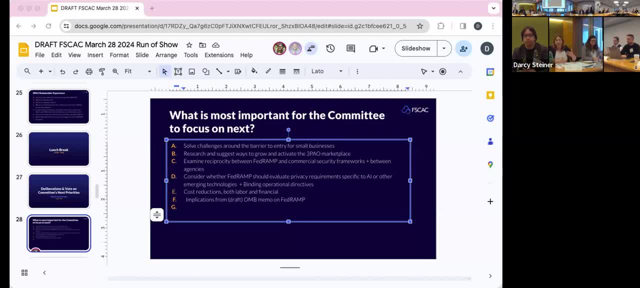 and how long realistically should they wait and what proactive actions can they take to accommodate the transition that you're planning to roll out? yeah, I think, like um, that's um. like I mentioned, we're in the process of standing up the FedRAMP board, so I think that's that board. 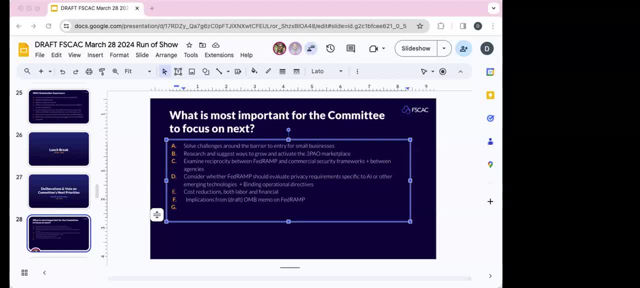 that's going to kind of um define what those next steps are. so I know that the JAB was working to, you know, finalize everything that was in the process currently, get those authorizations, uh, signed, you know, and added into the marketplace, and then everything new will kind of fall under. 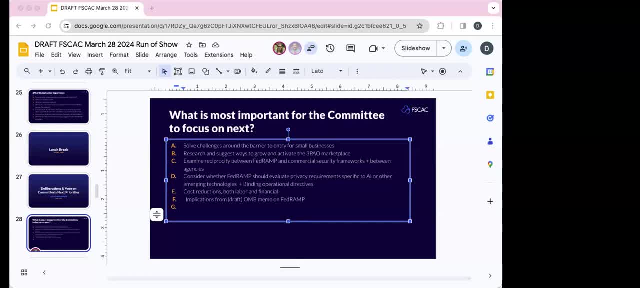 the new FedRAMP board and what plans that they'll have in place with respect to the authorizations and the priorities- gotcha, gotcha. for folks who are waiting now, is there any specific guidance you'd give them on continue to wait until you hear specific next steps from us, or is there anything you'd like? the 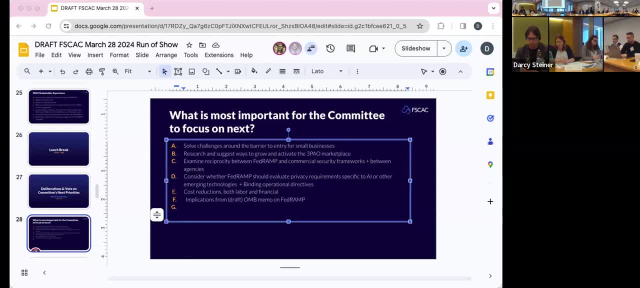 audience to proactively consider and start doing okay. so are you referring to maybe someone who's already started the process? um, because you know, I believe you know, if they've actually already started the process, the intent would be to: um, you know, continue, um, you know, continue um. 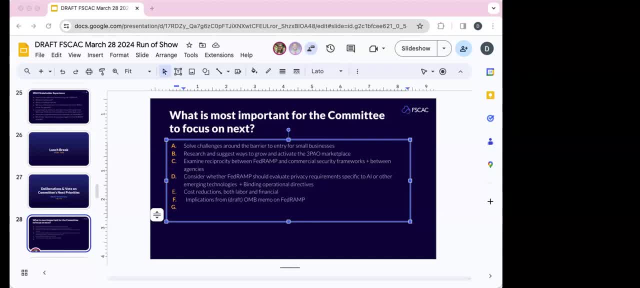 you know, continue um with that in completing the authorization, with that, in completing the authorization, with that, in completing the authorization, are there specific use cases? that folks that are there specific use cases, that folks that are there specific use cases, that folks that we're speaking of earlier and like to flag. 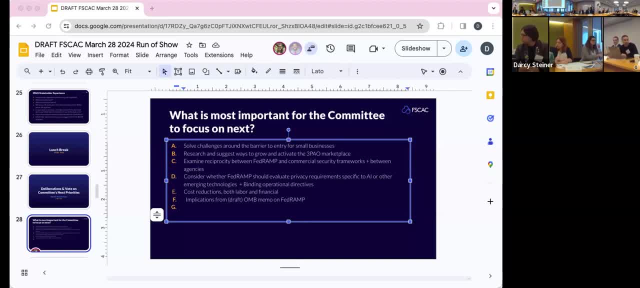 we're speaking of earlier and like to flag. we're speaking of earlier and like to flag for carol, for carol, for carol. yeah, I mean I'm worried about the FedRAMP. yeah, I mean I'm worried about the FedRAMP. yeah, I mean I'm worried about the FedRAMP queue of current accreditations that are in. 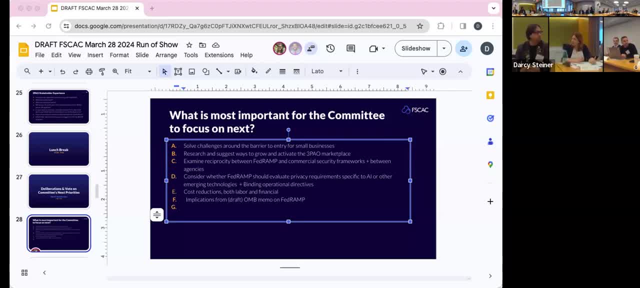 queue of current accreditations that are in queue of current accreditations that are in process. so in queue but not yet assigned process. so in queue but not yet assigned process. so in queue but not yet assigned to to to uh an agency, potentially at any stage, I 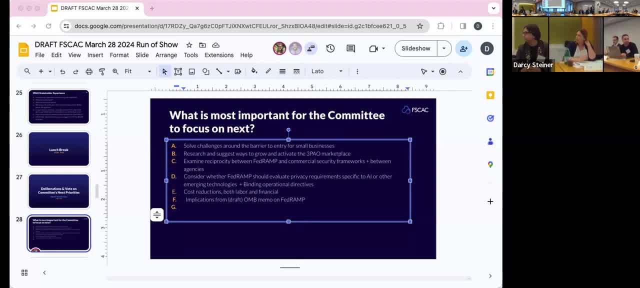 uh an agency potentially at any stage. I uh an agency potentially at any stage. I mean just anything that's gone out from, mean just anything that's gone out from, mean just anything that's gone out from the 3PAO and from the CSP to the JAB. 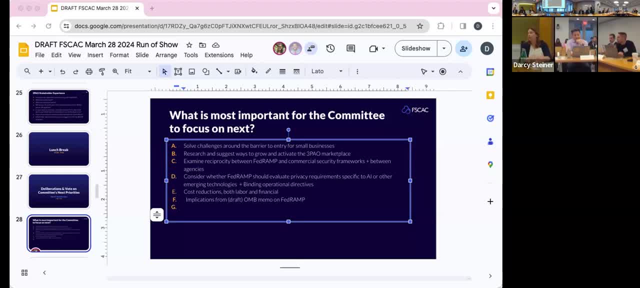 the 3PAO, and from the CSP to the JAB, the 3PAO, and from the CSP to the JAB for for sign up, and it looks like there's for for sign up and it looks like there's for for sign up, and it looks like there's 13 hot service providers that are in the. 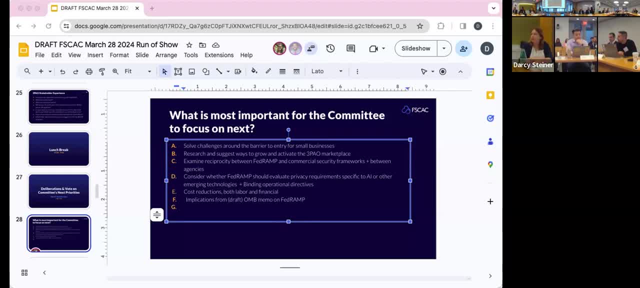 13 hot service providers that are in the 13 hot service providers that are in the FedRAMP jab queue with either a status of FedRAMP jab queue with either a status of FedRAMP jab queue with either a status of FedRAMP ready or FedRAMP process. 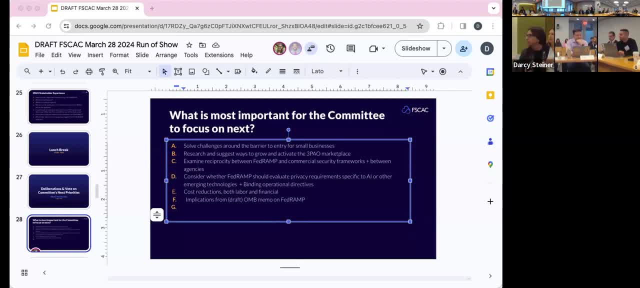 FedRAMP ready or FedRAMP process. FedRAMP ready or FedRAMP process? including one: google to gcd. including one google to gcd. including one google to gcd. probably, probably, probably, thinking broader, but yes, thinking broader, but yes. thinking broader, but yes. and if we're pushing the onus to the 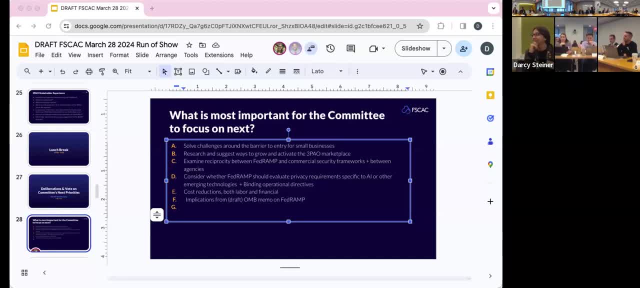 and if we're pushing the onus to the and if we're pushing the onus to the agencies, agencies, agencies, what support are they getting to? what support are they getting to? what support are they getting to? to be to sponsor packages? that that is to be to sponsor packages. that that is. 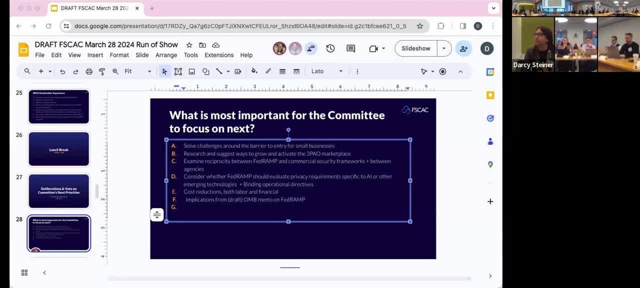 to be to sponsor packages. that that is going in the near near term, going to be going in the near near term, going to be going in the near near term, going to be the only option effectively, the only option effectively, the only option effectively. but, and if I just add a point, that 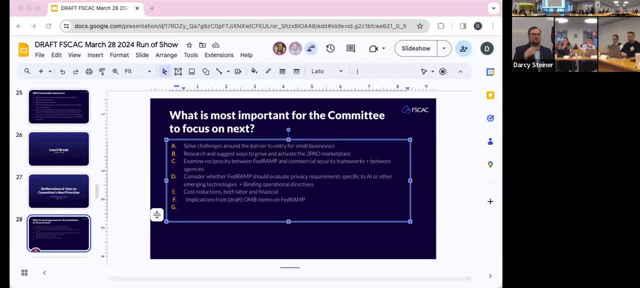 but and if I just add a point, that but, and if I just add a point that bill made before, I wouldn't assume that bill made before. I wouldn't assume that bill made before. I wouldn't assume that just because we're a larger agency than, just because we're a larger agency than. 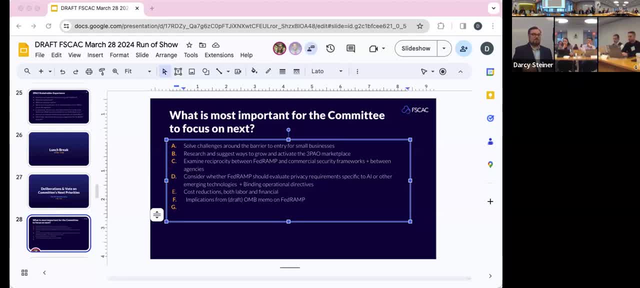 just because we're a larger agency than we have any less the budget. you know we have any less the budget. you know we have any less the budget. you know we're also responsible for a lot of. we're also responsible for a lot of. we're also responsible for a lot of things, and it should definitely not be. 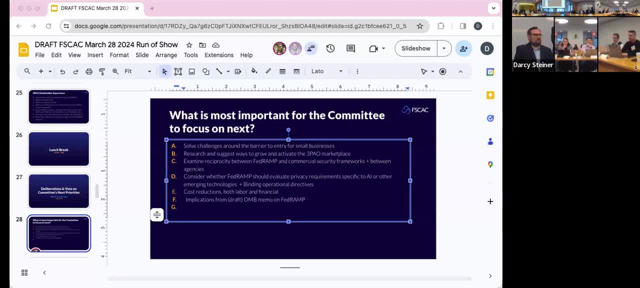 things and it should definitely not be things and it should definitely not be assumed that we would have additional, assumed that we would have additional. assumed that we would have additional- like we're all all our budgets are like we're all all our budgets are like we're all all our budgets are getting cut in the next couple years. so 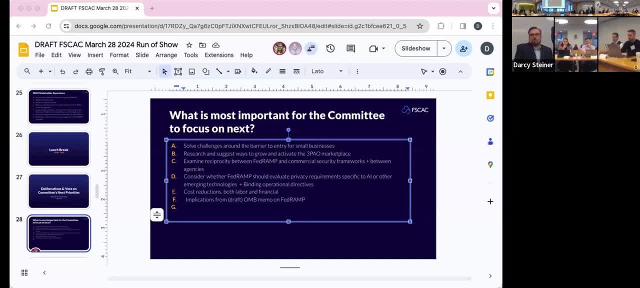 getting cut in the next couple years. so getting cut in the next couple years, so it's that's going to be a big challenge. it's that's going to be a big challenge. it's that's going to be a big challenge of that. uh so, and communication, I think. 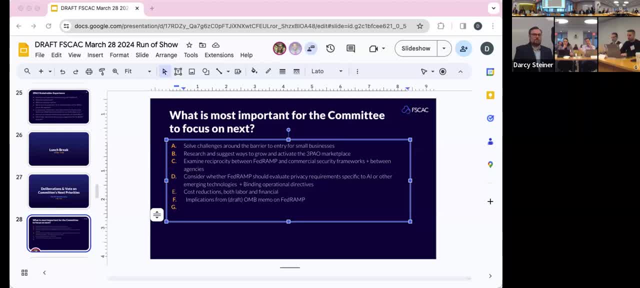 of that, uh so, and communication. I think of that, uh so, and communication. I think this would be very helpful there, but this would be very helpful there, but this would be very helpful there, but resources would probably as well. resources would probably as well. resources would probably as well. just to say the obvious thing: yeah, I. just to say the obvious thing. yeah, I just to say the obvious thing. yeah, I mean, I don't know who's read all the mean. I don't know who's read all the mean. I don't know who's read all the appropriations already. uh, but the 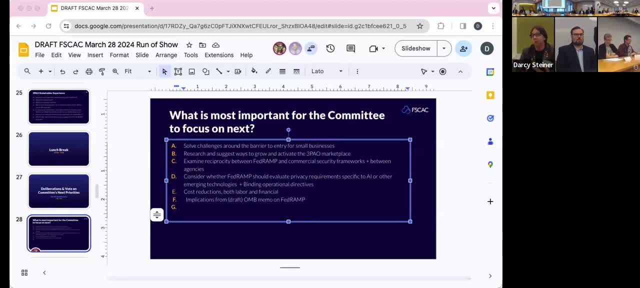 appropriations already: uh, but the appropriations already, uh, but the numbers don't go up. numbers don't go up. numbers don't go up. this year it's pretty astonishing most this year. it's pretty astonishing most this year. it's pretty astonishing. most of us took cuts or flat. I the notion. of us took cuts or flat. I the notion of us took cuts or flat. I the notion that agencies will suddenly be able to, that agencies will suddenly be able to, that agencies will suddenly be able to pick up all of this work that the jab. pick up all of this work that the jab. 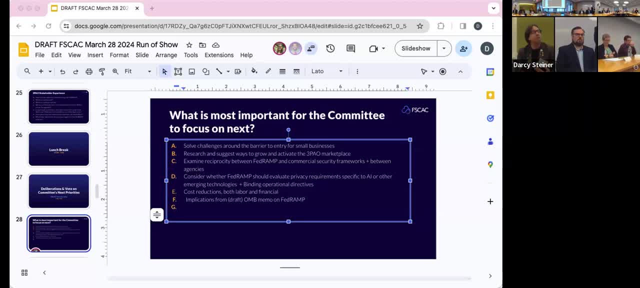 pick up all of this work that the jab didn't have time to do. um. I find a didn't have time to do. um. I find a didn't have time to do um. I find a little little little confusing and astonishing I'd say things. confusing and astonishing, I'd say things. 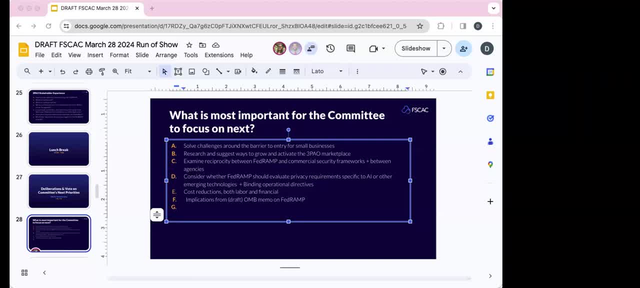 confusing and astonishing. I'd say things like this: yeah, yeah, like this, yeah, yeah, like this, yeah, yeah, yeah, and I think like what we're trying to, and I think like what we're trying to, and I think like what we're trying to do, for example, um, historically, you know, 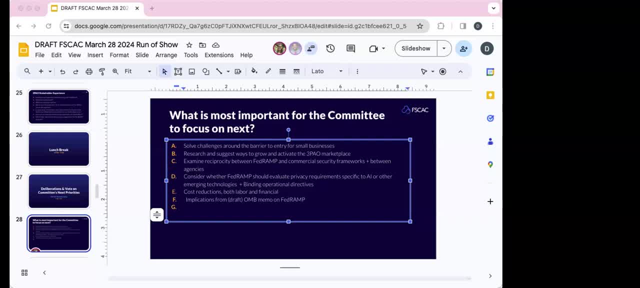 do, for example um historically, you know. do for example um historically, you know, the jab, the jab, the jab, um had been performing joint, um had been performing joint, um had been performing joint authorizations. there would not there authorizations, there would not there authorizations, there would not there. you know, there's nothing stopping. 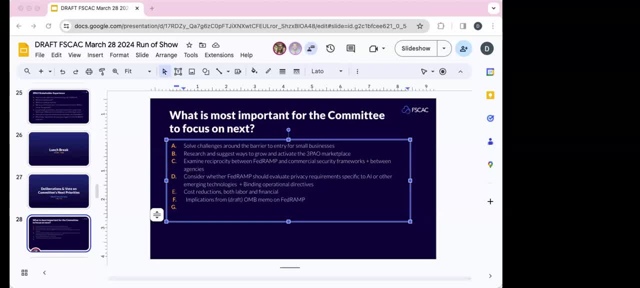 you know there's nothing stopping. you know there's nothing stopping. maybe the agencies different agencies, maybe the agencies different agencies, maybe the agencies different agencies, beyond those historical jab agencies, beyond those historical jab agencies, beyond those historical jab agencies, from kind of, from kind of, from kind of getting together and conducting joint. 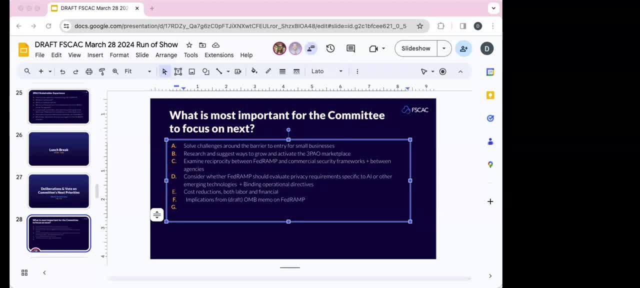 getting together and conducting joint getting together and conducting joint authorizations. so we're just trying to authorizations. so we're just trying to authorizations, so we're just trying to look at all the various ways that can look at, all the various ways that can look at, all the various ways that can kind of 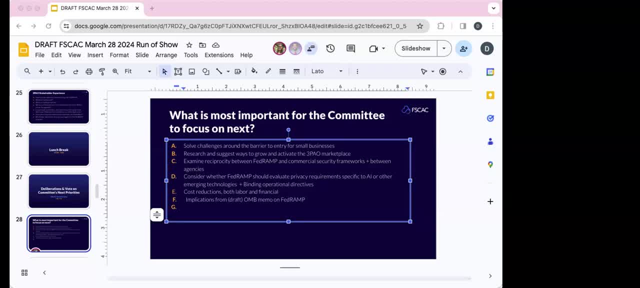 kind of kind of expand what we're currently doing in expand what we're currently doing in expand what we're currently doing in order to order to order: to help increase the number of solutions, help increase the number of solutions, help increase the number of solutions that are. 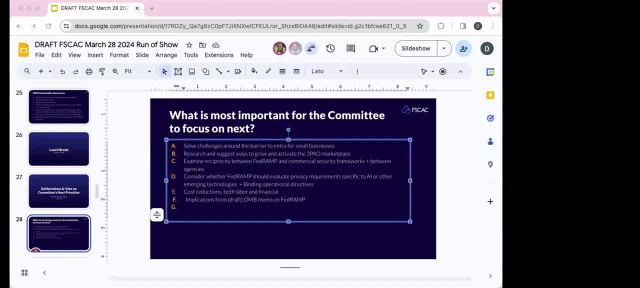 that are that are entered into the fed ramp marketplace. so entered into the fed ramp marketplace. so entered into the fed ramp marketplace. so, yeah, thanks for that, carol. i think that, yeah, thanks for that, carol. i think that, yeah, thanks for that, carol. i think that this group perceives there to be 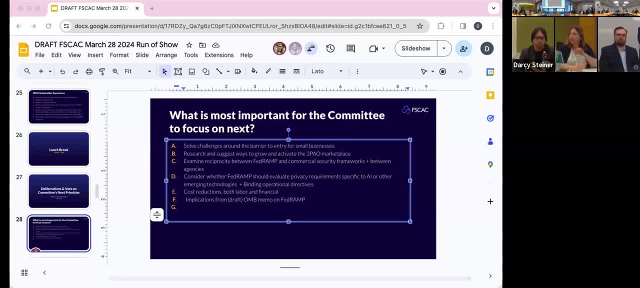 this group perceives there to be- this group perceives there to be barriers to barriers to barriers to agencies stepping in and doing more of agencies stepping in and doing more of agencies stepping in and doing more of this work, and one of them as a few, this work and one of them as a few. 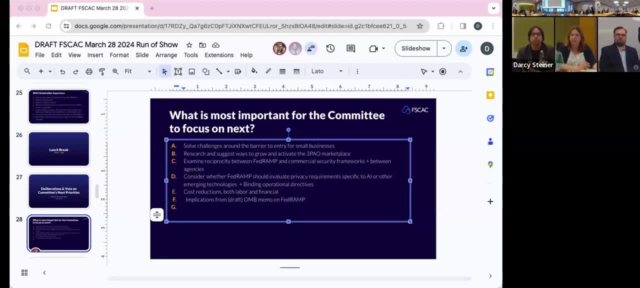 this work and one of them, as a few years ago, was describing the initial years ago, was describing the initial years ago was describing the initial authorization. that's in the order of authorization. that's in the order of authorization. that's in the order of magnitude of small digit millions. magnitude of small digit millions. magnitude of small digit millions, depending on the size of the cloud. depending on the size of the cloud, depending on the size of the cloud service provider, and then going forward service provider, and then going forward service provider, and then going forward indefinitely. there's a maintenance cost. 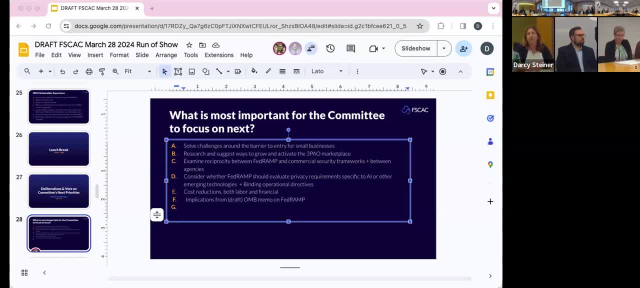 indefinitely, there's a maintenance cost. indefinitely, there's a maintenance cost of about what was it 1.3 million? one for of about what was it 1.3 million? one for of about what was it 1.3 million? one for every 20 cloud providers that we're. 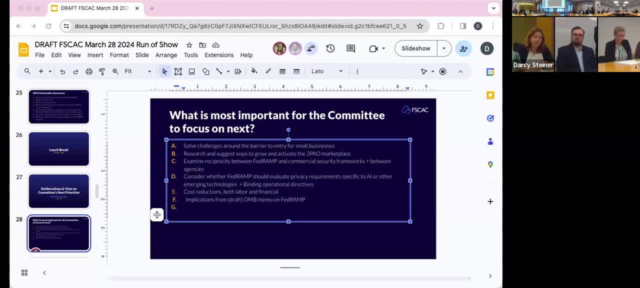 every 20 cloud providers that we're every 20 cloud providers that we're doing continuous monitoring for 1.3, doing continuous monitoring for 1.3, doing continuous monitoring for 1.3. million for every 20 cloud providers. so million for every 20 cloud providers. so 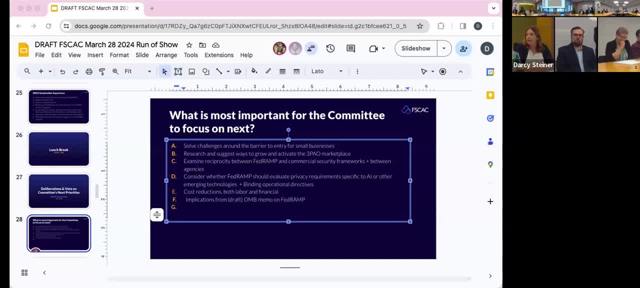 million for every 20 cloud providers. so it's, it's not nothing. it's it's part of it's. it's not nothing, it's it's part of it's. it's not nothing. it's it's part of the budget planning that that cios and 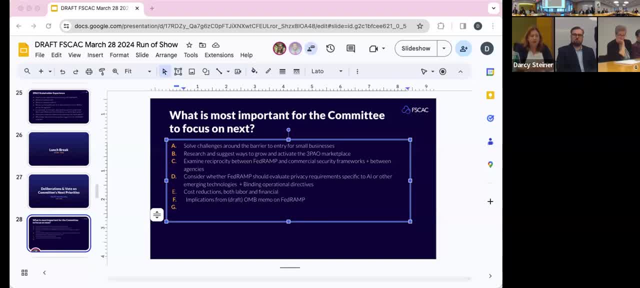 the budget planning that that cios and the budget planning that that cios and ciso shops have to do ciso shops have to do ciso shops have to do um so and i think also, uh it, i, i, um so, and i think also, uh it, i i. 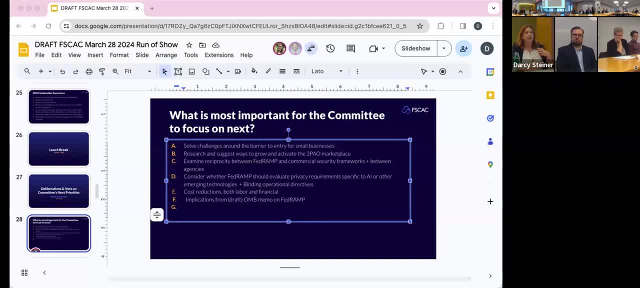 um so, and i think also: uh it, i, i, i'm reading in this situation: there's not. i'm reading in this situation: there's not. i'm reading in this situation: there's not necessarily agencies are not necessarily. agencies are not necessarily hearing a call to like raise. 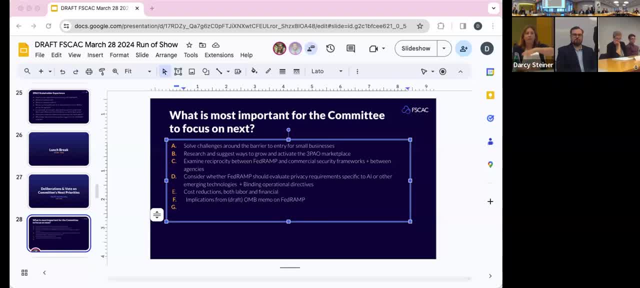 necessarily hearing a call to like raise. necessarily hearing a call to like raise your hand and help out with the 13, your hand and help out with the 13, your hand and help out with the 13 people in the queue, plus the 25 who are: 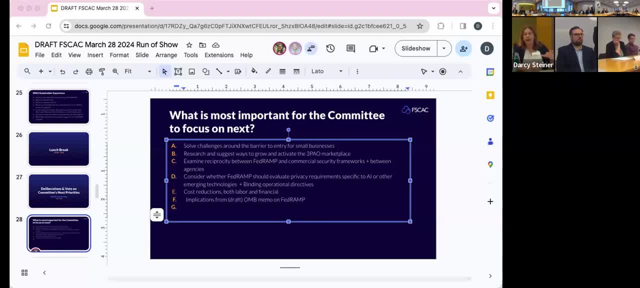 people in the queue plus the 25 who are people in the queue plus the 25 who are in unfunded kanban status or whatever. so in unfunded kanban status or whatever, so in unfunded kanban status or whatever. so i think it would be helpful that if the 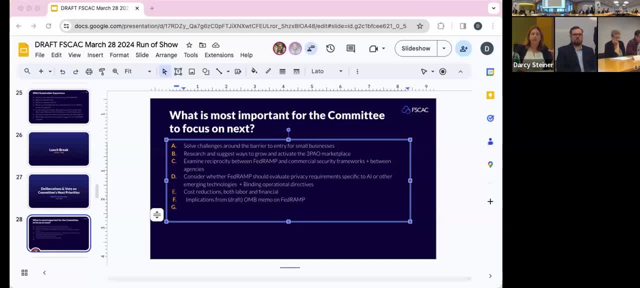 i think it would be helpful that if the. i think it would be helpful that if the total set of cloud service providers, who total set of cloud service providers, who total set of cloud service providers who are going to be affected by the are going to be affected by the, 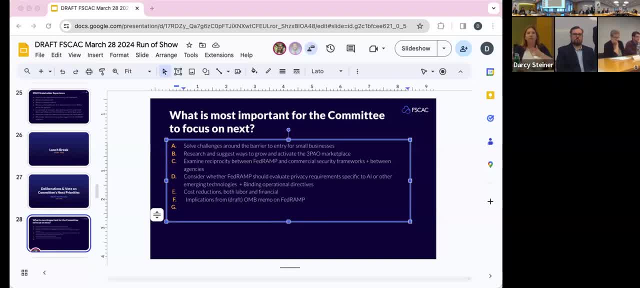 are going to be affected by the transition is something like 30 or 40.. i are going to be affected by the transition is something like 30 or 40.. i are going to be affected by the transition is something like 30 or 40. i think it could be helpful for. 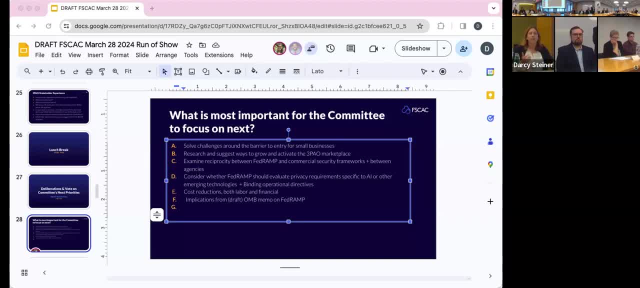 think it could be helpful, for think it could be helpful for federal and omb to sit down and make federal and omb to sit down, and make federal and omb to sit down and make that spreadsheet of 40 and come up with that spreadsheet of 40 and come up with 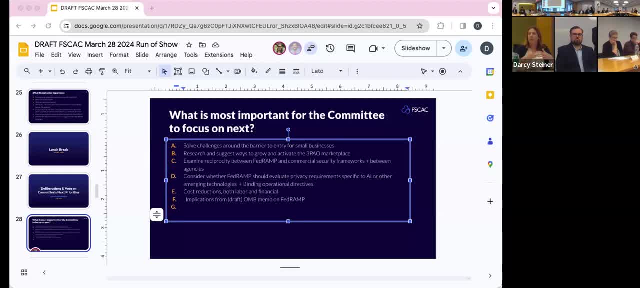 that spreadsheet of 40 and come up with a communication plan that not only a communication plan. that not only a communication plan that not only communicates to people who are awaiting communicates to people who are awaiting communicates to people who are awaiting what to expect it. uh, i'm sorry, cloud. 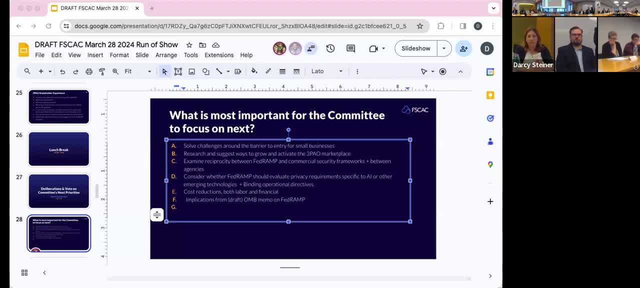 what to expect it? uh, i'm sorry. cloud: what to expect it? uh, i'm sorry. cloud service providers: what to expect? but service providers, what to expect? but service providers, what to expect? but also does some rabble rousing with? also does some rabble rousing with. 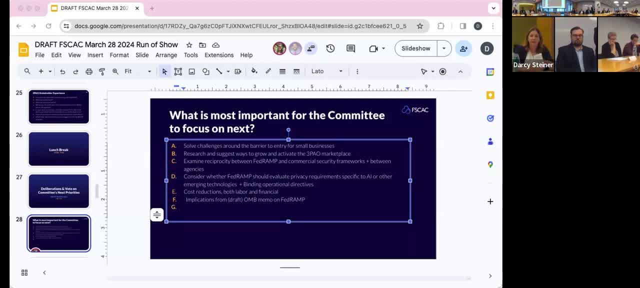 also does some rabble rousing with agencies and trying to understand who agencies and trying to understand who agencies and trying to understand who can step up and start engaging in this. can step up and start engaging in this. can step up and start engaging in this way and then try to understand what are. way and then try to understand what are way, and then try to understand what are the barriers, or what are the incentives, the barriers, or what are the incentives, the barriers, or what are the incentives that are needed to get agencies to the, that are needed to get agencies to the. 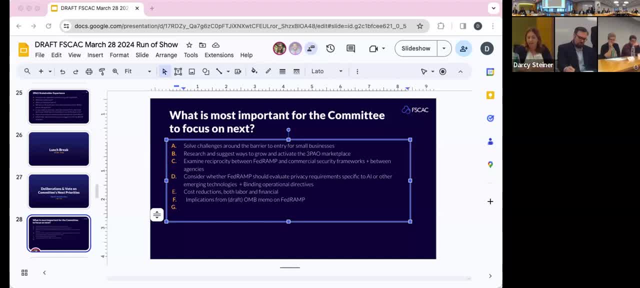 that are needed to get agencies to the table on this, on some kind of a table on this, on some kind of a table on this, on some kind of a timeline. if i could, just if i could, just if i could just from, from my perspective, just to make. 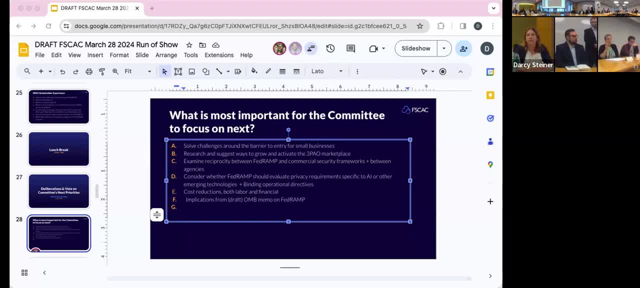 from my perspective, just to make, from my perspective, just to make sure that every level set is that sure that every level set is that sure that every level set is that from a jab authorization perspective, and from a jab authorization perspective, and from a jab authorization perspective? and maybe this is where you guys can. 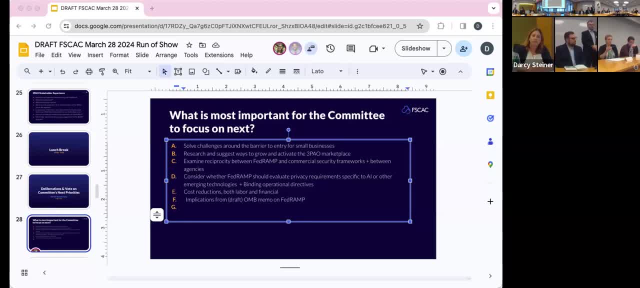 maybe this is where you guys can. maybe this is where you guys can answer this question. is we answer this question? is we answer this question? is we stopped doing jab authorizations? in stopped doing jab authorizations? in stopped doing jab authorizations in the december time frame. so that was three. 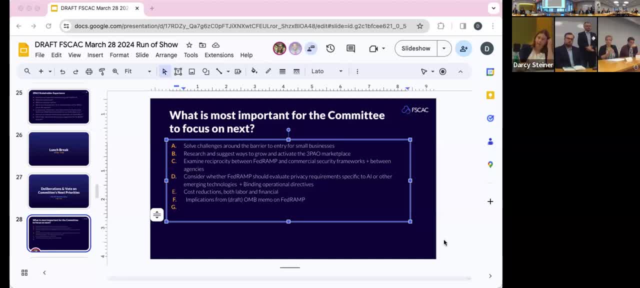 the december time frame, so that was three. the december time frame, so that was three and a half months ago and a half months ago and a half months ago you're saying the three trs, the dhs gsa. you're saying the three trs, the dhs gsa. 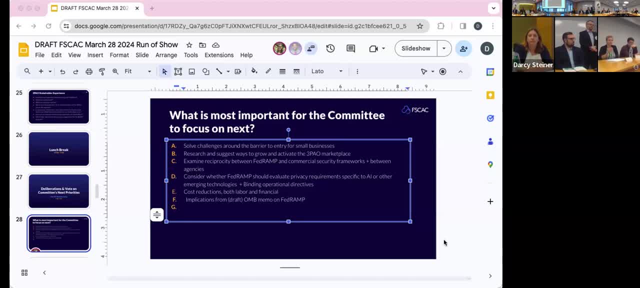 you're saying the three trs, the dhs, gsa and dod as members of the jab, the and dod as members of the jab, the and dod as members of the jab, the technical representatives- they're still technical representatives. they're still technical representatives, they're still doing the conmon on the jab. 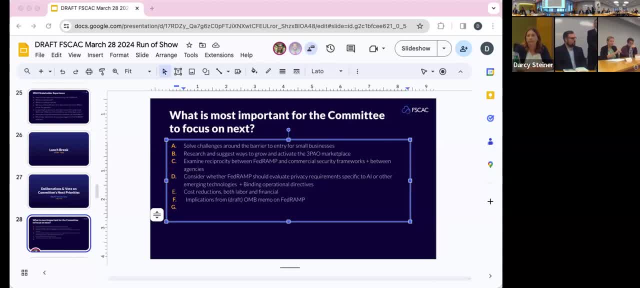 doing the conmon on the jab, doing the conmon on the jab authorizations, but if we have 13 and q authorizations, but if we have 13 and q authorizations, but if we have 13 and q and some in process and some in process, 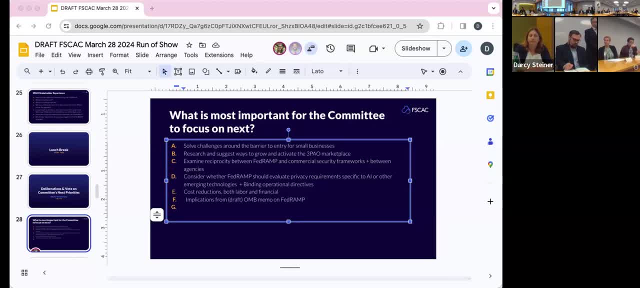 and some in process. who is actually doing that? or who's who is actually doing that? or who's who is actually doing that, or who's doing the in-process work today? is that doing the in-process work today? is that doing the in-process work today? is that just the pmo? because we're not doing. 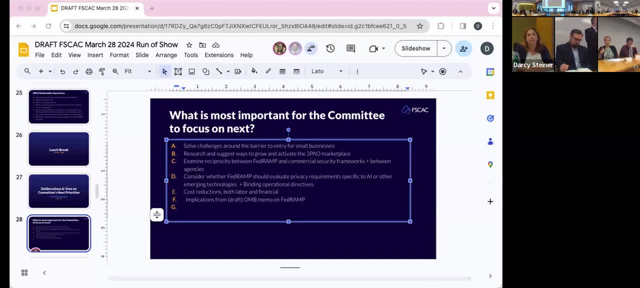 just the pmo. because we're not doing just the pmo, because we're not doing that anymore, that anymore, that anymore. we are working with the current, we are working with the current. we are working with the current providers who are in the queue. providers who are in the queue. 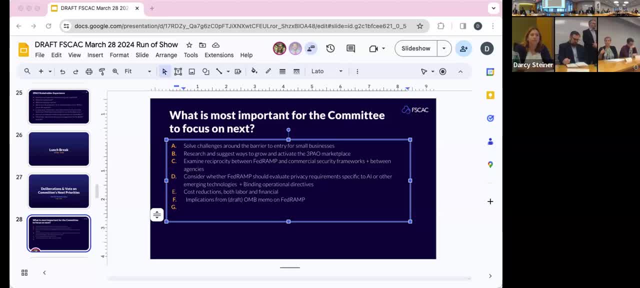 providers who are in the queue and they call making sure they make a and they call making sure they make a and they call making sure they make a good conversation process. yeah, and more good conversation process. yeah and more good conversation process. yeah, and more broadly, are tied, are tied with omb and 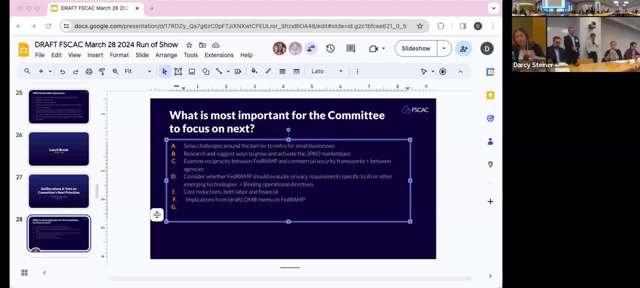 broadly are tied, are tied with omb and broadly are tied, are tied with omb. and in understanding, which of these may be in understanding, which of these may be in understanding, which of these may be good candidates for joint, good candidates for joint, good candidates for joint authorizations, which may be good. 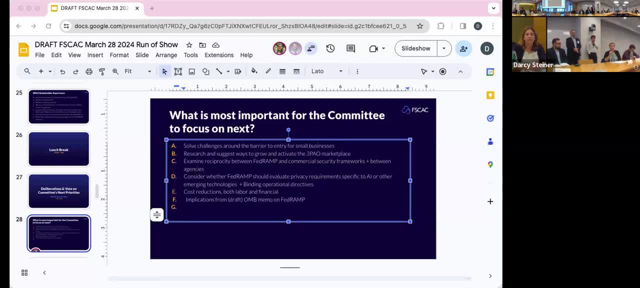 authorizations which may be good authorizations which may be good candidates for candidates, for candidates for pmo authorizations. we are pmo authorizations. we are pmo authorizations. we are, we are. you know our commitment is to not. we are, you know, our commitment is to not. 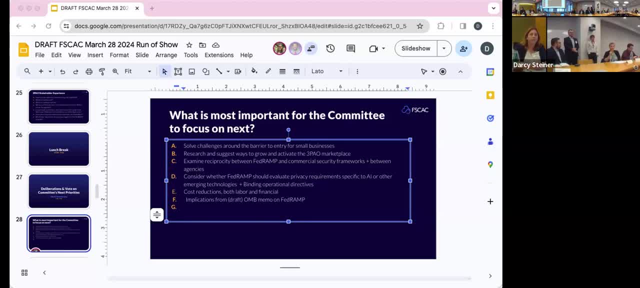 we are. you know, our commitment is to not leave the folks who are in the queue. leave the folks who are in the queue, leave the folks who are in the queue today, stuck there, today, stuck there, today, stuck there. um, there's a few ways that we could do. 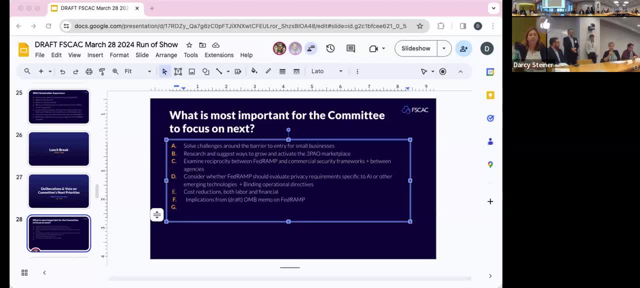 um, there's a few ways that we could do, um, there's a few ways that we could do that. it is is definitely still an in that it is is definitely still an in that it is is definitely still an in process, then process, then process, then, um, that, you know, is a multi-stakeholder. 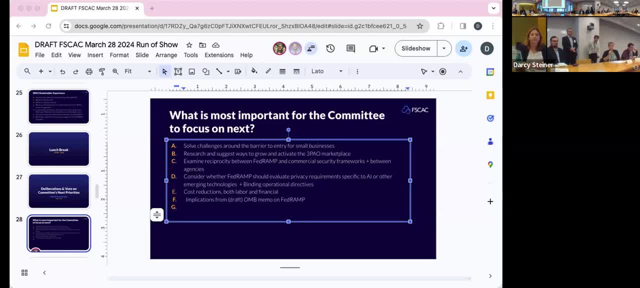 um that, you know, is a multi-stakeholder. um, that, you know, is a multi-stakeholder process. but that is the goal. okay, um daniel has a question virtually. okay, um daniel has a question virtually. okay, um daniel has a question virtually daniel, go ahead. hi, yes, no, i think it's. daniel go ahead, hi, yes, no, i think it's daniel. go ahead, hi, yes, no, i think it's just a comment to something. i heard just a comment to something. i heard just a comment to something i heard before you know. i think you know part of. 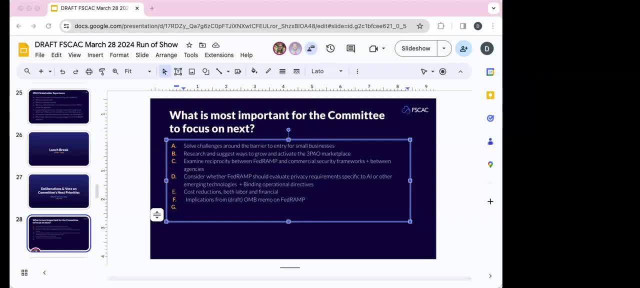 before you know, i think you know part of, before you know, i think you know part of the incentive is obviously being able. the incentive is obviously being able. the incentive is obviously being able to to use the product, but um to to use the product but um to to use the product but um, a lot of the you know the there's. a lot of the you know the. there's a lot of the you know the there's already been agency liaisons that have already been agency liaisons that have already been agency liaisons that have been identified from, i think every been identified from, i think every. 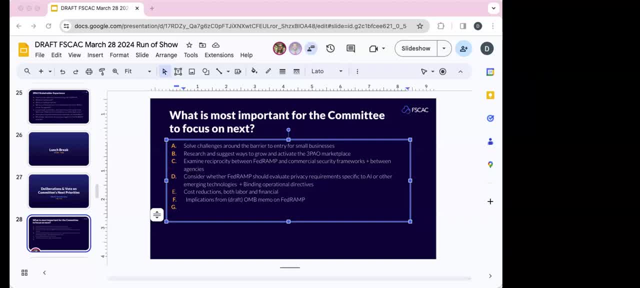 been identified from, i think, every agency and that was an initiative that agency and that was an initiative that agency and that was an initiative that happened, you know a couple years ago, happened you know a couple years ago, happened you know a couple years ago. so there should be at least one. 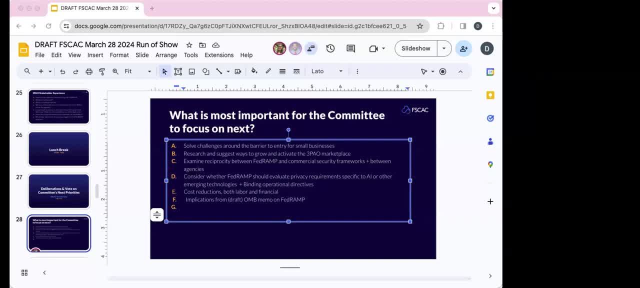 so there should be at least one. so there should be at least one representative at representative at, representative at. you know every agency that has um you. you know every agency that has um you. you know every agency that has um. you know a dog in the fight, so to speak. 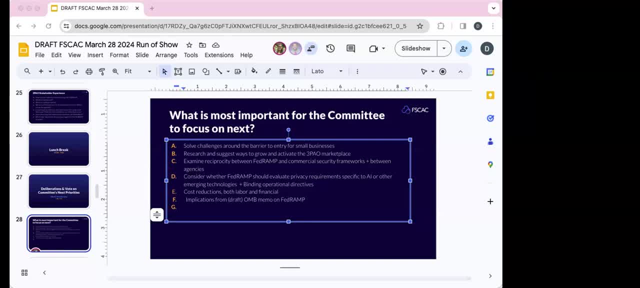 know a dog in the fight, so to speak. know a dog in the fight, so to speak, um to to you know getting cloud services, um to to you know getting cloud services, um to to you know getting cloud services through the process, through the process, through the process, um. i think that, in combination with some 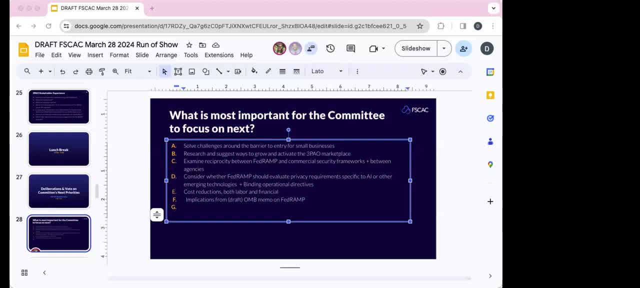 um, i think that in combination with some, um, i think that in combination with some sort of you know fedramp sherpa program, sort of you know fedramp sherpa program, sort of you know fedramp sherpa program, or or you know, having people at the or. or you know having people at the, or, or you know having people at the table here and obviously no one wants to table here. and obviously no one wants to table here and obviously no one wants to. necessarily, you know, raise their hand. necessarily, you know, raise their hand. 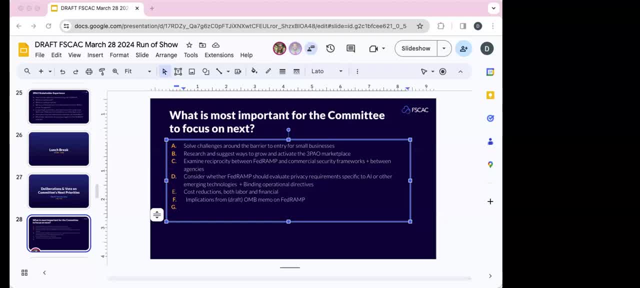 necessarily. you know raise their hand and do that, but and do that, but and do that, but um. you know having the people who do um. you know having the people who do um. you know having the people who do things really well, things really well, things really well. you know help those folks that don't. 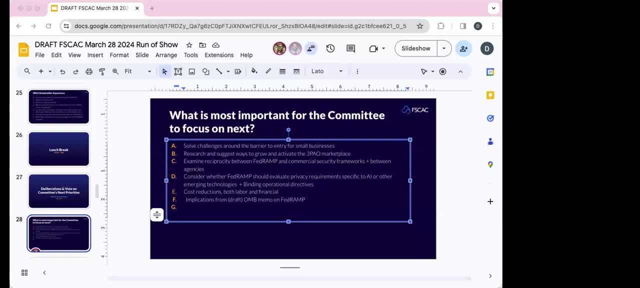 you know, help those folks that don't. you know, help those folks that don't have the resources. and, and if everyone have the resources, and and if everyone have the resources, and and if everyone puts a, you know a person in the mix puts a. you know a person in the mix. 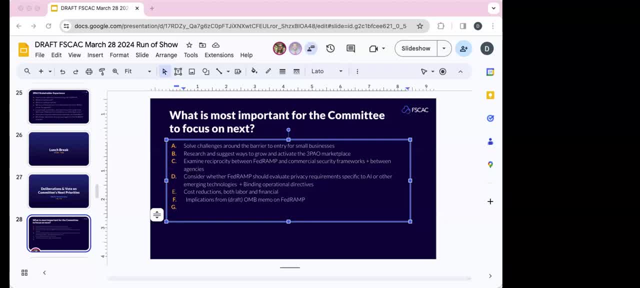 puts a you know a person in the mix. um, you know you only need four to five. um, you know you only need four to five. um, you know you only need four to five people, maybe to do a bunch of people, maybe to do a bunch of people, maybe to do a bunch of assessments. so 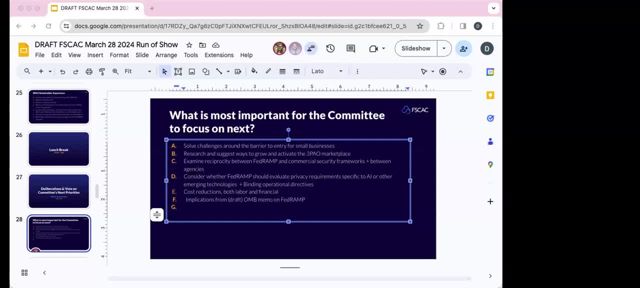 assessments, so assessments so um. i think i'd like to see um that um. i think i'd like to see um that um. i think i'd like to see um that incorporated in some way, um with the incorporated in some way, um with the incorporated in some way, um with the lazy liaison program. that's kind of. 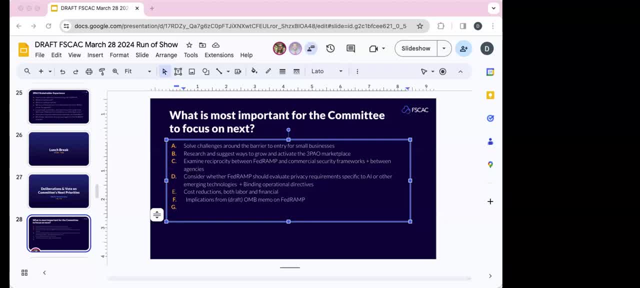 lazy liaison program. that's kind of lazy liaison program that's kind of already in existence, okay. so it sounds like the bed ramp. okay, so it sounds like the bed ramp. okay, so it sounds like the bed ramp. team has a plan. the plan is in process. team has a plan. the plan is in process. 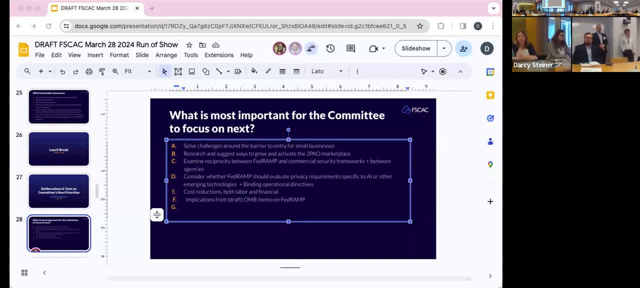 team has a plan. the plan is in process. we will all be hearing more about the. we will all be hearing more about the. we will all be hearing more about the plan as it's developed. plan as it's developed, plan as it's developed. yeah, yeah, yeah, but i think the barriers for one is: 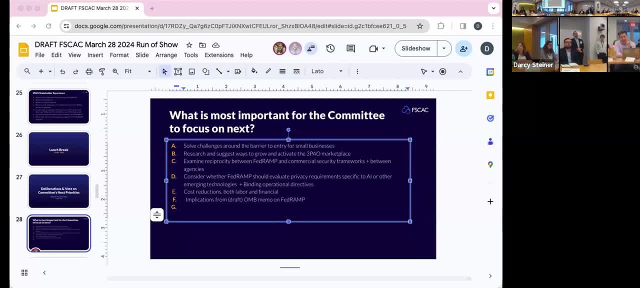 but i think the barriers for one is, but i think the barriers for one is right, but the barriers shouldn't be right, but the barriers shouldn't be right, but the barriers shouldn't be spec. i think what we're hearing right now- spec. i think what we're hearing right now. 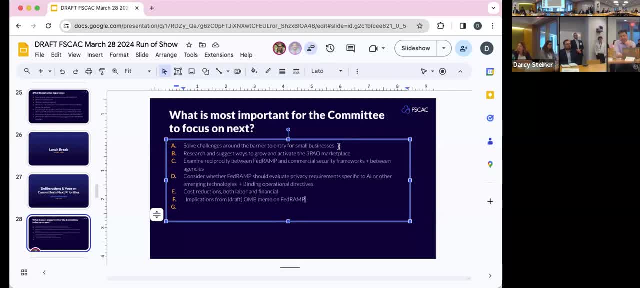 spec. i think what we're hearing right now is that the barriers are not just. is that the barriers are not just, is that the barriers are not just specific small business, specific small business, specific small business. there are barriers for you know. there are barriers for you know. 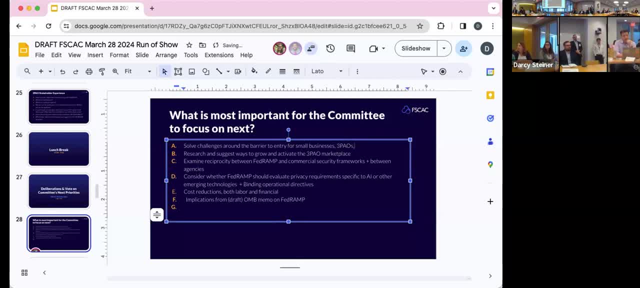 there are barriers for, you know, repows, repows, repows in terms of expanding the market, that, in terms of expanding the market, that in terms of expanding the market that aligns with the other, aligns with the other, aligns with the other priorities, and then there's barriers for 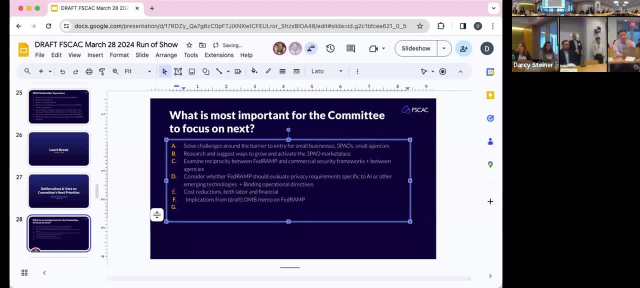 priorities, and then there's barriers for priorities, and then there's barriers for small agencies as well as larger, small agencies as well as larger, small agencies as well as larger agencies, particularly in terms of agencies, particularly in terms of agencies, particularly in terms of stepping up their facilities, and. 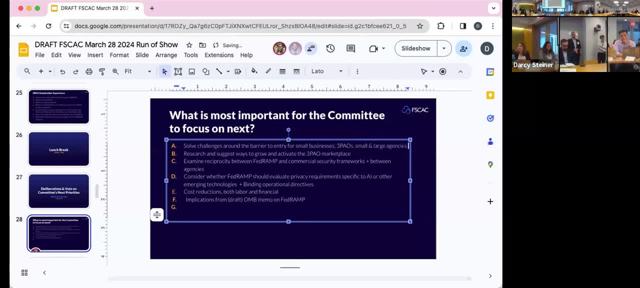 stepping up their facilities and stepping up their facilities. and sponsorships, sponsorships, sponsorships. uh, you know one thing i should add you. uh, you know one thing, i should add you. uh, you know one thing i should add, you know, to carol's point: we've engaged with 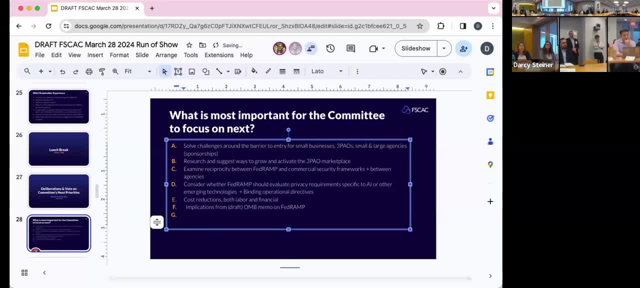 know to carol's point, we've engaged with know to carol's point, we've engaged with omb, omb, omb, ba, uh, you know hhs ba, uh, you know, hhs ba, uh, you know hhs cms, to really look at exploring this. 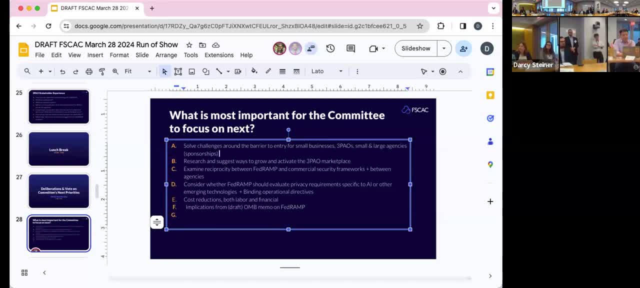 cms to really look at exploring this cms. to really look at exploring this joint agency authorization concept. joint agency authorization concept. joint agency authorization concept: uh between our respective agencies. have uh between our respective agencies. have uh between our respective agencies. have similar cloud stacks, if you will. and 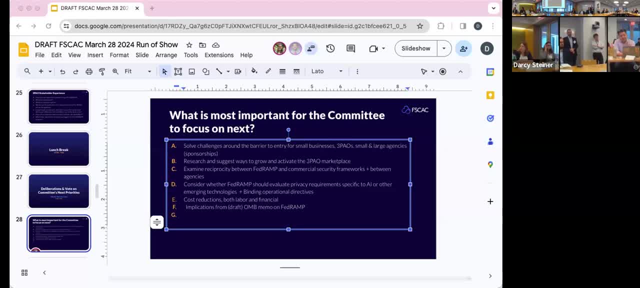 similar cloud stacks, if you will, and similar cloud stacks, if you will, and similar approaches to development, just to similar approaches to development, just to similar approaches to development. just to see if there is, see if there is, see if there is a set of cloud service providers with. 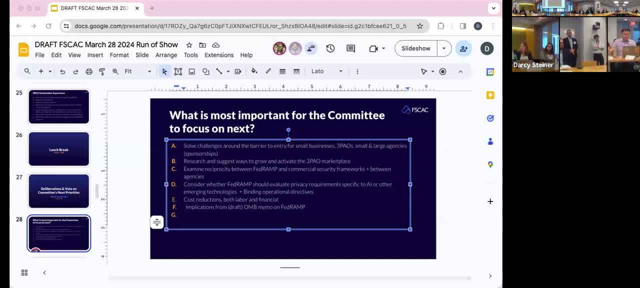 a set of cloud service providers with a set of cloud service providers with respect to our agencies, respect to our agencies, respect to our agencies, where, where, where you know there might be a sharing of you know there might be a sharing of you know there might be a sharing of that workload, to facilitate either a 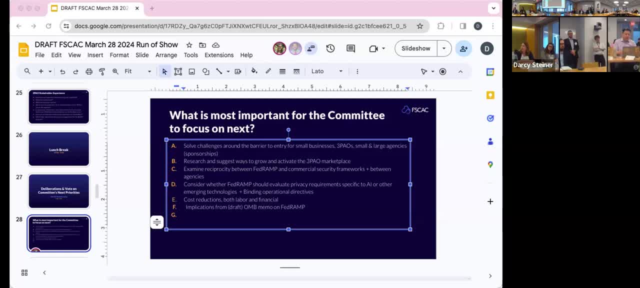 that workload to facilitate, either a that workload to facilitate either a joint authorization between the joint authorization between the joint authorization between the respective agencies, or perhaps to go respective agencies, or perhaps to go respective agencies, or perhaps to go through and say through and say through and say, in the aggregate, this triumvirate, if you. 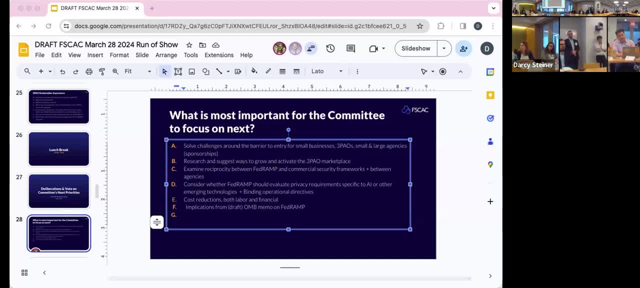 in the aggregate, this triumvirate, if you, in the aggregate, this triumvirate, if you will might have maybe a dozen cloud, will might have maybe a dozen cloud will might have maybe a dozen cloud service providers that are of need. service providers that are of need. 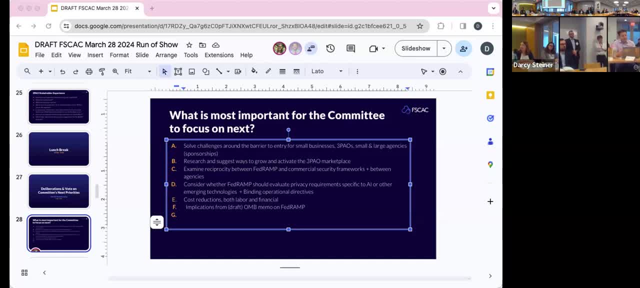 service providers that are of need. and, individually, we work to develop, and individually, we work to develop, and individually, we work to develop a common rubric, a common rubric, a common rubric. common set of principles in terms of show. common set of principles in terms of show. 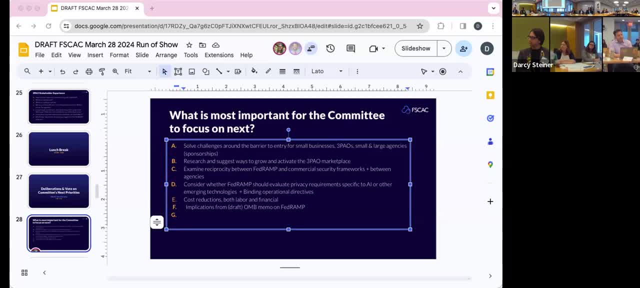 common set of principles in terms of show stoppers that might preclude an stoppers, that might preclude an stoppers, that might preclude an authorization, and then divvy up the work- authorization, and then divvy up the work authorization, and then divvy up the work with respect to our agencies, just to be. 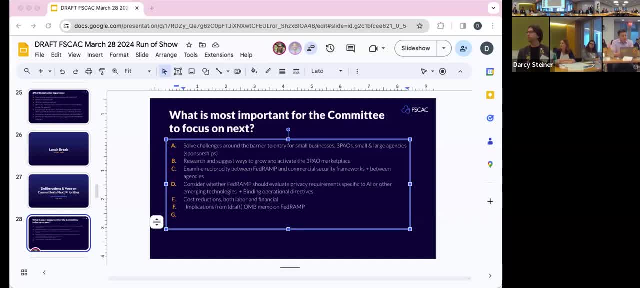 with respect to our agencies, just to be with respect to our agencies, just to be able to leverage one another, able to leverage one another, able to leverage one another, including our existing resources, to be including our existing resources, to be including our existing resources, to be able to get further. 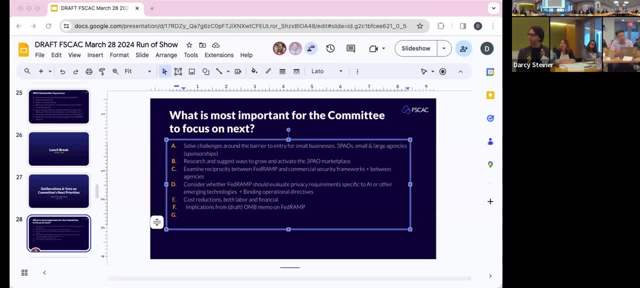 able to get further. able to get further. you know better together, and so i think you know better together, and so i think you know better together, and so i think there are some things that are happening. there are some things that are happening. there are some things that are happening particularly around exploring this joint. 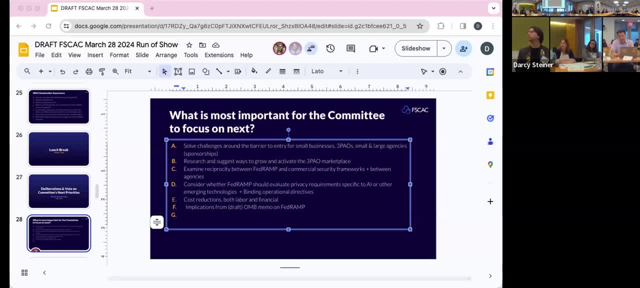 particularly around exploring this joint, particularly around exploring this joint agency authorization concept, agency authorization concept. agency authorization concept. that is going to be helpful, but it will. that is going to be helpful, but it will. that is going to be helpful, but it will take some time. take some time. 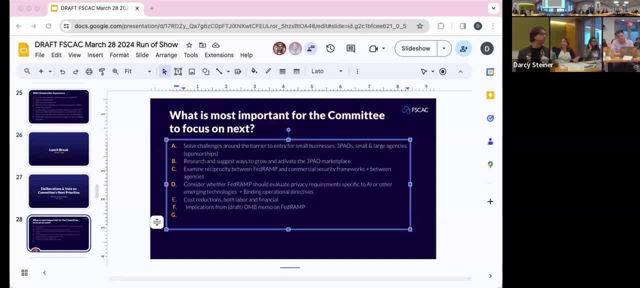 take some time. thank you, thank you, thank you. so the richness of that discussion, so the richness of that discussion, so the richness of that discussion suggests omb memo, suggests omb memo. suggests omb memo is a topic that could be a major, is a topic that could be a major. 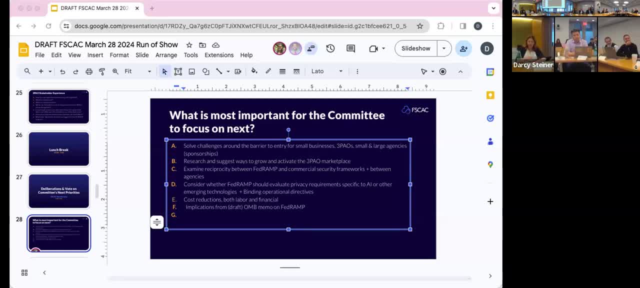 is a topic that could be a major priority, priority, priority, um, in the time that we have. are there, um, in the time that we have, are there are other priorities that are coming to? are other priorities that are coming to, are other priorities that are coming to the forefront? and i also just wanted to the forefront and i also just wanted to the forefront and i also just wanted to say- i've heard the feedback here- that we say, i've heard the feedback here, that we say, i've heard the feedback here- that we need to make sure that our 2023. 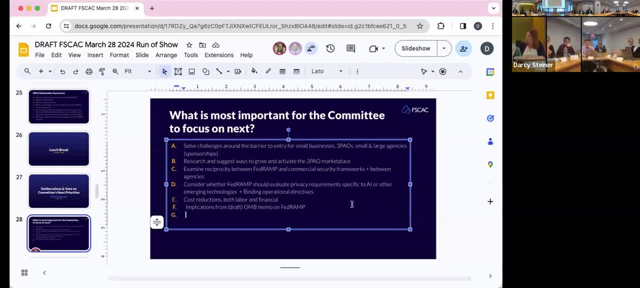 need to make sure that our 2023 need to make sure that our 2023 initiatives also, initiatives, also, initiatives also- are carried through. that that's going to are carried through. that that's going to are carried through. that that's going to be happening, be happening. 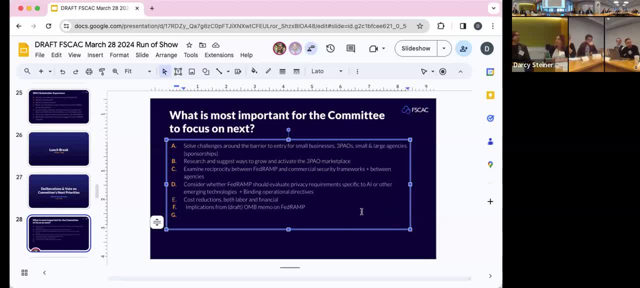 be happening. the federal team is actively working on. the federal team is actively working on. the federal team is actively working on that. but i agree that we should that, but i agree that we should that, but i agree that we should continue to get updates and provide. continue to get updates and provide. 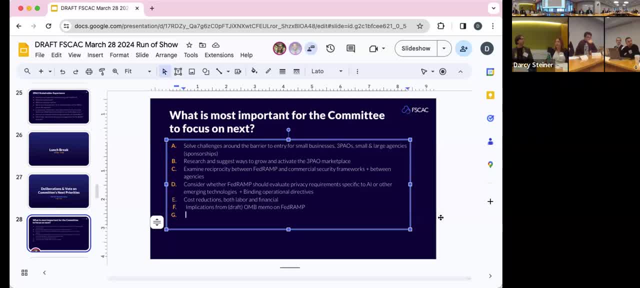 continue to get updates and provide feedback, feedback, feedback. i also agree that a lot of the things. i also agree that a lot of the things. i also agree that a lot of the things that are in that list are table stakes. that are in that list are table stakes. 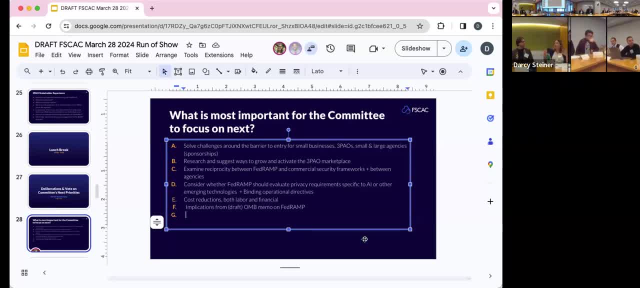 that are in that list are table stakes, but i want to encourage us to think, but i want to encourage us to think, but i want to encourage us to think iteratively about, iteratively about, iteratively about engaging with feedback for the grant. engaging with feedback for the grant. 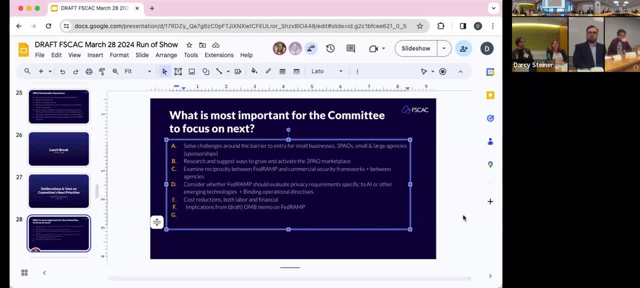 engaging with feedback for the grant team. that works to be ongoing, but it's team that works to be ongoing. but it's team that works to be ongoing, but it's not like, not like, not like. they're starting the process of doing. they're starting the process of doing. 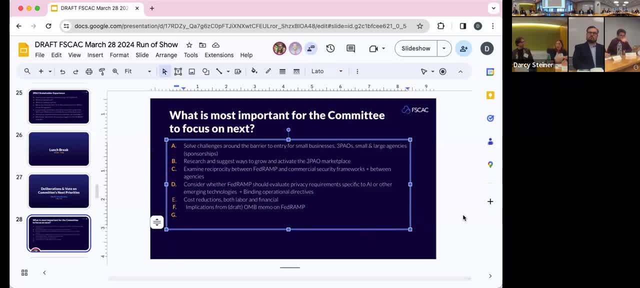 they're starting the process of doing that work. we'll work in a. you know that work. we'll work in a. you know that work. we'll work in a you know uh on it without any outside input, or uh on it without any outside input, or uh on it without any outside input or feedback, and then we'll be done at a. feedback, and then we'll be done at a feedback and then we'll be done at a certain point. they're going to work certain point. they're going to work certain point. they're going to work iteratively. they're going to communicate iteratively, they're going to communicate. 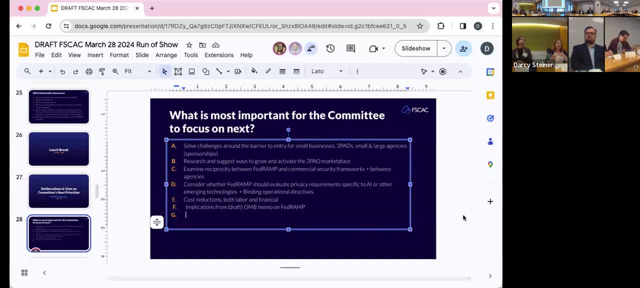 iteratively. they're going to communicate their progress iteratively, and so their progress iteratively, and so their progress iteratively, and so there'll be multiple checkpoints that we, there'll be multiple checkpoints that we, there'll be multiple checkpoints that we and other stakeholders can use to provide. 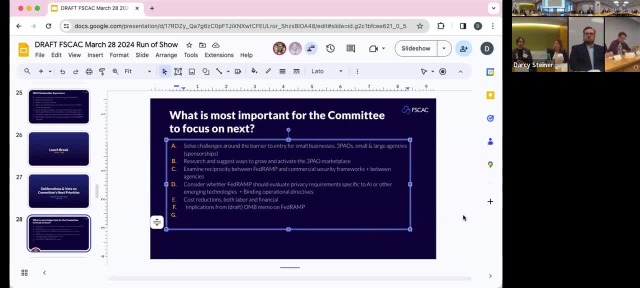 and other stakeholders can use to provide, and other stakeholders can use to provide feedback. so i think there are ways feedback. so i think there are ways feedback. so i think there are ways to like hold the line on those things. to like hold the line on those things. 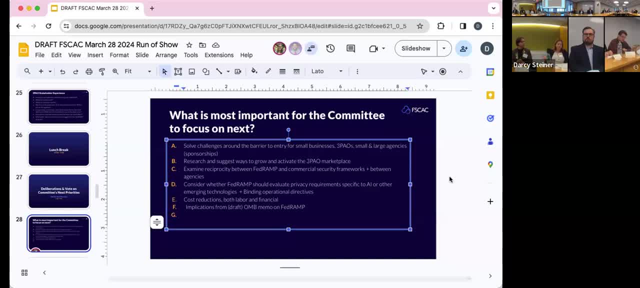 to like hold the line on those things being table stakes that also provide being table stakes, that also provide being table stakes that also provide feedback. and i think there's a risk of feedback, and i think there's a risk of feedback and i think there's a risk of us if we just say we're just going to. 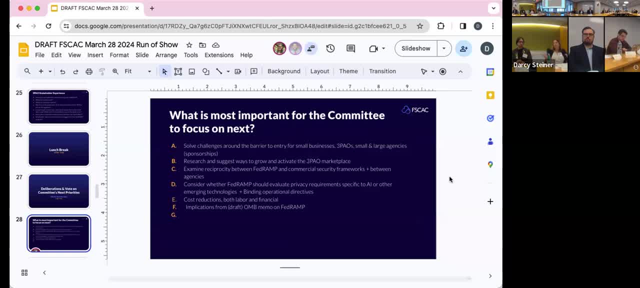 us if we just say we're just going to us, if we just say we're just going to monitor what we told them to do last, monitor what we told them to do last monitor what we told them to do last year, that we'll miss the industry will. 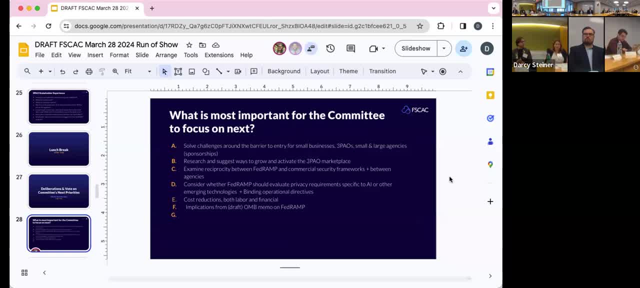 year that we'll miss the industry will year that we'll miss the industry will move out from under us when it comes to move out from under us, when it comes to move out from under us when it comes to things like emerging technology generative things like emerging technology generative. 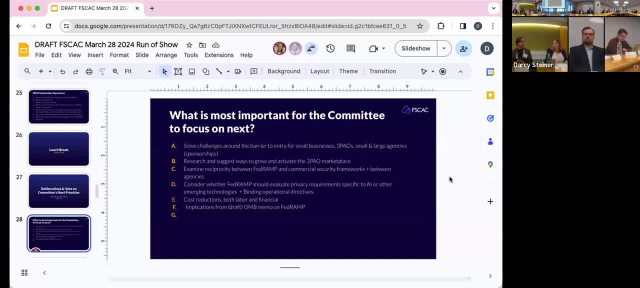 things like emerging technology, generative ai large language models, etc. so ai large language models etc. so ai large language models, etc. so, um. so i just want to encourage us to um. so i just want to encourage us to um. so i just want to encourage us to consider additional priorities. 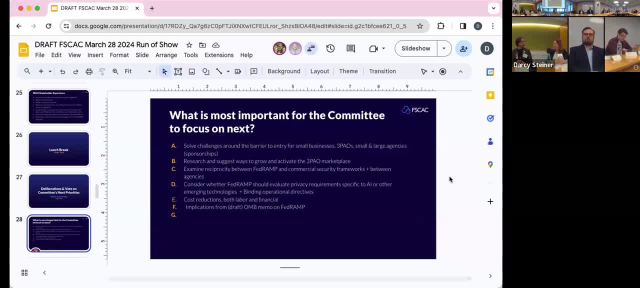 consider additional priorities. consider additional priorities interleaved into. interleaved into. interleaved into discussions about monitoring. against the discussions about monitoring. against the discussions about monitoring. against the table stakes goals. we identified last table stakes goals. we identified last table stakes goals. we identified last year year year. we have a virtual uh henry's from. 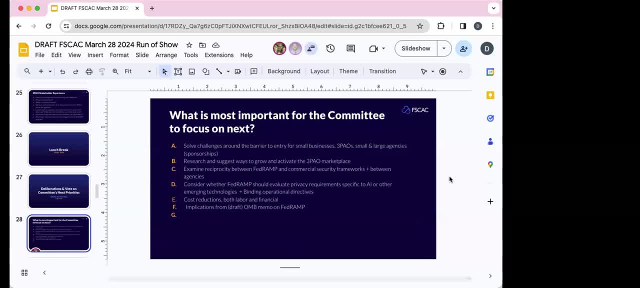 we have a virtual uh henry's from. we have a virtual uh henry's from lomond lomond, lomond. go ahead, hi lamont hhs. go ahead, hi lamont hhs, go ahead, hi lamont hhs. agree with many of the points. one: 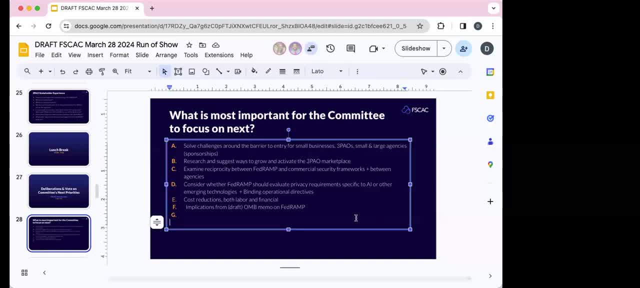 agree with many of the points. one agree with many of the points. one additional one that i might offer, just additional one that i might offer, just additional one that i might offer, just based upon the feedback i get, based upon the feedback i get based upon the feedback i get, the variety of discussions i have within. 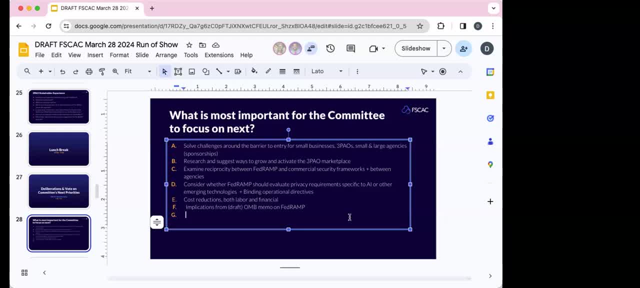 the variety of discussions i have within, the variety of discussions i have within my sizzle council, my sizzle council, my sizzle council, of course we can all appreciate, you know. of course we can all appreciate, you know, of course we can all appreciate, you know, the diversion pass that you can. 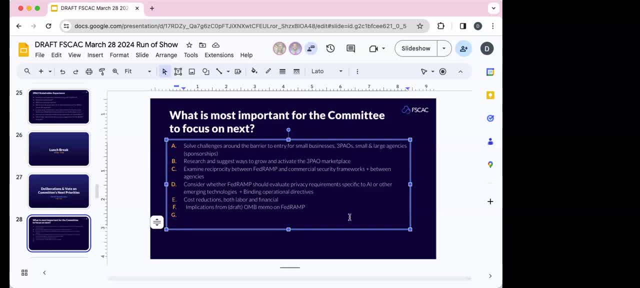 the diversion pass that you can the diversion pass that you can start and finish through the fed ram. start and finish through the fed ram. start and finish through the fed ram. certification process right, and you can certification process right and you can certification process right and you can do a number of things to kind of. 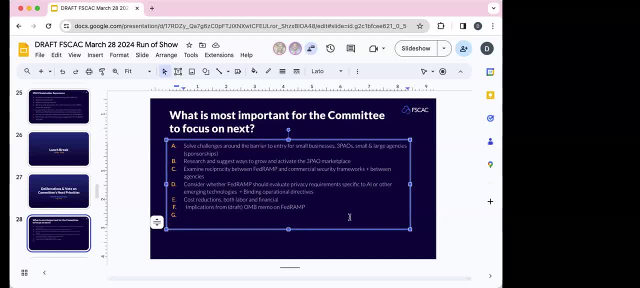 do a number of things to kind of do a number of things to kind of accelerate that process. but even, even if accelerate that process, but even, even if accelerate that process, but even even if you can take advantage of things that you can take advantage of things that 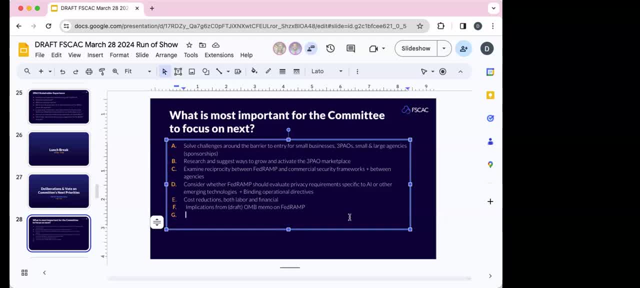 you can take advantage of things that accelerates that process. you're still accelerates that process. you're still accelerates that process. you're still looking at roughly a 12 to 18 month, looking at roughly a 12 to 18 month, looking at roughly a 12 to 18 month window. so i think i would just offer if 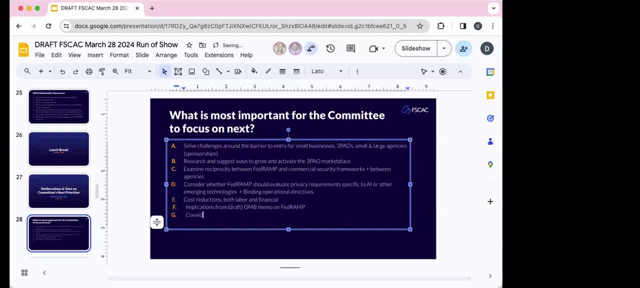 window, so i think i would just offer. if window, so i think i would just offer. if there's anything we could even do to there's anything we could even do to. there's anything we could even do to consider, consider, consider this work um, the longer it's in a queue. 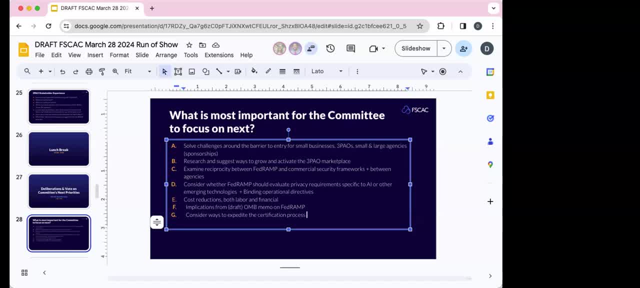 this work um. the longer it's in a queue, this work um. the longer it's in a queue, the more you know, the more resources it, the more you know, the more resources it, the more you know, the more resources it takes. and i would just simply offer to: 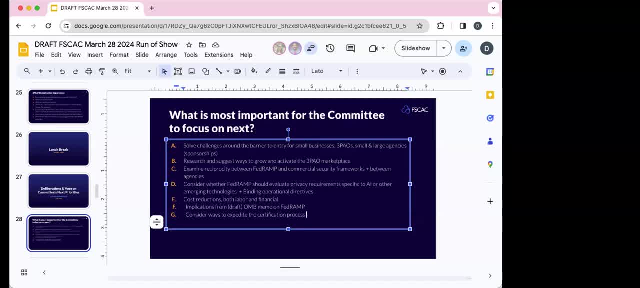 takes, and i would just simply offer to takes, and i would just simply offer to the extent that we can kind of discern, the extent that we can kind of discern, the extent that we can kind of discern ways in which we can even reduce that, ways in which we can even reduce that. 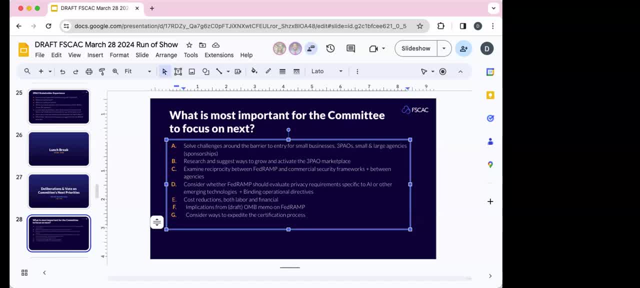 ways in which we can even reduce that timeline would be of great benefit. all right, we've got jackie and limbo. all right, we've got jackie and limbo. all right, we've got jackie and limbo. jack's not because. so the only things i 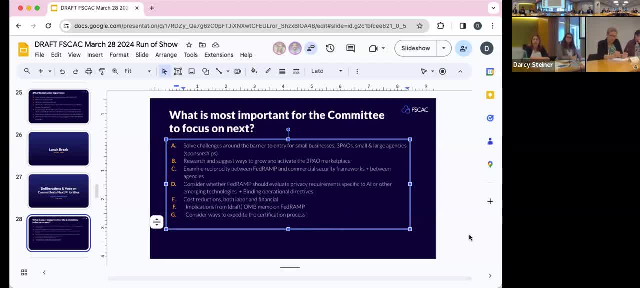 jack's not because, so the only things i jack's not because, so the only things i kept hearing was we need an agile. kept hearing was we need an agile. kept hearing was we need an agile methodology to publish guidance methodology, to publish guidance methodology, to publish guidance to address community needs. 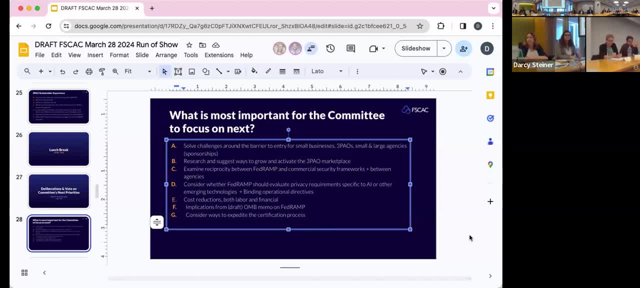 to address community needs. to address community needs, whether that's three po's authorizing, whether that's three po's authorizing, whether that's three po's authorizing agencies, agencies, agencies. examples we had were poems and examples we had were poems and examples we had were poems. and operational requirements and fips. and 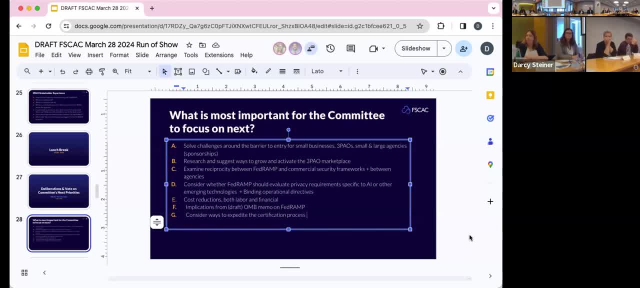 operational requirements and fips, and operational requirements and fips and those types of things, those types of things, those types of things, uh, uh, uh, you know, you know, you know, uh listening to uh omb earlier, uh listening to uh omb earlier, uh listening to uh omb earlier. drew made. 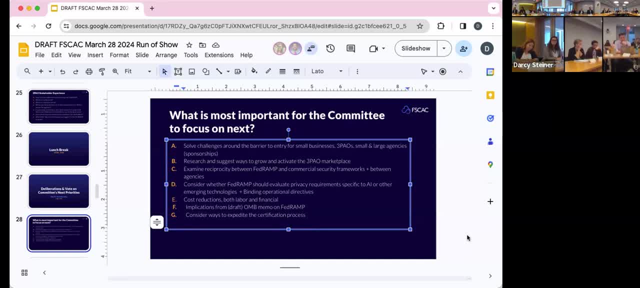 drew made, drew made, uh three, uh three, uh three, three points. one was the barriers to three points. one was the barriers to three points. one was the barriers to entry for small business between entry for small business, between entry for small business, between expanded and a to cover other. 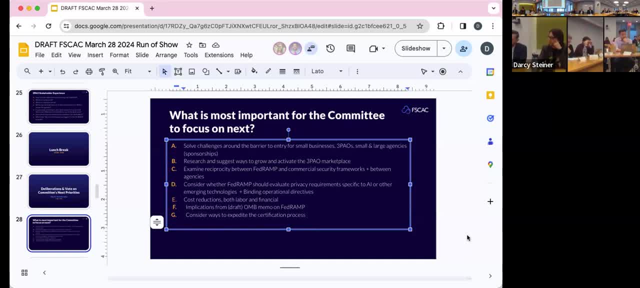 expanded and a to cover other expanded and a to cover other stakeholders, stakeholders, stakeholders. the other two that he mentioned was the. the other two that he mentioned was the. the other two that he mentioned was the cost of veteran, cost of veteran, cost of veteran. i think making sure that we're receptive. 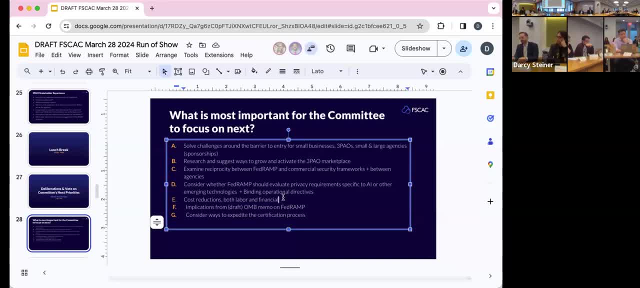 i think making sure that we're receptive, i think making sure that we're receptive to what omb is thinking is important, to what omb is thinking is important, to what omb is thinking is important. then the third was really around the. then the third was really around the. 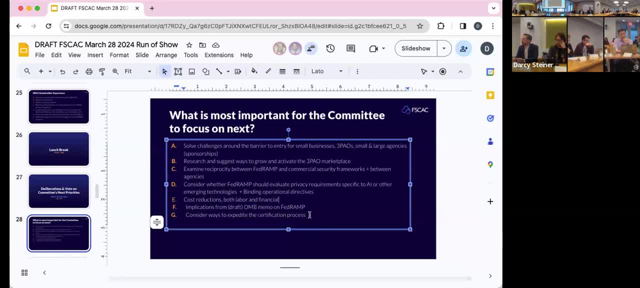 then the third was really around the metrics to be able to track utility and metrics to be able to track utility and effectiveness relative to. i think effectiveness relative to. i think effectiveness relative to. i think, outcomes, outcomes, outcomes. um, i had a couple other ones that, uh, i 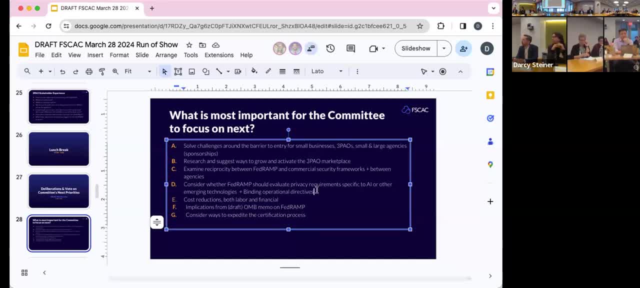 um, i had a couple other ones that, uh, i, um, i had a couple other ones that, uh, i was thinking about, was thinking about, was thinking about, or even when we're talking about finding, or even when we're talking about finding, or even when we're talking about finding operational directives, and 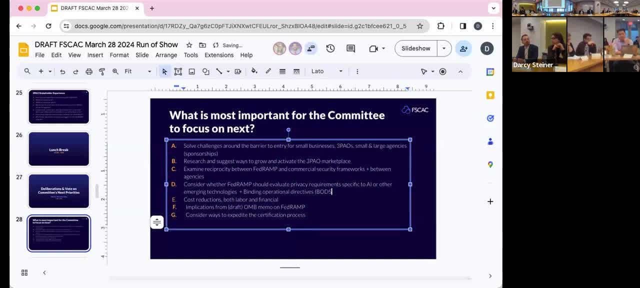 operational directives and operational directives and emerging tech like ai. i don't think it's emerging tech like ai. i don't think it's emerging tech like ai. i don't think it's just exclusive for bots, just exclusive for bots, just exclusive for bots. i think it's really more a matter of 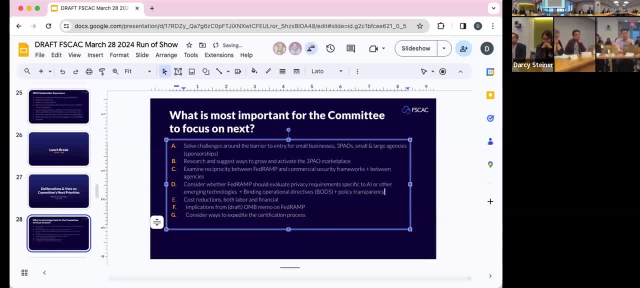 i think it's really more a matter of. i think it's really more a matter of policy: transparency policy, transparency policy, transparency right, particularly around eos m's bots right, particularly around eos, m's bots right, particularly around eos m's bots evs, you name it. particularly relative to 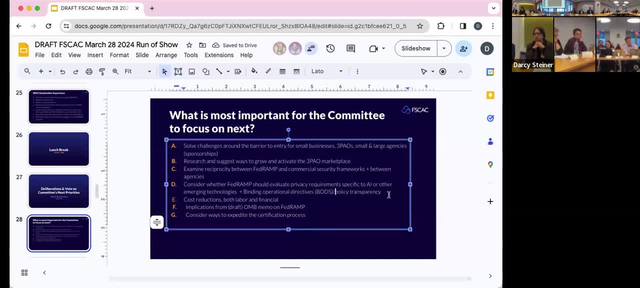 evs. you name it particularly relative to evs. you name it particularly relative to how they impact csps to the federman, how they impact csps to the federman, how they impact csps to the federman, baseline, baseline, baseline. so ensuring that we have a consistent 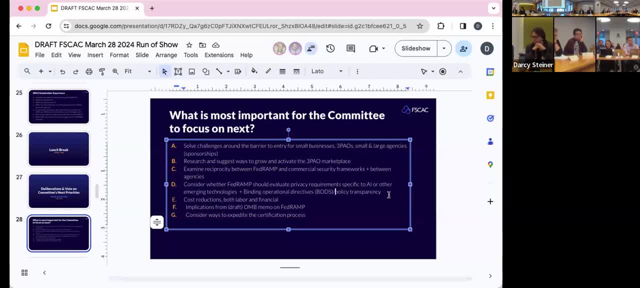 so ensuring that we have a consistent, so ensuring that we have a consistent approach to applicability, approach to applicability, approach to applicability- uh to drive implementation. i think is uh to drive implementation. i think is uh to drive implementation. i think is important, important, important. um, i think those two are related, they are. 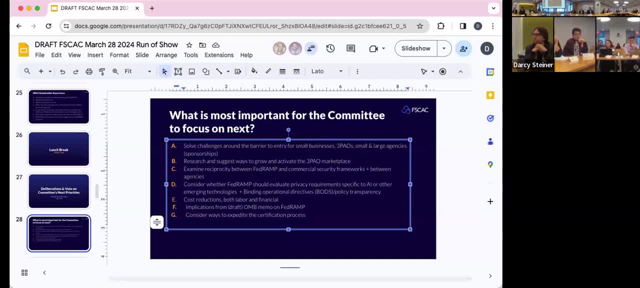 um, i think those two are related. they are, um, i think those two are related. they are to the, to the, to the guidance, guidance, guidance mechanisms. yeah, very, we were hearing our friends from the. we were hearing our friends from the. we were hearing our friends from the three power organization. they're talking. 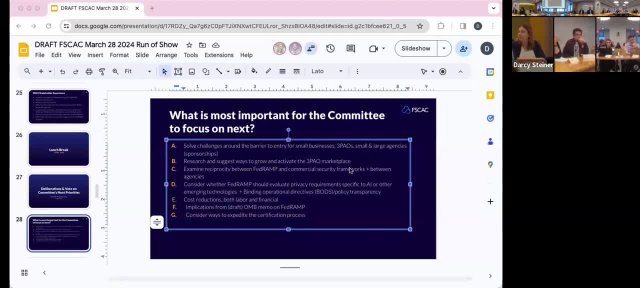 three power organization. they're talking three power organization. they're talking about some barriers, about some barriers, about some barriers or challenges that they were commonly, or challenges that they were commonly or challenges that they were commonly experiencing, experiencing, experiencing. there was mention of boundary scope. there was mention of boundary scope. 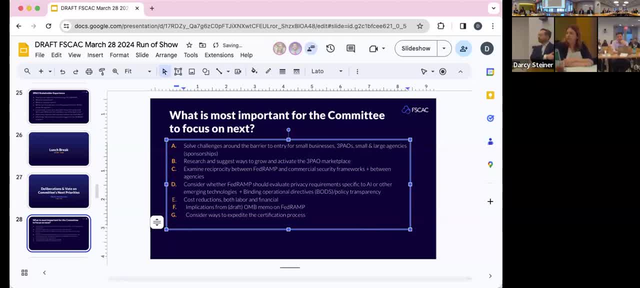 there was mention of boundary scope guidance. there was mention of fifth guidance. there was mention of fifth guidance. there was mention of fifth validation: validation, validation. i think this group could potentially be. i think this group could potentially be. i think this group could potentially be helpful if we tackled that issue head-on. 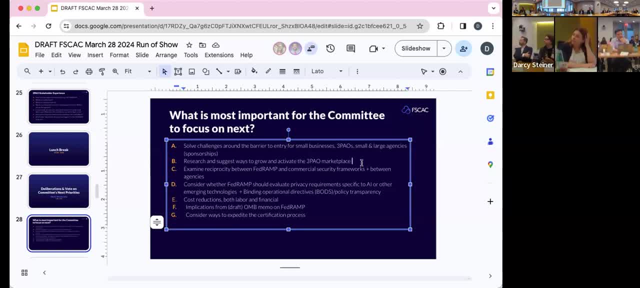 helpful if we tackled that issue head-on. helpful if we tackled that issue head-on, um in terms of providing a common voice, um in terms of providing a common voice, um in terms of providing a common voice through the fs cac, in terms of through the fs cac, in terms of. 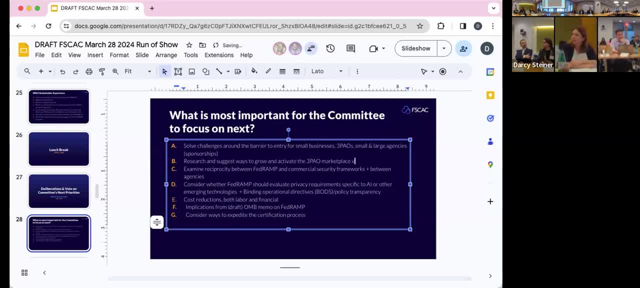 through the fs cac in terms of: uh, you know approach to validating. uh, you know approach to validating. uh, you know approach to validating crypto. not to replace this, not to crypto, not to replace this, not to crypto, not to replace this, not to replace omd, but just to add. 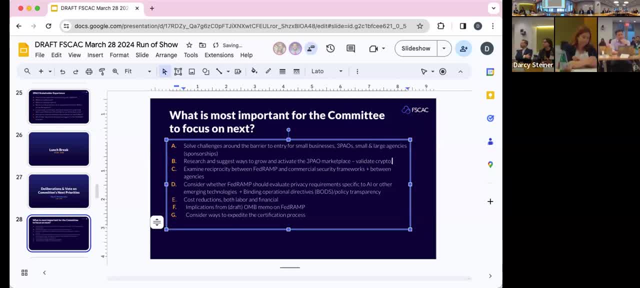 replace omd, but just to add, replace omd, but just to add a voice that reflects both industry, a voice that reflects both industry, a voice that reflects both industry agencies as well as three pounds agencies, as well as three pounds agencies as well as three pounds, uh, in terms of boundary guidance. 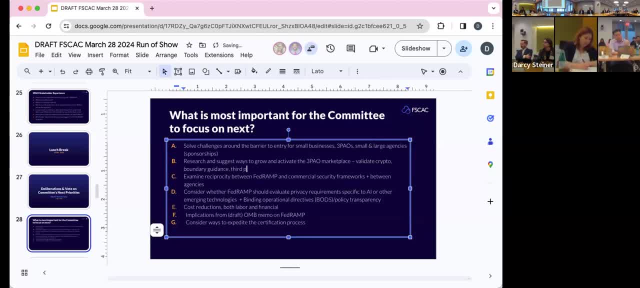 uh, in terms of boundary guidance? uh, in terms of boundary guidance. fifth validation third party. fifth validation, third party. fifth validation third party: integrations api secure. you name it: integrations api secure. you name it. integrations api secure. you name it. the list can go on, but you know just. 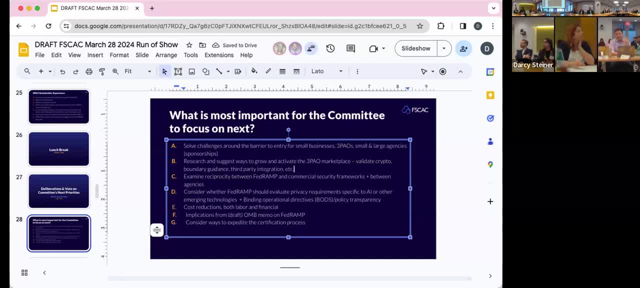 the list can go on, but you know just. the list can go on, but you know just prioritizing on the highest set of risk. prioritizing on the highest set of risk, prioritizing on the highest set of risk areas that tend to preclude, areas that tend to preclude. 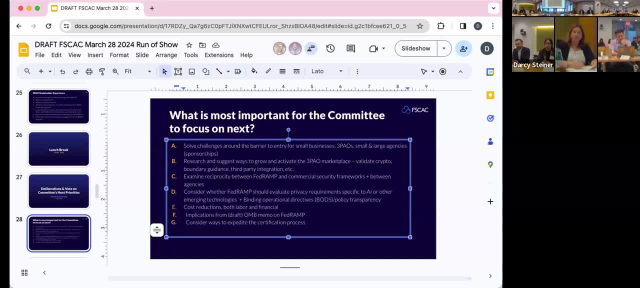 areas that tend to preclude authorizations or prolong authorizations or prolong authorizations or prolong authorization decisions, authorization decisions, authorization decisions, um, and then one last one that i was um, and then one last one that i was um, and then one last one that i was thinking: uh, 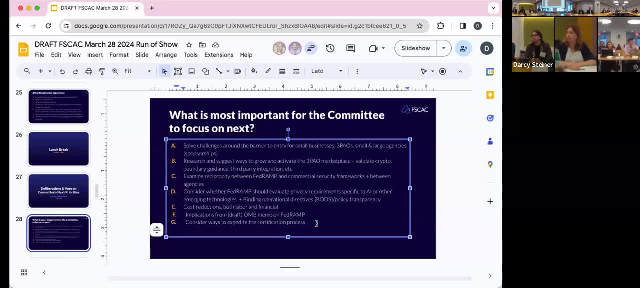 thinking, uh, thinking, uh. you know we mentioned agile like agile. you know we mentioned agile like agile. you know we mentioned agile like agile. authorizations, authorizations, authorizations. right, that might be something for small, right, that might be something for small, right, that might be something for small business in particular, where 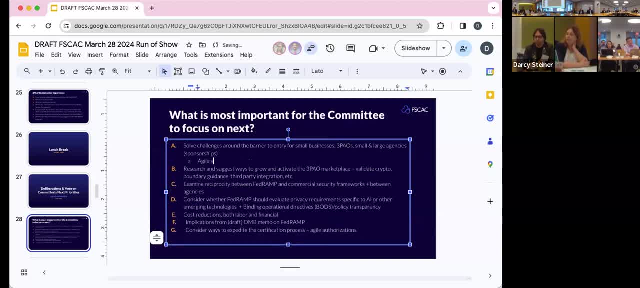 business in particular, where business in particular where it takes 12 months, 18 months. is there a it takes 12 months, 18 months? is there a it takes 12 months, 18 months? is there a step in between where we can issue an, step in between where we can issue an? 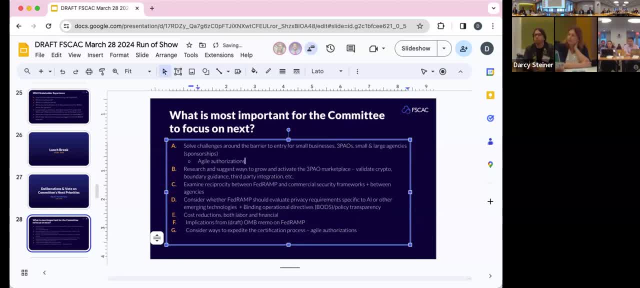 step in between where we can issue an initial authorization to allow initial authorization, to allow initial authorization to allow onboarding, onboarding, onboarding to realize some monetary gain, to be able to realize some monetary gain, to be able to realize some monetary gain, to be able to eventually go through and achieve. 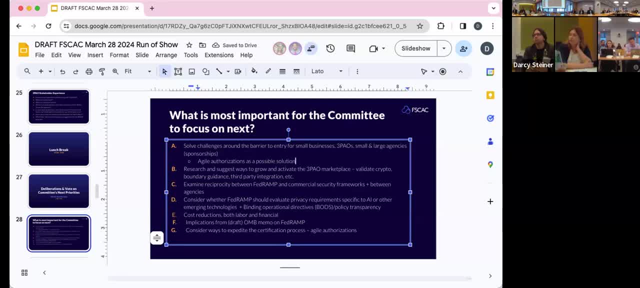 to eventually go through and achieve, to eventually go through and achieve that ultimate veteran authorization, that ultimate veteran authorization, that ultimate veteran authorization, down the line, down the line, down the line, um, and then one thing that we're doing, um, and then one thing that we're doing: 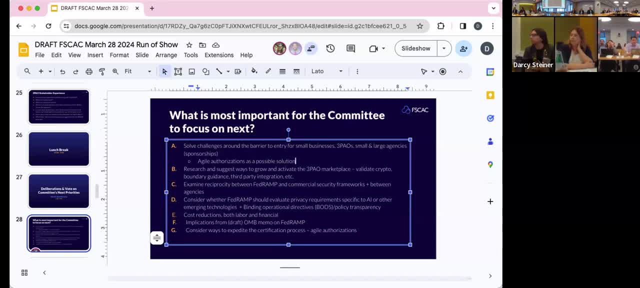 um, and then one thing that we're doing at gsa that i think is important at gsa, that i think is important at gsa. that i think is important: uh, we're engaged in, uh, you know c scrum. uh, we're engaged in, uh, you know c scrum. 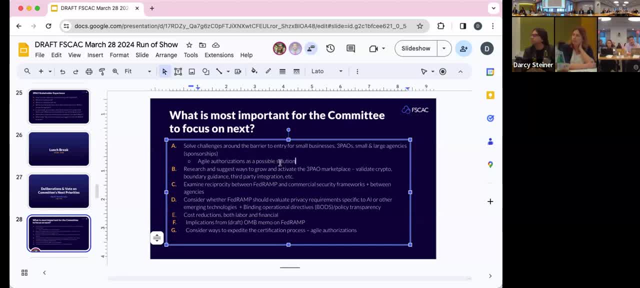 uh, we're engaged in- uh, you know c scrum- vendor risk monitoring, vendor risk monitoring, vendor risk monitoring leveraging. you know industry uh tool leveraging. you know industry uh tool leveraging. you know industry uh tool sets- cloud related tool sets. that sets cloud related tool sets. that sets cloud related tool sets that really focus on identifying vendor. 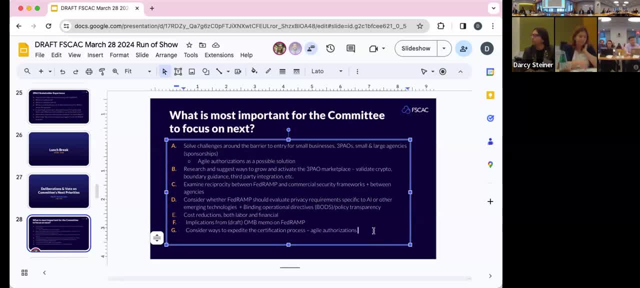 really focus on identifying vendor, really focus on identifying vendor risk, supply chain risk risk, supply chain risk risk, supply chain risk, organizational risks, particularly around organizational risks, particularly around organizational risks, particularly around we're organized where our vendor, we're organized where our vendor we're organized where our vendor solutions are domicile leadership. 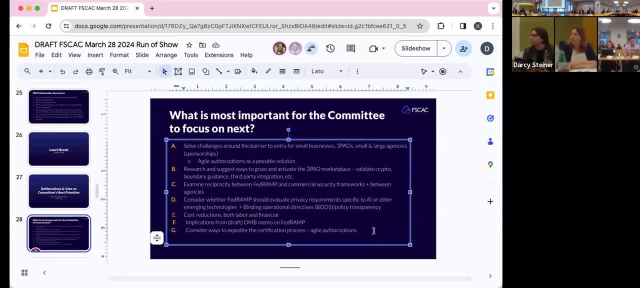 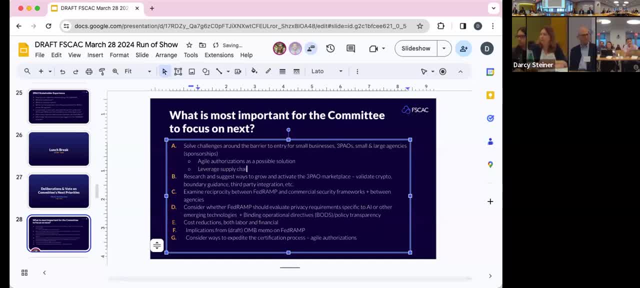 and it's been impactful, at least relative to our usage of gsa, our usage of gsa, our usage of gsa, and it's not corresponding to anything, and it's not corresponding to anything and it's not corresponding to anything within the federated baseline that might. 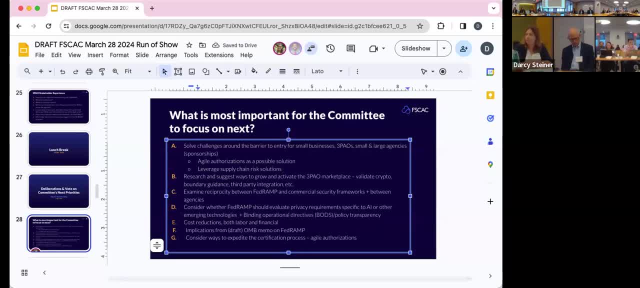 within the federated baseline, that might, within the federated baseline, that might be an opportunity set and ideally be an opportunity set and ideally be an opportunity set and ideally, perhaps, a shared service through system, perhaps a shared service through system, perhaps a shared service through system. um, that was about 100 interesting ideas. 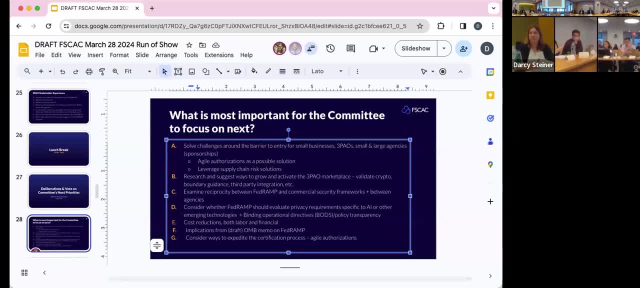 um, that was about 100 interesting ideas. um, that was about 100 interesting ideas trying to still down. if you don't go trying to still down, if you don't go trying to still down, if you don't go ahead- yeah, and i mean pivoting on that, i ahead, yeah, and i mean pivoting on that. i ahead, yeah, and i mean pivoting on that. i think each one of these has a metric think. each one of these has a metric think. each one of these has a metric element to it. right, right, and so you. 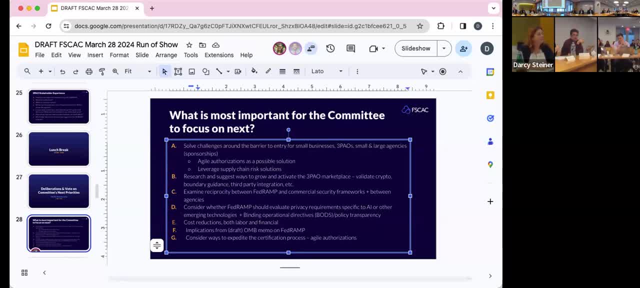 element to it, right, right, and so you element to it, right, right, and so you know a through g, know a through g, know a through g. and then franco said something about, and then franco said something about, and then franco said something about trade, or something might happen. trade or something might happen. trade or something might happen, we'll feel free to interrupt if it. we'll feel free to interrupt if it. we'll feel free to interrupt if it comes back to you. so i'm going to try. comes back to you, so i'm going to try. 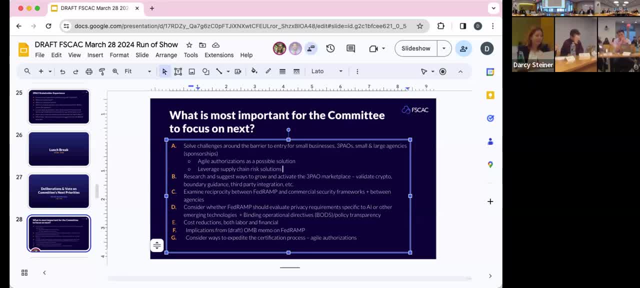 comes back to you. so i'm going to try and distill down some of what we just and distill down some of what we just and distill down some of what we just discussed into priority areas, discussed into priority areas, discussed into priority areas. um, um. 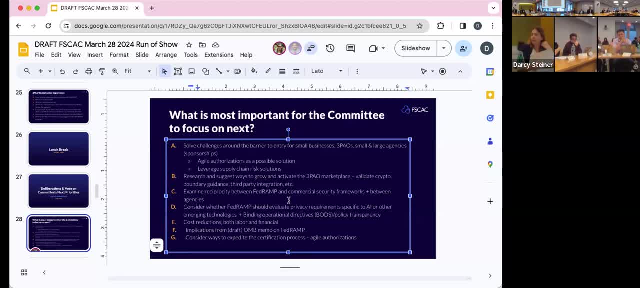 um, so drew from. oob mentioned the need for so drew from. oob mentioned the need for so drew from. oob mentioned the need for metrics. we've also been bringing up the metrics. we've also been bringing up the metrics. we've also been bringing up the idea of metrics and just trying to 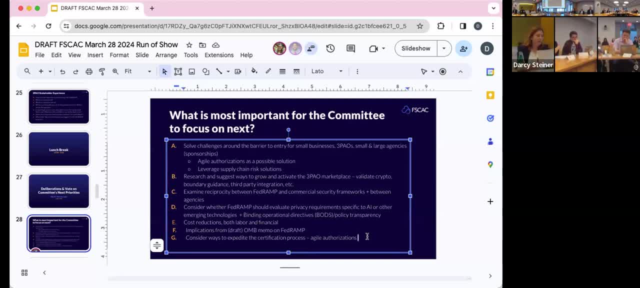 idea of metrics and just trying to idea of metrics and just trying to figure out. how can we track meaningful figure out? how can we track meaningful figure out? how can we track meaningful progress towards existing goals, new progress towards existing goals, new progress towards existing goals, new goals? i wonder if metrics by itself, like 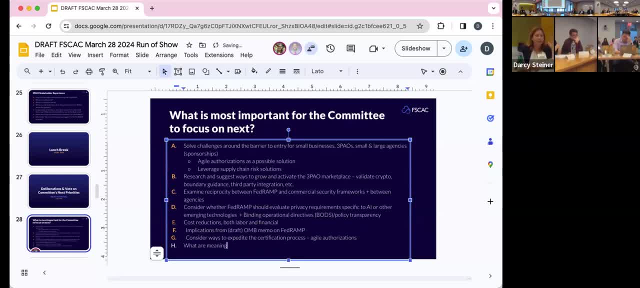 goals. i wonder if metrics by itself like goals. i wonder if metrics by itself like: what are some meaningful metrics to? what are some meaningful metrics to? what are some meaningful metrics to recommend to the bed ramp team, that recommend to the bed ramp team, that recommend to the bed ramp team that incentivize the right kinds of 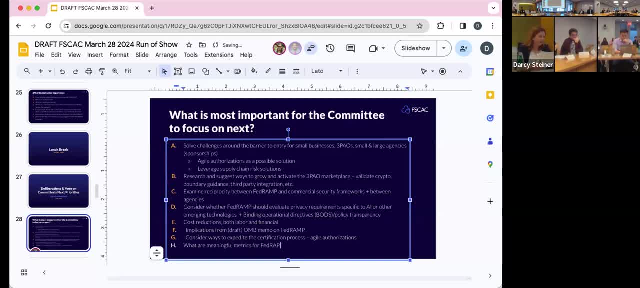 incentivize the right kinds of incentivize the right kinds of prioritization actions from that team, prioritization actions from that team, prioritization actions from that team. that could be an area here, that could be an area here, that could be an area here. um, and then within that we could. 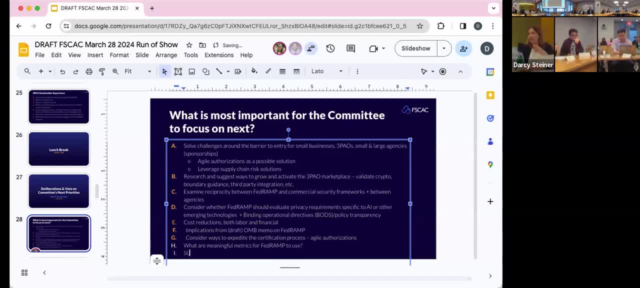 um and then within that we could um and then within that we could potentially discuss things like: are potentially discuss things like. are potentially discuss things like: are there slas for different steps, or there slas for different steps, or there slas for different steps or different? you know methodologies that. 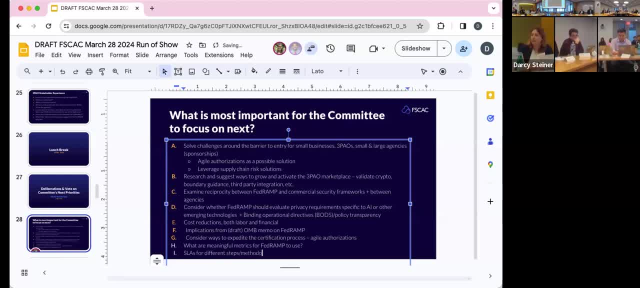 different. you know methodologies that different. you know methodologies that would encourage things like agile. would encourage things like agile. would encourage things like agile practices brought into the authorization practices, brought into the authorization practices, brought into the authorization process. i know the veteran team is process. i know the veteran team is. 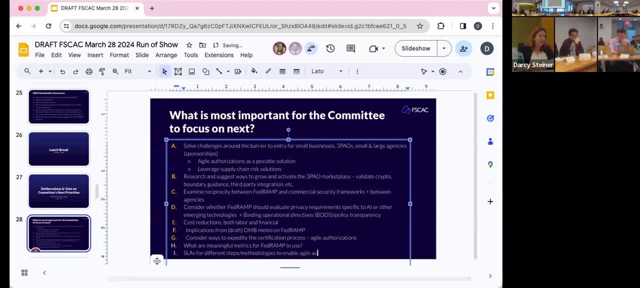 process. i know the veteran team is already based on their roadmap, looking already based on their roadmap, looking already based on their roadmap, looking into agile iterative ways of handling, into agile iterative ways of handling, into agile iterative ways of handling. significant change requests, but we could. significant change requests, but we could. 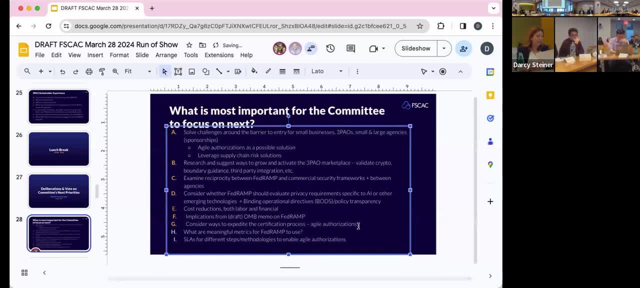 significant change requests. but we could, we could prioritize that within the, we could prioritize that within the. we could prioritize that within the context of a conversation about metrics, context of a conversation about metrics, context of a conversation about metrics: um, um, um. so that's one, so that's one. 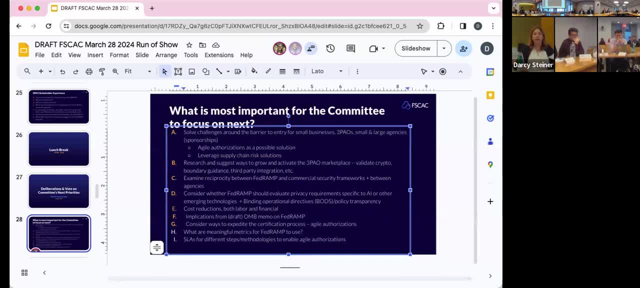 so that's one. yeah. the idea of a knowledge base. that's yeah, the idea of a knowledge base. that's yeah, the idea of a knowledge base that's contributed to by a variety of, contributed to by a variety of, contributed to by a variety of different stakeholder groups. 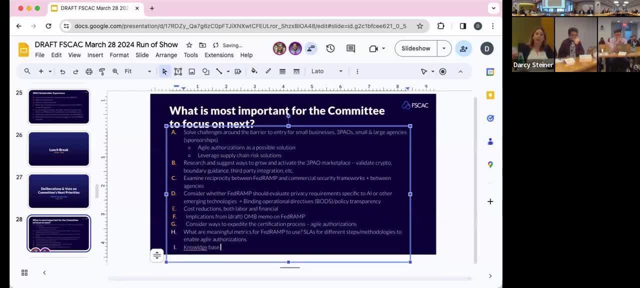 different stakeholder groups, different stakeholder groups in an incrementally updated way with in an incrementally updated way, with in an incrementally updated way, with some ownership, making sure that all the some ownership, making sure that all the some ownership, making sure that all the content is evergreen up to date. 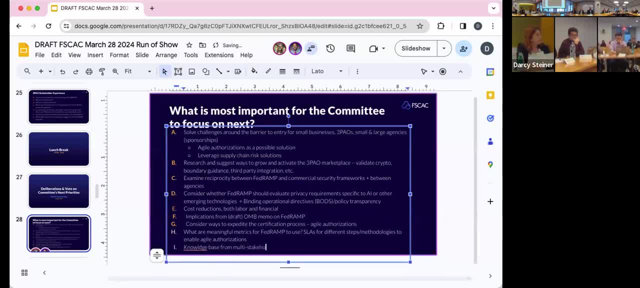 content is evergreen up to date. content is evergreen up to date. something a few of you brought up something. a few of you brought up something a few of you brought up. some knowledge base could be another one. some knowledge base could be another one, some knowledge base could be another one. uh, 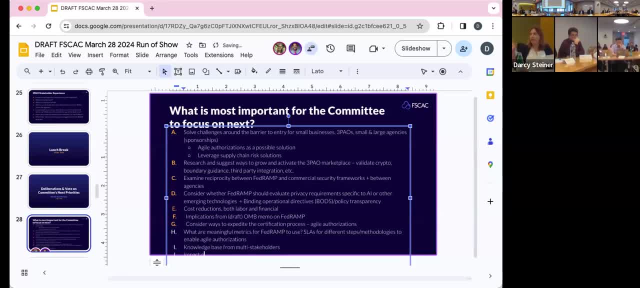 uh uh policy. the impact of policy on policy. the impact of policy on policy. the impact of policy on everything here in terms of like what? everything here in terms of like what. everything here in terms of like what- we're trying to get cloud service. we're trying to get cloud service. 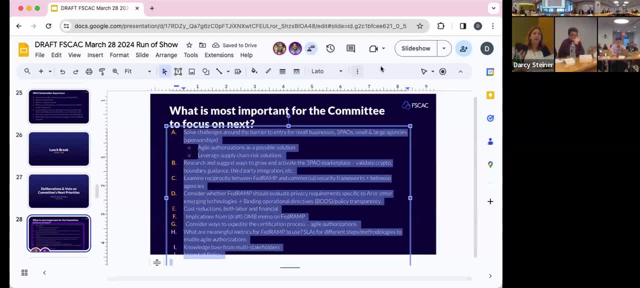 we're trying to get cloud service providers to do through fedramp providers to do through fedramp providers, to do through fedramp authorization in terms of how controls authorization, in terms of how controls authorization, in terms of how controls are structured and updated, are structured and updated. 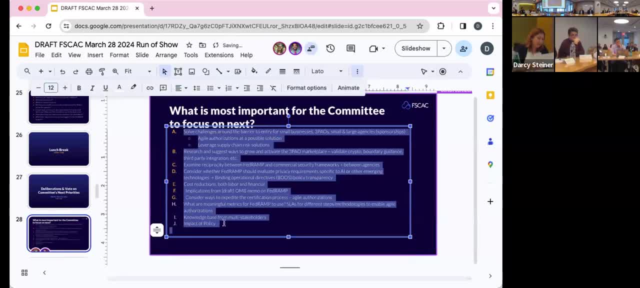 are structured and updated. um, i think bo the way that you just um, i think bo the way that you just um, i think bo the way that you just described, that was making sure that described, that was making sure that described, that was making sure that policy leads to consistent. 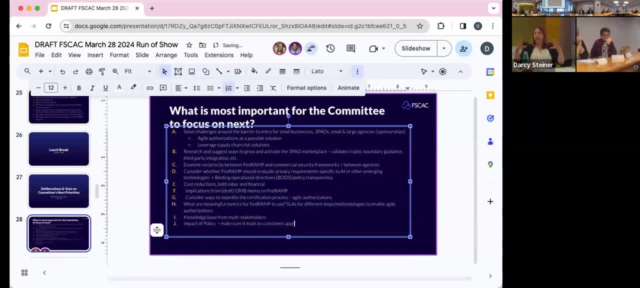 policy leads to consistent policy leads to consistent approach and applicability, approach and applicability, approach and applicability. but maybe, maybe just to pop that up, but maybe, maybe just to pop that up, but maybe, maybe just to pop that up into a category. maybe the impact of 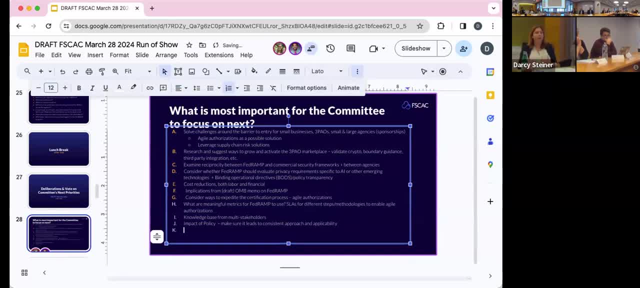 into a category. maybe the impact of policy choices on the implementation policy choices, on the implementation policy choices, on the implementation concerns shared by agencies, cloud service concerns shared by agencies, cloud service concerns shared by agencies, cloud service providers, providers, providers um 3po's could be a category. 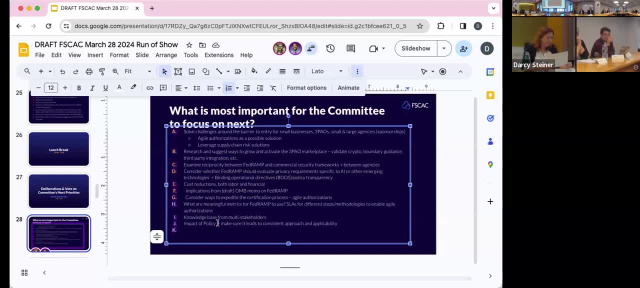 um 3po's could be a category. um 3po's could be a category, so i just put policy there. it's another. so i just put policy there. it's another, so i just put policy there. it's another k and it's and policy boundaries. 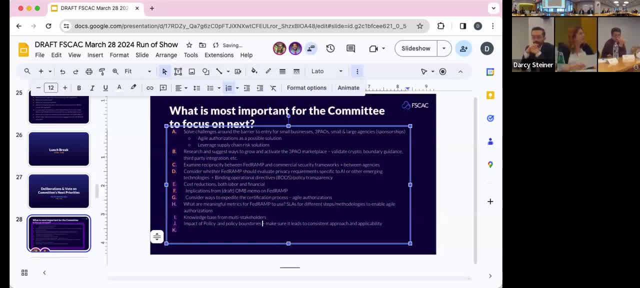 k and it's and policy boundaries- k and it's and policy boundaries. yeah, yeah, yeah, you know, you know, you know, authorities, boundaries, scope, authorities, boundaries, scope, authorities, boundaries, scope. yeah, that's great, yeah, so policy. yeah, that's great, yeah, so policy. yeah, that's great, yeah, so policy colon. 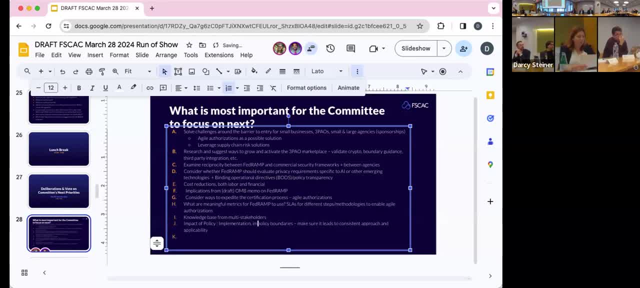 colon, colon implementation implications: boundaries, implementation implications, boundaries, implementation, implications, boundaries, scope, scope, scope, um. and then, like you know so, bo brought um, and then, like you know so, bo brought um, and then, like you know so, bo brought up the vips issue. that's also come up a. 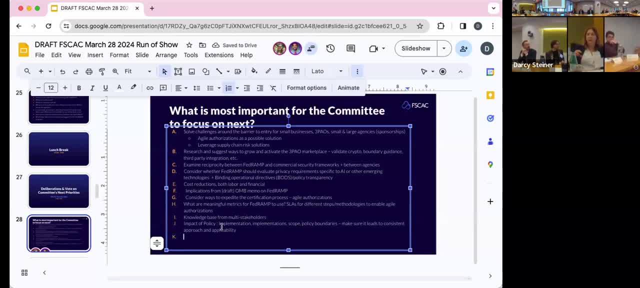 up the vips issue. that's also come up. a up the vips issue. that's also come up a lot over the last six months. i wonder if lot over the last six months. i wonder if lot over the last six months. i wonder if we want to have a category here. that's. 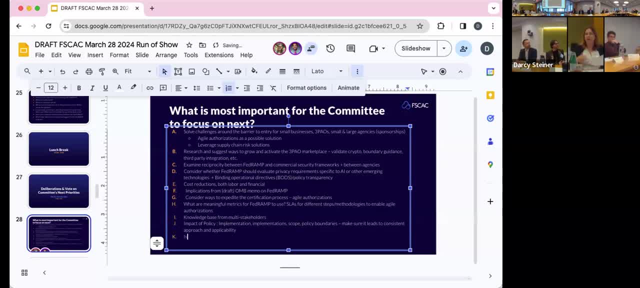 we want to have a category here that's. we want to have a category here that's like issues related to specific controls, like issues related to specific controls, like issues related to specific controls that we know are problematic or that we know are problematic, or that we know are problematic or complicated or expensive in specific ways. 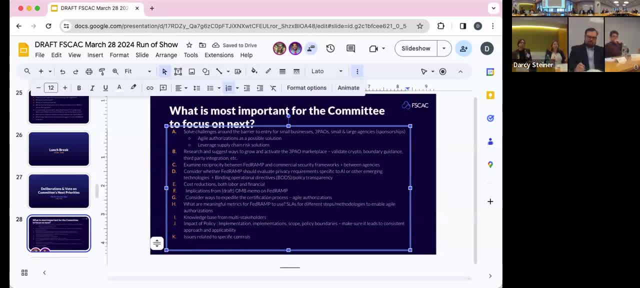 complicated or expensive in specific ways. complicated or expensive in specific ways like: if we want to hold space for like. if we want to hold space for like. if we want to hold space for talking about controls that are having, talking about controls that are having, talking about controls that are having an implication that the ramp team should. 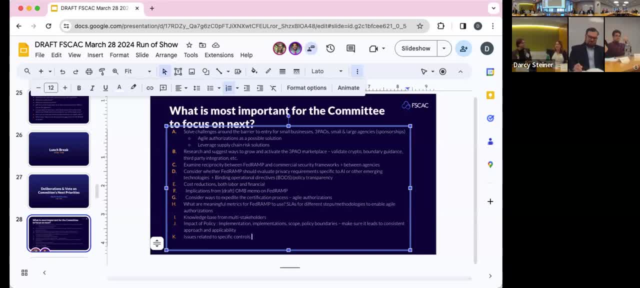 an implication that the ramp team should, an implication that the ramp team should be aware of, be aware of, be aware of. so that's my attempt to, so that's my attempt to, so that's my attempt to summarize the 1 000 great ideas that summarize the 1 000 great ideas that 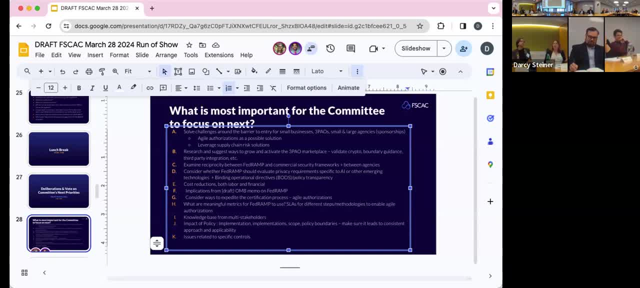 summarize the 1 000 great ideas that you guys have just brought up here. you guys have just brought up here. you guys have just brought up here: uh, now we have a list that's too long. uh, now we have a list that's too long. uh, now we have a list that's too long, so okay, 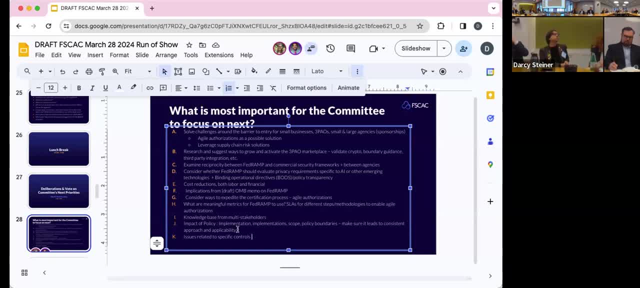 so okay, so okay. isn't j related to? isn't j related to? isn't j related to? uh, uh, uh, sorry d, sorry d, sorry d. could those be merged? could those be merged? could those be merged, sure, yeah, yeah, d could go under g. yeah, he is related to g, sure, and c could. yeah, he is related to g sure and c could. yeah, he is related to g sure and c could be removed. that's the one that's be removed. that's the one that's be removed. that's the one that's duplicative of what's already on the. 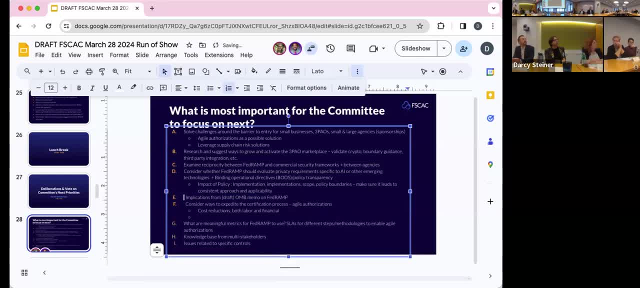 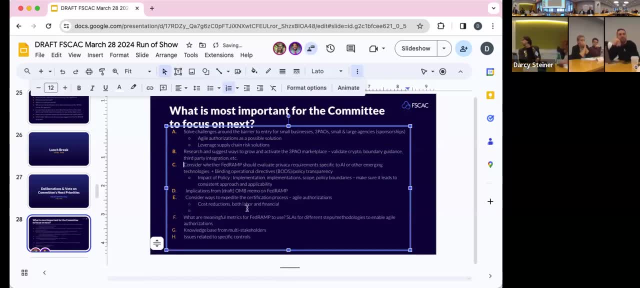 duplicative of what's already on the duplicative of what's already on the roadmap: roadmap, roadmap. great thanks, great thanks, great thanks, which is great, which is great, which is great, great to hear. is there anything you want to? is there anything you want to? is there anything you want to potentially think about it? 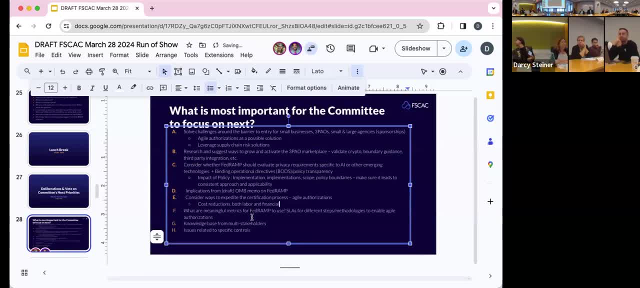 potentially think about it, potentially think about it as a committee on, as a committee on, as a committee on speaking broader with other committees, speaking broader with other committees, speaking broader with other committees or other agencies or other agencies or other agencies in terms of, uh like, aligning on. 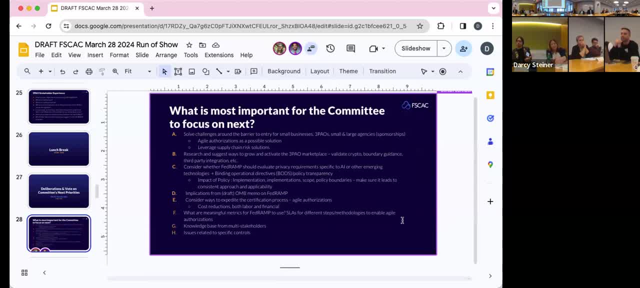 in terms of uh like aligning on, in terms of uh like aligning on controls or controls or controls, or like, like, like, that's that word, that's that word, that's that word: committee reciprocity- like. is there committee reciprocity? like, is there committee reciprocity? like: is there anything? well, is there any like are? 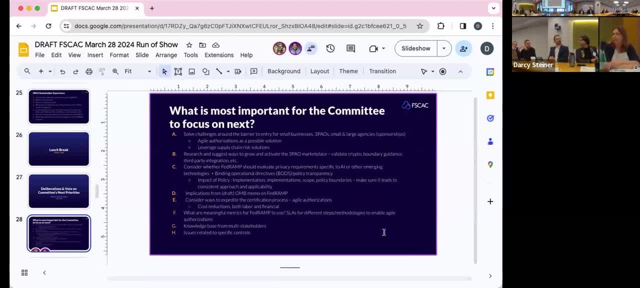 anything well? is there any like? are anything well? is there any like? are there any connective tissues? we should be there? any connective tissues? we should be there? any connective tissues we should be building potentially other like. maybe building potentially other like. maybe building potentially other like, maybe similar to this. i don't know, what do you? 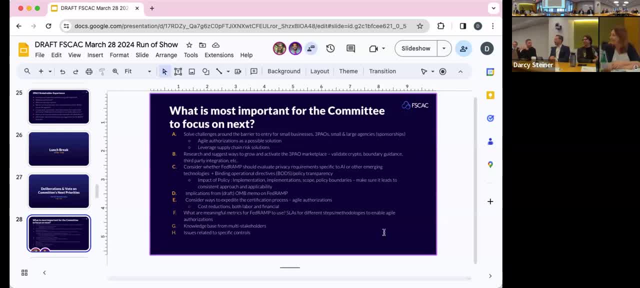 similar to this. i don't know what do you? similar to this. i don't know what do you think? jackie bronco's natural. think jackie bronco's natural. think jackie bronco's natural. i would say rather. i would say rather. i would say rather yeah. 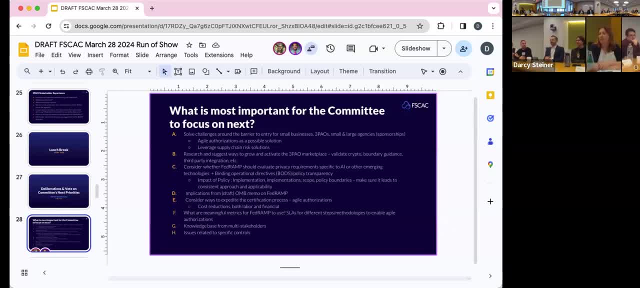 yeah, yeah, i think the parties are, i think the parties are, i think the parties are got it, got it, got it. that's what you want to do. yeah, well, that's what you want to do. yeah well, that's what you want to do. yeah, well, i'm thinking like things, like state. 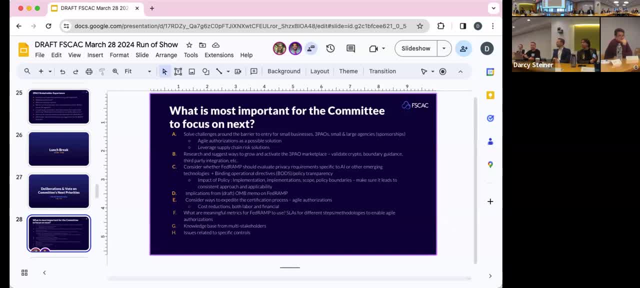 i'm thinking like things like state. i'm thinking like things like state branch things like cmc branch things like cmc, branch things like cmc, like uh, you know like areas like uh, you know like areas like uh, you know like areas a little bit broader maybe, that where 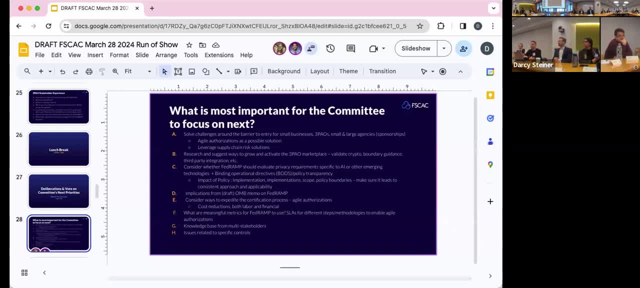 a little bit broader, maybe that where a little bit broader, maybe that where csps we get input from all of these csps. we get input from all of these csps. we get input from all of these different places, different places, different places, like they're a way that we could. 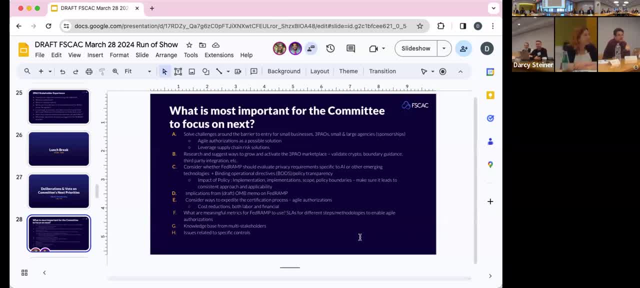 like they're a way that we could, like they're a way that we could potentially integrate, potentially integrate, potentially integrate. yeah, the difficulty is as the board we are. the difficulty is as the board we are. the difficulty is as the board we are not the owner of the construct. 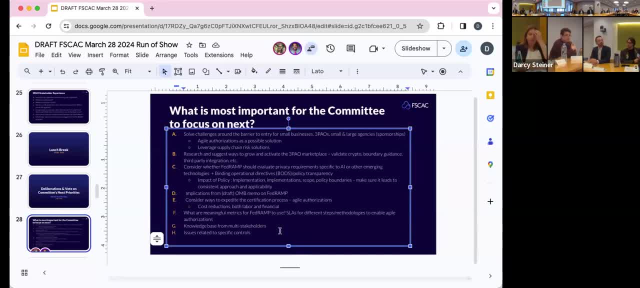 not the owner of the construct, not the owner of the construct. so so, so you know, you know, you know somebody who does a lot of these, somebody who does a lot of these, somebody who does a lot of these mappings exhaustively and exhaustingly. mappings exhaustively and exhaustingly. 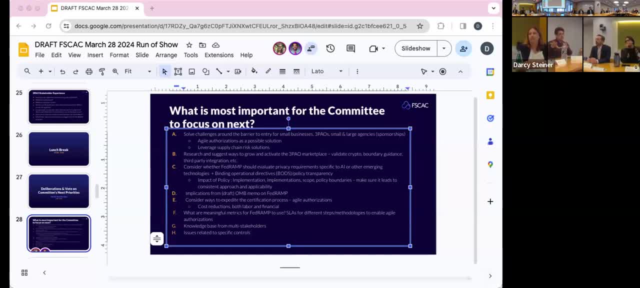 mappings exhaustively and exhaustingly. um, they're great if you are, you know. um they're great if you are, you know. um, they're great if you are, you know, fedramp owns one side of it. so at least fedramp owns one side of it. so at least. 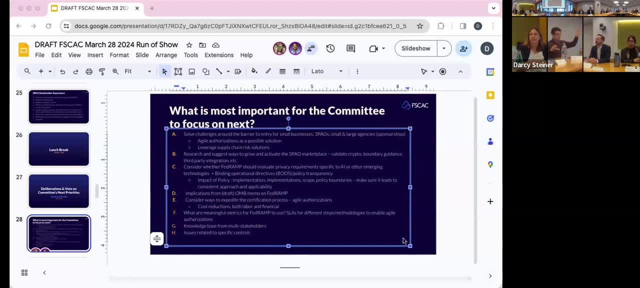 fedramp owns one side of it, so at least it will be a one side map. it's best it will be a one side map. it's best it will be a one side map. it's best, then, if they get the authorized owner of. then if they get the authorized owner of. 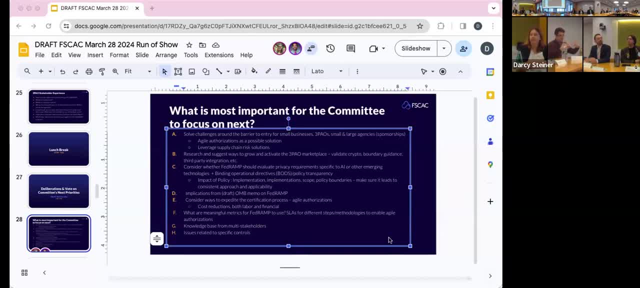 then if they get the authorized owner of the other construct, and then there can the other construct, and then there can the other construct, and then there can be a five level agreement on the mapping, be a five level agreement on the mapping, be a five level agreement on the mapping, if that's even possible. 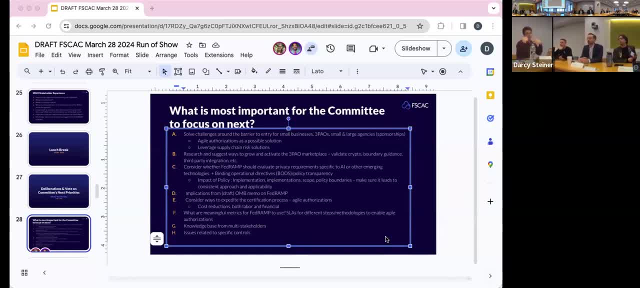 if that's even possible. if that's even possible, is that what we could ask gsa to ask? is that what we could ask gsa to ask? is that what we could ask gsa to ask right now? this would be more of a right now. this would be more of a. 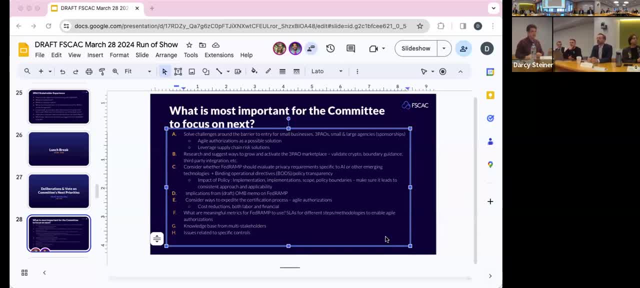 right now. this would be more of a discussion recommendation to say you, discussion recommendation to say you, discussion recommendation to say: you know, fedramp, get the csa and come up. know fedramp, get the csa and come up. know fedramp, get the csa and come up with a bilateral agreement. 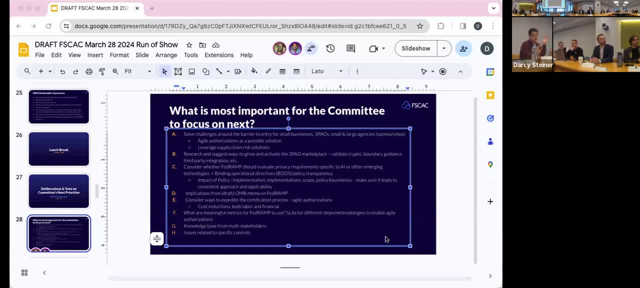 with a bilateral agreement, with a bilateral agreement, or whatever, or whatever, or whatever. you'll never get it with isaac, but you'll never get it with isaac. but you'll never get it with isaac. but there's others who might. maybe there's. there's others who might. maybe there's. 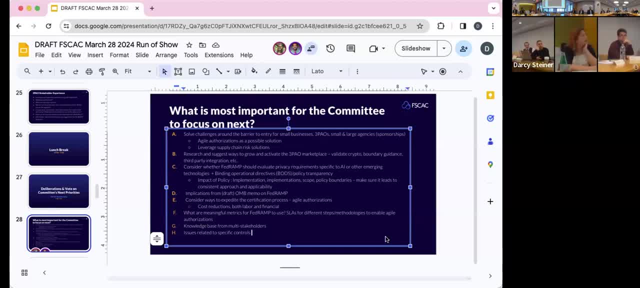 there's others who might. maybe. there's only cost reductions. that's just a only cost reductions. that's just a only cost reductions. that's just a simple way forward, or reciprocity. simple way forward, or reciprocity, although i guess we did take that off, although i guess we did take that off. 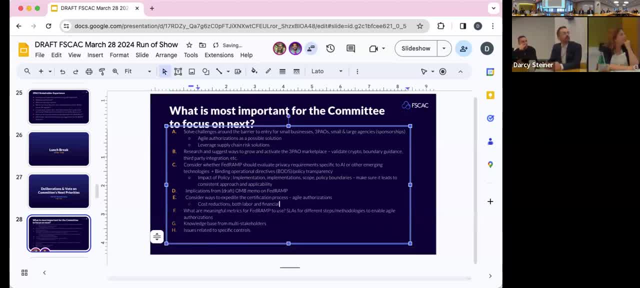 although i guess we did take that off the list, the list, the list, but then isn't it something that's? but then isn't it something that's? but then isn't it something that's already in the memo and in already in the memo and in? already in the memo and in gsa's roadmap? we just had two in the last two weeks. we just had two in the last two weeks. we just had two in the last two weeks: two congressional hearings at the hask, two congressional hearings at the hask, two congressional hearings at the hask. uh, where reciprocity and ato were. 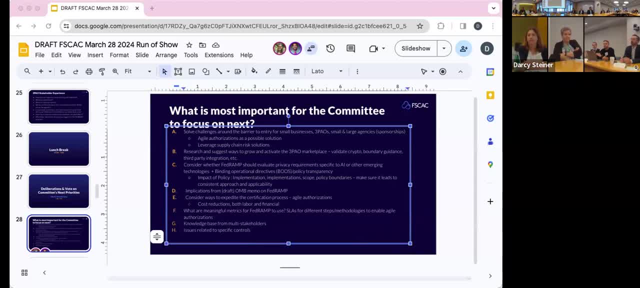 uh where reciprocity and ato were. uh, where reciprocity and ato were discussed, discussed, discussed, um and um and um, and one of them specifically referenced- the one of them specifically referenced, the one of them specifically referenced- the 12 authorizations from the dab, 12 authorizations from the dab. 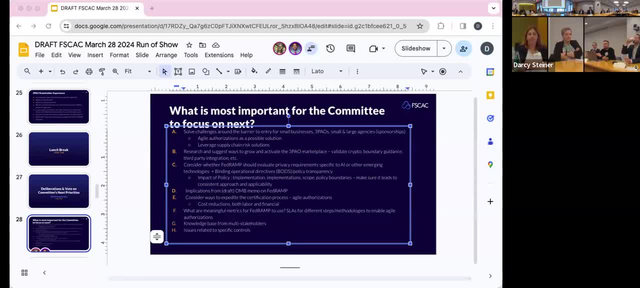 12 authorizations from the dab um and they used that in terms of you um, and they used that in terms of you um, and they used that in terms of you know they can only do 12 a year and know they can only do 12 a year. and 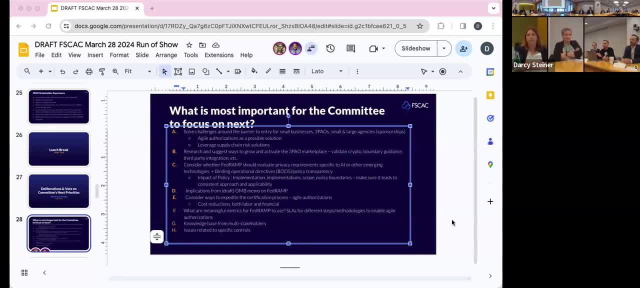 know they can only do 12 a year and, but it was referencing atos and and my but it was referencing atos and and my but it was referencing atos and. and my boss asked me: you know, jackie, what is? boss asked me: you know, jackie, what is? 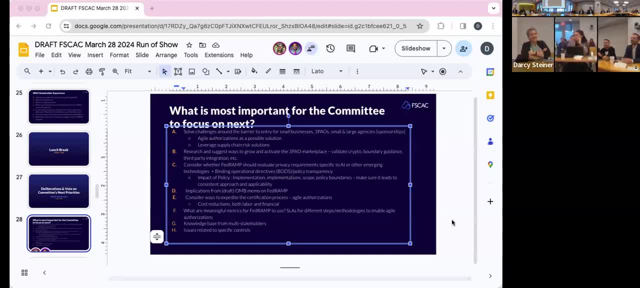 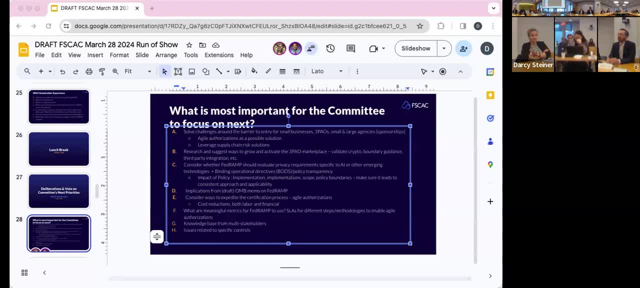 authorization perspective? oh, it's not authorization perspective. oh, it's not regular atos does that, but regular atos does that, but regular atos does that. but reciprocity was huge and all of the reciprocity was huge and all of the reciprocity was huge, and all of the conversations in the hask and so 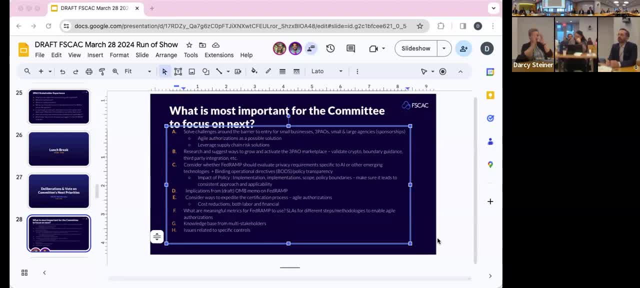 conversations in the hask, and so conversations in the hask. and so you know when you look at it from a, you know when you look at it from a, you know when you look at it from a fed ramp perspective, not even looking at fed ramp perspective, not even looking at. 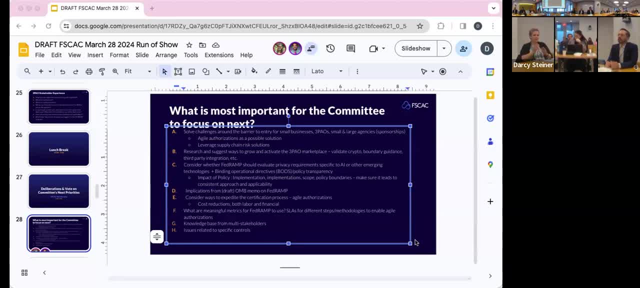 fed ramp perspective, not even looking at other frameworks, other frameworks. other frameworks is: how do i partner with gsa? it's is: how do i partner with gsa? it's again part of what the omb memo is you again part of what the omb memo is you. 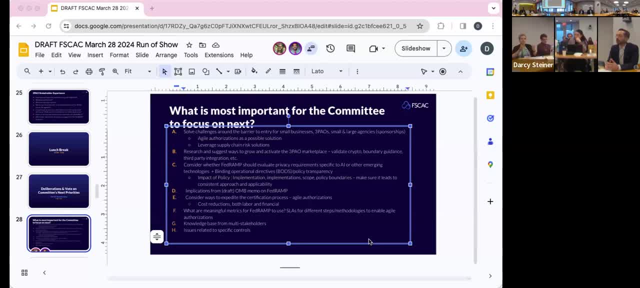 again part of what the omb memo is. you know, know, know. can somebody take an hhs authorization? can somebody take an hhs authorization? can somebody take an hhs authorization and i use it in in the department or do and i use it in in the department or do? 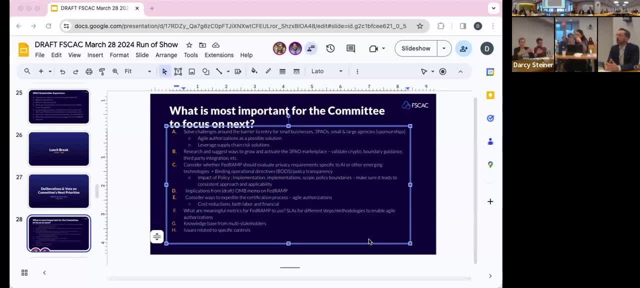 and i use it in in the department? or do i have to retest and you know what are i have to retest and you know what are i have to retest and you know what are my requirements. what are somebody else's my requirements? what are somebody else's? 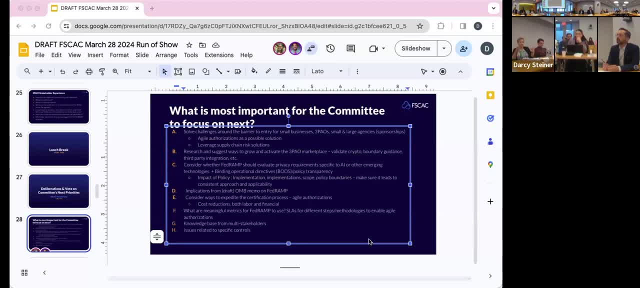 my requirements. what are somebody else's requirements? how do we look at this? and requirements, how do we look at this? and requirements, how do we look at this? and are we all looking across the same? are we all looking across the same? are we all looking across the same standards? and so some of this goes back. 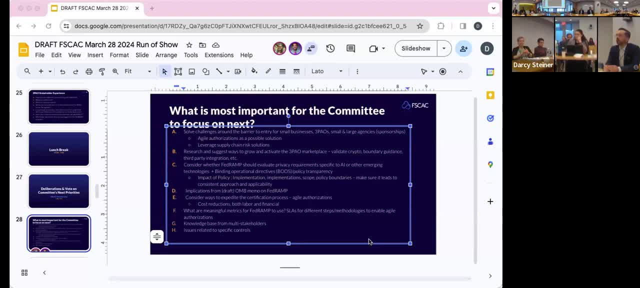 standards, and so some of this goes back standards and so some of this goes back to the knowledge base and the three paos, to the knowledge base and the three paos, to the knowledge base and the three paos and making sure that we are all looking. 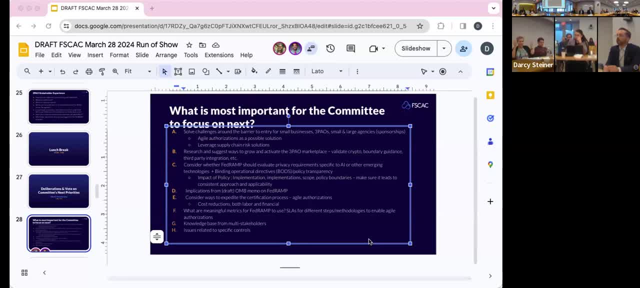 and making sure that we are all looking, and making sure that we are all looking at this from the same lens, at this from the same lens, at this from the same lens, but just to give you a perspective. if, but. just to give you a perspective, if, but just to give you a perspective. if you haven't seen some of the, the hask, 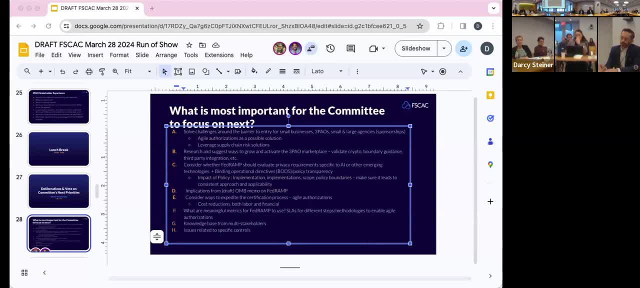 you haven't seen some of the the hask. you haven't seen some of the the hask. testimony over the last couple weeks. testimony over the last couple weeks. testimony over the last couple weeks. this has been the topic of conversation. this has been the topic of conversation. 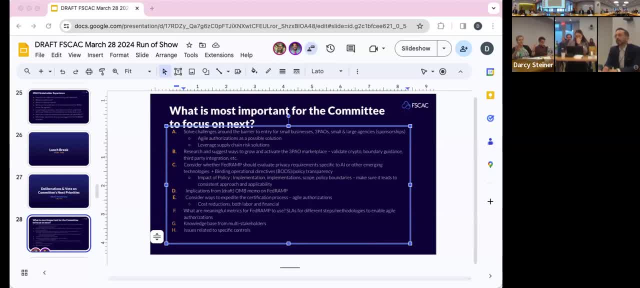 this has been the topic of conversation- um so you know we don't even reciprocate. um so you know we don't even reciprocate um so you know we don't even reciprocate among the fedramp program, and we're among the fedramp program and we're. 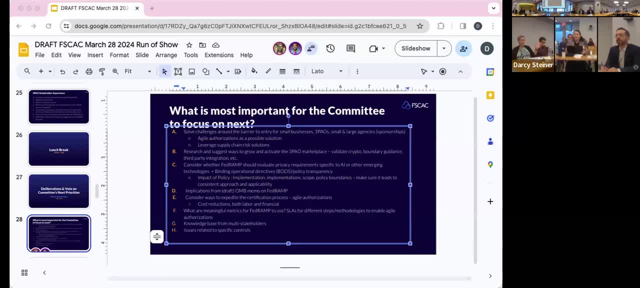 among the fedramp program and we're talking about how do we incorporate cnoc. talking about how do we incorporate cnoc, talking about how do we incorporate cnoc. so we really need to start in our own. so we really need to start in our own. 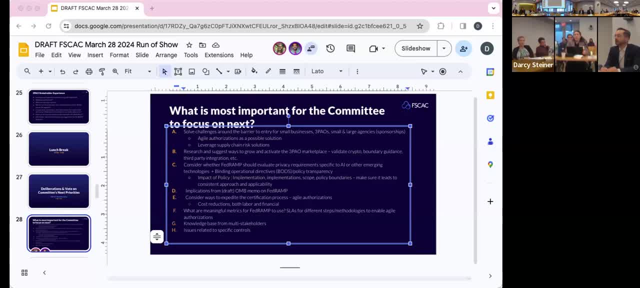 so we really need to start in our own backyard, backyard, backyard, uh, and figuring out how we can uh, uh and figuring out how we can uh uh and figuring out how we can uh leverage other test results. is that as leverage other test results? is that as leverage other test results? is that as much of business risk acceptance from the? 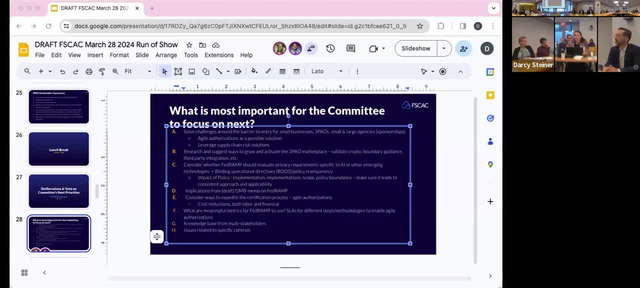 much of business risk acceptance from the much of business risk acceptance from the agencies as security. that's what i agencies as security. that's what i agencies as security. that's what i was gonna say like feel like. in was gonna say like, feel like in was gonna say like, feel like in getting agency buy-in to what is. 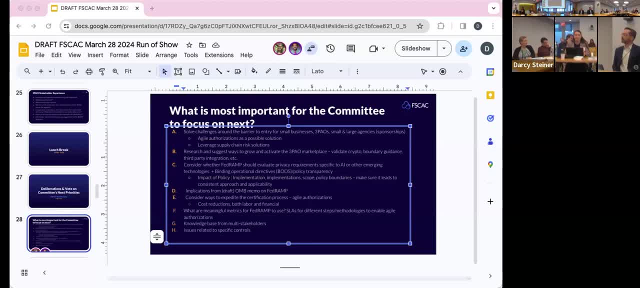 getting agency buy-in to what is getting agency buy-in to what is happening across the government, so to happening across the government. so to happening across the government, so to speak, in the existing program, like speak in the existing program, like speak in the existing program, like. so that would be an area we want to. 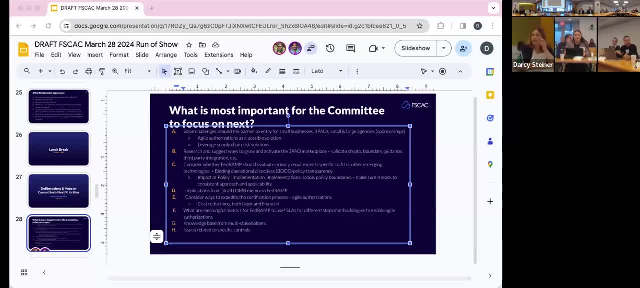 so that would be an area we want to. so that would be an area we want to strategize on and potentially perform, strategize on and potentially perform, strategize on and potentially perform. and, specifically, i wonder if there's like, and specifically, i wonder if there's like. 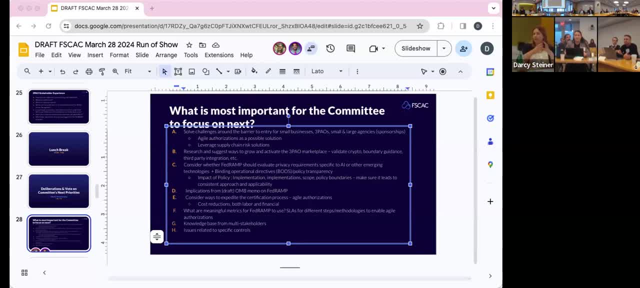 and specifically, i wonder if there's like a pilot of reciprocity, that we might a pilot of reciprocity, that we might a pilot of reciprocity that we might want to construct like a universe around, want to construct like a universe around. want to construct like a universe around like is it? is it? just ask providers, is? 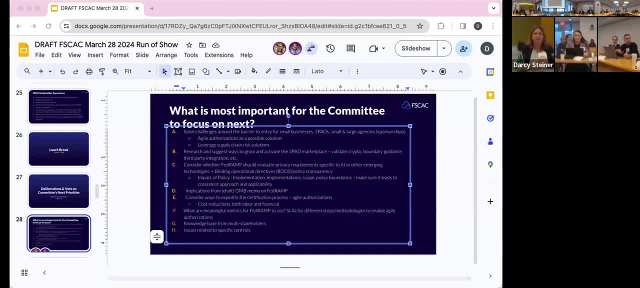 like: is it? is it just ask providers? is like: is it, is it just ask providers? is it just fed ramp low or just fed ramp? it just fed ramp low or just fed ramp? it just fed ramp low or just fed ramp medium? are there specific types of tools? 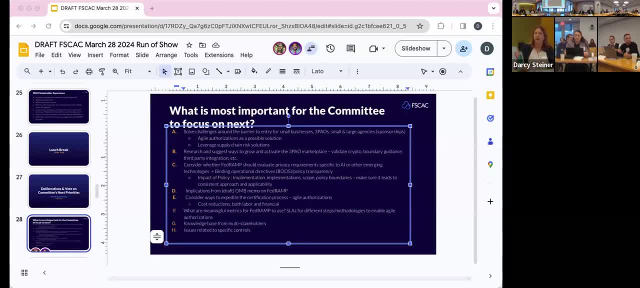 medium. are there specific types of tools? medium? are there specific types of tools? like collaboration tools would be a good. like collaboration tools would be a good. like collaboration tools would be a good example for a pilot. because of the example for a pilot. because of the example for a pilot, because of the impact and ability to control risk. 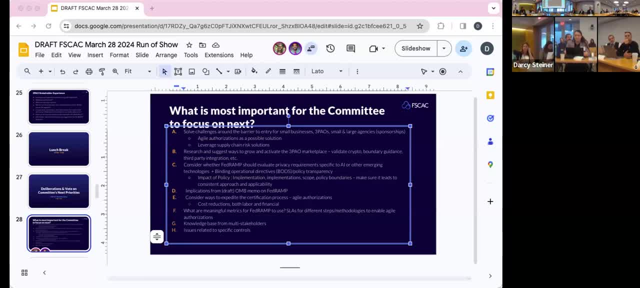 impact and ability to control risk. impact and ability to control risk. this group together could potentially- this group together could potentially this group together could potentially define a pilot that would be a most define a pilot that would be a most define a pilot that would be a most like a pretty meaningful example, if like. 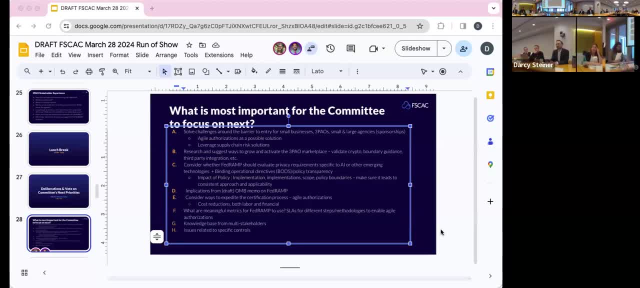 like a pretty meaningful example. if, like like a pretty meaningful example. if, like, we can get this to work and we can. we can get this to work and we can. we can get this to work and we can generalize from it: gob is undertaking a pilot with fed ramp. 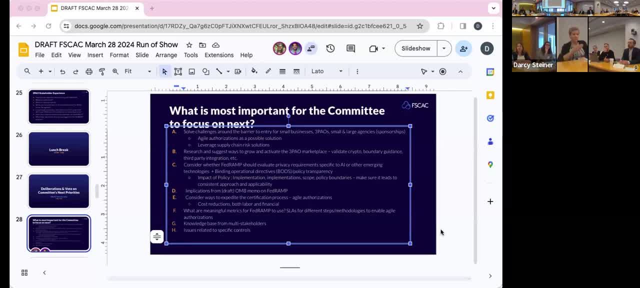 gob is undertaking a pilot with fed ramp. gob is undertaking a pilot with fed ramp. you saw that on the roadmap um and that you saw that on the roadmap um and that you saw that on the roadmap um. and that is to. to shorten the time from is to to shorten the time from. 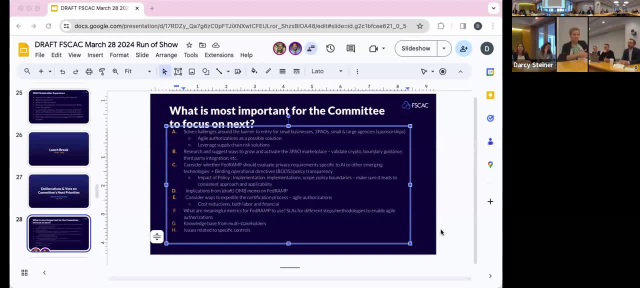 is to to shorten the time from authorization to marketplace, authorization to marketplace, authorization to marketplace. um, you know so, um, you know so, um, you know so, examining what we do and how we would examining what we do and how we would examining what we do and how we would set up a checklist, or whatever to say. 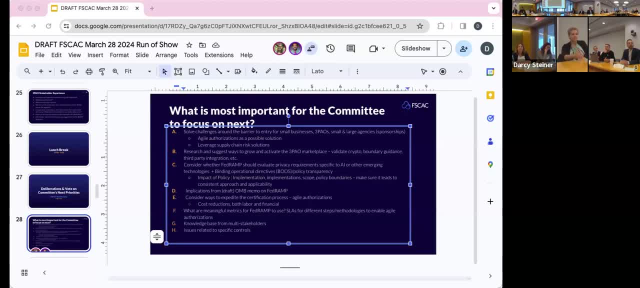 set up a checklist or whatever to say. set up a checklist or whatever to say, we're following the standards to. we're following the standards to. we're following the standards to authorization, and so when you issue authorization, and so when you issue authorization, and so when you issue something, we can put it to marketplace. 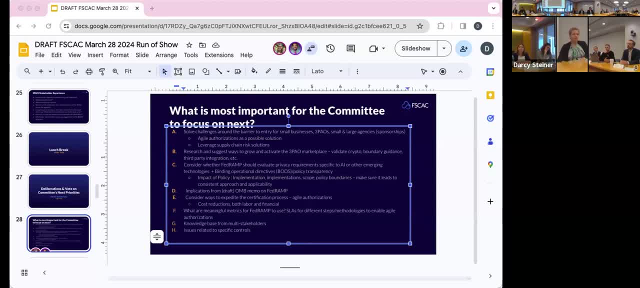 something we can put it to marketplace, something we can put it to marketplace without you know six months, you know, or without you know six months, you know, or without you know six months, you know, or whatever, whatever, whatever, um, and, and i think that um, and and i think that 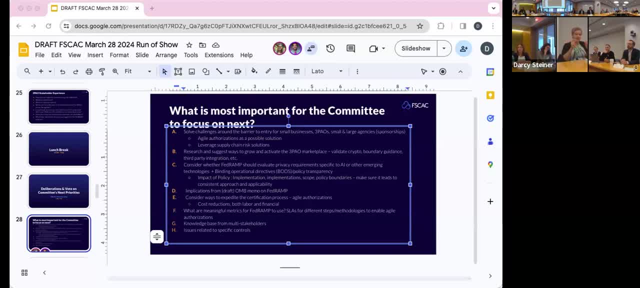 um, and, and i think that, um, you know, um, you know, um you know, today, today, today, the jab and dod, and i don't know about the jab and dod, and i don't know about the jab and dod and i don't know about other agencies, but we issue a. 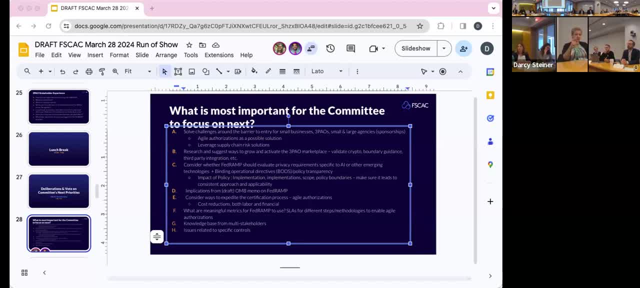 other agencies, but we issue a other agencies, but we issue a provisional authorization which is provisional authorization, which is provisional authorization, which is really looking only at the cloud, really looking only at the cloud, really looking only at the cloud. provider agency atos also look at the provider agency atos also look at the. 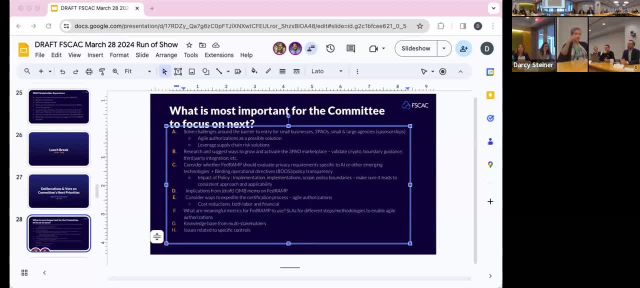 provider agency atos, also look at the implementation and look at their own implementation and look at their own implementation and look at their own system. so there's a lot of system, so there's a lot of system, so there's a lot of uh controls in there. that actually 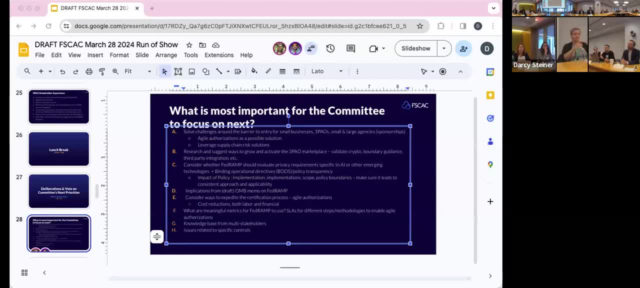 uh controls in there that actually uh controls in there that actually belong to a system, as opposed to just belong to a system, as opposed to just belong to a system, as opposed to just what belongs. and so it is hard to what belongs, and so it is hard to. 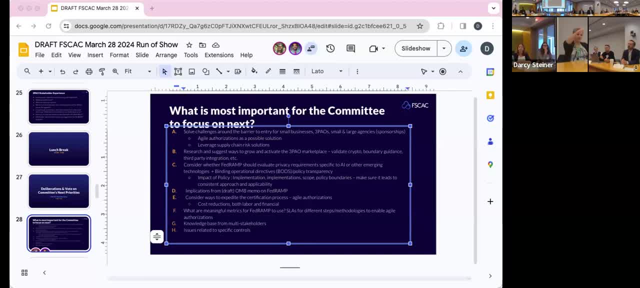 what belongs. and so it is hard to reciprocate some agency packages, reciprocate some agency packages, reciprocate some agency packages because they issue an ato inclusive of, because they issue an ato inclusive of, because they issue an ato inclusive of their system implementation. 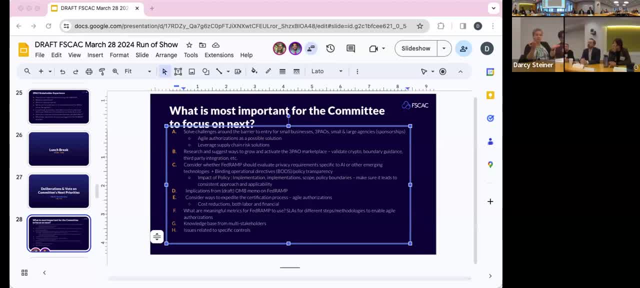 their system implementation, their system implementation, and so it's hard to peel that layer, and so it's hard to peel that layer, and so it's hard to peel that layer apart from a reciprocity perspective, apart from a reciprocity perspective, apart from a reciprocity perspective. and so you know, if we wanted to, to gain. 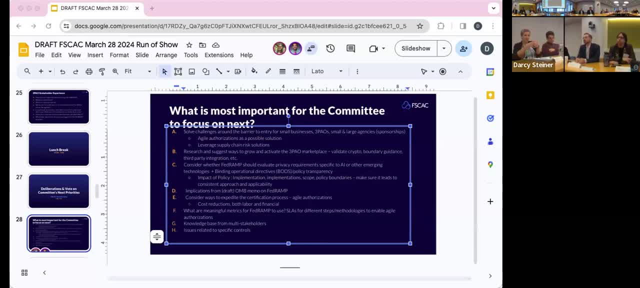 and so you know, if we wanted to to gain, and so you know, if we wanted to to gain some synergy, it would be some synergy, it would be some synergy, it would be. i think of how we do agency. i think of how we do agency, i think of how we do agency authorizations. and can we separate out? 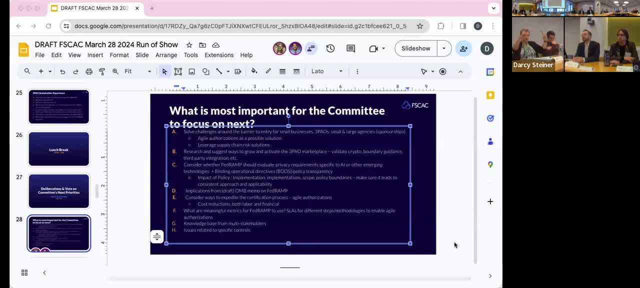 authorizations and can we separate out authorizations and can we separate out three pao results and the cloud, three pao results and the cloud. three pao results and the cloud infrastructure from the system or the infrastructure from the system or the infrastructure from the system or the mission layer cloud that's been added to. 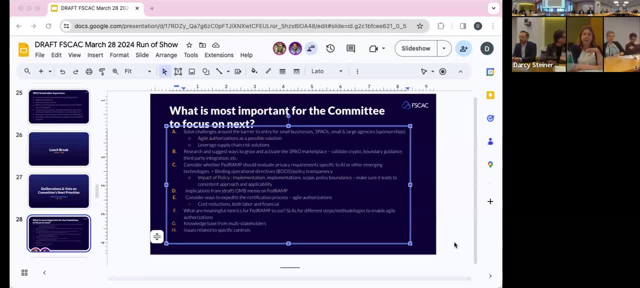 mission layer cloud. that's been added to mission layer cloud. that's been added to it it it. that's really interesting. i mean, do you that's really interesting? i mean, do you that's really interesting? i mean, do you think it would be possible for the think it would be possible for the? 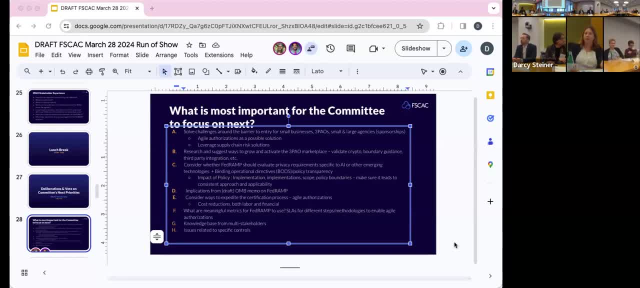 think it would be possible for the agencies to do that- to have more modular agencies, to do that, to have more modular agencies, to do that, to have more modular atos instead of atoing a monolith of atos, instead of atoing a monolith of. 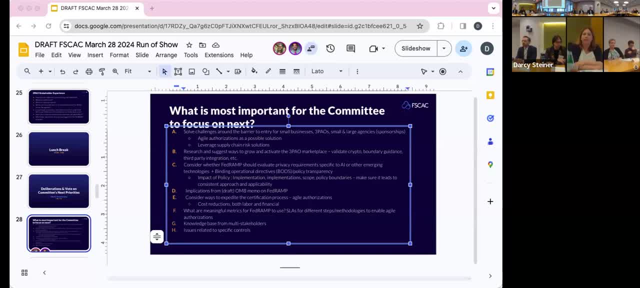 atos instead of atoing a monolith of everything from the cloud service, everything from the cloud service, everything from the cloud service provider to the implementation provider, to the implementation provider, to the implementation. that's what we've attempted to do in. that's what we've attempted to do in. 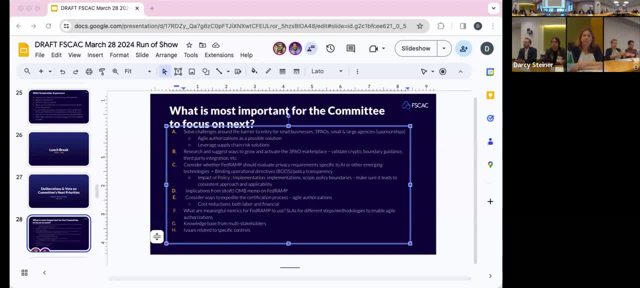 that's what we've attempted to do in the department, so that, and that's the the department, so that, and that's the the department, so that, and that's the same principle as the jab, which is you. same principle as the jab which is you. same principle as the jab which is you issue the authorization for the cloud. 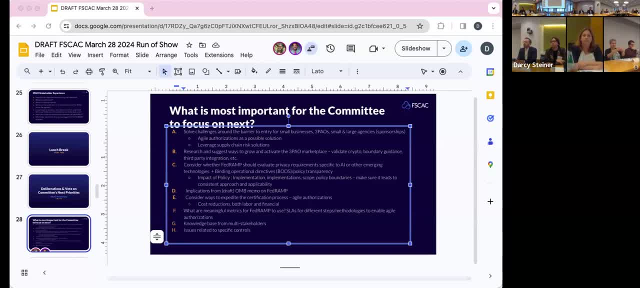 issue, the authorization for the cloud issue, the authorization for the cloud infrastructure and the sas infrastructure and the sas infrastructure and the sas, and, and and again i, i think again, those and and and again i, i think again, those and and and again i, i think again, those need to be pulled apart even further now. 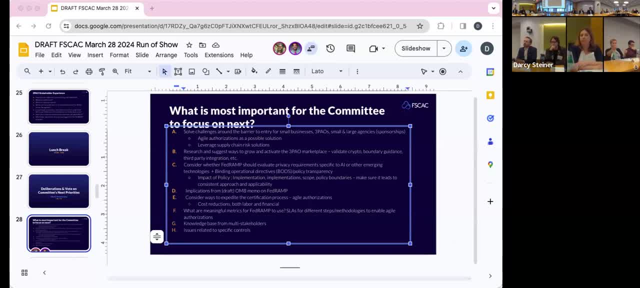 need to be pulled apart even further now. need to be pulled apart even further now, so that an agency authorizing official, so that an agency authorizing official, so that an agency authorizing official that builds a mission system or uses a that builds a mission system or uses a. 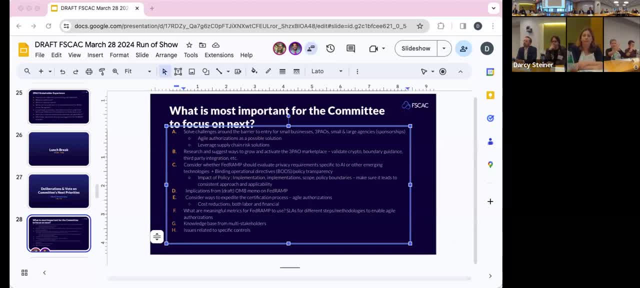 that builds a mission system or uses a sas can actually understand risk from sas, can actually understand risk from sas, can actually understand risk from that? not necessarily the cloud that not necessarily the cloud that not necessarily the cloud infrastructure which needs to be, infrastructure which needs to be. 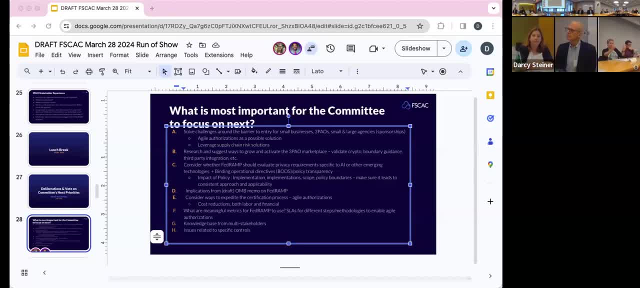 infrastructure, which needs to be considered by fedran, considered by fedran, considered by fedran, but um, but um, but um. but it is modular, and so we will have, but it is modular, and so we will have, but it is modular, and so we will have. you know three. 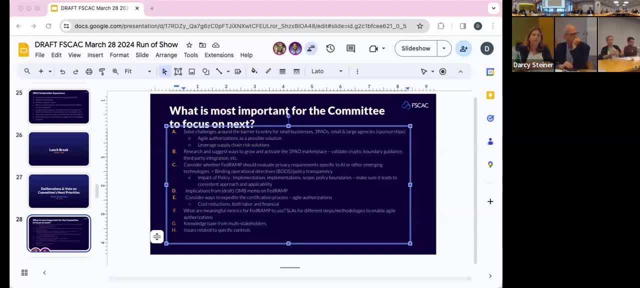 you know three. you know three uh department activities inheriting from a uh department activities inheriting from a uh department activities inheriting from a single package, single package, single package, um, and all they have to do is that last um, and all they have to do is that last. 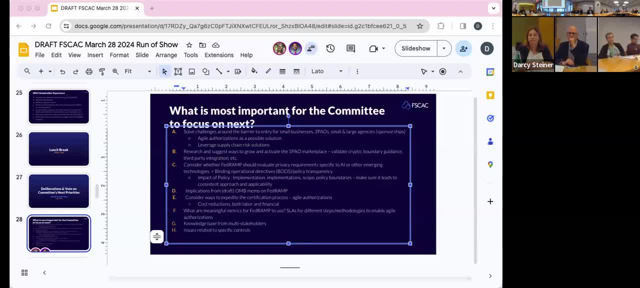 um, and all they have to do is that last mile controls that are in the mile controls, that are in the mile controls that are in the responsibility matrix, responsibility, matrix, responsibility, matrix. just to echo onto jackie's point this, just to echo onto jackie's point this: 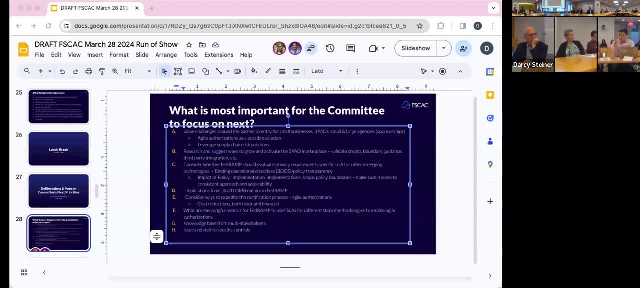 just to echo onto jackie's point, this speaks to a fundamental problem. speaks to a fundamental problem. speaks to a fundamental problem in turn, or misunderstanding of how to in turn, or misunderstanding of how to in turn, or misunderstanding of how to facilitate federman, facilitate federman. 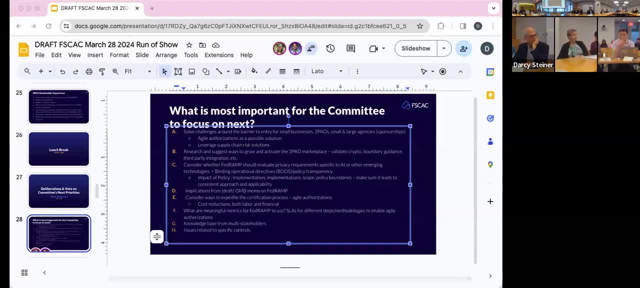 facilitate, federman, because every time we facilitate a because, every time we facilitate a because, every time we facilitate a federal authorization. there's two federal authorization, there's two federal authorization. there's two authorizations, authorizations, authorizations, one corresponding to the underlying, one corresponding to the underlying. 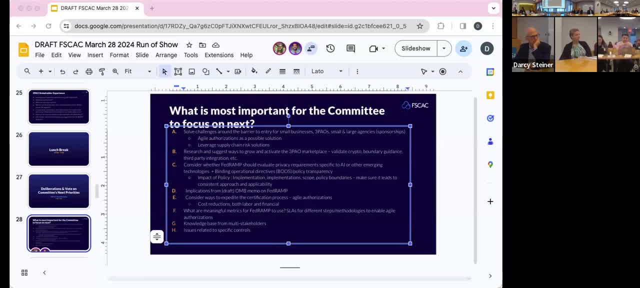 one corresponding to the underlying platform or infrastructure, or sas platform or infrastructure, or sas platform or infrastructure, or sas itself itself, itself that is focused around everything, that that is focused around everything, that that is focused around everything that the vendor has to do with a. 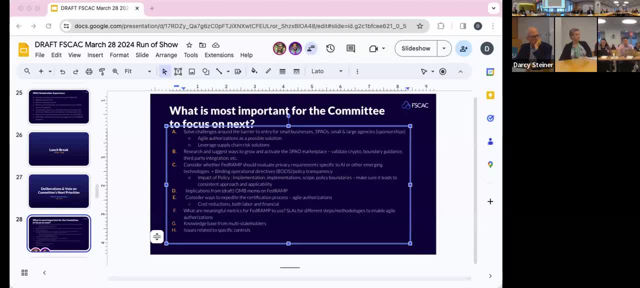 the vendor has to do with a. the vendor has to do with a corresponding set of responsibilities, corresponding set of responsibilities, corresponding set of responsibilities that tenants have to do, that tenants have to do, that tenants have to do, and then the secondary authorization is. and then the secondary authorization is. 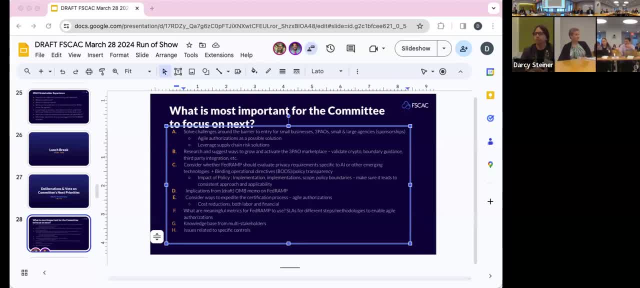 and then the secondary authorization is our tenant, our tenant, our tenant right. so, to the extent that you have right, so, to the extent that you have right, so, to the extent that you have organizations that are issuing a single organizations that are issuing a single organizations that are issuing a single authorization for everything, it just. 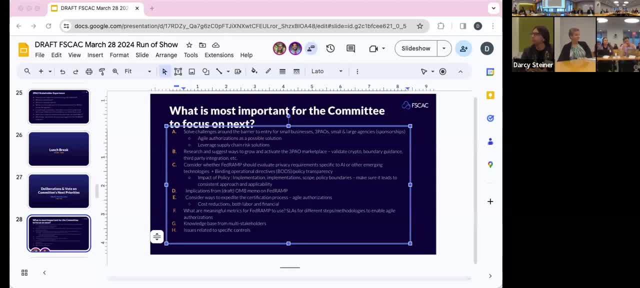 authorization for everything. it just authorization for everything. it just simply shows, simply shows, simply shows a fundamental misunderstanding of this, a fundamental misunderstanding of this, a fundamental misunderstanding of this bifurcated responsibility model. because bifurcated responsibility model? because bifurcated responsibility model? because they're just using it up. 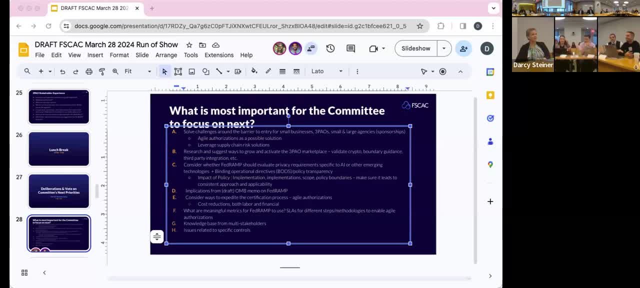 they're just using it up. they're just using it up. well, it really is. well, it really is. well, it really is. yeah, well, it does it's a guidance issue. yeah, well, it does it's a guidance issue. yeah, well, it does it's a guidance issue, but it really does limit the use. 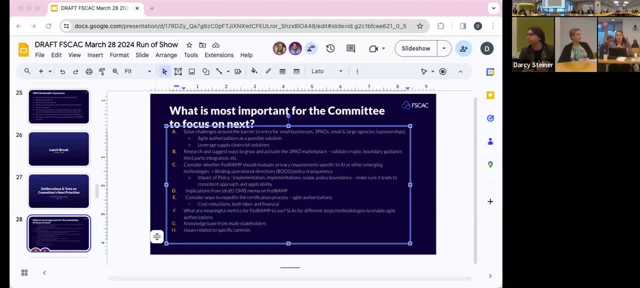 but it really does limit the use, but it really does limit the use of the information. and i'll ask from of the information, and i'll ask from of the information, and i'll ask: from the free field perspective. we have no. the free field perspective, we have no. 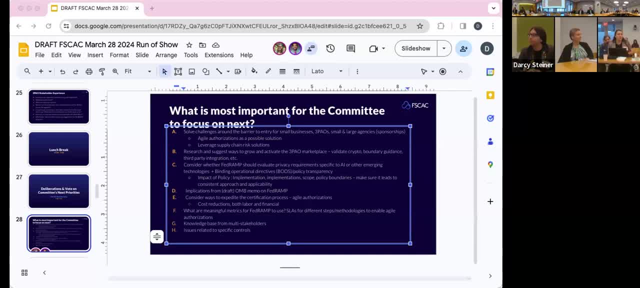 the free field perspective. we have no idea that that actually happens. like idea that that actually happens. like idea that that actually happens. like that's not something that we're involved, that's not something that we're involved, that's not something that we're involved in. and like the the two layers of ato. in and like the, the two layers of ato, in and like the, the two layers of ato. and so it's like, well, what could we do? and so it's like, well, what could we do? and so it's like, well, what could we do in the program and from our 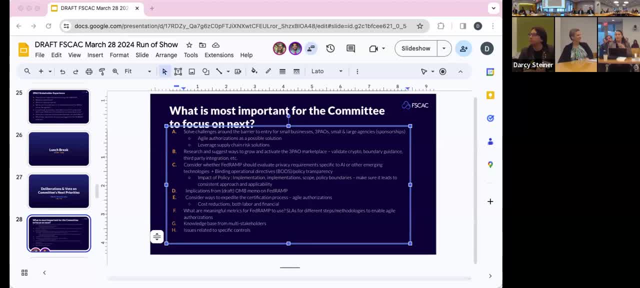 in the program and from our in the program and from our documentation perspective, to facilitate documentation perspective. to facilitate documentation perspective, to facilitate that better um, how you know to that better um, how you know to that better um, how you know to i. i like this idea, i think it's a. i? i like this idea. i think it's a? i i like this idea. i think it's a thing that we potentially think on, so thing that we potentially think on, so thing that we potentially think on. so it built. but i don't know if it's. 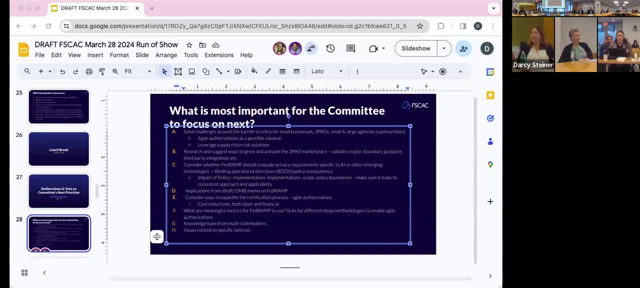 it built. but i don't know if it's it built. but i don't know if it's within our, within our, within our purview, but we, we get to decide if purview. but we, we get to decide if purview. but we, we get to decide if it's in our. yeah, fair enough, i think we. 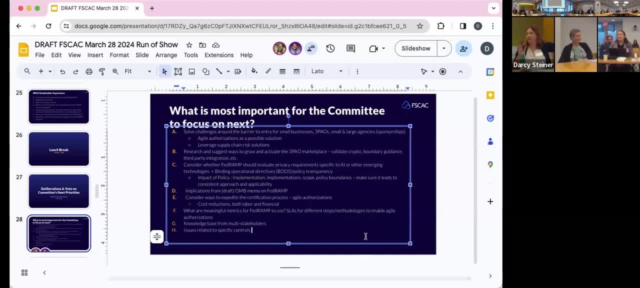 it's in our- yeah, fair enough. i think we it's in our- yeah, fair enough. i think we we've added reciprocity and then taken. we've added reciprocity and then taken. we've added reciprocity and then taken it off in this discussion. but i, i don't. 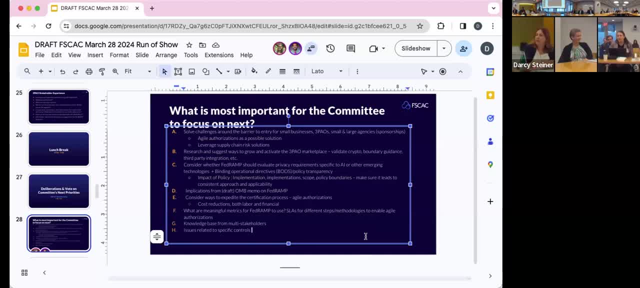 it off in this discussion, but i, i don't it off in this discussion, but i, i don't think it's reciprocity. okay, like i think think it's reciprocity. okay, like i think think it's reciprocity. okay. like i think that's the wrong term- like mod, like. 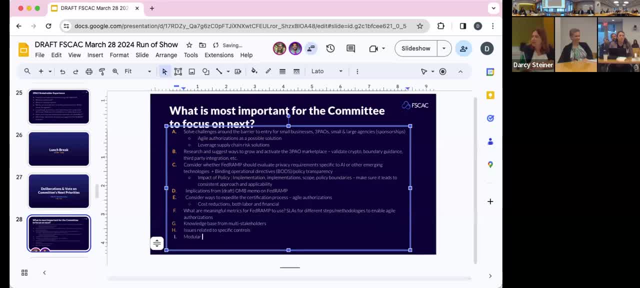 that's the wrong term, like mod, like that's the wrong term, like mod, like modularizing. i don't know. my risk is modularizing. i don't know my risk is modularizing, i don't know. my risk is except acceptance, except acceptance, except acceptance. what i don't know, what do you do in? 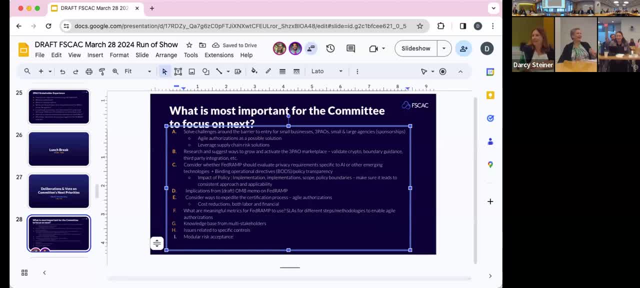 what i don't know? what do you do in what i don't know? what do you do in your project, your project, your project reading an education help into the guidance. but i'm gonna ask help into the guidance. but i'm gonna ask help into the guidance, but i'm gonna ask it in fact. 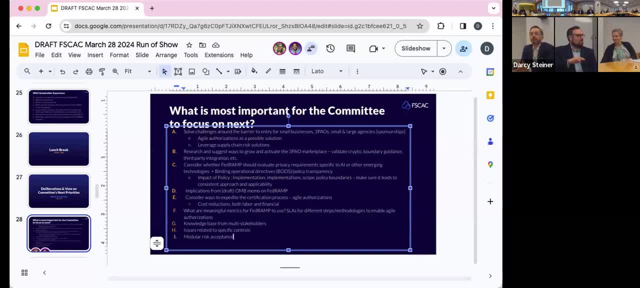 it, in fact it, in fact i, i, i met this with the least i, i i met this with the least i i, i met this with the least background and all of this but and background and all of this but and background and all of this but, and that's, i think, why i'm asking the. 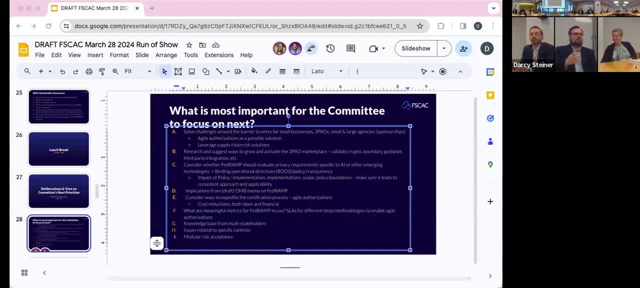 that's, i think, why i'm asking the, that's, i think, why i'm asking the question. but is that something that question? but is that something that question? but is that something that would require, would require, would require? so guidance is one thing, but i don't. 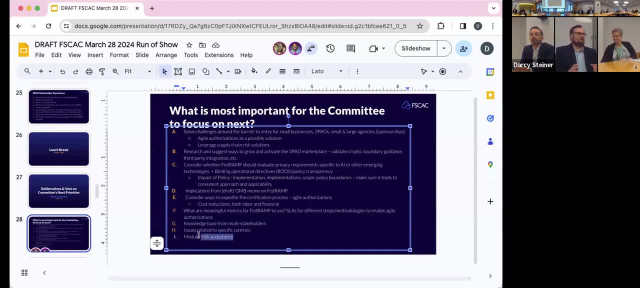 so guidance is one thing, but i don't. so guidance is one thing, but i don't think the legislation being the right. think the legislation being the right. think the legislation being the right rule, but it like is is the way rule, but it like is is the way. 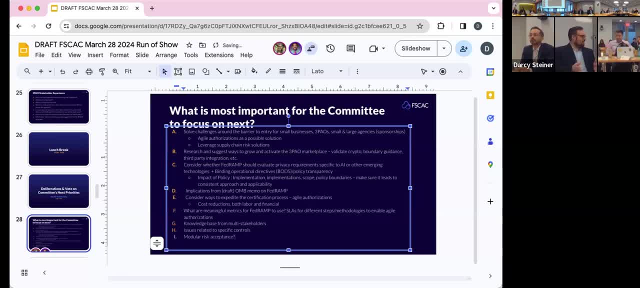 rule, but it like is, is the way it's set up currently fundamentally not. it's set up currently fundamentally not. it's set up currently fundamentally not. set up for that. set up for that. set up for that. like you can put out all the guidance, like you can put out all the guidance. like you can put out all the guidance you want. but if you want someone to do a, you want. but if you want someone to do a, you want. but if you want someone to do a modular atl, which i understood to be like modular atl, which i understood to be like 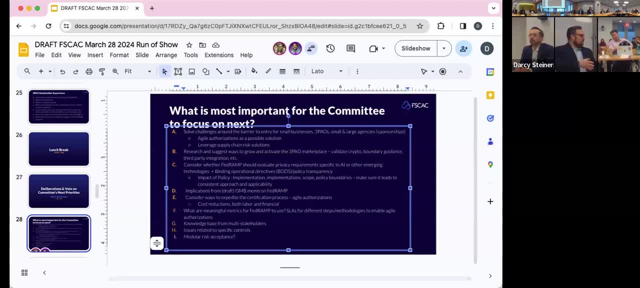 modular atl, which i understood to be like: you would do an atl, you would do an atl, you would do an atl tech stack, then agencies could look at tech stack. then agencies could look at tech stack. then agencies could look at the part of it they want, not the rest of. 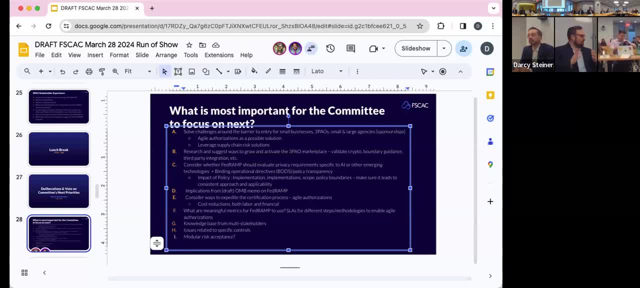 the part of it. they want not the rest of the part of it. they want not the rest of it- right? is there anything currently it right? is there anything currently it right? is there anything currently that provides any kind of roadmap for, that provides any kind of roadmap for? 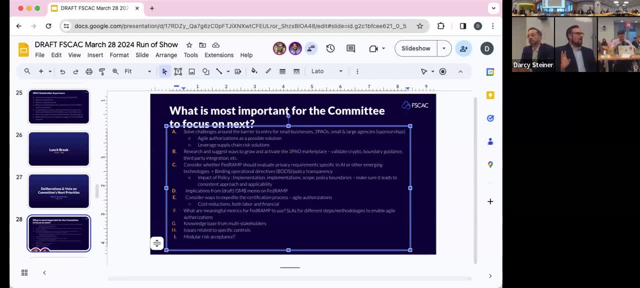 that provides any kind of roadmap for that, or are we just that? or are we just that? or are we just not to suggest? that's not something we not to suggest, that's not something we not to suggest, that's not something we should take on, but just understanding. 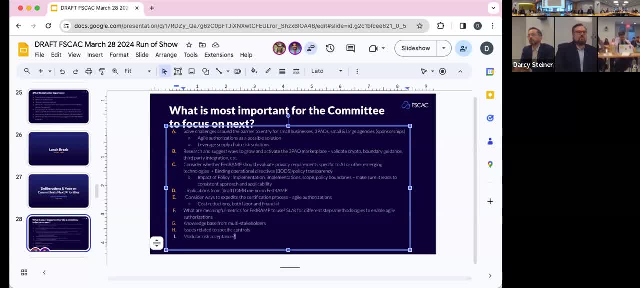 should take on, but just understanding should take on, but just understanding the limitations of we're an advisory. the limitations of we're an advisory, the limitations of we're an advisory committee is that committee? is that committee? is that? is that something that, if we were to put? 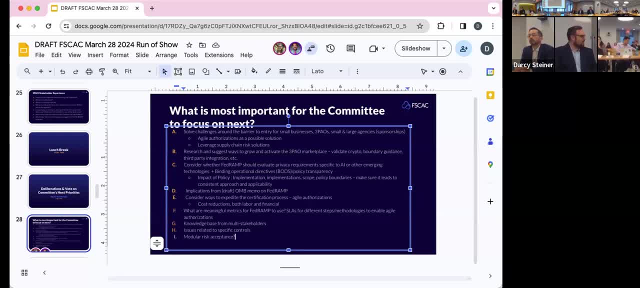 is that something that, if we were to put? is that something that, if we were to put a some thought to, it could happen? a some thought to it could happen, a some thought to it could happen without there being additional policy, without there being additional policy, without there being additional policy regulations. 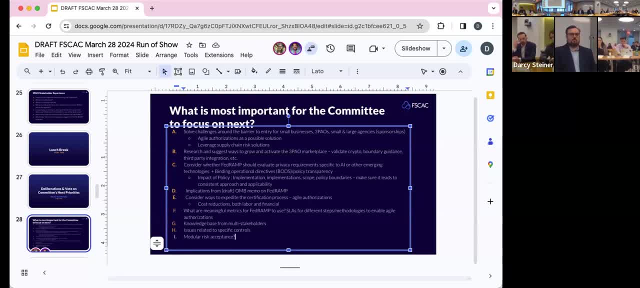 regulations, regulations. i, i have many thoughts. i think i think i, i have many thoughts, i think i, i have many thoughts. i think this is all a solid thing. i think most of this is all a solid thing. i think most of this is all a solid thing. i think most of us should upload a giant ssp pdf into 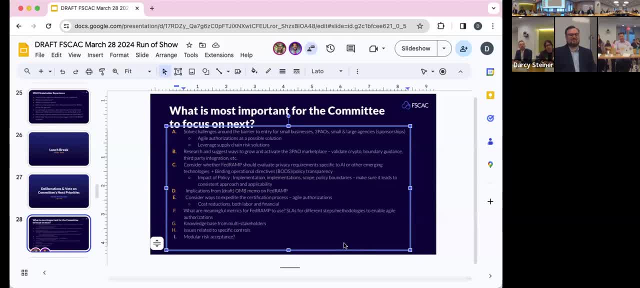 us. should upload a giant ssp pdf into us. should upload a giant ssp pdf into archer and call the day archer and call the day archer and call the day. just being brutally honest here, yeah, um. just being brutally honest here, yeah, um. just being brutally honest here, yeah, um. but but to the, the last half of your. but, but to the the last half of your but, but to the the last half of your point, and i don't want to lose the point, and i don't want to lose the point and i don't want to lose the threat of the threat of the. 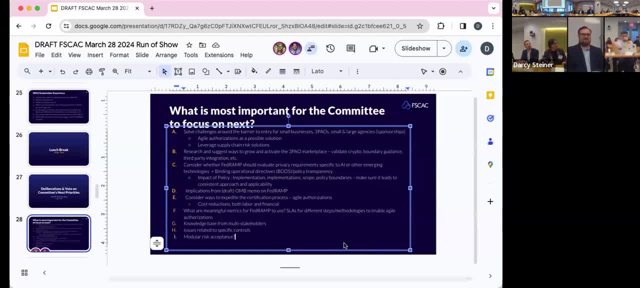 threat of the? um what, what do we do as a committee? um, what, what do we do as a committee? um what, what do we do as a committee and how do we prioritize? and i think, and how do we prioritize, and i think and how do we prioritize, and i think that we have a lot of things here that 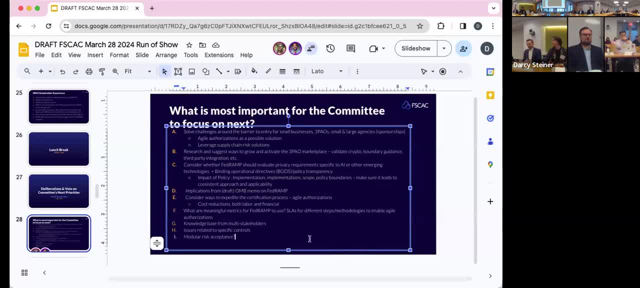 that we have a lot of things here, that that we have a lot of things here that are covered, and i do want to give um are covered and i do want to give um are covered and i do want to give um full kudos to the fed ramp team. it was. 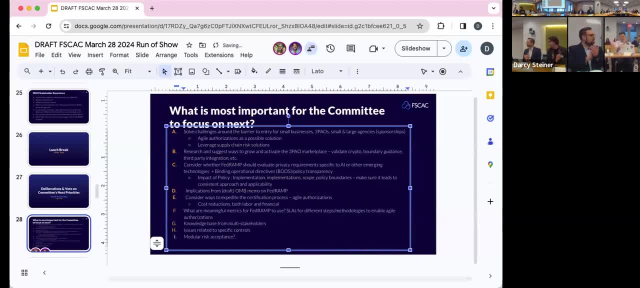 full kudos to the fed ramp team. it was full kudos to the fed ramp team. it was amazing, by the way, and my favorite, amazing, by the way, and my favorite, amazing, by the way, and my favorite: government program, government program, government program, thank you, thank you. um, i don't say that. 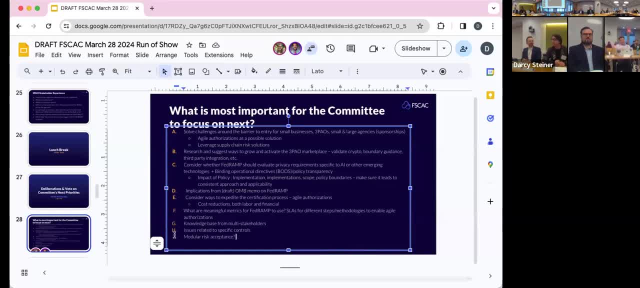 thank you, thank you, um. i don't say that, thank you, thank you, um. i don't say that lightly for those of y'all who know i'm lightly for those of y'all who know i'm lightly for those of y'all who know i'm a governor, um, and they are very smart. 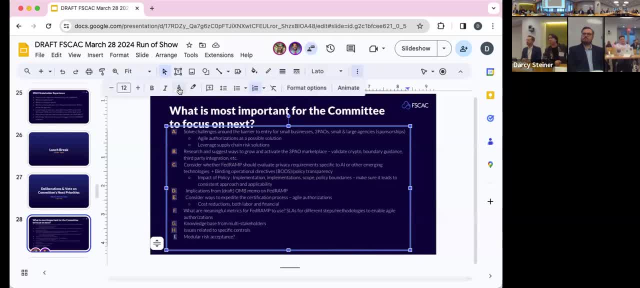 a governor, um, and they are very smart. a governor, um, and they are very smart people and they have very great staff people and they have very great staff people and they have very great staff. they're going to be working on many of. they're going to be working on many of. 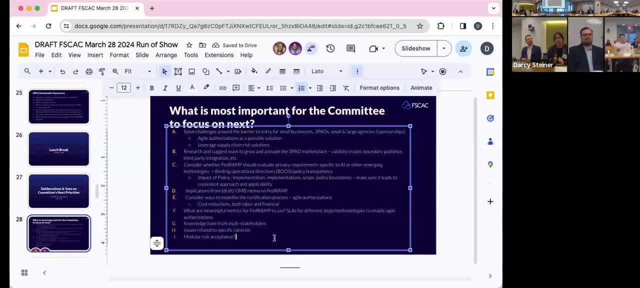 they're going to be working on many of the things that we are discussing here, the things that we are discussing here, the things that we are discussing here. so, if i can put a plea to the committee, so if i can put a plea to the committee, so if i can put a plea to the committee, we should focus on the areas where we 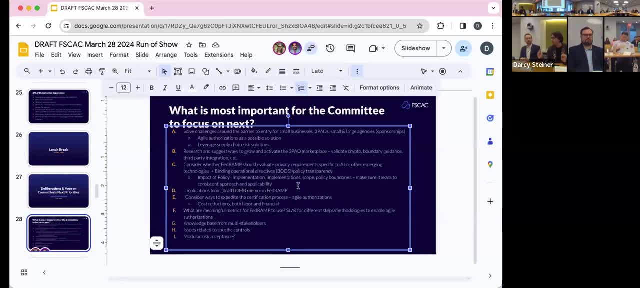 we should focus on the areas where we we should focus on the areas where we think that this group of unique think that this group of unique think that this group of unique individuals has a distinctive advantage. individuals has a distinctive advantage, individuals has a distinctive advantage and viewpoint that the fed ramp team. and viewpoint that the fed ramp team and viewpoint that the fed ramp team. we think that they wouldn't be able to. we think that they wouldn't be able to. we think that they wouldn't be able to figure out on their own for whatever. figure out on their own for whatever. 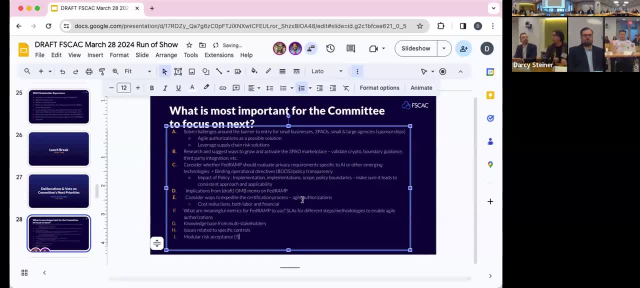 figure out on their own. for whatever reason. you're all brilliant people, but reason. you're all brilliant people, but reason. you're all brilliant people, but we have a lot of nerds at the table here. we have a lot of nerds at the table here. we have a lot of nerds at the table here who might have different things that. 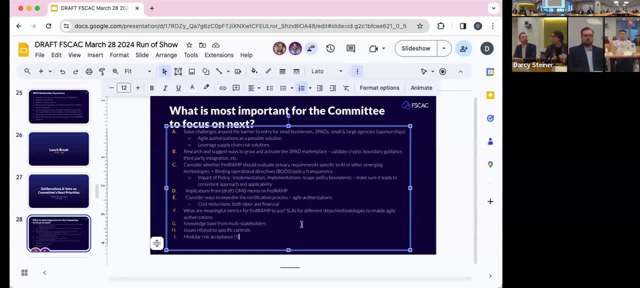 who might have different things, that who might have different things that could bring things in. so i would could bring things in, so i would could bring things in. so i would recommend that we look for those recommend, that we look for those recommend, that we look for those differentiation points between what we. 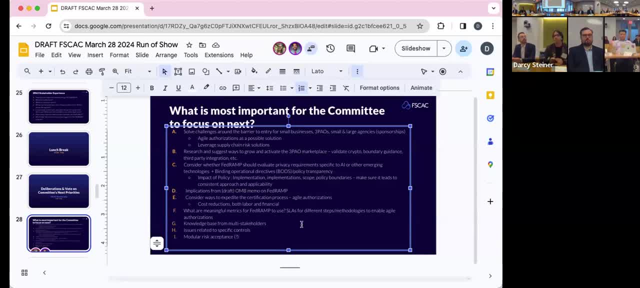 differentiation points between what we differentiation points between what we can do as a group together versus what can do as a group together, versus what can do as a group together versus what we think the fed ramp team, we can just. we think the fed ramp team, we can just. we think the fed ramp team, we can just give them a memo and say: have you all give them a memo? and say: have you all give them a memo? and say: have you all thought about this? you have, okay, we're thought about this. you have, okay, we're. 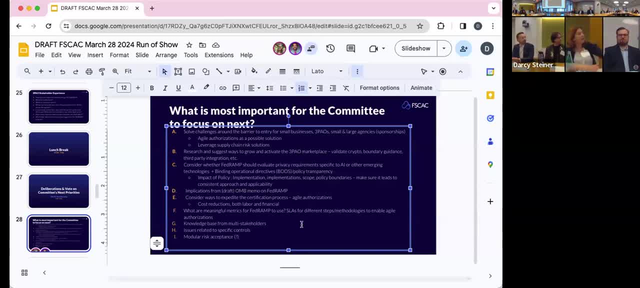 thought about this you have: okay, we're good and follow that good and follow that good and follow that good point- all right. what's the um of good point? all right. what's the um of good point? all right. what's the um of this list? is anything rising to the top? 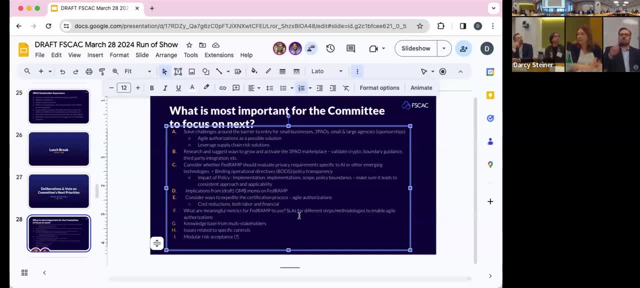 this list is anything rising to the top. this list is anything rising to the top is the? is the? is the best use of our shared perspective of? is the best use of our shared perspective of? is the best use of our shared perspective of? the next year? i'm going to look for one. 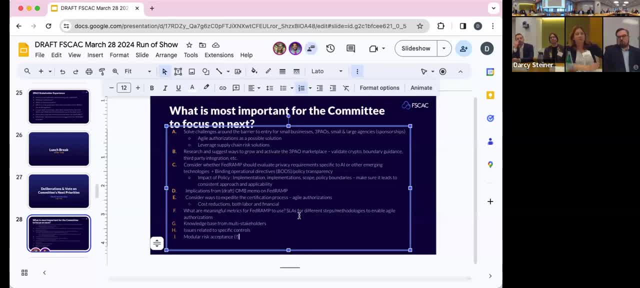 the next year i'm going to look for one, the next year i'm going to look for one. i just want to clarify one one thing, the. i just want to clarify one one thing, the i just want to clarify one one thing, the top priority. i'm just trying to use a. 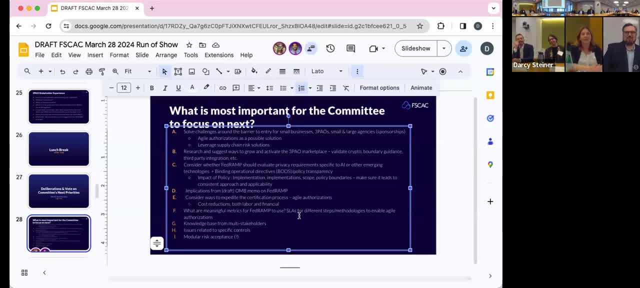 top priority. i'm just trying to use a top priority, i'm just trying to use a forcing function to see if forcing function, to see if forcing function, to see if, sorry, uh compliance, sorry, uh compliance, sorry, uh compliance. guys, i actually go, i actually go, i actually go off a little bit bigger, or can we just? 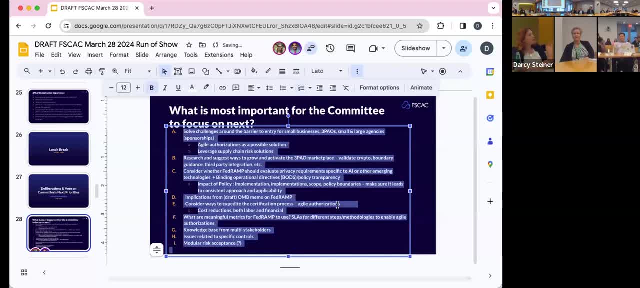 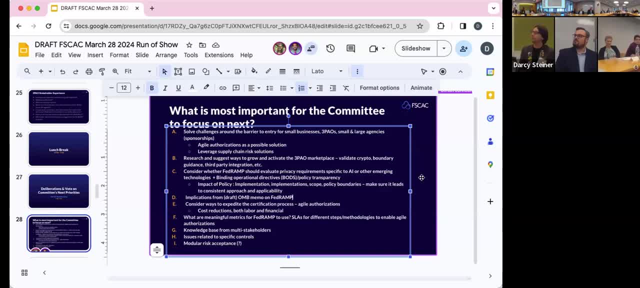 you know something we've also talked. you know something we've also talked about, which i think should be a footnote about, which i think should be a footnote about, which i think should be a footnote on every slide that we have, is you know, on every slide that we have, is you know? 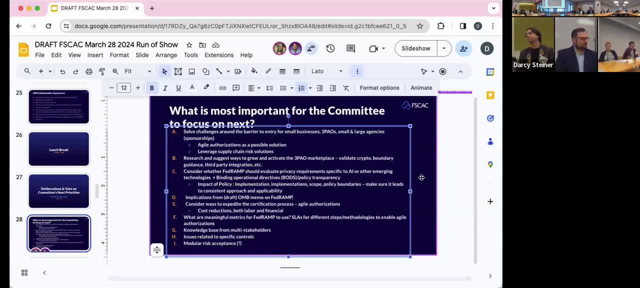 on every slide that we have is, you know, and the board should continuously, and the board should continuously, and the board should continuously advocate for resources and funding for advocate for resources and funding, for advocate for resources and funding for the people, the people, the people, in order to achieve any. 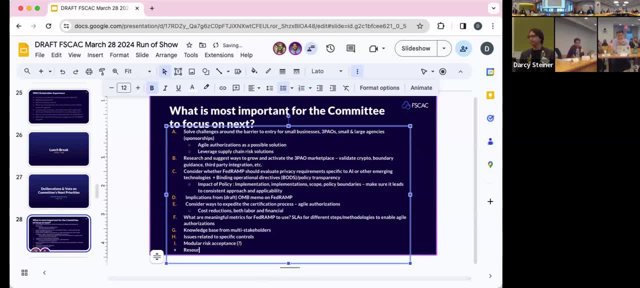 in order to achieve any, in order to achieve any of this going forward. i mean we all all of this going forward. i mean we all all of this going forward. i mean we all all the spets here know how tight times are. the spets here know how tight times are. 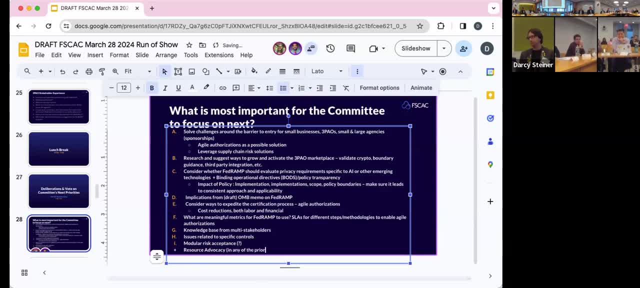 the spets here know how tight times are and i would be remiss to ask anybody to, and i would be remiss to ask anybody to, and i would be remiss to ask anybody to do anything more. do anything more. do anything more. otherwise, we should look at how federal 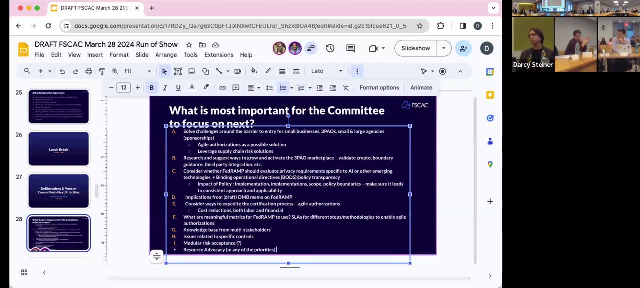 otherwise we should look at how federal, otherwise we should look at how federal could be- could be- could be less with less and focus on what the less with less. and focus on what the less with less and focus on what the core capacities are going to be. it's 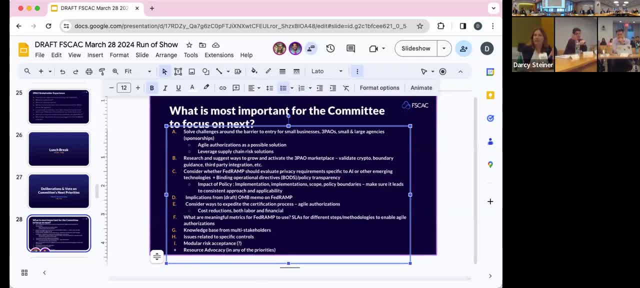 core capacities are going to be. it's core capacities are going to be. it's easier to ask for more budget if you easier to ask for more budget, if you easier to ask for more budget if you have a strategic thing. have a strategic thing, have a strategic thing. our time can be focused towards things. 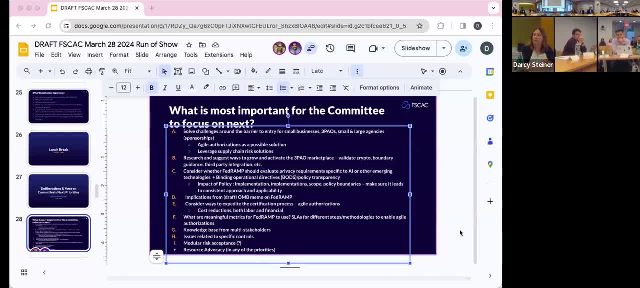 our time can be focused towards things. our time can be focused towards things we'd like to do, but i, but also yes to we'd like to do, but i, but also yes to we'd like to do, but i, but also yes to including budget support, including budget support. 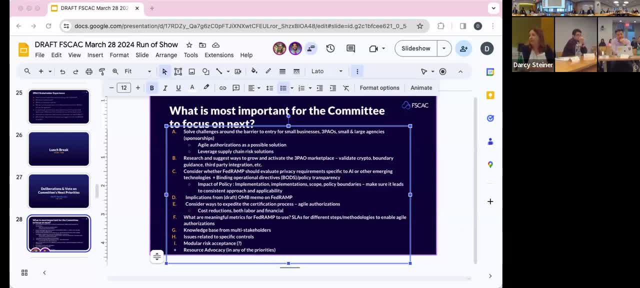 including budget support, and just so, just i think, and you know, and just so, just i think, and you know, and just so, just i think, and you know this for ourselves at gsa, i mean this for ourselves at gsa, i mean this for ourselves at gsa. i mean we, we do a lot of sponsorships at gsa. 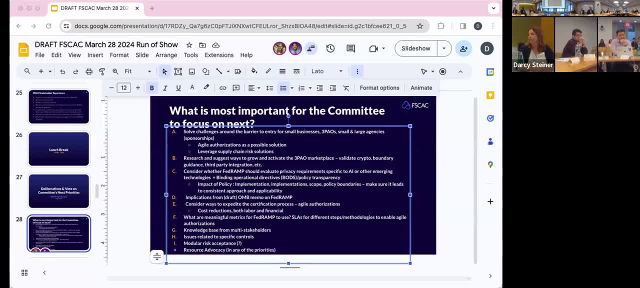 we, we do a lot of sponsorships at gsa. we, we do a lot of sponsorships at gsa, particularly for ourselves, between, particularly for ourselves, between particularly for ourselves, between 2030 to date, 2030 to date, 2030 to date, and the challenge is that. 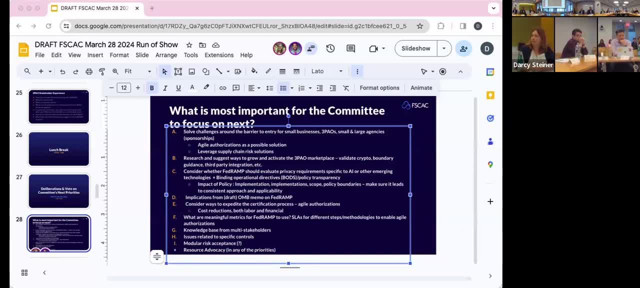 and the challenge is that. and the challenge is that you know each of those sponsorships has. you know each of those sponsorships has. you know each of those sponsorships has a related cost association. where we go a related cost association. where we go a related cost association, where we go to the business line and ask them to go. 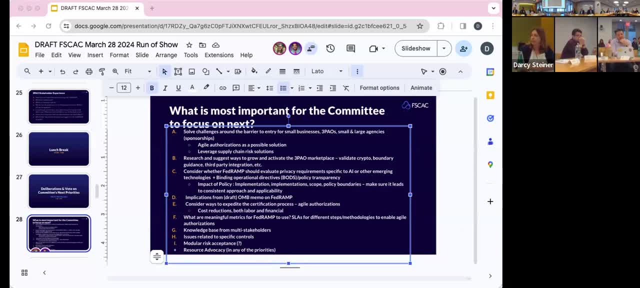 to the business line and ask them to go to the business line and ask them to go through and fund the work, to facilitate through and fund the work to facilitate through and fund the work to facilitate the sponsorship, the sponsorship, the sponsorship, so like when we're talking about 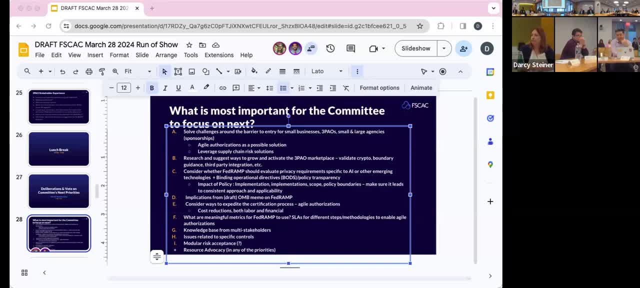 so, like when we're talking about, so, like when we're talking about resource advocacy, i think it's resource advocacy, i think it's resource advocacy. i think it's important to talk about resources, for important to talk about resources, for important to talk about resources for the corresponding sets of sponsoring. 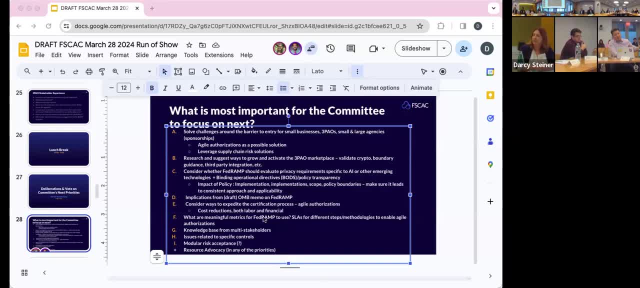 the corresponding sets of sponsoring, the corresponding sets of sponsoring agencies, agencies, agencies such that we're not making dining our, such that we're not making dining our, such that we're not making dining our. individual programs across the agency, individual programs across the agency, individual programs across the agency because they're going to be focused. 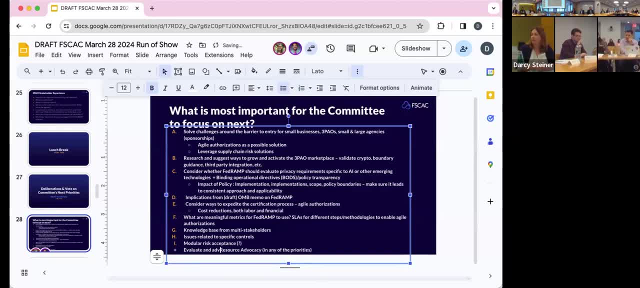 because they're going to be focused, because they're going to be focused around, around, around. point that, uh, a friend from bluescape. point that, uh, a friend from bluescape. point that, uh, a friend from bluescape mentioned, mentioned, mentioned, you know, five thousand dollar license. you know five thousand dollar license. 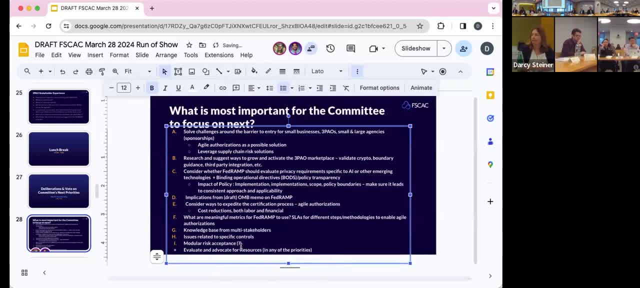 you know, five thousand dollar license agreement and then i go to the business agreement and then i go to the business agreement and then i go to the business line and i'm asking for sixty thousand line and i'm asking for sixty thousand line and i'm asking for sixty thousand dollars to facilitate a sponsorship. 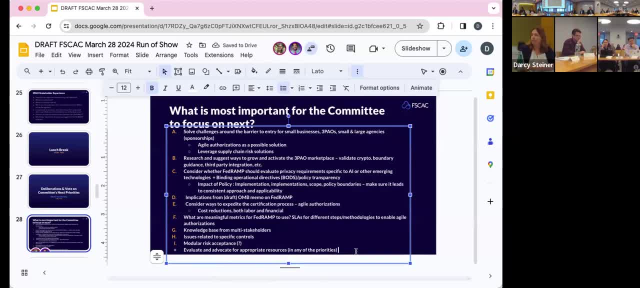 dollars to facilitate a sponsorship, dollars to facilitate a sponsorship action. all of a sudden, that five action. all of a sudden that five action. all of a sudden that five thousand dollar investment is now a thousand dollar. investment is now a thousand dollar investment is now a sixty five thousand dollar investment. so 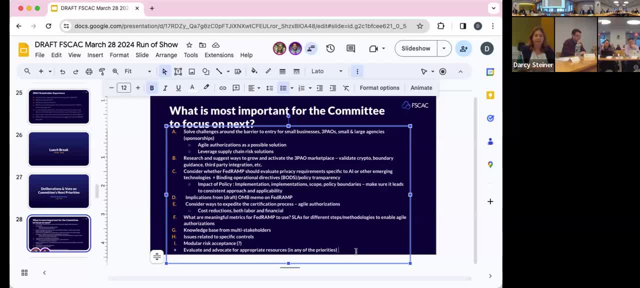 sixty five thousand dollar investment. so sixty five thousand dollar investment. so it starts to become, it starts to become, it starts to become more of a challenge, more of a challenge, more of a challenge. yeah, yeah, yeah, and also, and also and also some of the first names would you choose? 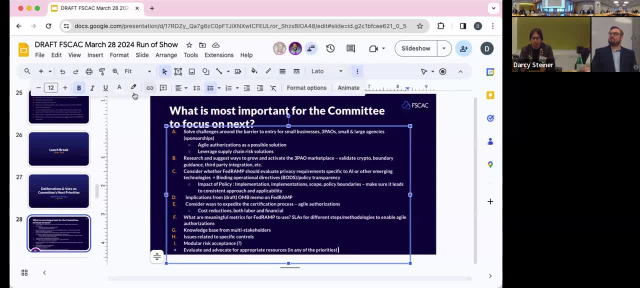 some of the first names. would you choose some of the first names would you choose in this list and we will come up with in this list and we will come up with in this list and we will come up with: copperiness of supportive budget. copperiness of supportive budget. 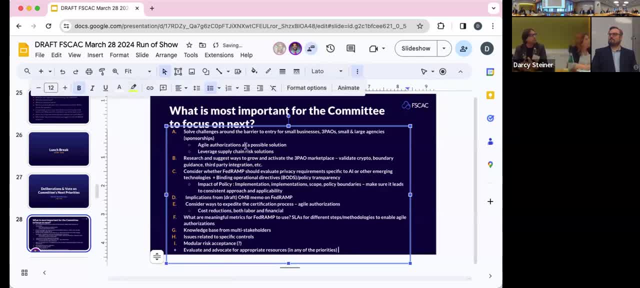 copperiness of supportive budget. arguments for arguments for arguments for: oh, i need more time to say yes. oh, i need more time to say yes. oh, i need more time to say yes, it's hard to pick one. yeah, that's also. it's hard to pick one. yeah, that's also. 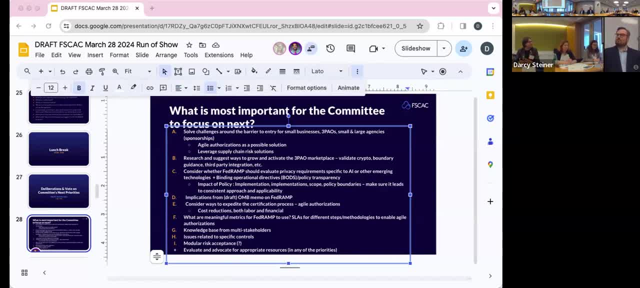 it's hard to pick one. yeah, that's also okay. yeah, i mean we do not have to okay. yeah, i mean we do not have to okay. yeah, i mean we do not have to. um agree on our next priorities today. um agree on our next priorities today. 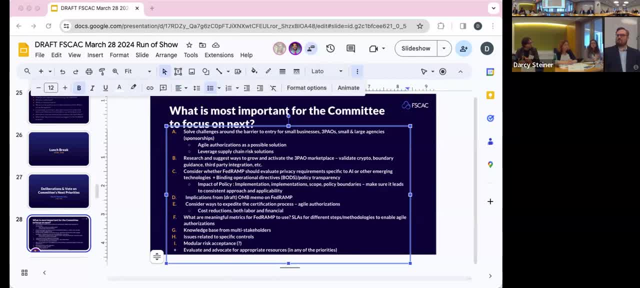 um agree on our next priorities today. we can um pause and uh if you have. we can um pause and uh if you have. we can um pause and uh if you have requirement for more information, of any requirement for more information, of any requirement for more information of any of these topics. we can have some more. 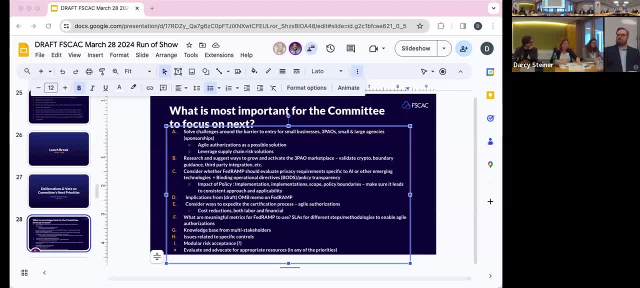 of these topics. we can have some more of these topics. we can have some more presentations in a future meeting. presentations in a future meeting, presentations in a future meeting. or um you know, gather any information. or um you know, gather any information. or um you know, gather any information that you need to come to your conclusion. 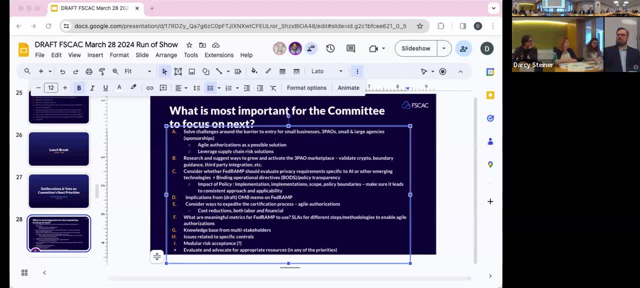 that you need to come to your conclusion, that you need to come to your conclusion, um, um, um, but we do have a vote scheduled for today. but we do have a vote scheduled for today, but we do have a vote scheduled for today. so, um, so, um, so um. would a member of the committee make a? 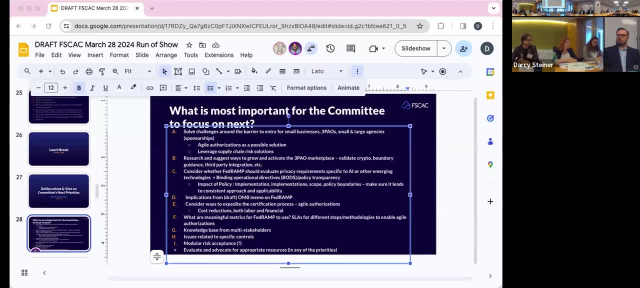 would a member of the committee make a? would a member of the committee make a motion to delay the selection of the motion? to delay the selection of the motion to delay the selection of the committee's next priorities until committee's next priorities, until committee's next priorities, until- um, we have either identified some. 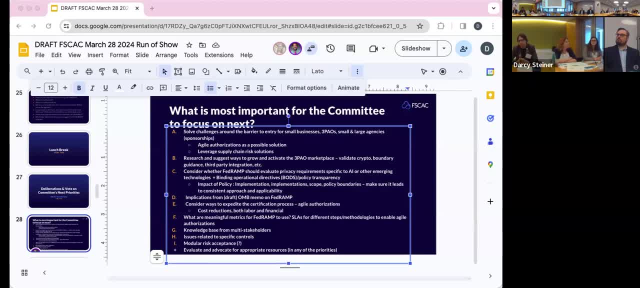 um. we have either identified some um. we have either identified some additional um additional um additional um presentations or information that we presentations, or information that we presentations, or information that we would want, would want, would want. can i actually i think it's a question? can i actually i think it's a question? 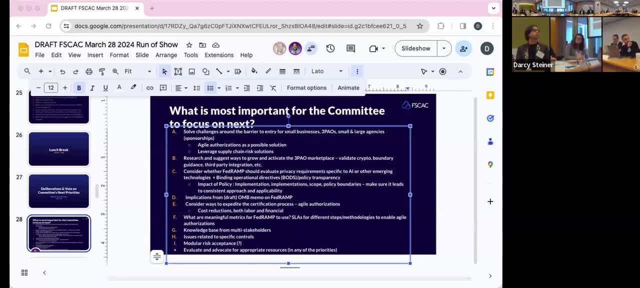 can i actually- i think it's a question um. i think last time we did the voting um. i think last time we did the voting um. i think last time we did the voting in this. that's where she that just seems in this. that's where she that just seems. 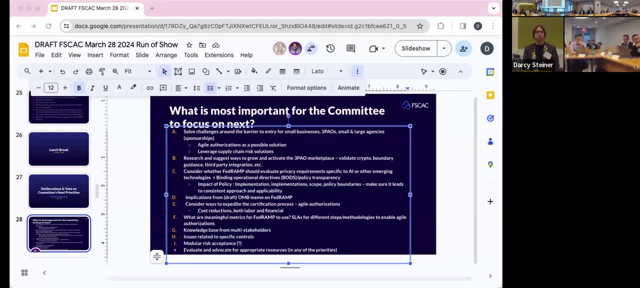 in this. that's where she, that just seems to be secret to be secret to be secret. yeah, that seems to be effective to get it. yeah, that seems to be effective to get it. yeah, that seems to be effective to get it to a quick, at least to see if we're. 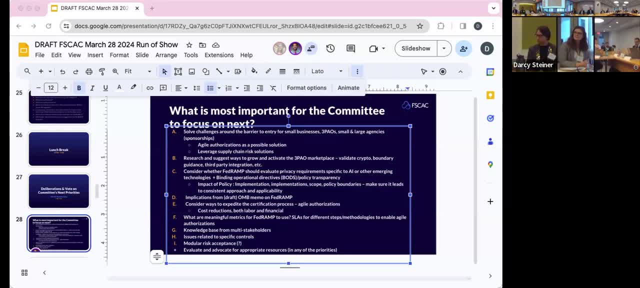 to a quick at least to see if we're to a quick at least to see if we're aligned or not. okay, yeah, aligned or not, okay, yeah, aligned or not. okay, yeah, we can definitely do that. okay, but we, we can definitely do that. okay, but we. 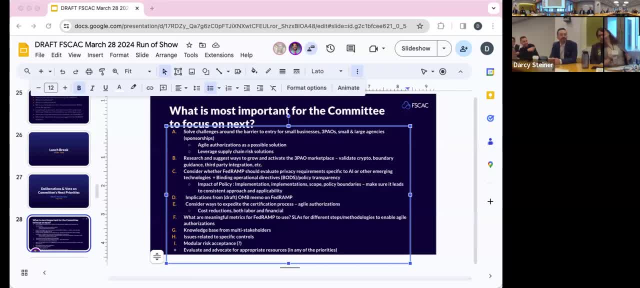 we can definitely do that, okay, but we need a motion to. all right, i'm going to go ahead and do a. all right, i'm going to go ahead and do a. all right, i'm going to go ahead and do a roll call, just uh. roll call, just uh. 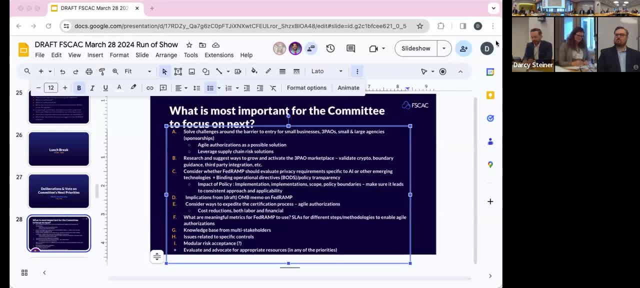 roll call, just uh, to make sure that we can close without, to make sure that we can close without, to make sure that we can close without. and how do you vote? and how do you vote? and how do you vote? uh support uh, daniel, how do you vote? 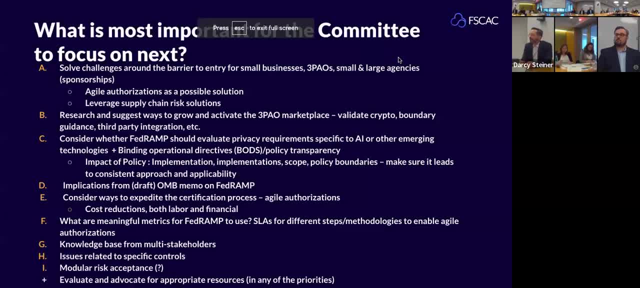 uh support uh daniel. how do you vote? uh support uh daniel. how do you vote? support, support, support uh michael support. uh michael support. uh michael support. uh john support. uh john support. uh john support. uh marcy support. uh marcy support. uh marcy support. franco support matt support bo. 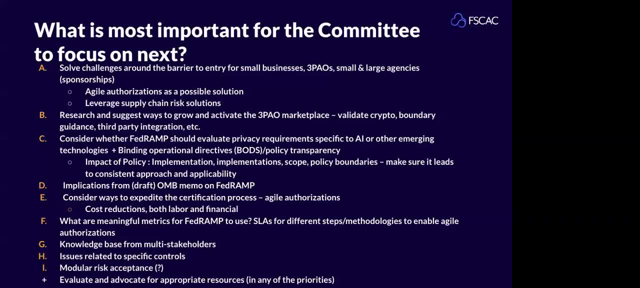 franco support. matt support bo. franco support. matt support, support, support, support. nomin jackie support bill. jackie support bill. jackie support bill and joshua support and joshua support and joshua support. great, great, well. thank you all um the great, great well, thank you all um the. 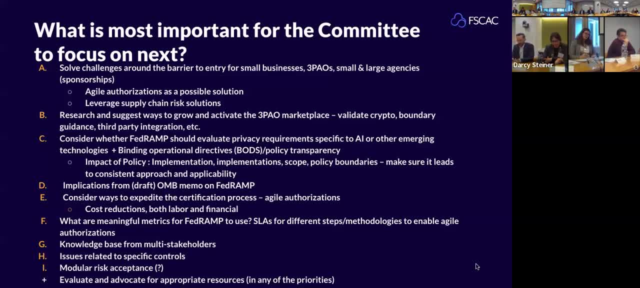 great, great well, thank you all. um the escat escat escat staff will get to work on um staff will get to work on um staff will get to work on um uh uh, uh. you know gathering some additional. you know gathering some additional. you know gathering some additional background. uh, for our next uh meeting. 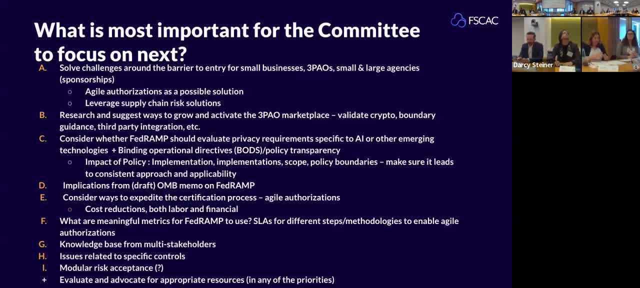 background: uh for our next uh meeting. background: uh for our next uh meeting: uh to help you uh come to a conclusion. uh to help you. uh come to a conclusion. uh to help you. uh come to a conclusion on which of these areas. on which of these areas? 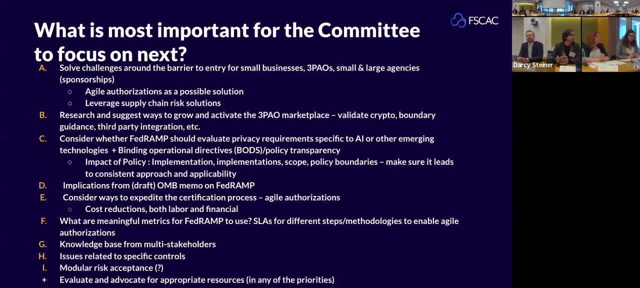 on which of these areas would be more beneficial for the use would be more beneficial for the use, would be more beneficial for the use of that time, of that time, of that time. um, um, um and uh. our next steps, uh will be to. and uh, our next steps, uh will be to. 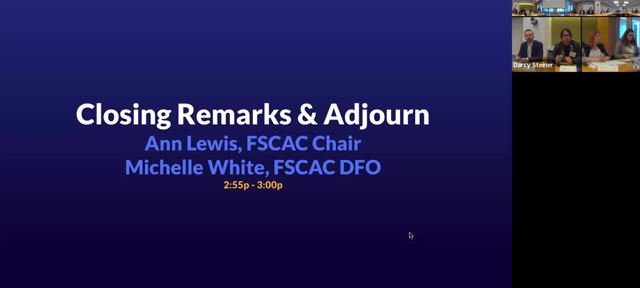 and uh, our next steps, uh, will be to develop an agenda item to set up, develop an agenda item to set up, develop an agenda item to set up, um, and with that, we have our closing rumors. we have our closing rumors, we have our closing rumors. right um, ann, would you like to um go? 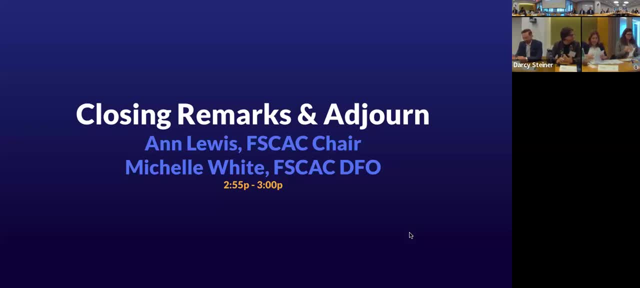 right? um ann, would you like to um go right? um ann, would you like to um go ahead and um ahead and um ahead and um start with them. start with them. start with them. um yeah, thanks, michelle, i it's possible. um yeah, thanks, michelle, i it's possible. 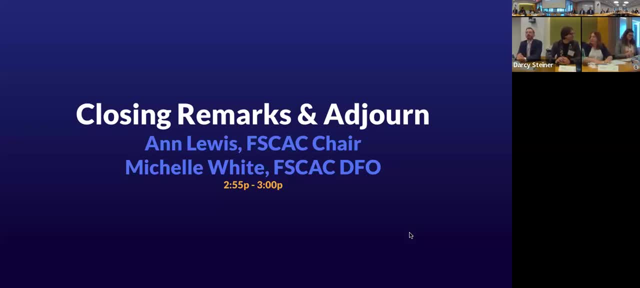 um, yeah, thanks, michelle, i it's possible, i have some points here, but i just i have some points here, but i just i have some points here, but i just wanted to say, wanted to say, wanted to say, um, this is a great discussion, i just. um, this is a great discussion, i just 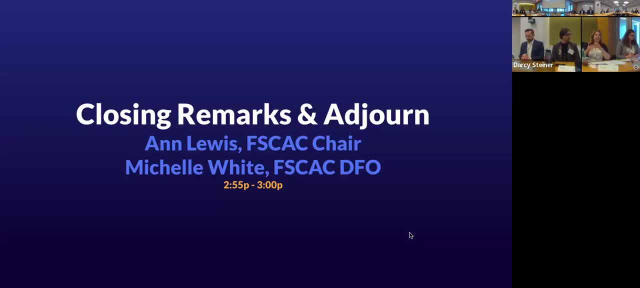 um, this is a great discussion. i just wanted to appreciate, wanted to appreciate, wanted to appreciate um how well we've represented agencies. um how well we've represented agencies, um how well we've represented agencies, cloud service providers, small cloud service providers, small cloud service providers, small businesses, 3dos, and had a really rich 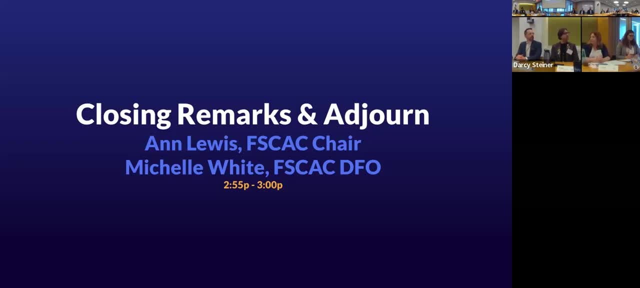 businesses 3dos and had a really rich businesses 3dos and had a really rich, rigorous discussion um the fact that we rigorous discussion um the fact that we rigorous discussion um the fact that we again have a list that's too long and we again have a list that's too long and we 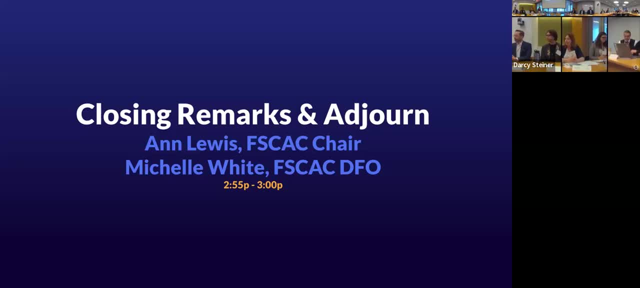 again have a list that's too long and we need to get more information on shows, need to get more information on shows, need to get more information on shows just at the table and um engage just at the table and um engage just at the table and um engage everyone this year. so i just wanted to. 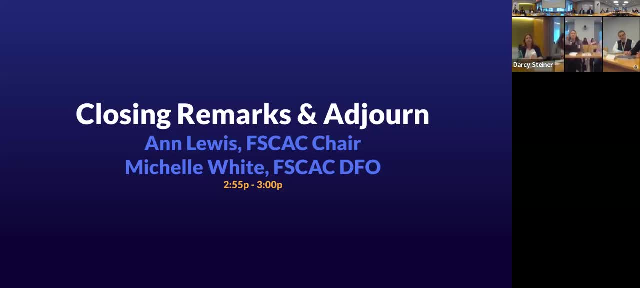 everyone this year, so i just wanted to everyone this year. so i just wanted to thank you all for the great discussion. thank you all for the great discussion. thank you all for the great discussion. we're looking forward to your meetings. we're looking forward to your meetings. 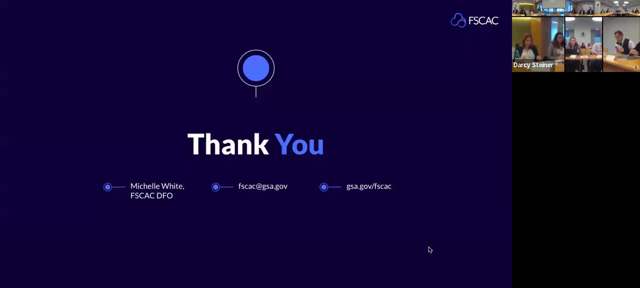 we're looking forward to your meetings. that was great well. thank you all for that was great well. thank you all for that was great well. thank you all for joining with that. i will go ahead and joining with that. i will go ahead and joining with that. i will go ahead and adjourn this meeting. thank you.